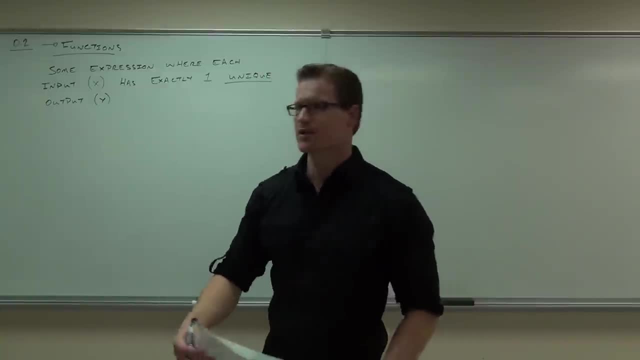 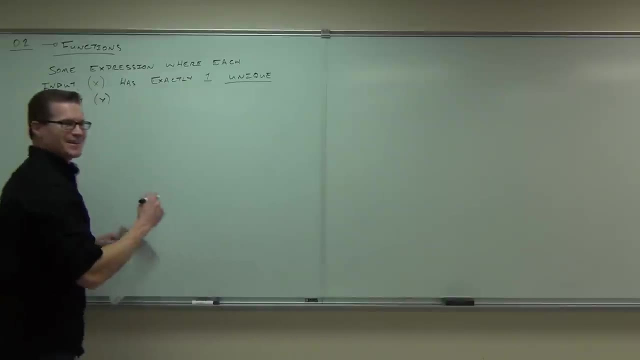 a lot of ways, though, We can represent with tables, graphs, formulas. One time I was fishing and I caught four fish and because I'm a math dork, I made a table table of it, And I was not able to see the table of it because you don't do that. Is that not normal? 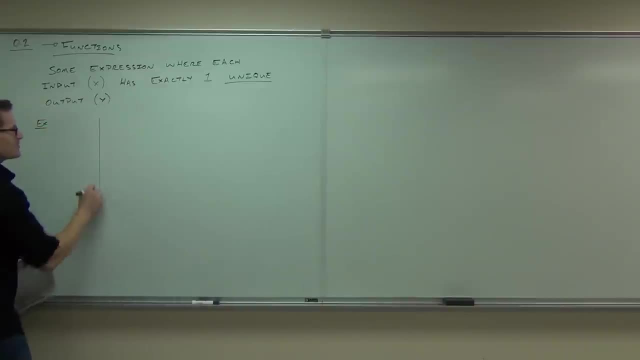 Anyway, Here's one example of a function, A very easy function. Here's my fishes. I think that's fish, Fish caught and the number of pounds that they were. So my first fish, second fish, third fish: I caught four that day. First one was 3.2 pounds, Not bad. Next, was 1.4., Then 2.8,, then 2.9. Then 3.4., Then 1.8., Then 1.2., Then 1.2., Then 1.4., Then 1.3. Then. 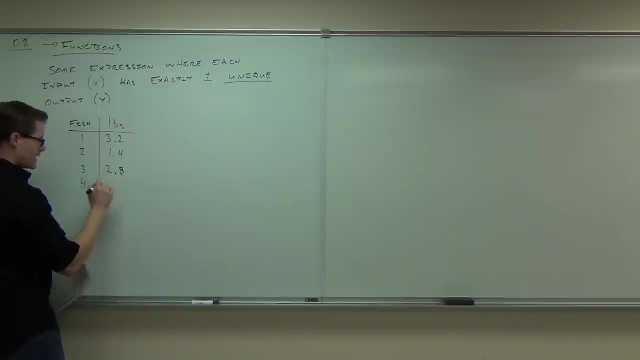 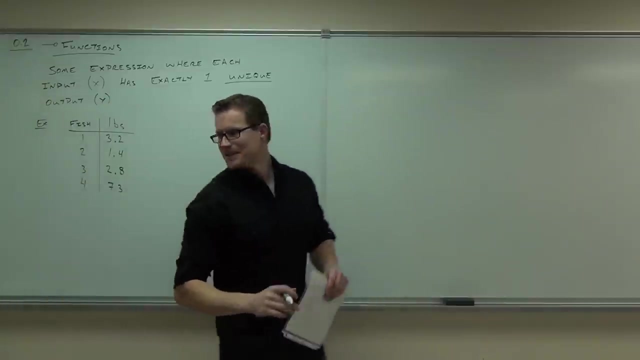 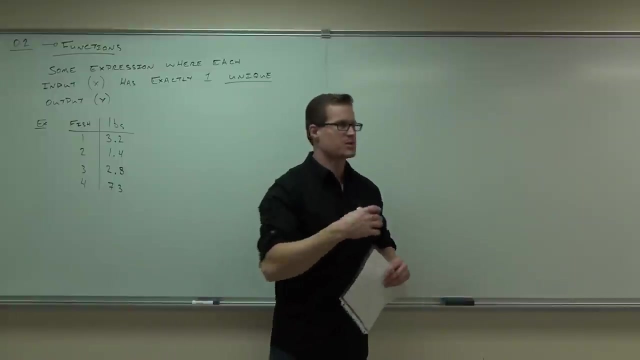 than 2.8, and then I caught a massive bass for 7.3.. Good day, Good day. Threw them all back. Firstly, let's define what the inputs and outputs are for this particular well, this one, we're going. 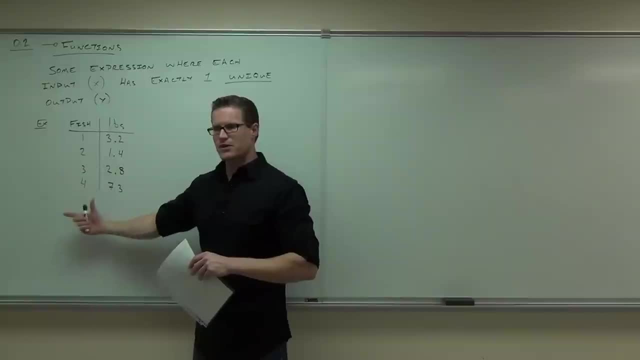 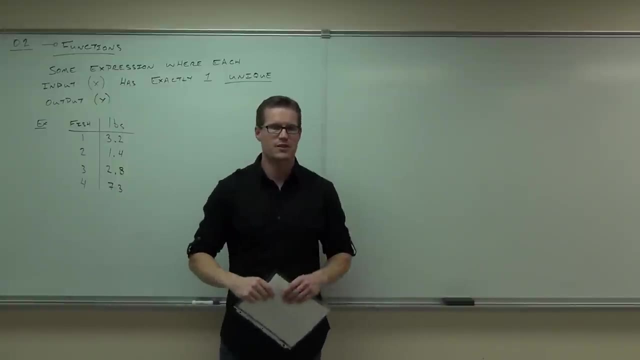 to see if it's a function in just a second. Firstly, my inputs are well the fish that I caught. in this instance, The outputs would be well, they're weights. when I weighed them, because the scale would be like my function, right, I put my first fish on there. it gave me a weight. 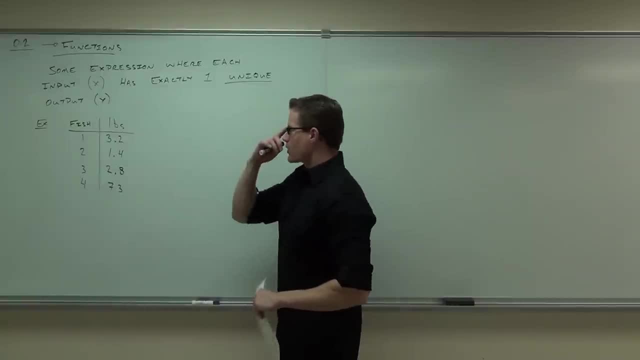 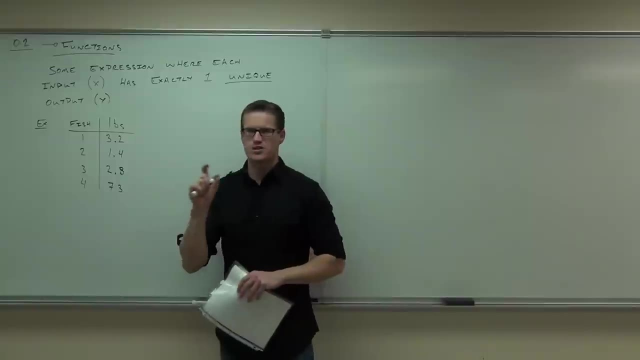 Put my second fish on there, it gave me a weight. Now the question is: is it a function? Is it a function? Does each input, does each fish have one specific weight? Yeah, Okay, You know what I need to erase something right here? One, exactly one, not unique, but one output, Unique output. 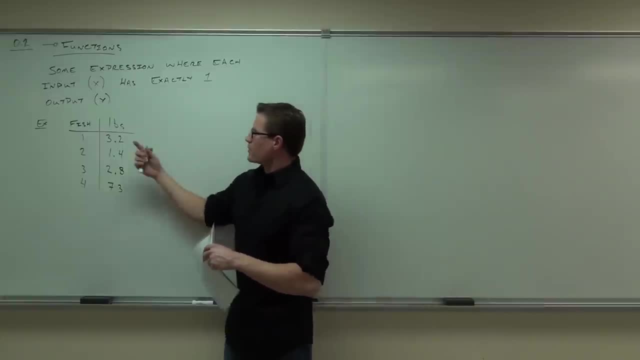 would be a one-to-one function, and we're not there yet. So when we say it has one output, I mean that I don't have fish number one weighed 3.2 pounds and 4.7 pounds, Because you'd say: 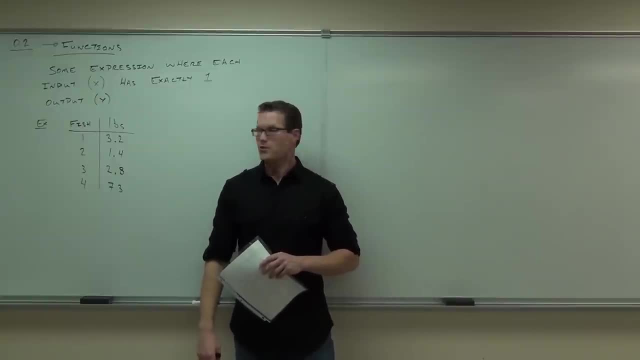 how much did your first fish weigh? I'd say 3.8 or 4,, 3.2 or 4.7.. Would that make sense to you? Well, no, seriously, how much did your fish weigh? 3.2 or 4.7.. That doesn't make any sense, You're. 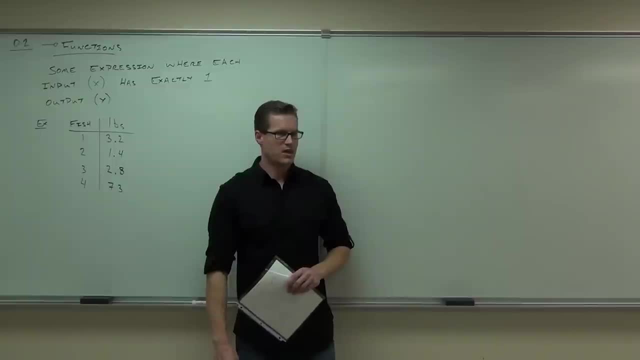 giving me two weights for the same fish. Does that make sense to you? Would that make sense If you ask me that question? how much did your first fish weigh? And I said, oh well, either 3.2 or 4.7.. 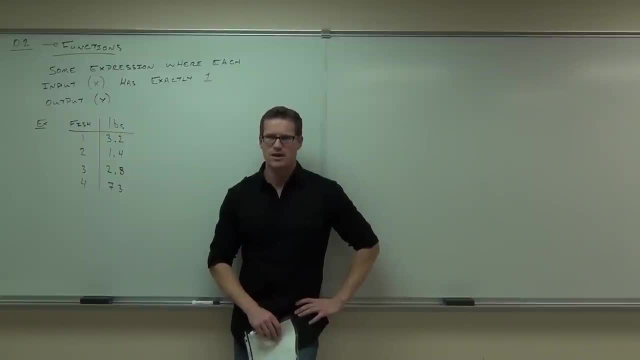 You say: aren't we talking about your first fish? Yes, we are 3.2 or 4.7.. You're like, well, if I'm having dinner with you tonight, I need to know if I'm going to be hungry at 3.2 pounds or if I'm 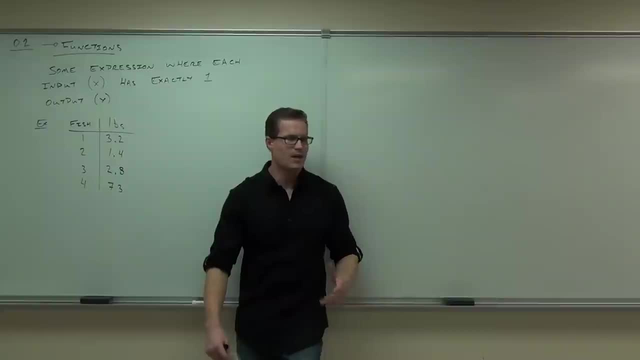 going to be satisfied at 4.7.. I go 3.2 or 4.7.. It doesn't make any sense, right? I have to give you a specific weight for that one fish. That's what a function does. It says, if you say fish number one. 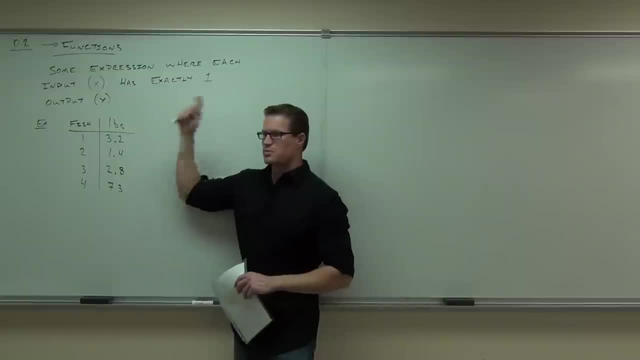 you're talking about one specific weight. okay, Maybe I should say the word specific output, not unique, Because one unique output we will be talking about one-to-one in just a little bit. How about number two? Does number two give me? 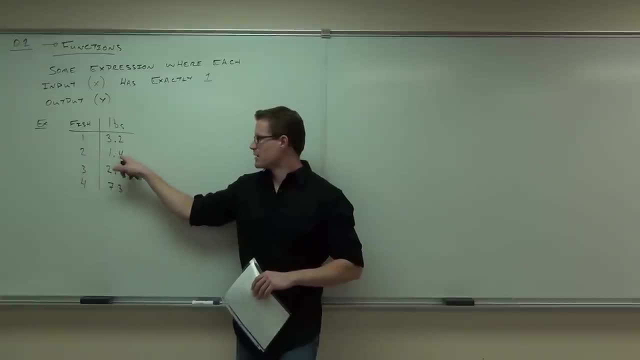 give me out just one weight. Yeah, it doesn't say 1.4, and then something else over here. That would not be a function. So this thing is a function. Any, any fish that I have, it has one specific weight that we're talking about. If I did this, 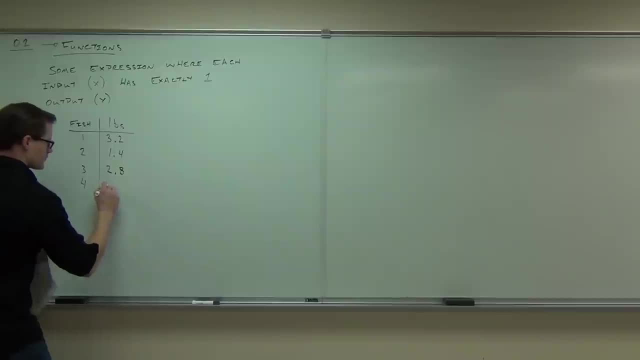 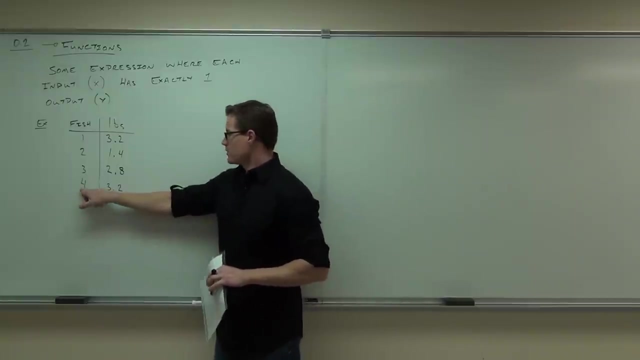 would it still be a function? The answer is yeah. Yeah, it would be a function. This way, this fish four weighed 3.2 pounds, not something else. It doesn't matter that these things are the same. That can happen. 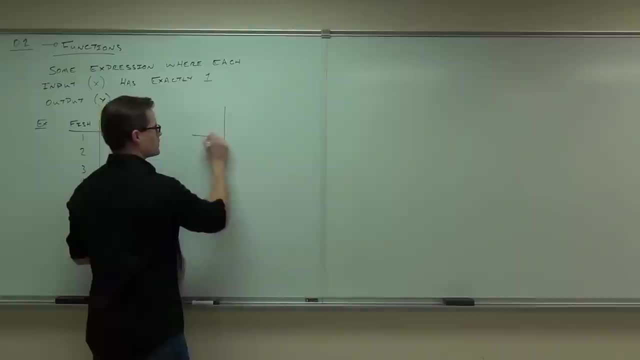 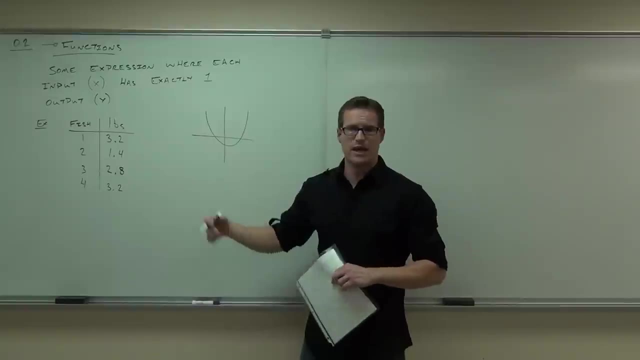 Let me give you a, for instance, as far as a graph goes, That, right, there has the same output at a at a several different spots. right That that would be some sort of an x squared. It says: if I'm at this point or this point, I still have the same exact output. That that's okay, This is. 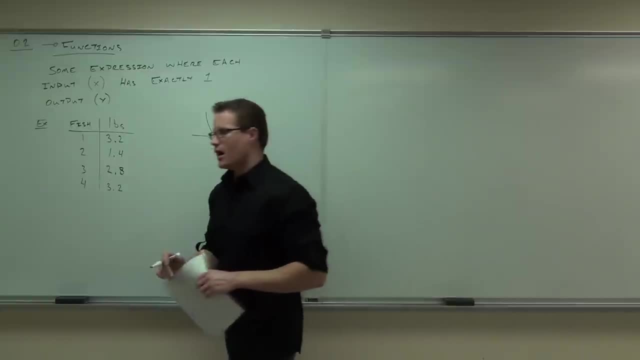 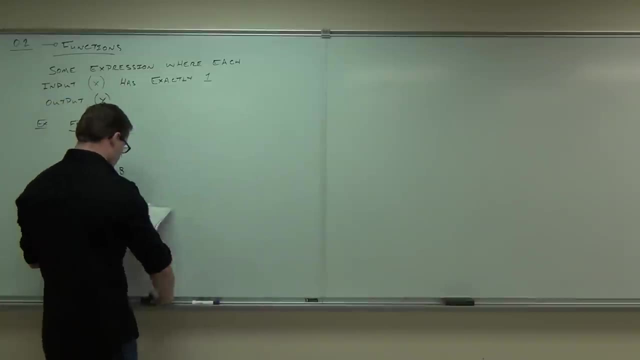 still a function. We're going to talk about vertical line test too. It's a function. It wouldn't be a one-to-one function. It wouldn't pass a horizontal line test, but it would be a function. We can also talk about functions, really. 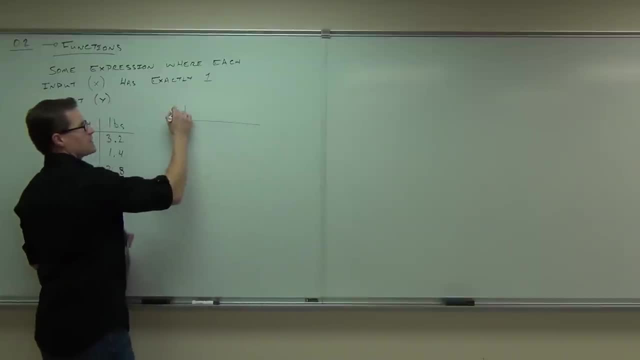 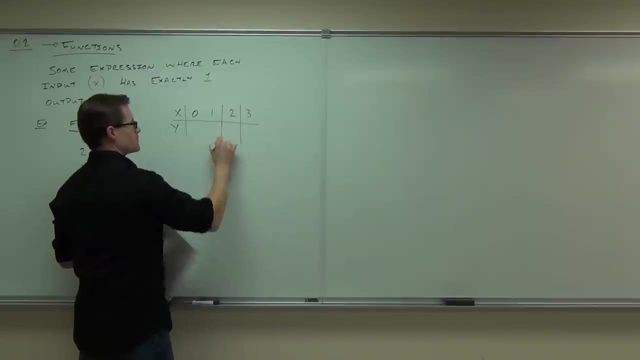 because we don't see fish caught. normally We see some sort of function like this: especially if you're doing any mathematical modeling, you might see this: where you have a set of inputs or x's, You got a set of output, outputs. That thing would be a function: Every one of our inputs. 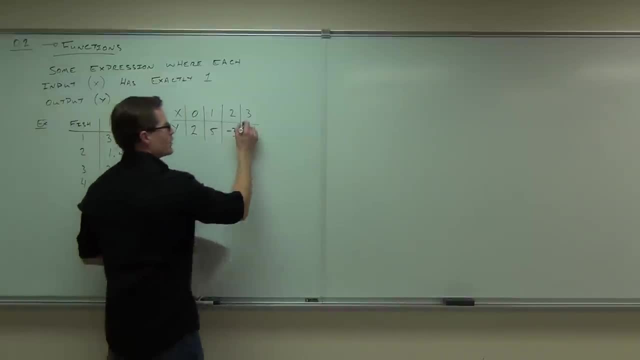 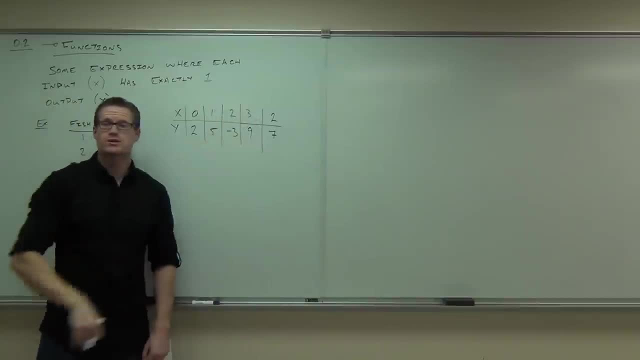 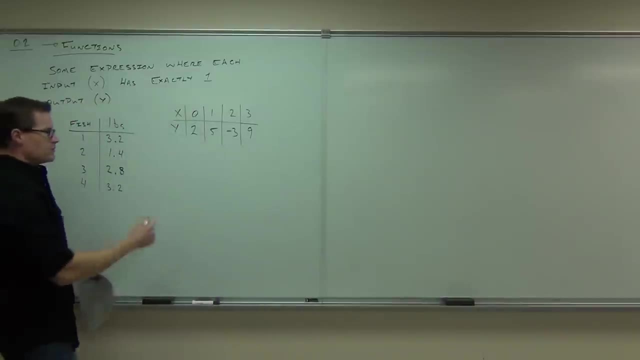 No, No. If your inputs are repeated with different outputs, well then you don't have a function there. So that would be a no bueno. Sometimes you actually have formulas, too, that are functions. This is a function. What is that? by the way, 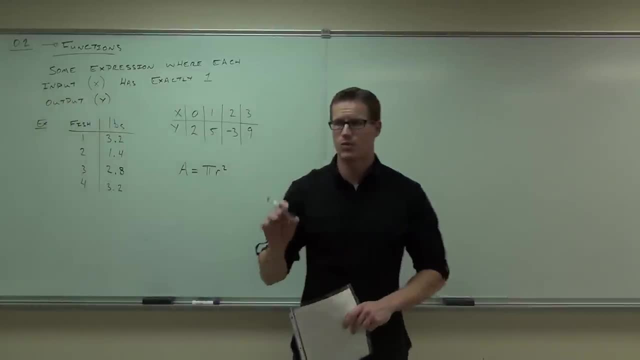 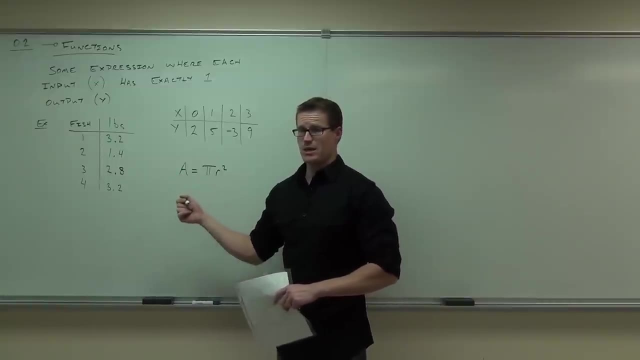 Area Sure, And it's a function, because if you give me a radius, it's going to give me out one area, isn't it? So our area depends on the radius you have for your circle. It's not like I say you have a radius. 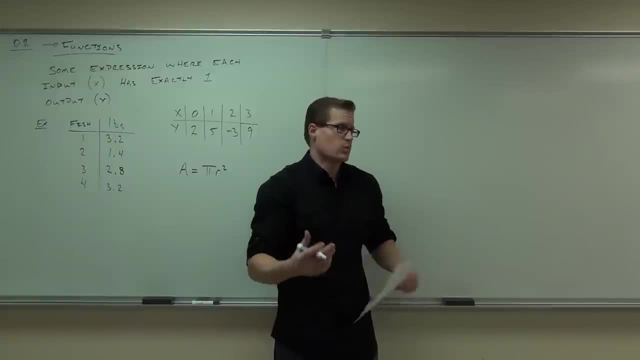 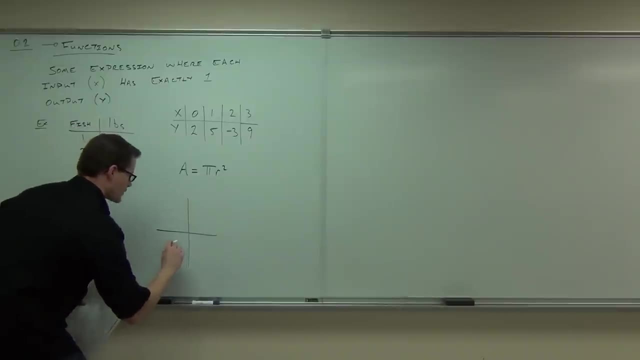 a radius of three. what's your area? And you give me two different answers. That wouldn't make any sense. It wouldn't be a function. The formula would fail. Also, we can have some graphs Graphically. if we did something like that, we can have, we can represent them lots of different ways. 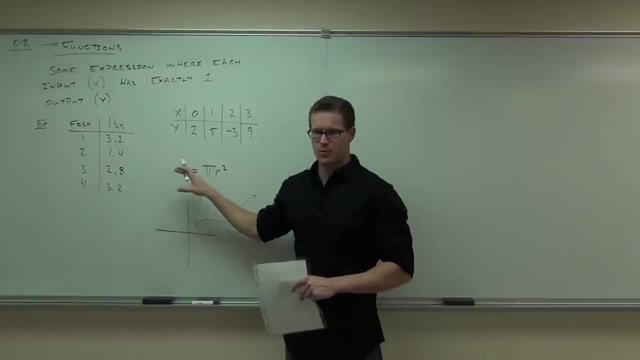 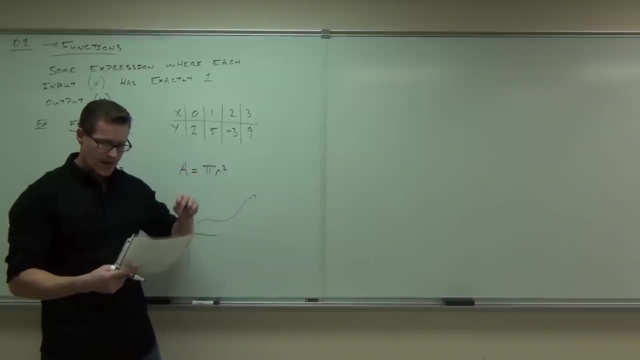 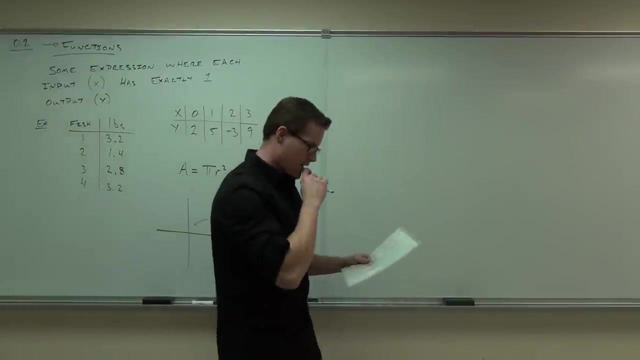 Basic tables here, formulas, which we spend most of our time in, formulas and graphs. That's another way we represent functions. Just one note: functions have to have only one output for each input. That's the key thing. I hope that you got that from this. Now one more thing about this one. 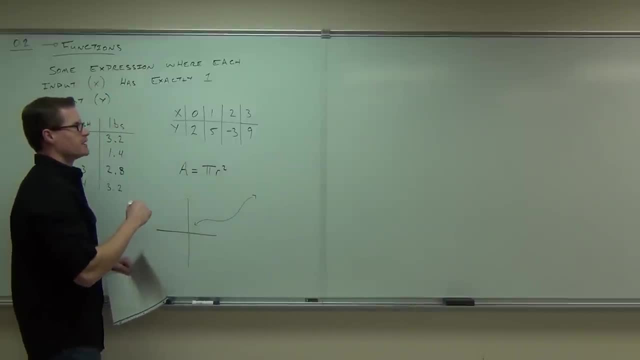 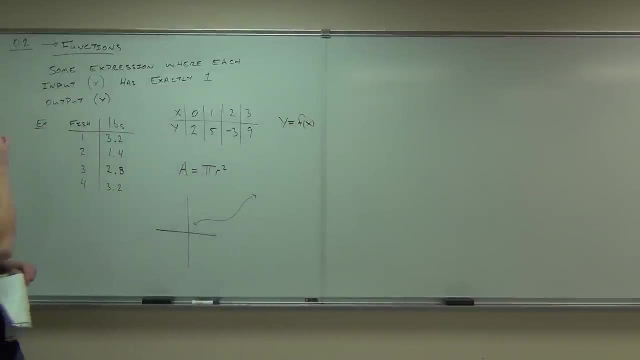 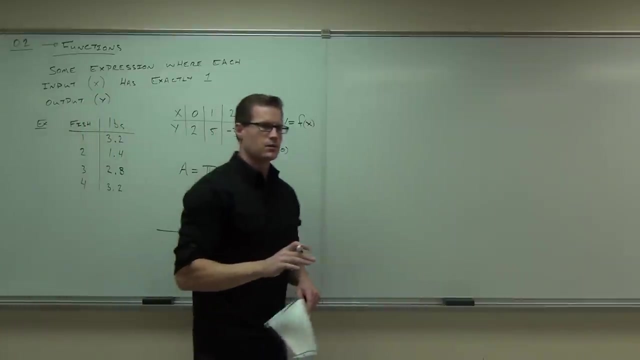 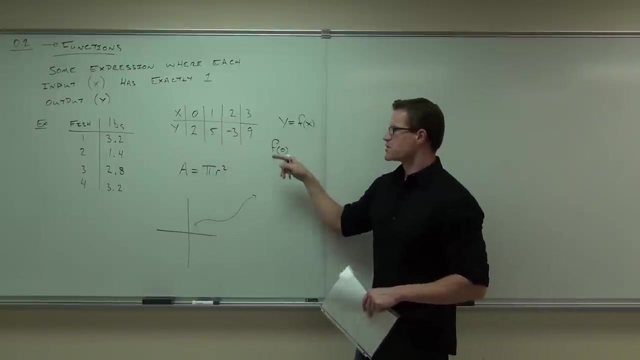 Let's say we change it just a bit and we say y equals f of x. Could you find f of zero? What would that mean to do? It would mean, if y is f of x, if it says y is a function of x and I'm asking for f of zero. 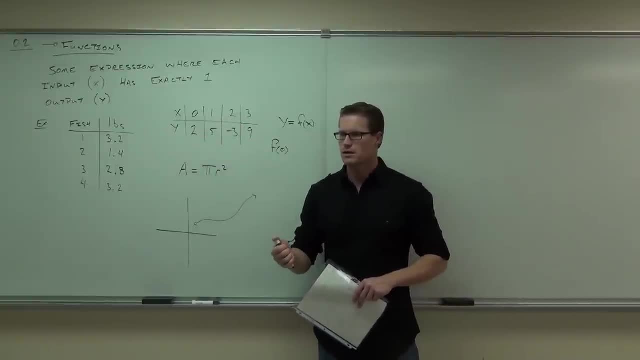 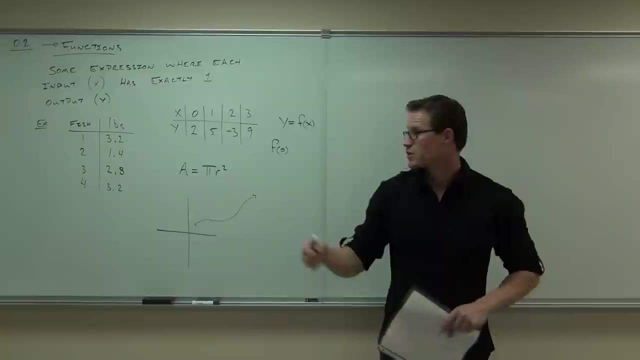 can you tell me what is f of zero, in this case Two? Okay, it is. how much Two, Two? because it says you go over to the input of zero. you look up the output for that particular input. So here it says: find your input. remember this is f of x, right? So go to your x, go to zero. tell me what the output is. 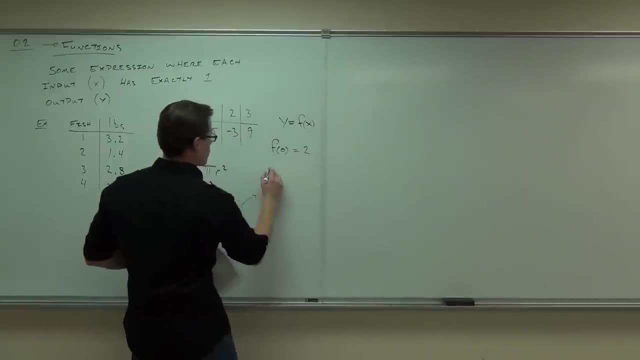 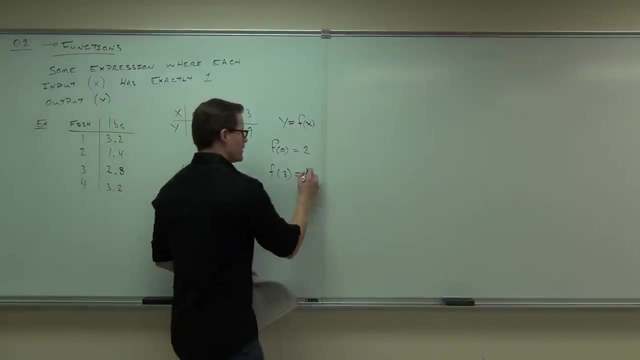 Oh, it's two. How about f of three? What's f of three? everybody? Nine, That wasn't everybody, but I'll take it. Yeah, it just says: you go to your input of three. you find out what that output was. 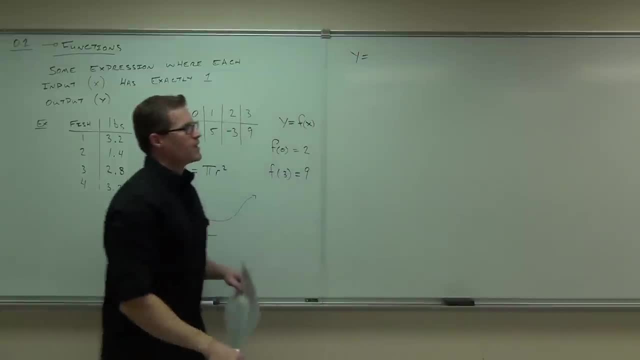 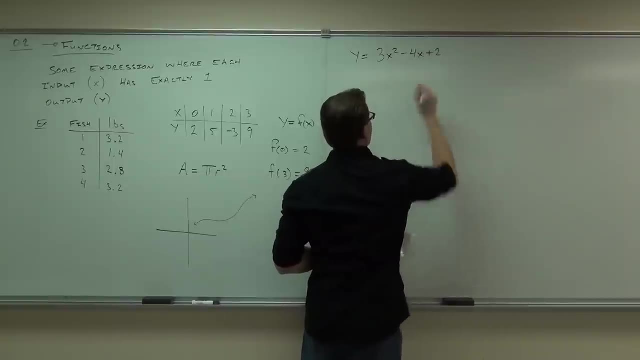 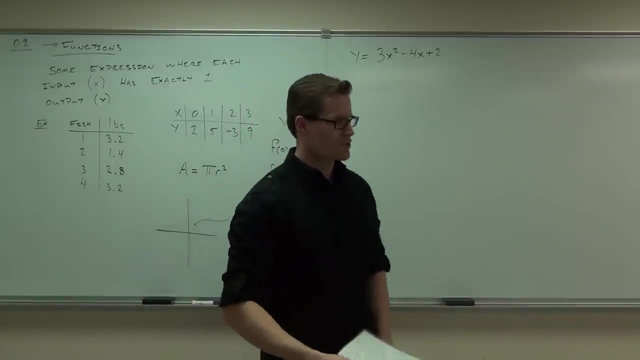 Typically we'll use this in this type of situation where you have some sort of equation: y equals 3x squared minus 4x plus 2.. The y equals thing isn't always the best for us to represent a function. The reason is is because in this class we're going to look at a lot of different functions at once and you want to be able to distinguish between them. 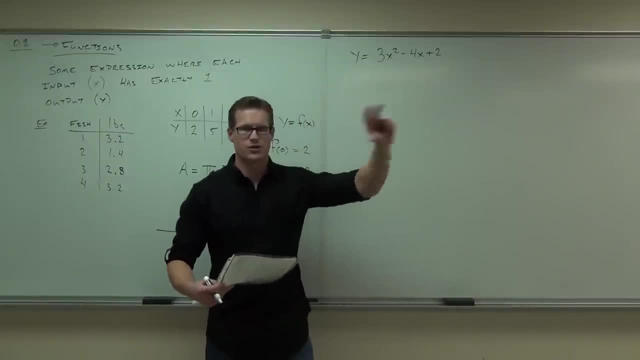 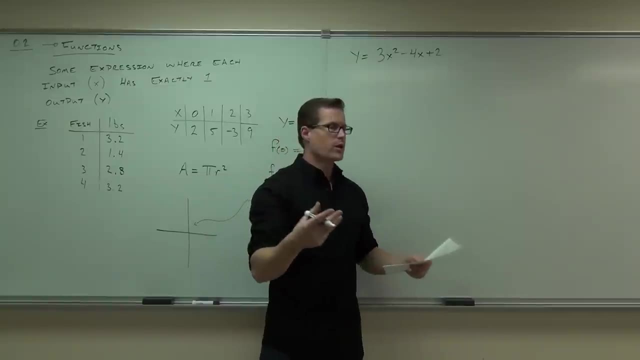 If I have just y equals a function, then y equals another function. y equals another function and I say, look at the function y. you're going to be like there's three of them. which one are you talking about? We often use this type of notation to distinguish between them. 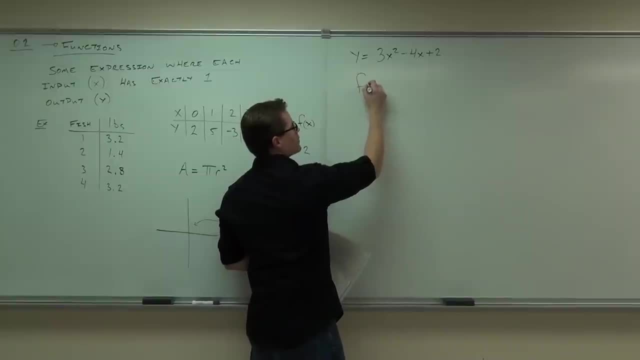 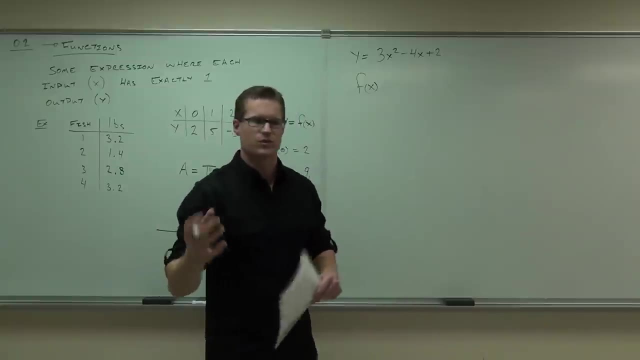 So if I said instead of y equals f of x, I'm sorry, y equals that function. I want f of x or g of x or h of x. That way we can distinguish between those graphs and those formulas And these equations. 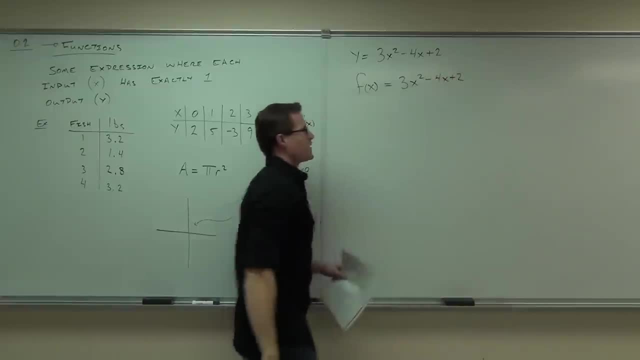 Also, what it lets us do is, if I ask you to plug in a number, it will tell you inherently what number you plugged in. For instance, if I say for you: here can you find me f of 0? Well, what does f of 0 do? 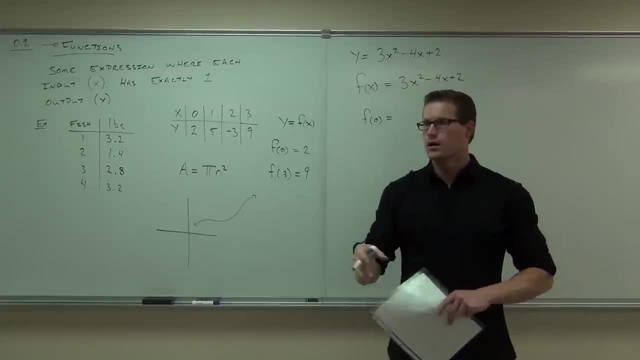 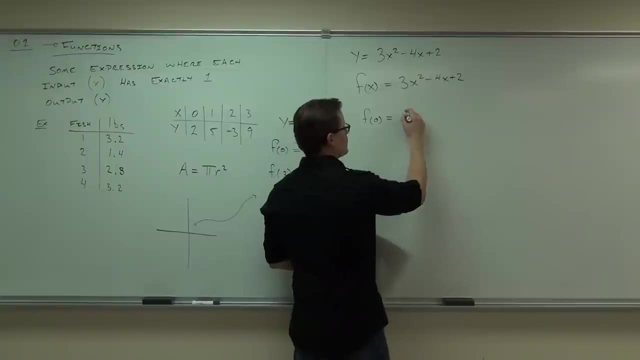 What's that supposed to do for you? It gives you the y-axis. Oh, it's supposed to plug in 0 and find out what the output is. Can you plug in 0? here You have 2.. So you plug in 0,, 0, yeah, you get the 2.. 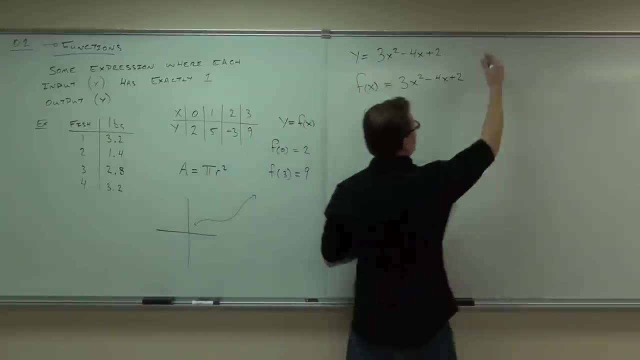 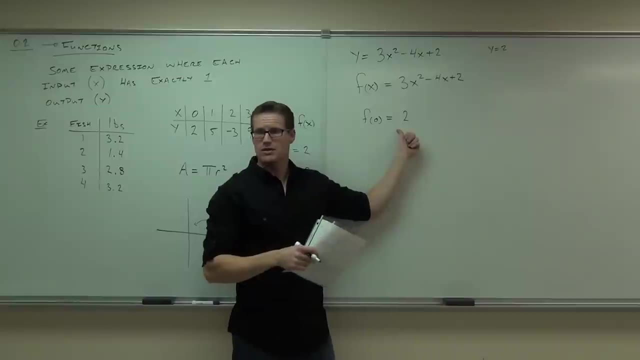 What's nice about this is, if you plug in 2 from this one, well, you're going to get y equals 2.. But does this tell you what you plugged in to get the 2?? No, Does this one tell you what you plugged in to get the 2?? 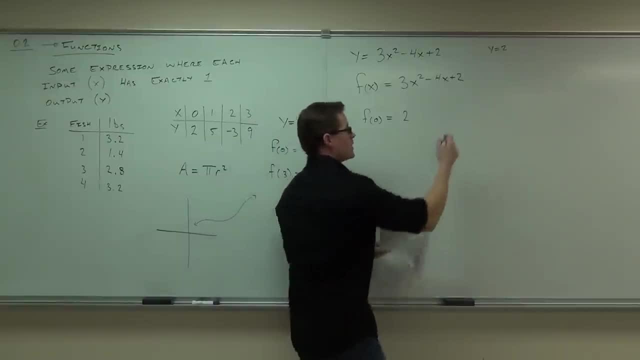 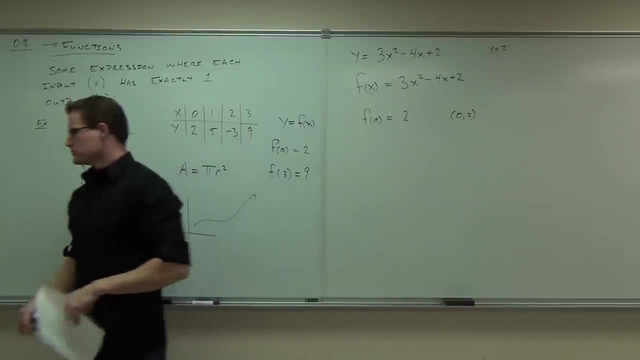 Yeah, This actually will give you a coordinate point. It will say: you plugged in 0,, you got out 2.. And that's kind of nice. This is one other reason why we use that function notation. Let's go back to those graphs too. 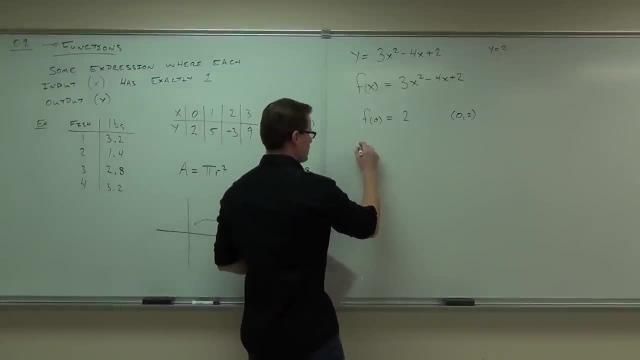 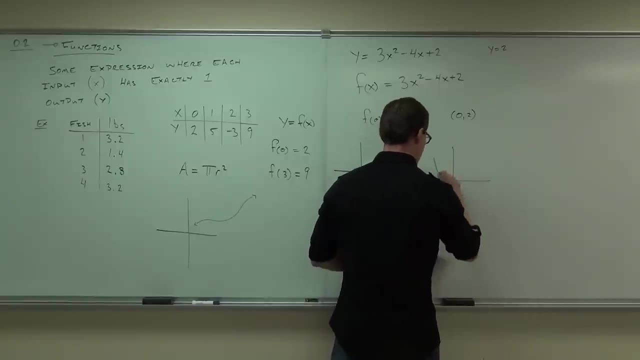 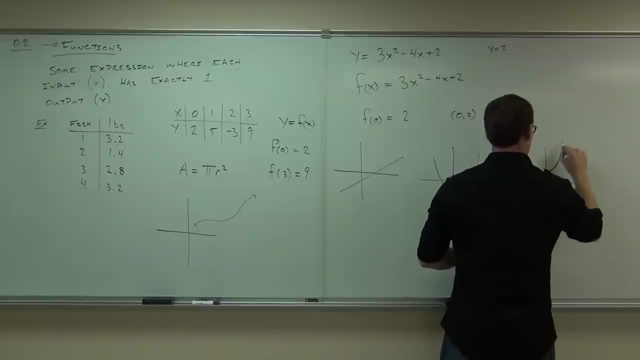 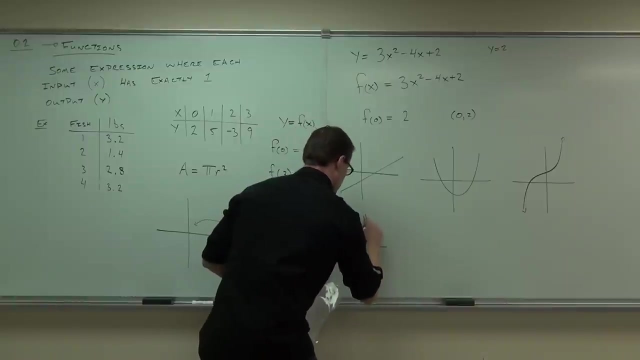 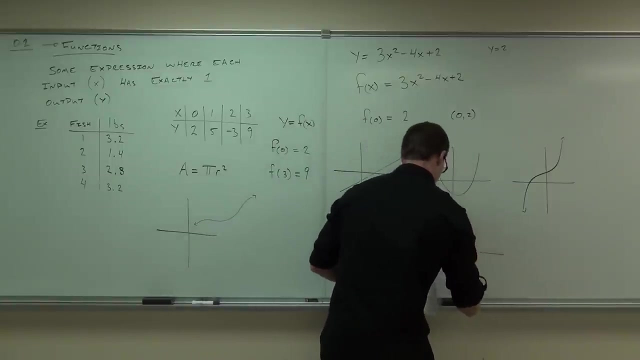 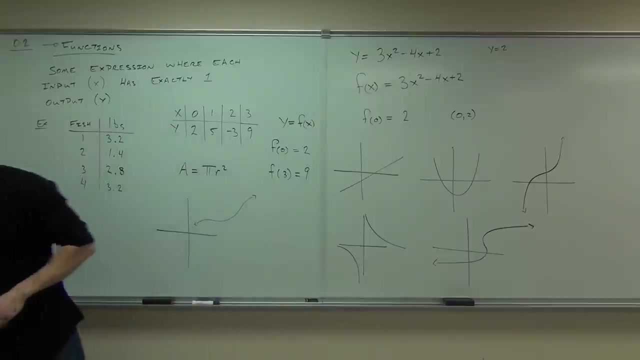 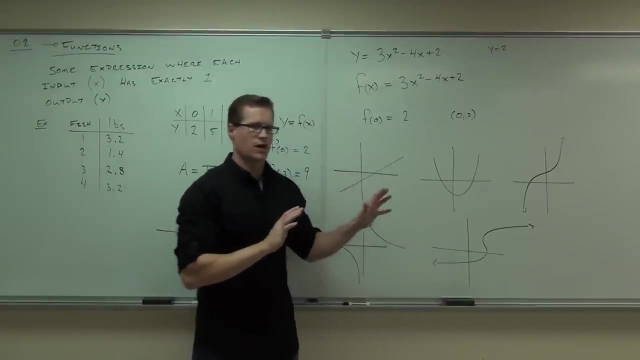 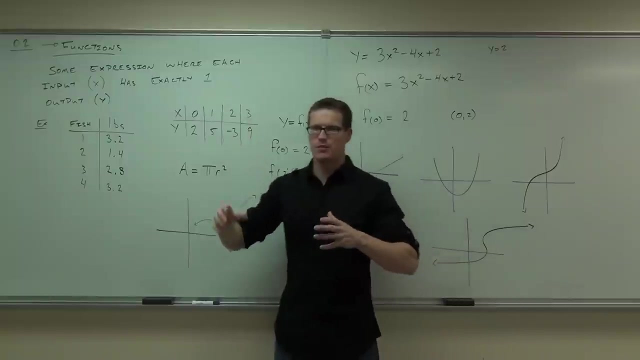 Can you tell what is a function just by looking at the graph? So, for instance, For instance, can you tell me whether these things are functions or not just by looking at them? We know we can tell with tables, right, Because if we have an input repeated with a different output, well that says it right. 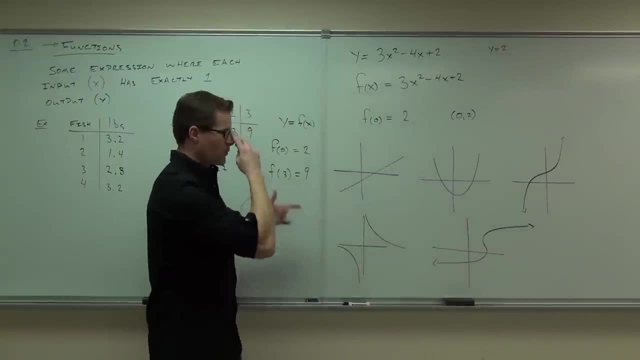 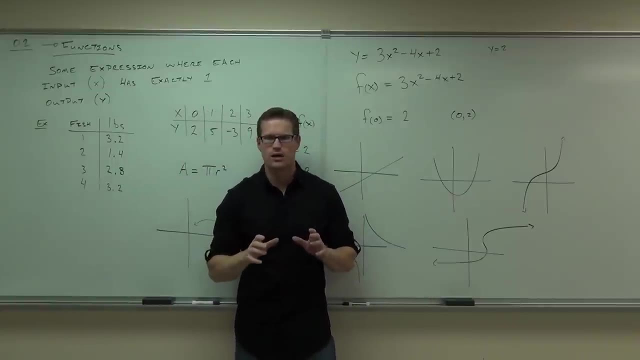 there We're going to be able to tell formulaically in just a little bit, But right here just biographically, what's that thing called where you test a line to see whether or not it is a function or not- Vertical line- 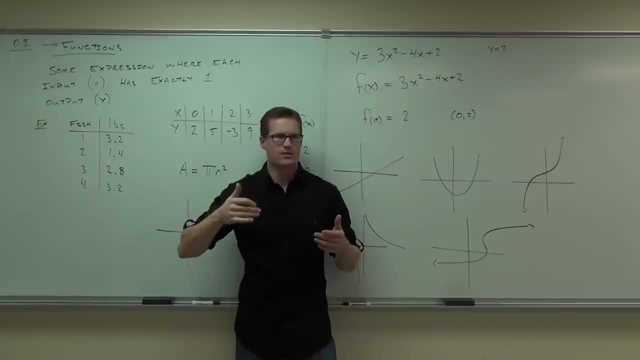 Vertical line: Yeah, we can have a vertical line test. Can you imagine? Bless you. Wow, that was a powerful one. It was like a sneeze grenade going off. Sneeze grenade. That would be so gross, So disgusting. 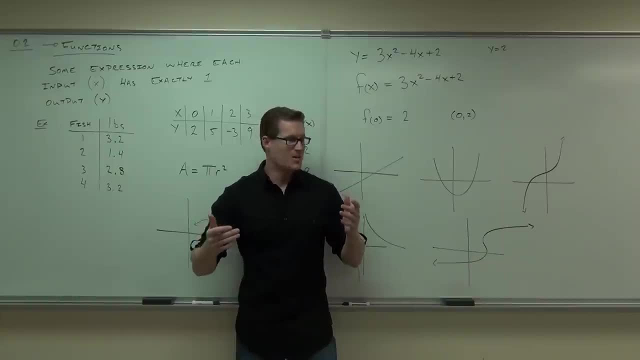 That's where my mind is right now. OK, So if you imagine every vertical line, it's supposed to touch your graph at only one spot, if it touches at all. So is this thing a function? Yeah, Yeah, For sure. 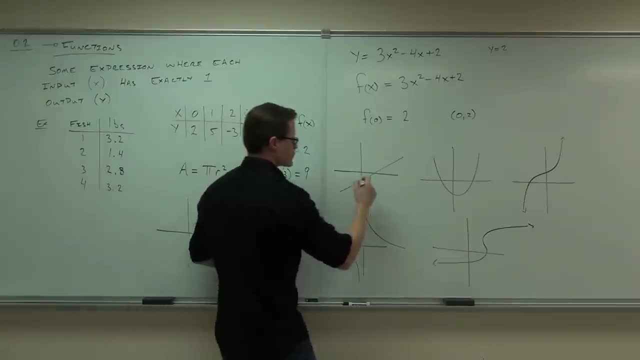 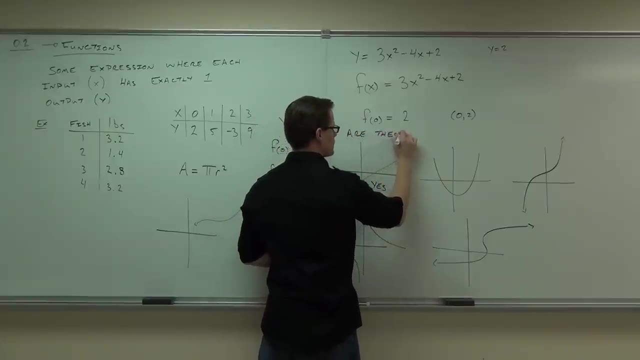 Every vertical line hits this diagonal at only one spot. So yeah, this is a function. How about that one? Is that a function? Yeah, Yeah, Parabolas are basic functions. Every vertical line hits this. Is it a one-to-one function? 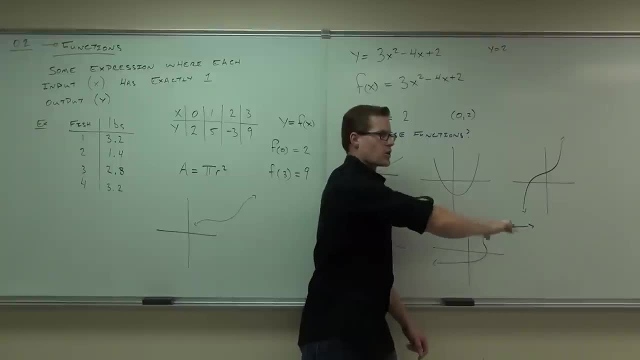 Do you know that? No, No, One-to-one function would be the horizontal line test saying that every incoming line has one unique output. It says it doesn't happen again. This is not one-to-one, but it is certainly a function. 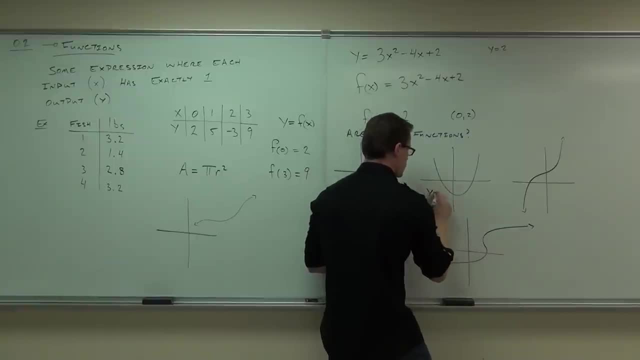 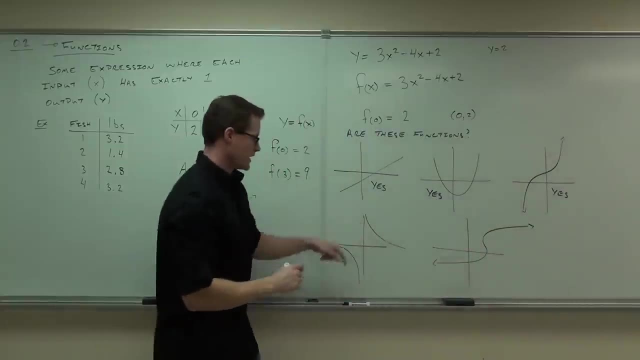 How about this one? Is this a function? Yeah, Yeah, sure. Now what about? this is an interesting case. What about this one? Is this a function? Yeah, Yeah, No. Does every vertical line hit the graph at it most once? 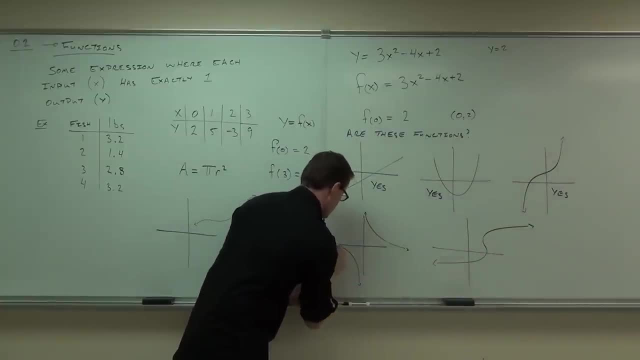 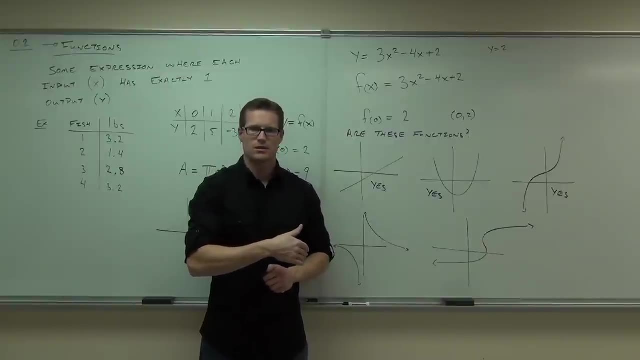 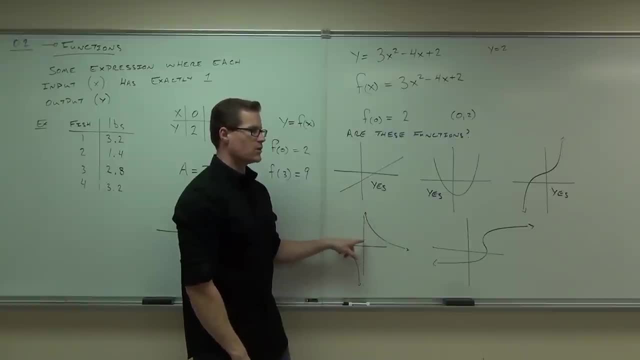 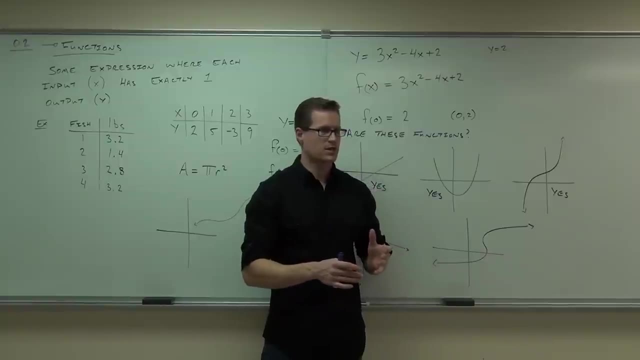 Why Don't you have to have something at this point? zero? And the answer's no. Not every input has to have an output, but if it does, it only happens once. Do you see the difference there? This doesn't have an output, it's undefined zero. 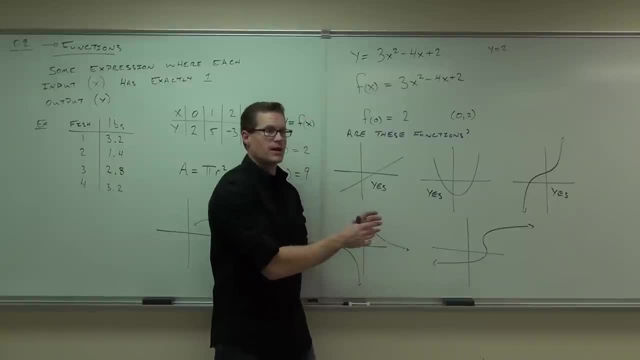 This would be like one over X. But if it is defined, then that definition has to be one exact point to be a function. So, yeah, this is still a function. How about this one? No, No, This fails it, because if you plug in this point, you actually get one, two, three. 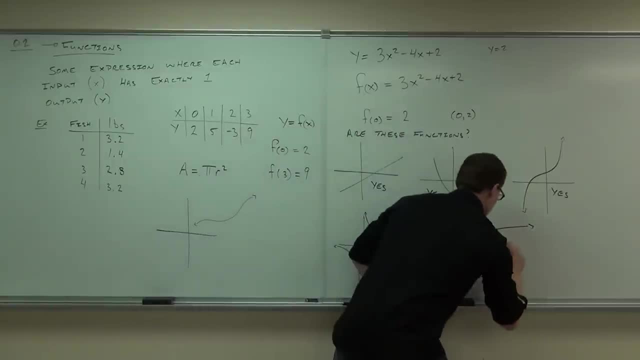 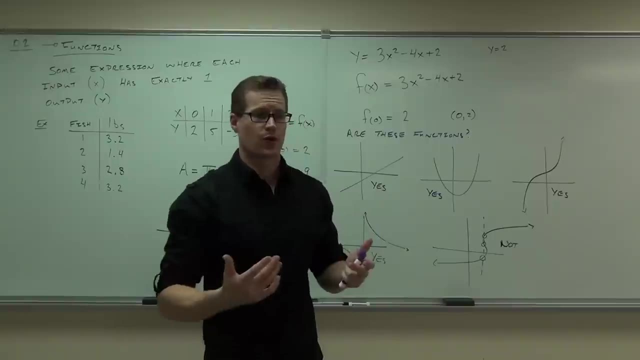 three points out and we can't deal with that. So this is not a function, So a vertical line test. verbally I'm not going to write it down because I know y'all know it says that you imagine every possible vertical line, that vertical 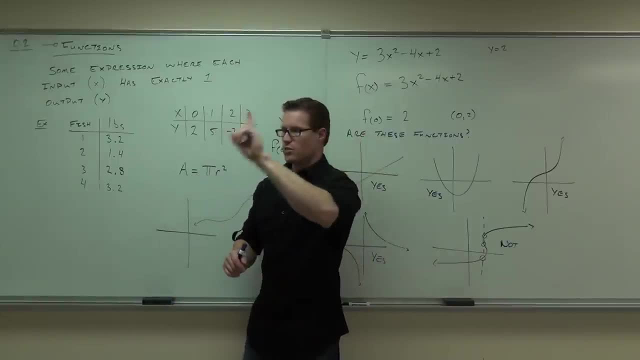 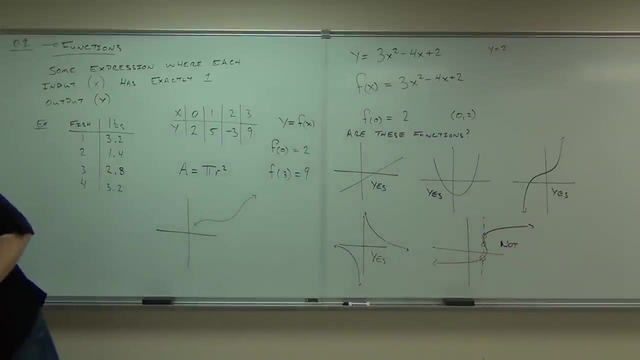 lines have to touch every point of that graph at most one spot. So touch the graph at most one spot. It can't ever cross over more than one spot. How many of you feel okay with our very quick introduction to functions? so far, You having fun yet 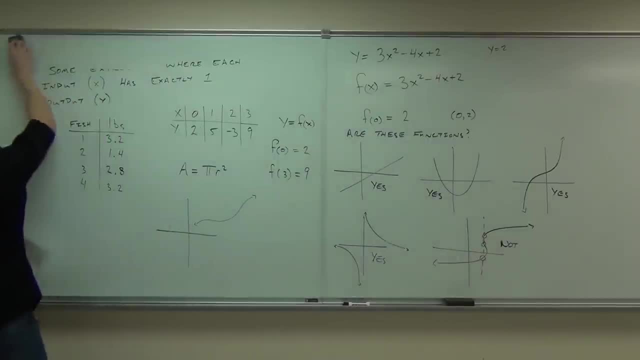 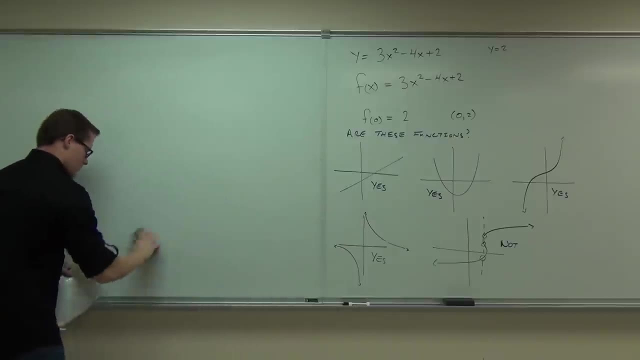 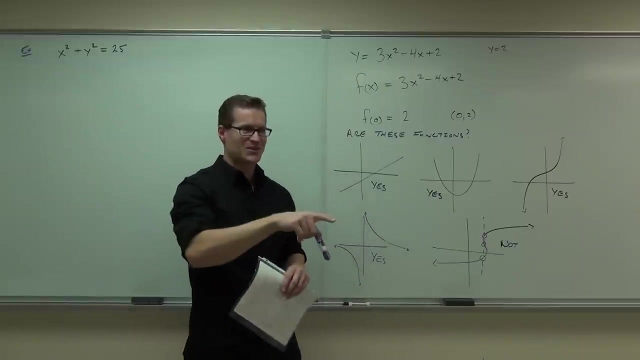 Enjoy, Enjoy, enjoy. There you go. Well, let's consider one more thing. What is that? Say it louder: Circle, Circle. Did y'all know it was a circle? Did you read the section on circles? I told you. 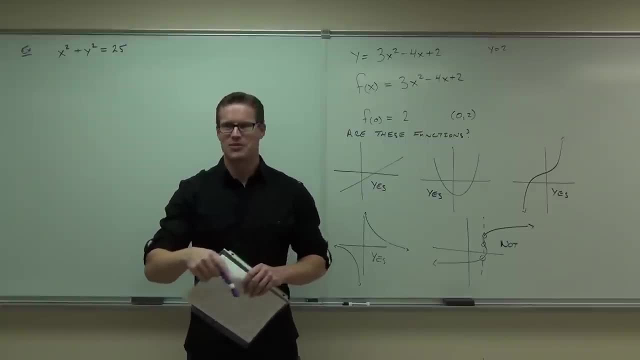 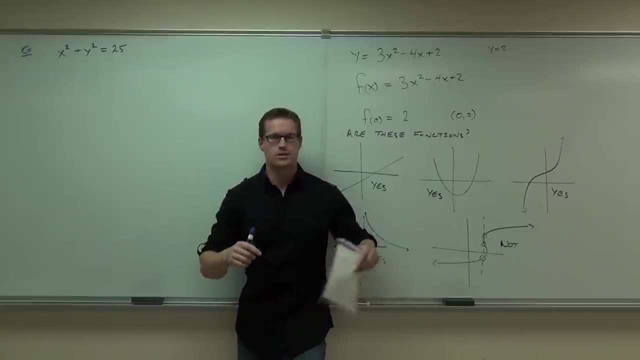 I said: read circles. right, Did you read circles? Hopefully you read circles. That's a circle. What's it centered at, Center of the origin? Very good, Zero, zero. The way you shift circles around. hopefully you remember this from your 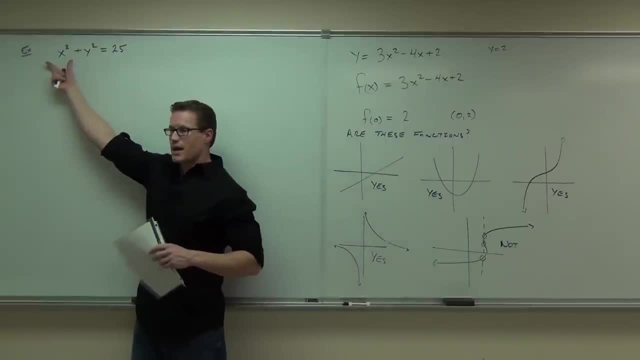 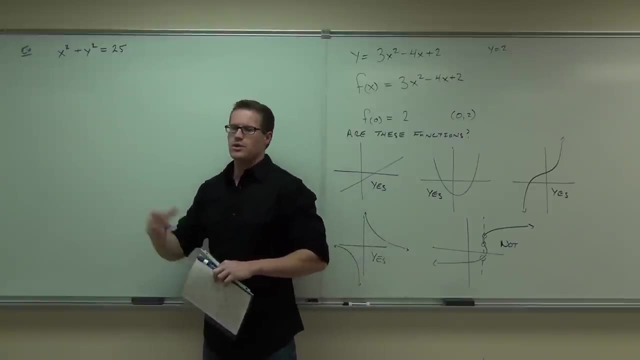 intermediate algebra days is. you have some parentheses in here, like x minus h and y plus k. That would shift that around. okay, What's your radius? Good, Because we know this is the radius, The radius squared, so our radius would be 5.. 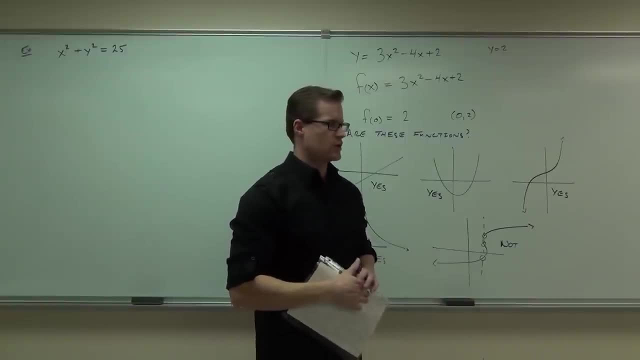 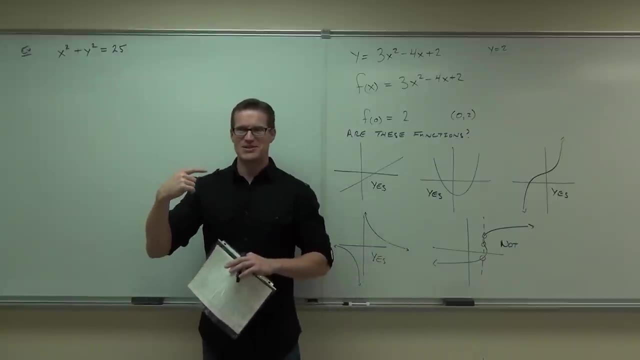 Is it a function? Is it a function, Why not? Well, yeah, I mean visually. we know it's a circle, right, That's circular reasoning, isn't it? Get it, Thanks, Where's my drums? It's a circle, so it's not going to pass the vertical line test. 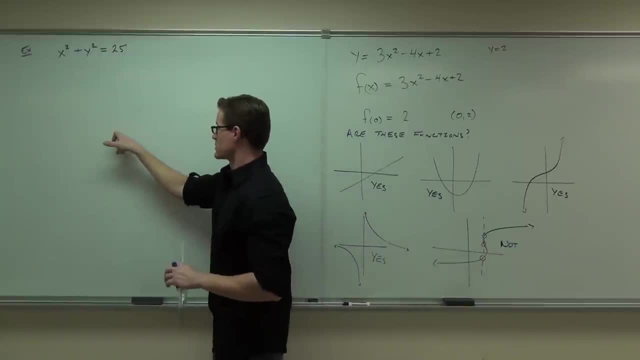 That's one way we define it. We actually graph this. It's a center, zero, zero, Radius of 5, it looks like this: It's certainly not going to pass the vertical line test, However. can you see it formulated? 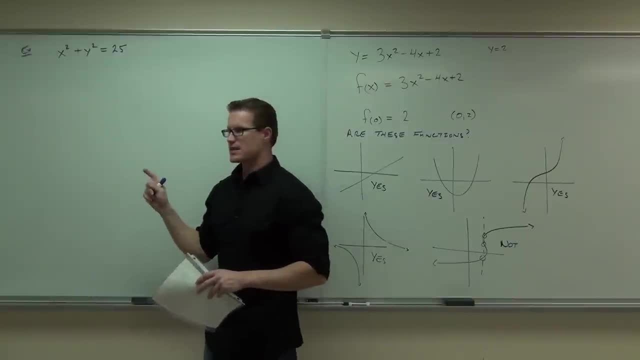 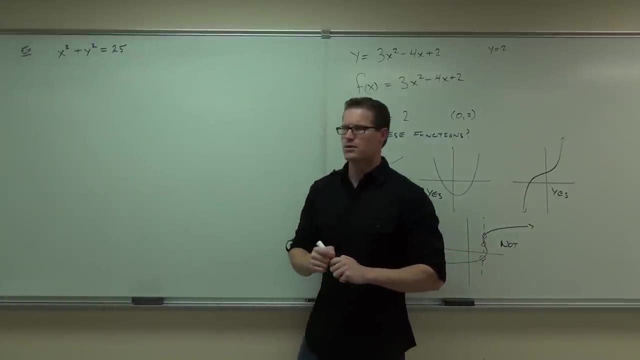 It does. It does Specifically, can you solve this for y and see that this is not a function? Let's try that. How would you solve this for y? What would you do first? Okay, so probably isolate the y, Get the x squared over there somehow. 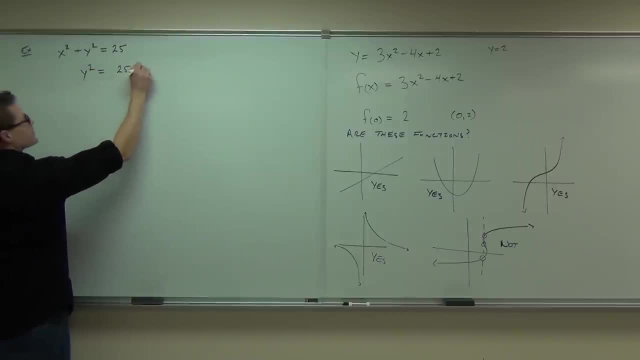 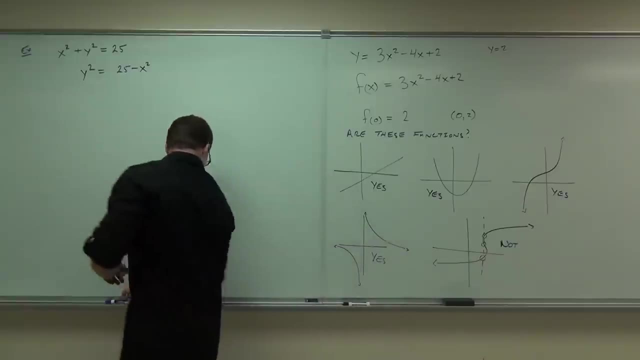 You know you're going to get: y squared equals 25 minus x squared, True. Now, y is not completely isolated. What would we have to do to get y all by itself? Let's do that. So, if we take the square root, of course that means both sides. 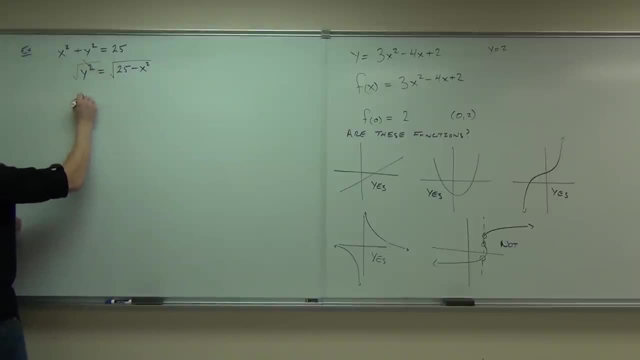 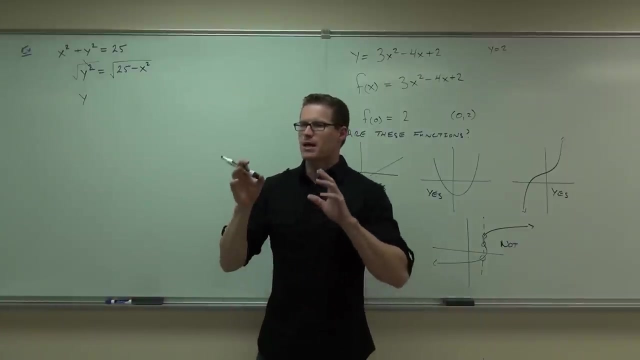 That's legal to do On the left-hand side. we get y On the right-hand side. tell me what I'm forgetting right here. Oh yeah, Every time you take a square root of something, you've got to have a plus or minus. 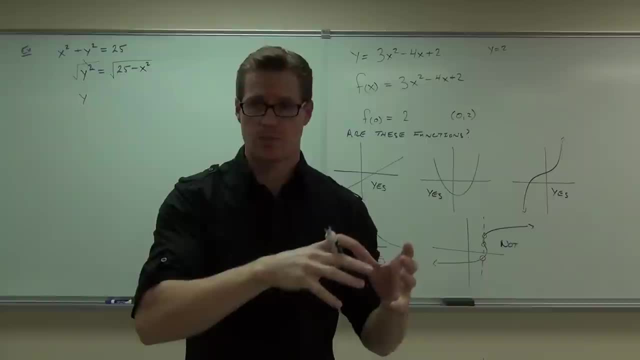 So if the square root's on your paper, no big deal. But if it's not there and you put it on your paper like we did up here, right, We didn't start with that square root, We introduced it to the problem. 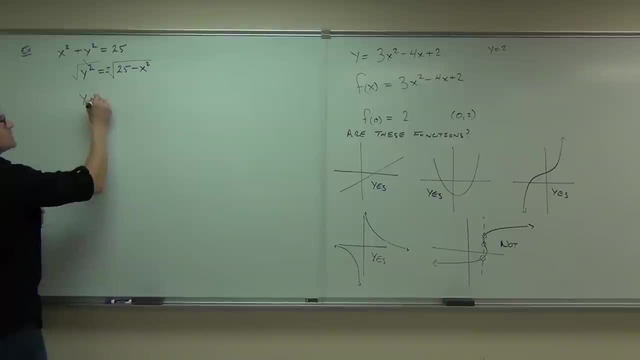 When you do that, you absolutely must have a plus or minus. Do you see the situation? now? I want you to try to plug in a number and tell me how many answers you get out, how many outputs you get out, How many are you going to get? 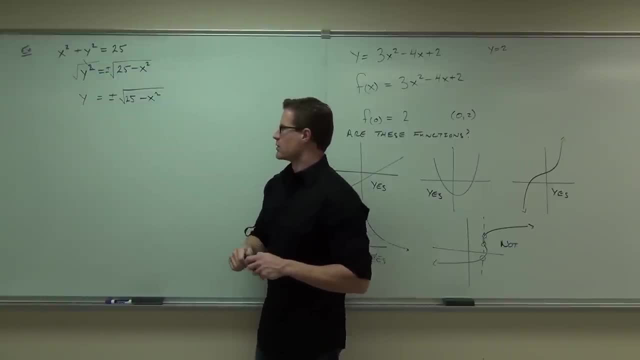 Yeah, because if you plug in something like I don't know, 4,, you're going to get 25 minus 16, right, Right, You're going to get 9.. The square root of 9.. But then you're going to take plus 3 and minus 3.. 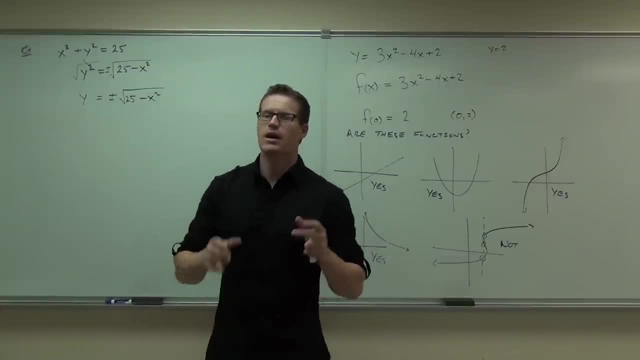 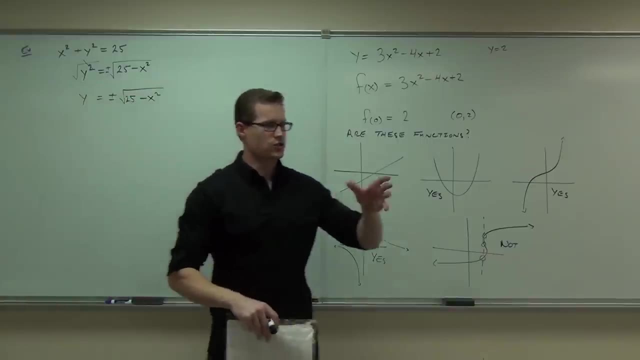 That's giving you those two answers. As soon as you have that out of a formula, you're going to have a function. Now the question is: could you work with it to look at parts of this function? And that answer is yeah, absolutely. 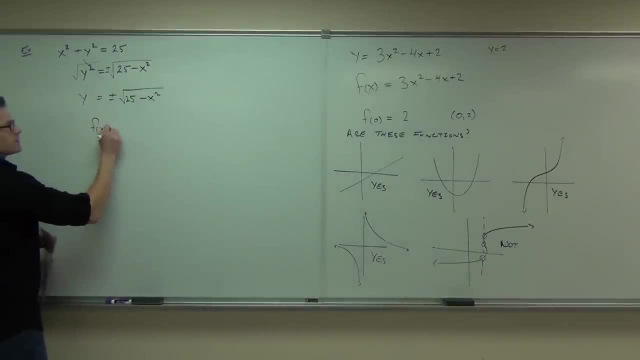 If we define this a little bit differently, if we say: well, let's call f of x the square root of 25 minus x squared, and g of x the negative square root of 25 minus x squared. Now let me ask you a question. 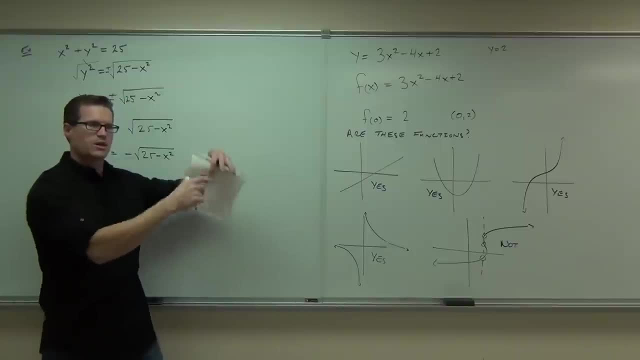 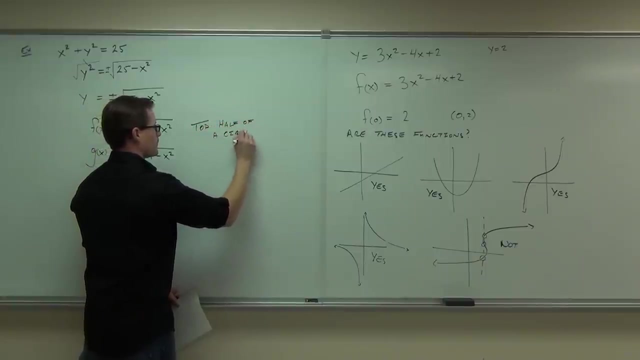 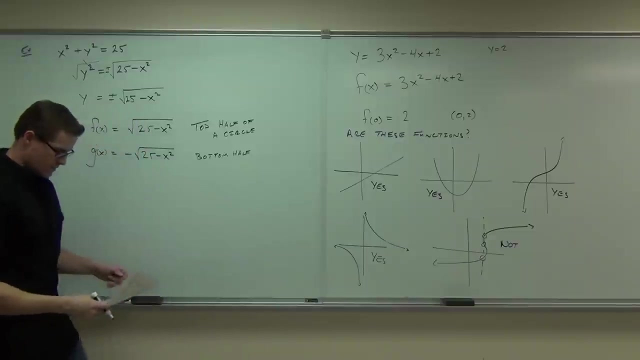 Is this a function? Yeah, sure is this a function. Well, we could talk about each piece. That'd be fine. What would this be? The top half or the bottom half of a circle, Top half, bottom half? Then we could talk about them. 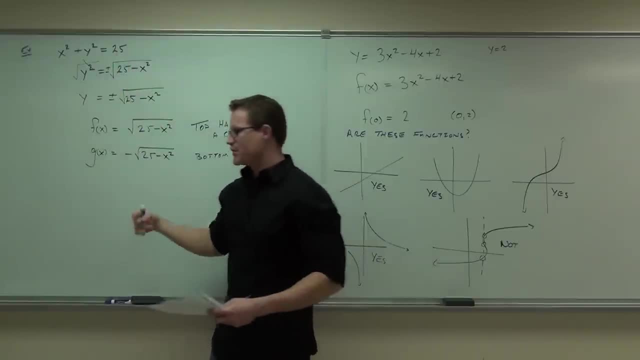 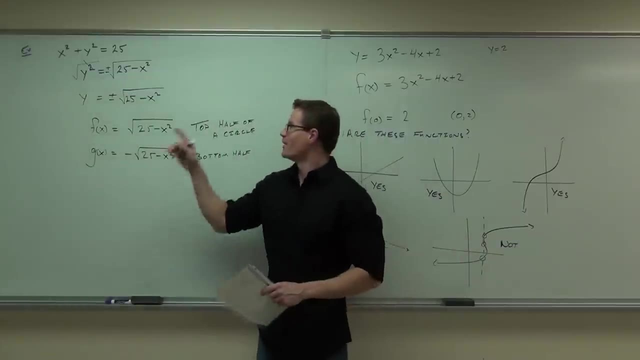 But altogether, when we look at that thing, certainly we don't have a function there. We can talk about one of them. It's called piecewise functions. Before we go on to that, are there any questions on the line test or what we're doing over here? 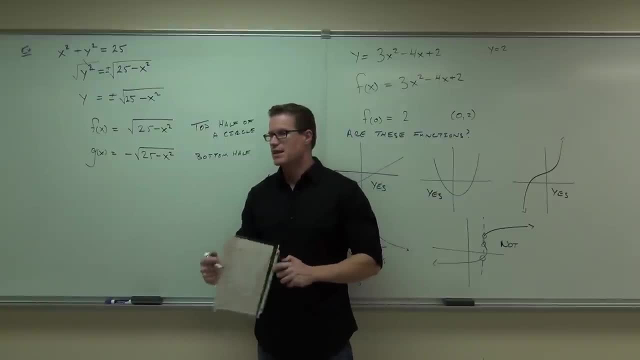 kind of just showing that all formulas aren't functions. I mean, we don't have that necessity. When we solve them, though, we can talk about pieces of them as functions. Are you guys all with me on this so far? You ready to talk about piecewise functions? 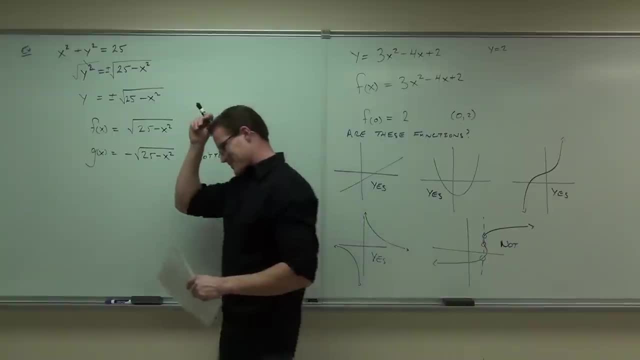 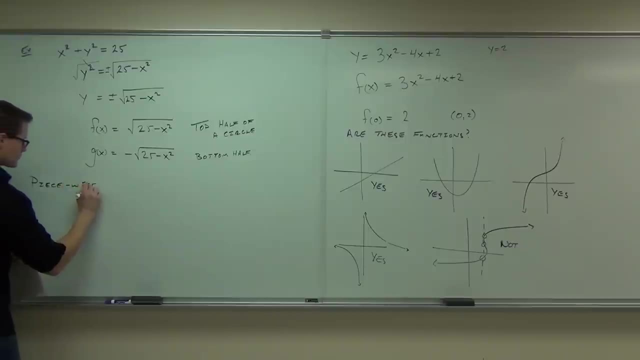 You sure? Sure? All right, Here's what a piecewise function basically is. Have you guys seen a piecewise function before? Yeah, Okay, I know you have. You're supposed to have seen it. It is to be in this class. 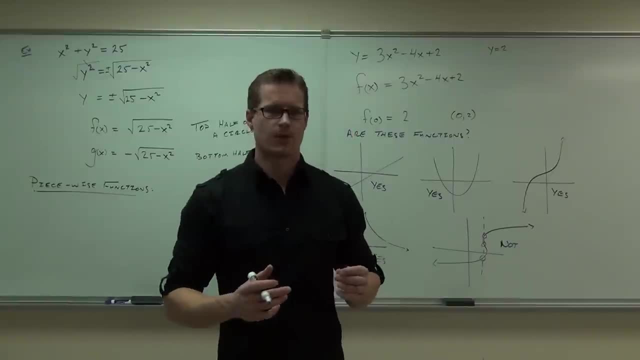 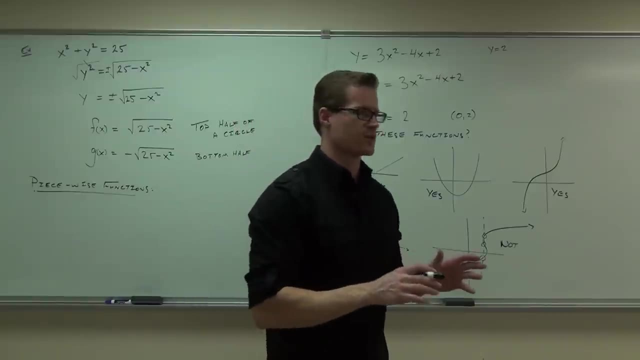 You've seen it before, One very basic piecewise function we're going to deal with in just a second. The idea is, though, with piecewise in general, that the formula depends on how much of a function you have. So, for example, 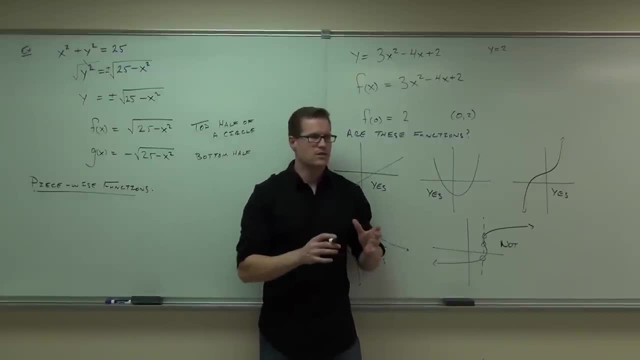 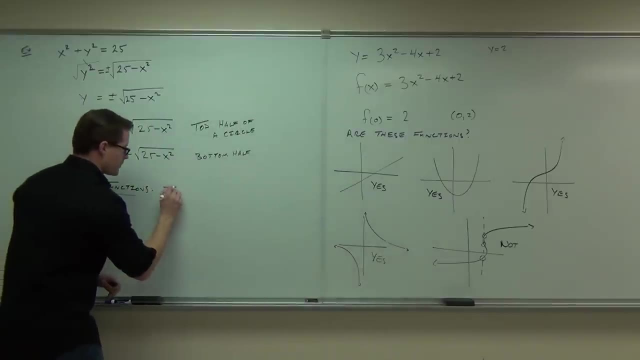 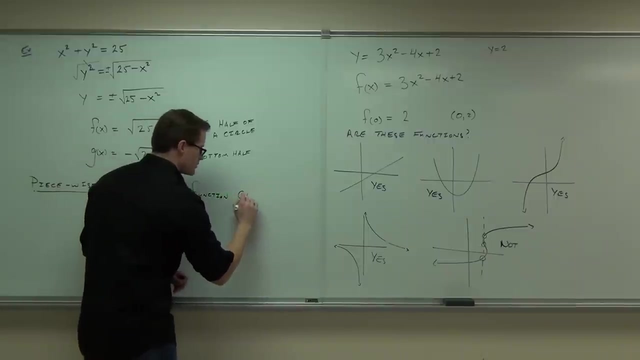 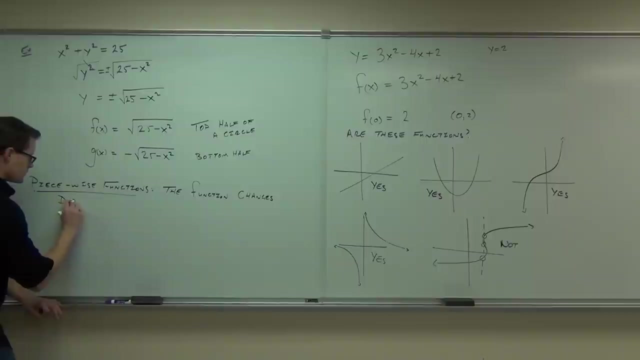 the formula for the function depends on what value you're trying to plug in. So piecewise functions work where the function changes depending on the value of x- your input. So the function changes depending on the value of x- your input. So 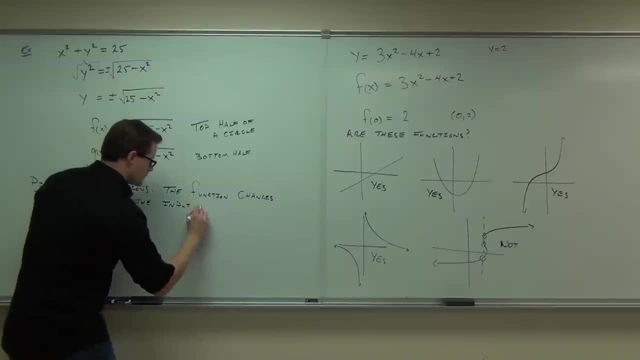 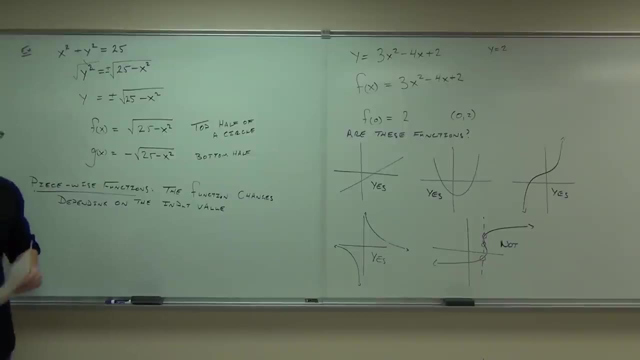 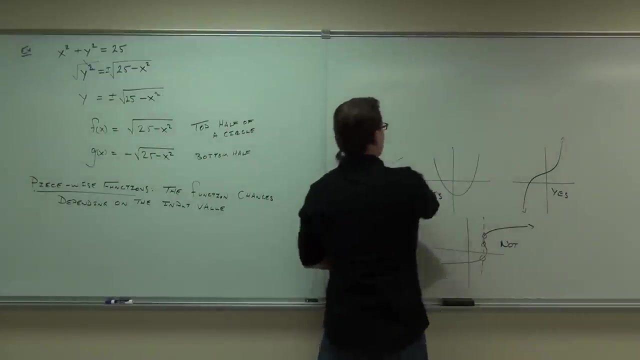 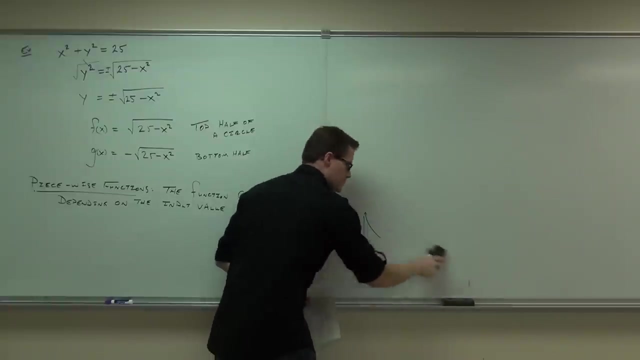 the formula changes depending on the value of x, your input. Move over here for some room. The most simple one I can think of- and this is really a really simple one that people introduce piecewise functions with, It's one you deal with. 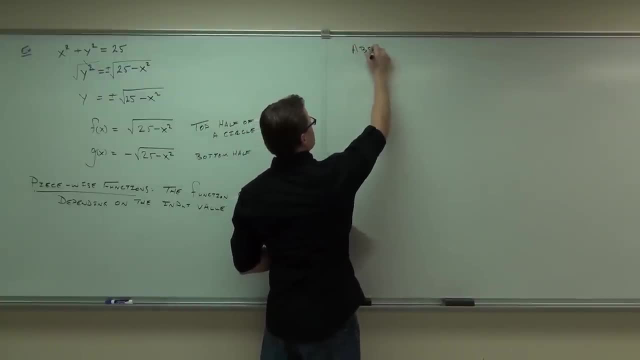 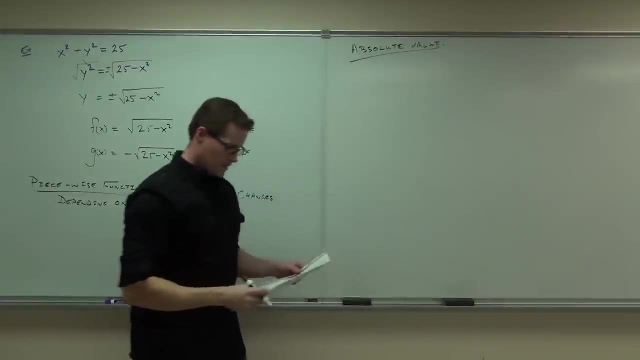 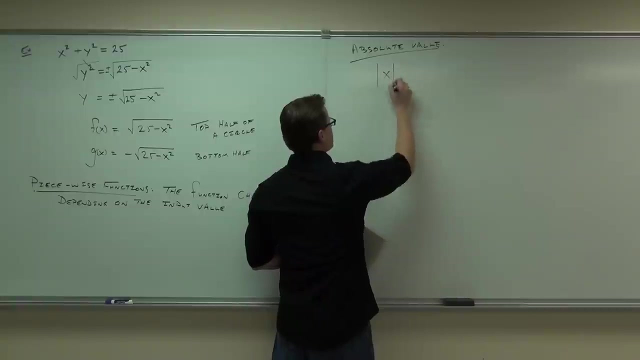 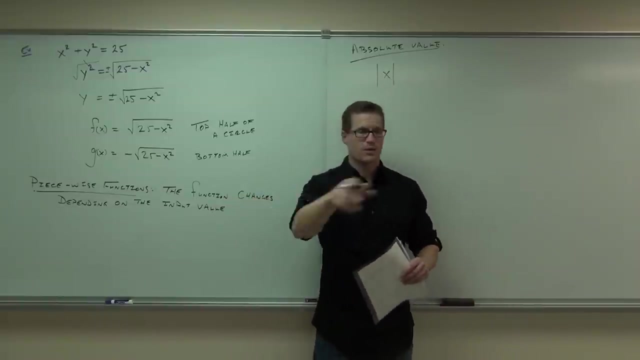 it's the absolute value function. What's the symbol for absolute value? What do you do with that? If I see the absolute value of x, what does absolute value do? Yeah, that's right, And some other people you said: 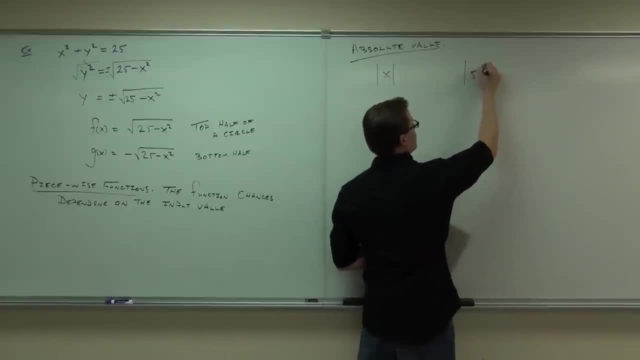 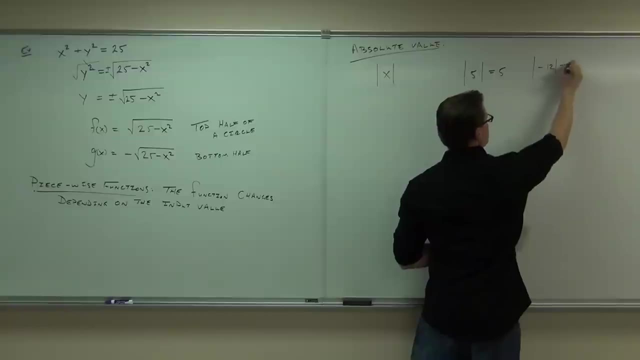 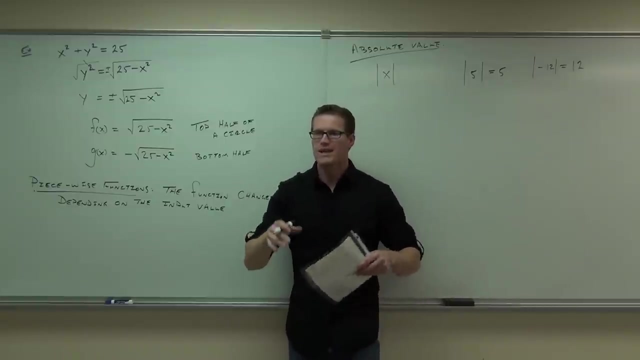 if I put a number in there, I say absolute value of 5.. What's absolute value of 5?? Okay, And I say absolute value of negative 12 and you tell me it's 1.. It's a distance from 0,. 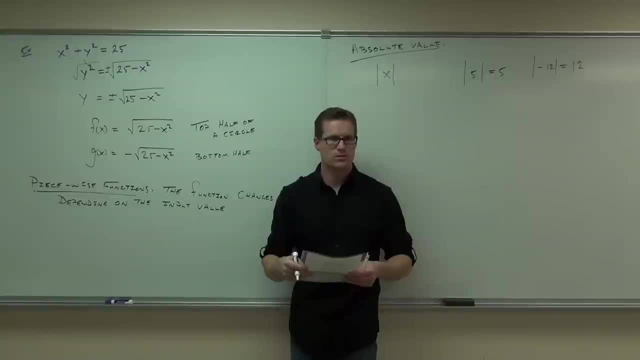 we're counting over. What does it do? What does it do? Okay, so make everything be more specific. 1 is already positive, So what does it do? If the number's positive? does it change it? No, If the number's negative, 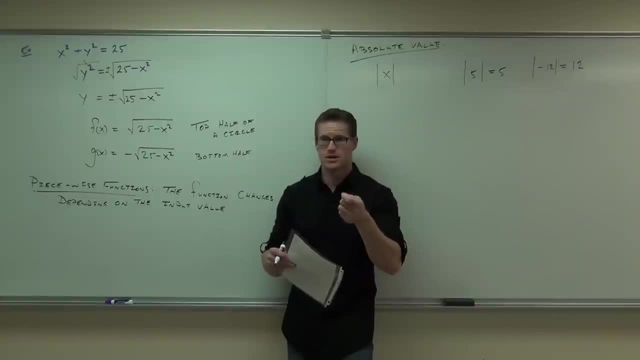 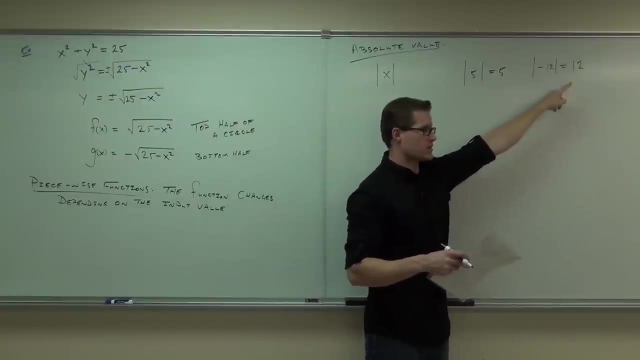 does it change it? So you're telling me that this function does two different things, depending on what value x is? That's really what you're telling me, right? If x is positive, I leave the number alone. If x is negative. 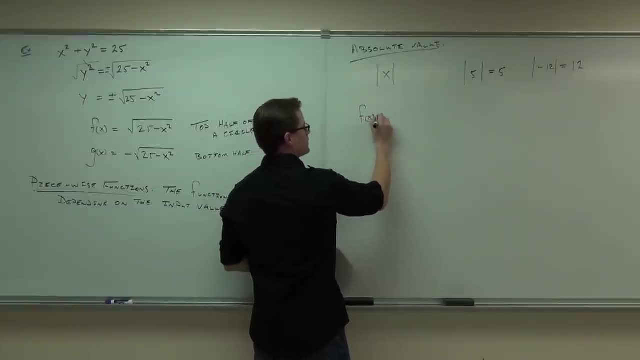 if we say, okay, f of x is absolute value of x squared. it's really hard to think about that. as far as a graph goes, I mean you might know what the graph looks like, but how would you say you might have memorized that. 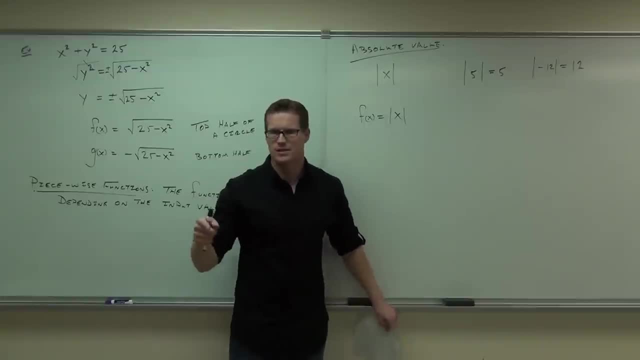 do you know what the graph of absolute value of x looks like? Yeah, show me with your hands how it looks. Don't throw up gang signs, I'm just kidding. No, yeah, it's a v Now. how can you get that from this? 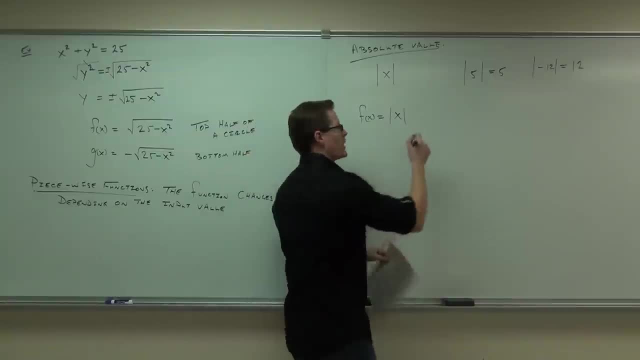 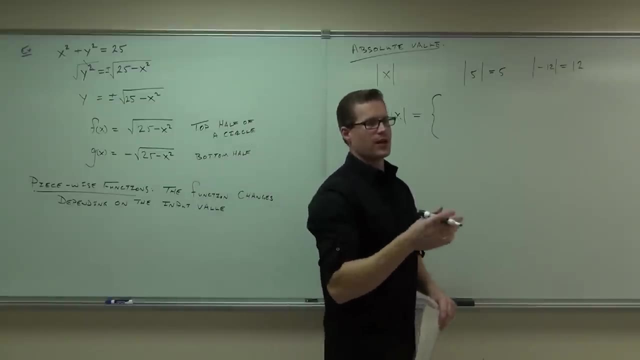 You have to figure it out or you have to define it piecewise. Here's how a piecewise definition looks. It has that funny bracket that says all this stuff goes together, And then we have to define it on a piece-by-piece basis. 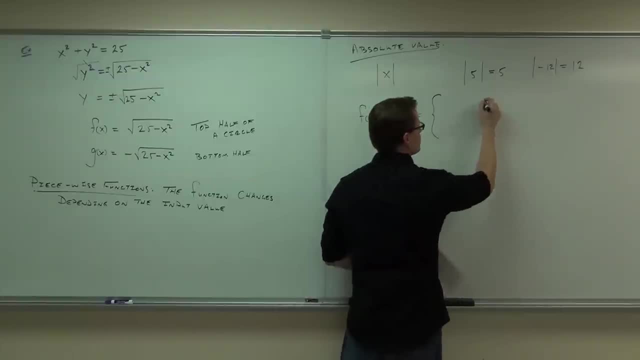 Here's what the absolute value does. It says you're going to do something if x is greater than or equal to 0.. You're going to do something else if x is less than 0.. Some people define it as strictly greater than, strictly less than. 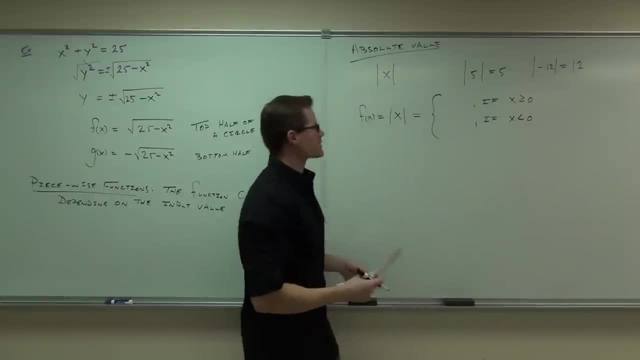 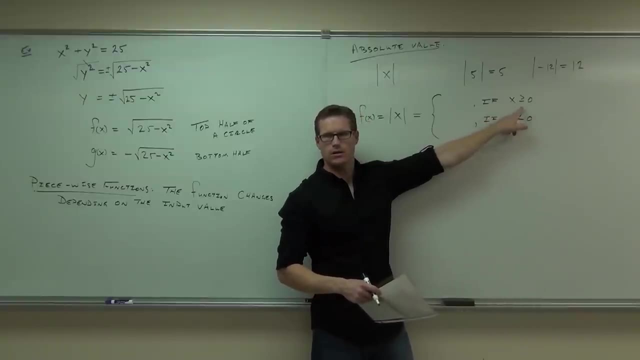 and then when x equals 0 itself, we're going to define it like this: What do you do if x is bigger than 0?? Do you have to change it at all? Now, like this: 5, you didn't have to change the 5,. 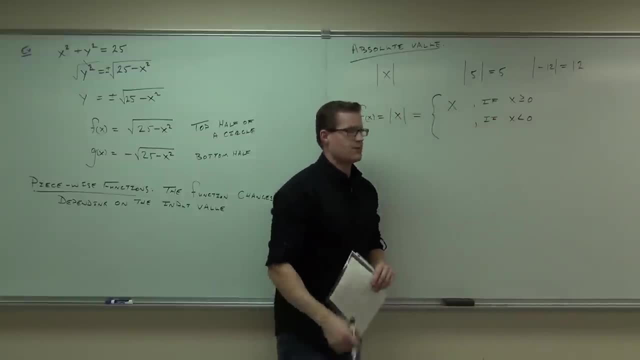 you just pretty much dropped the absolute value. So we leave the x alone if it's bigger than 0.. What do you do if x is less than 0? Change it. What now? Okay, so we change the sign. You said negative x. 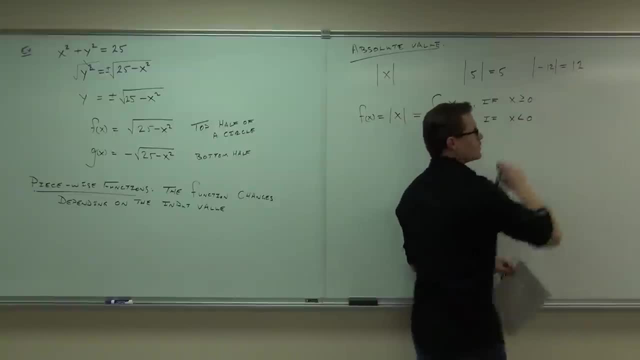 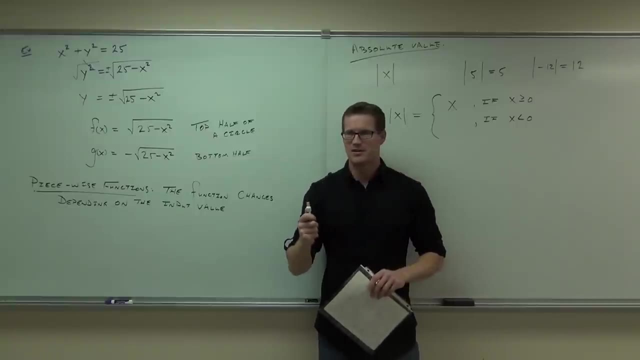 That's when we can change it right. If I did this and said: how do I get from negative 12 to 12? What math did you do? Magic? I'm Harry Potter. Negative's gone right there. Alright, Voldemort, I'll show you who's boss. 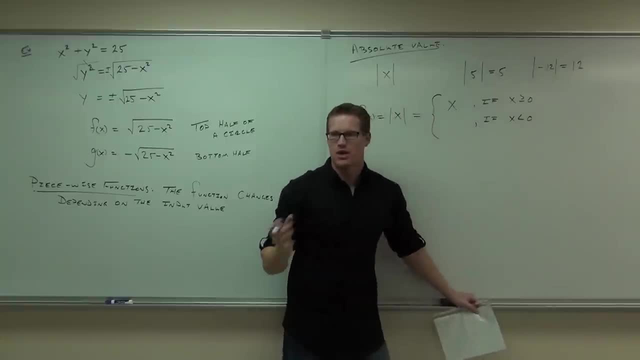 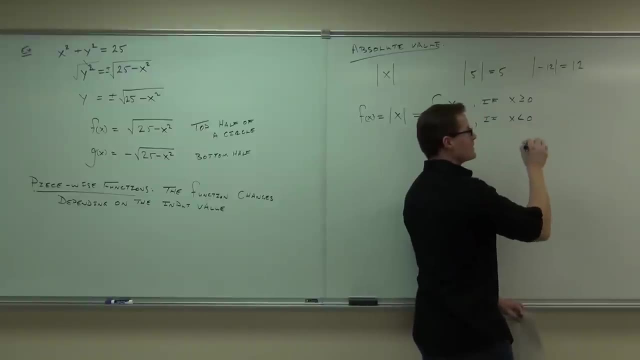 Too much. What this really says is you have to find some math way to change a sign. So absolute value of negative 12 really says follow this formula and it says you take the negative of negative 12.. Does that give you back? 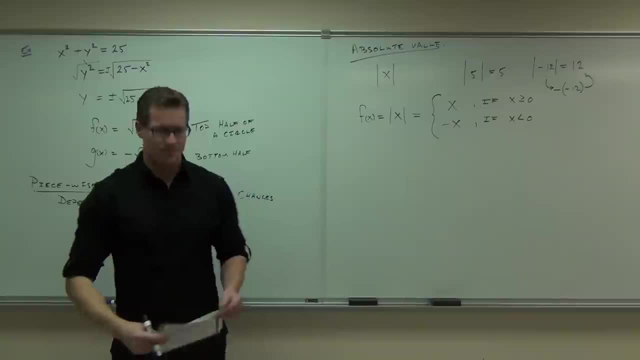 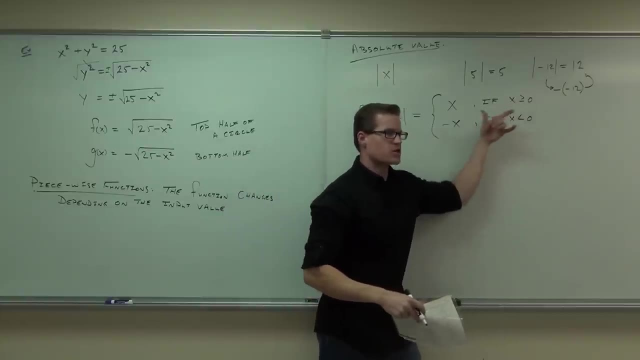 positive 12?? That's the piecewise definition. right there, That's it, And it works for anything. You can follow these directions for your piecewise function. It will tell you which part to use. Now, of course, we know this one from a long time ago. 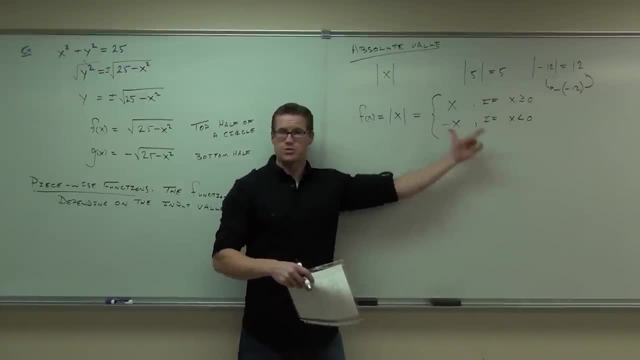 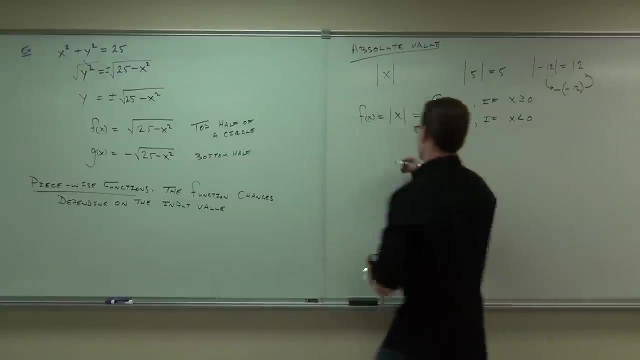 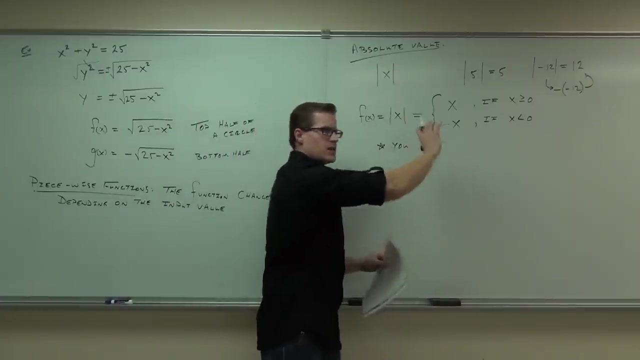 but can you see that? this is the definition of that. What's kind of cool is that any piecewise function can be graphed by using their pieces, So we're going to do that next. You can graph any piecewise function by graphing each piece. 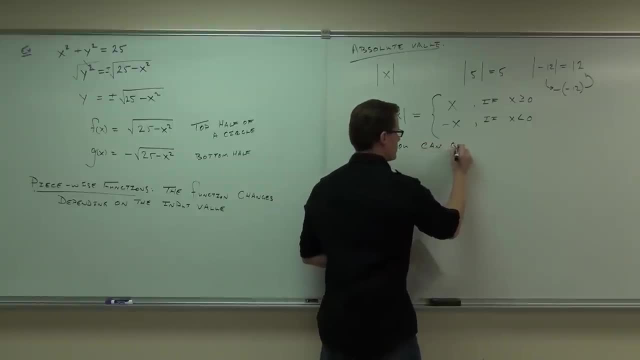 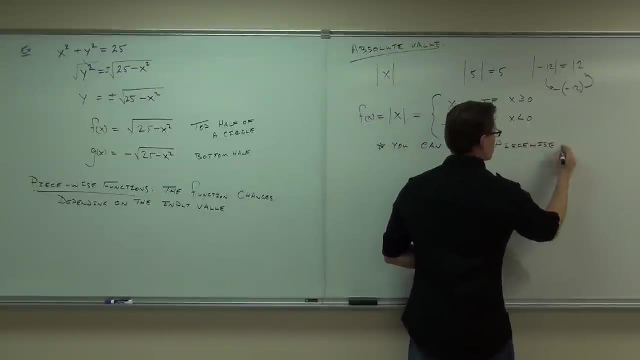 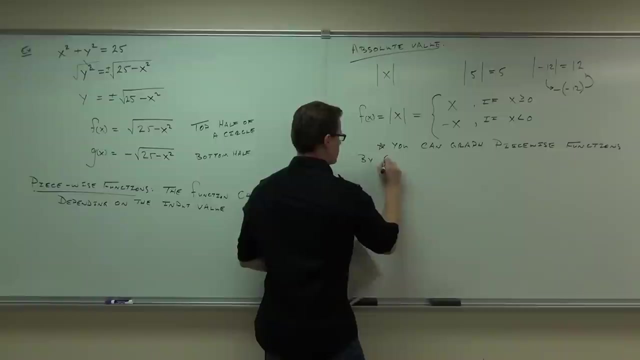 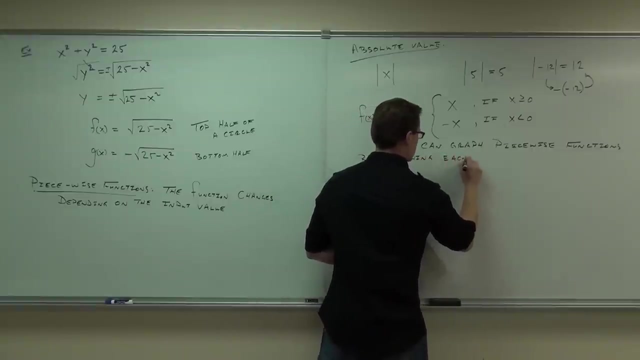 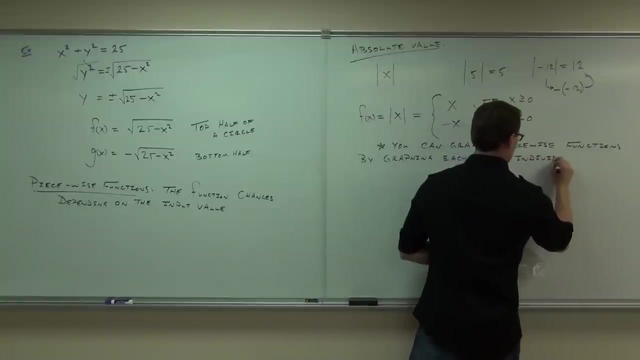 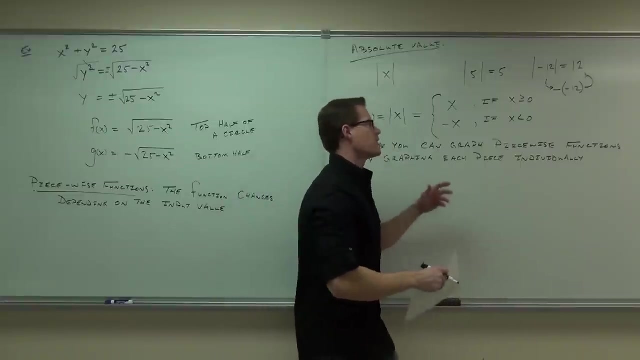 individually. The only thing you have to be concerned about is that you use the appropriate range. That's really it. So we're going to tack on just a little bit. You can graph piecewise functions by graphing each piece individually, but you have to do it for the given range. 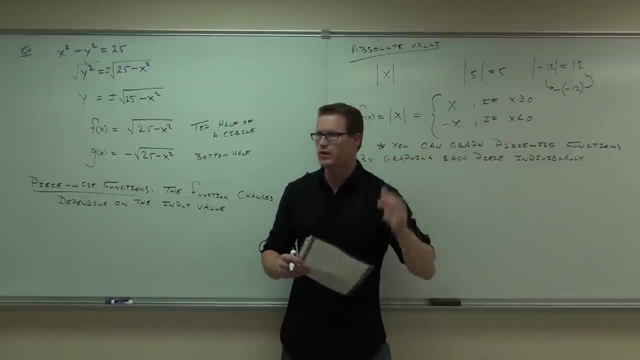 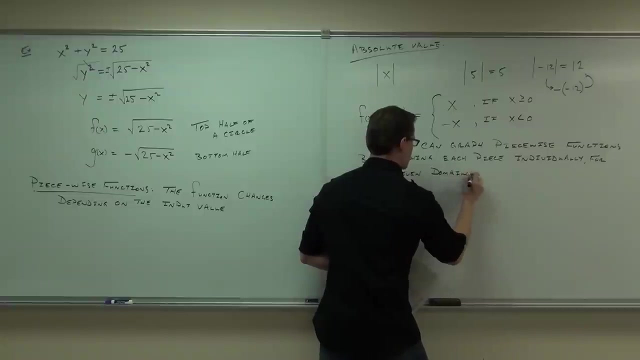 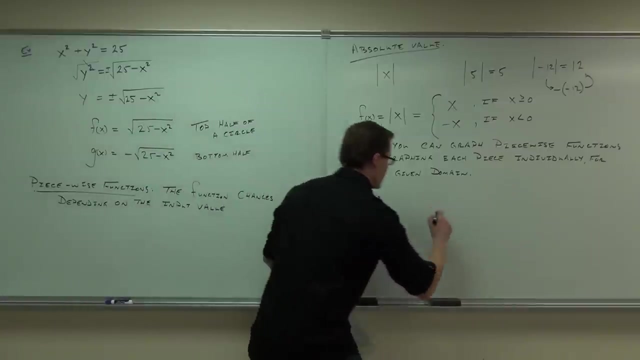 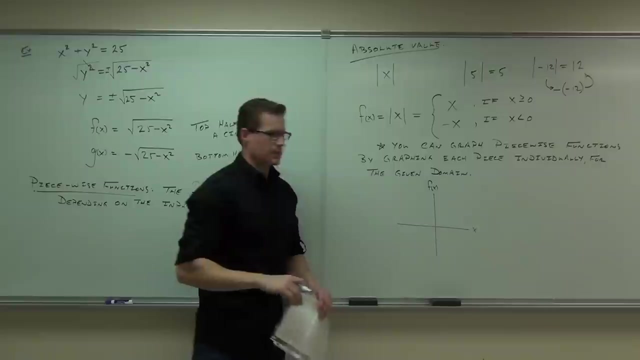 So we're not going to graph the whole line of f of x equals x, We're just going to do it for a little bit of it. I'm going to use that word domain. Let's give that a try. 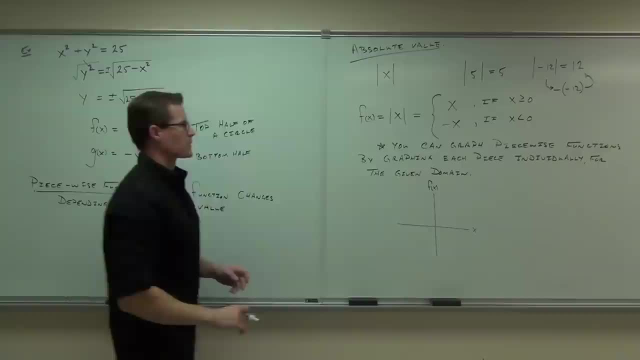 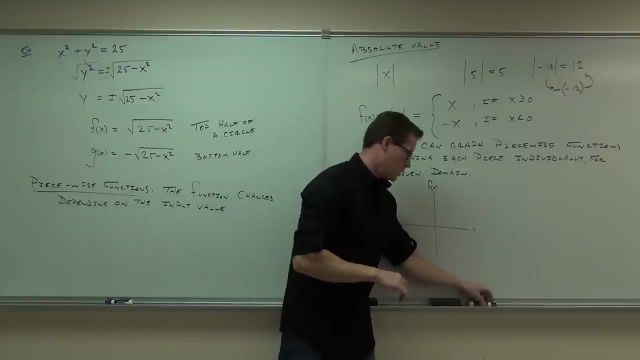 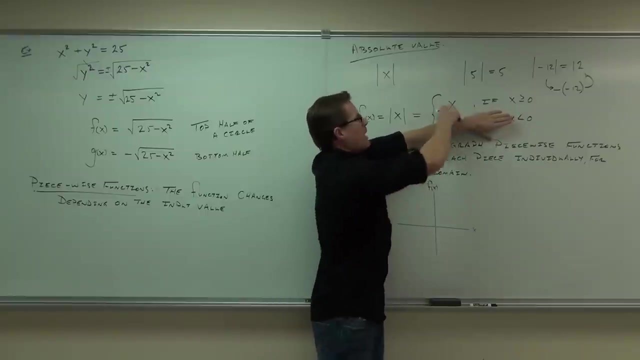 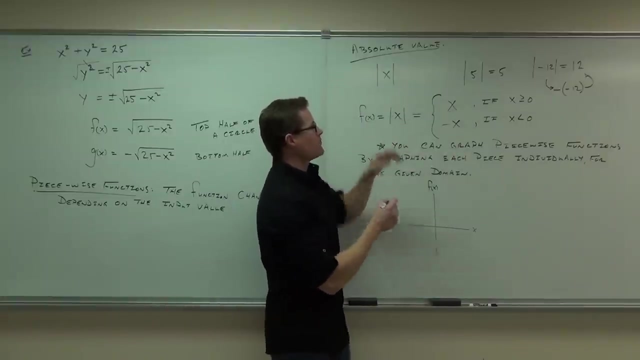 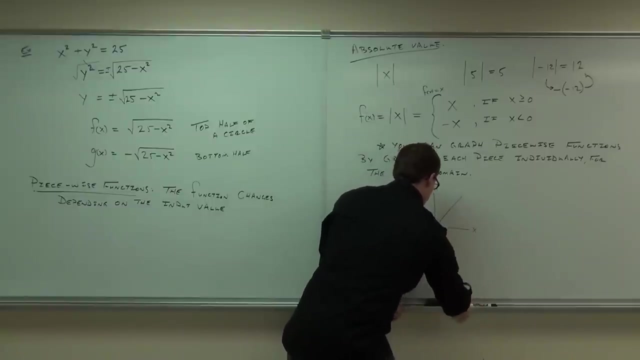 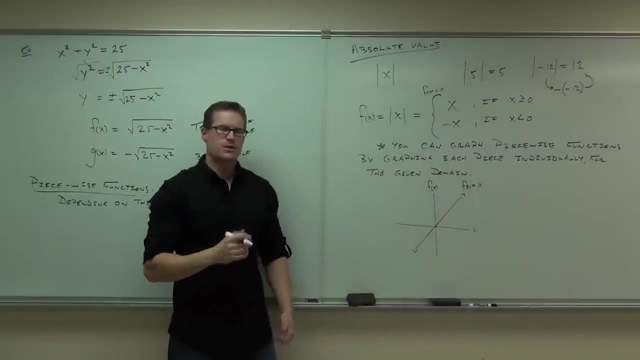 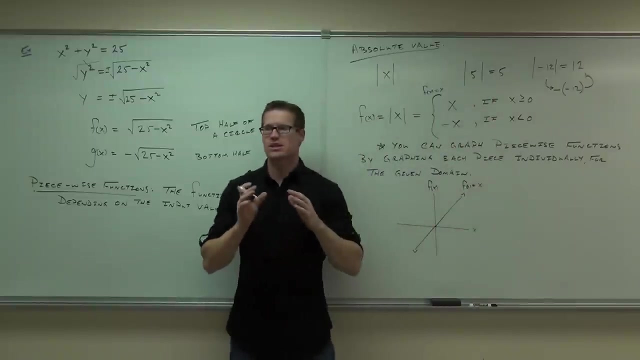 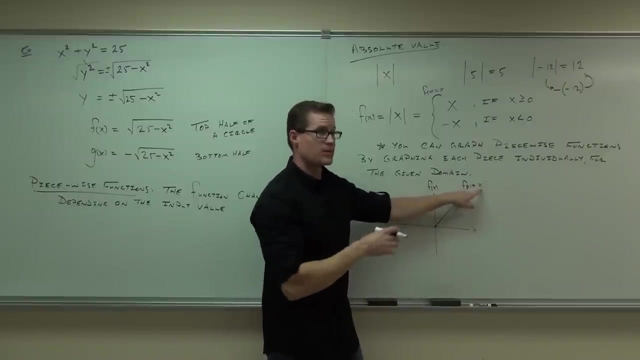 Since we know this, already has the piece of the graph. 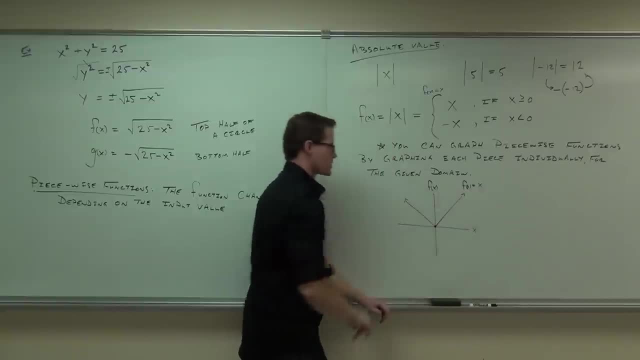 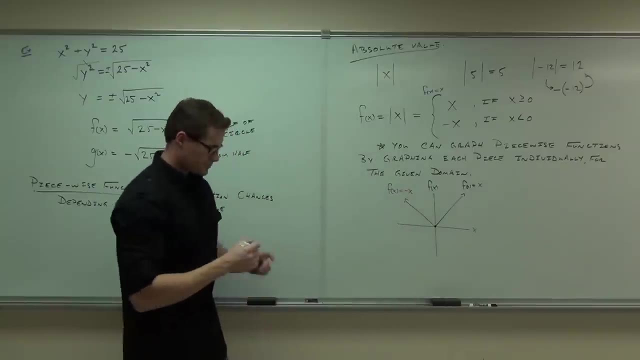 we can't put anything else, otherwise it won't be a function. We're going to leave it just like that. That's where you get your v from. This is the f of x. equals negative x. Are you ready to try something just a little bit more advanced? 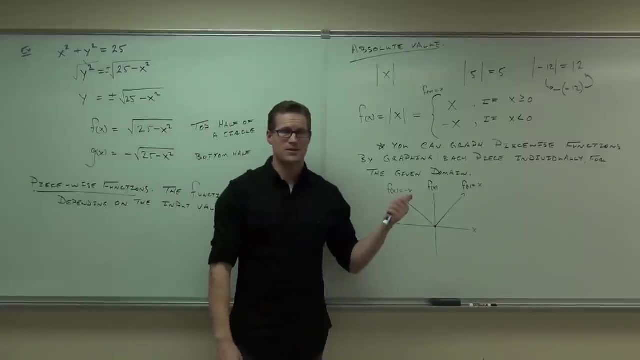 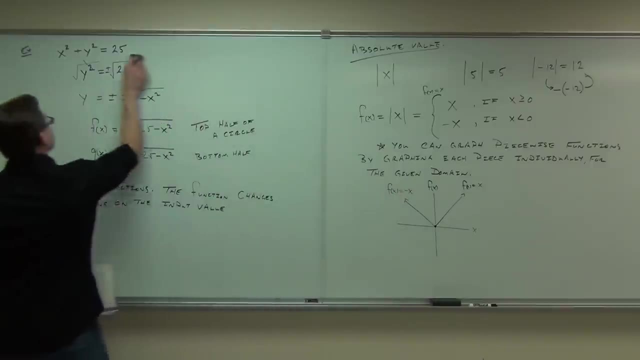 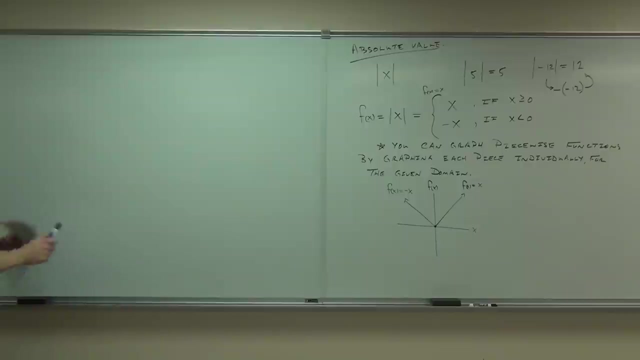 Can we do that? You guys have any questions on the absolute value. You've all seen that before. yes, Let's see if we can sketch something a little bit. funner Is funner a word. That's better. 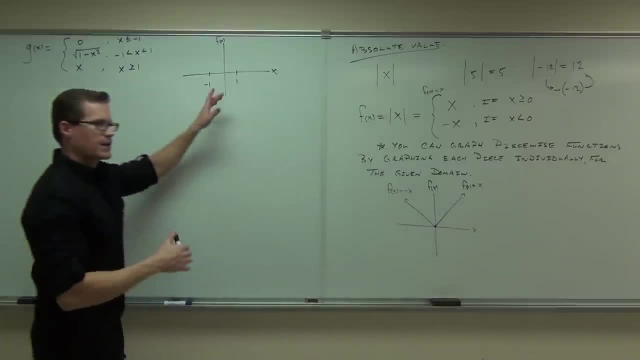 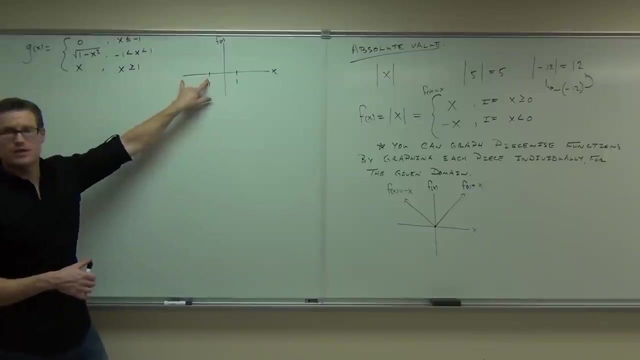 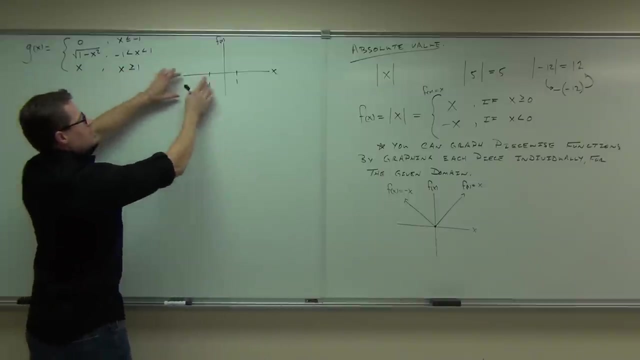 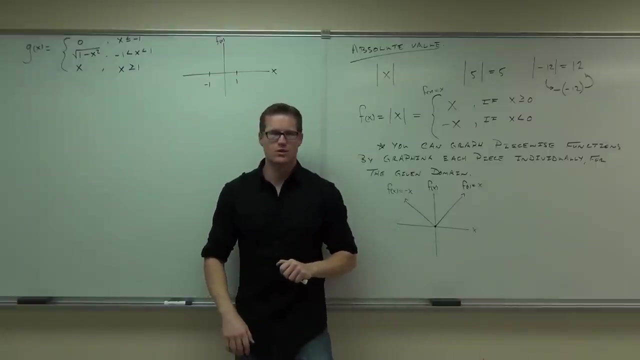 What does zero mean? What's zero mean? Horizontal line Good, where On This Y equals zero. This, which one? this Do you know? 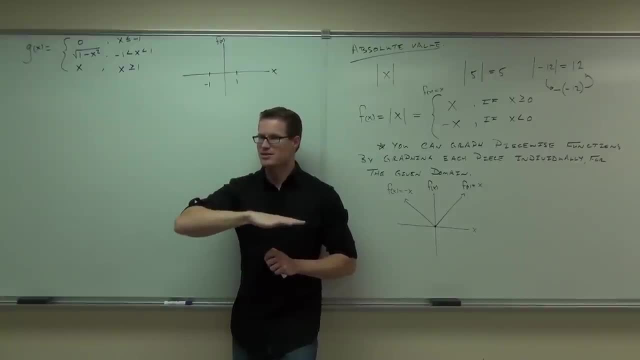 Have I lost ya? Where I've lost ya? like this, Have I lost ya? It would have to be horizontal. to be like that, It would have to be horizontal. Listen, if the whole grouping of this kind of confuses you. 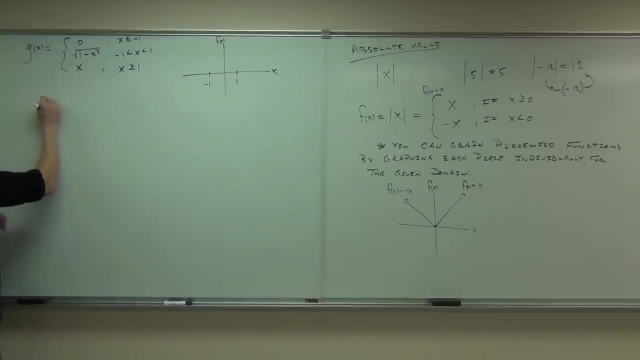 just write them out differently. Say that you have y equals zero for a certain bit. Say you have y equals the square root of one minus x squared for a certain bit. Say you have y equals x for a certain bit, It's the same thing. 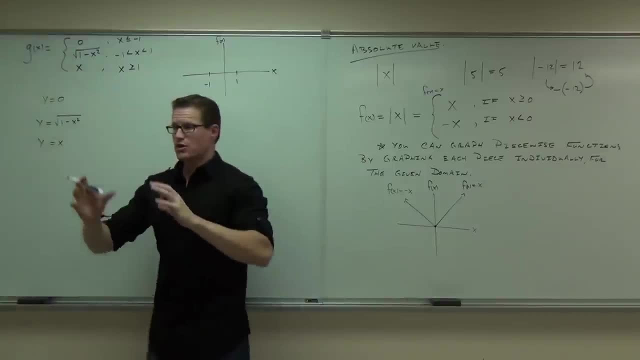 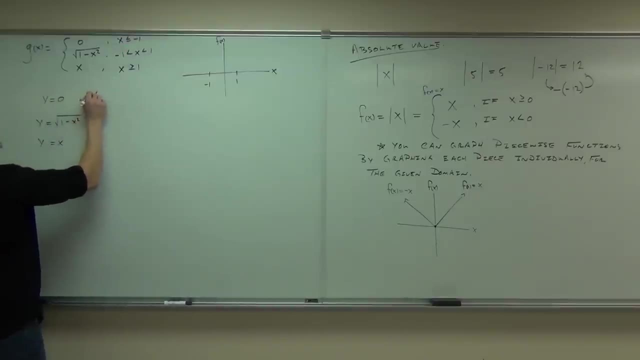 You're just grouping all these together in function and graphing them piece by piece. Do you see that? Okay, so this is the piece that's working. where your x is less than eight, It's negative one or equal to it. This is the piece that's working. 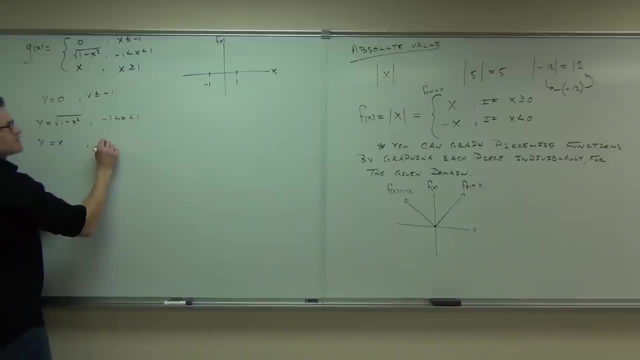 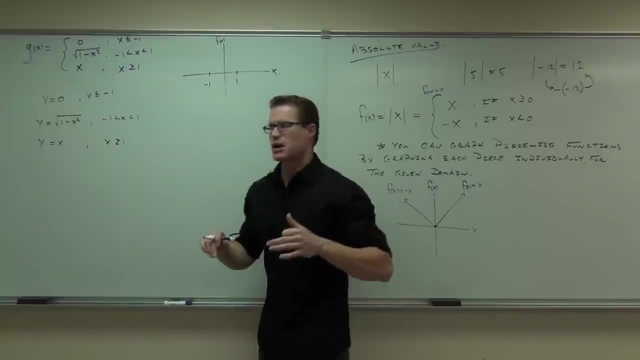 when you're between negative one and one, And this is the piece that's working. when you're greater than or equal to one, Split it up if you have to, but you need to be able to graph each of those functions. So can you all tell me now? 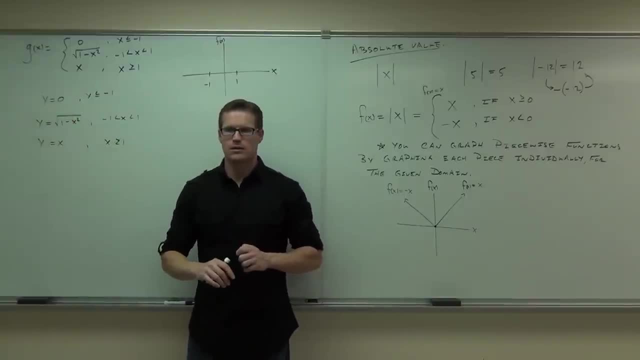 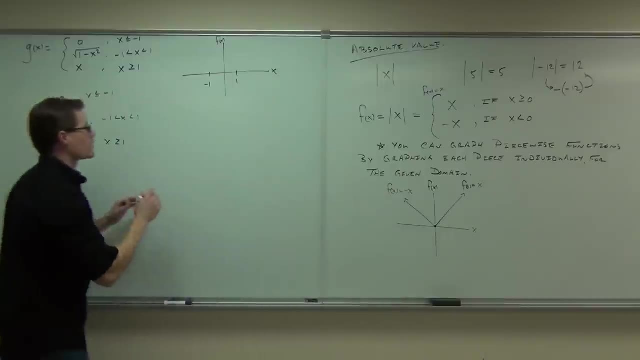 what does y equals zero look like The x-axis. That is the x-axis. yeah, That's a horizontal line at y equals zero. Y equals a constant right. We talked about that last time, that it's a horizontal line, So we're talking about this right there. 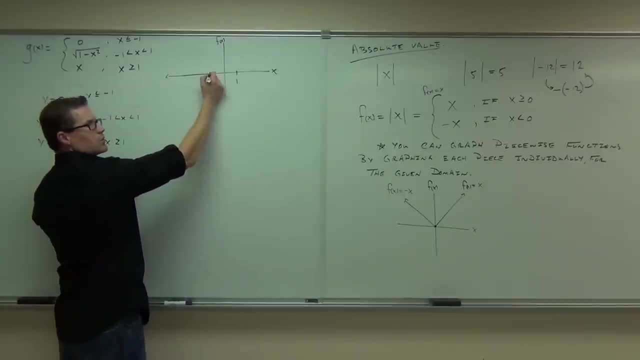 One question I have for you: should I have an open circle or a closed circle here, and why Closed circle? And why? Because it's equal to it. Good, Good, very good. Okay, check, Got it. Let's go to the next piece. 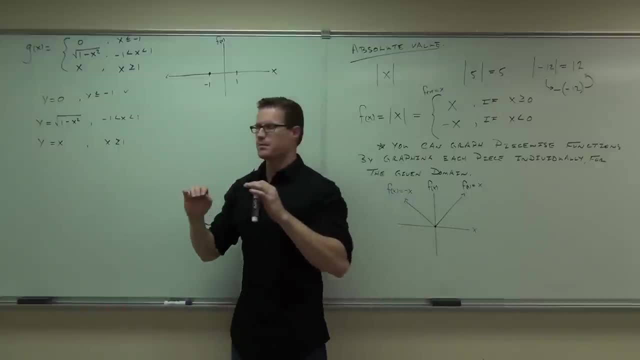 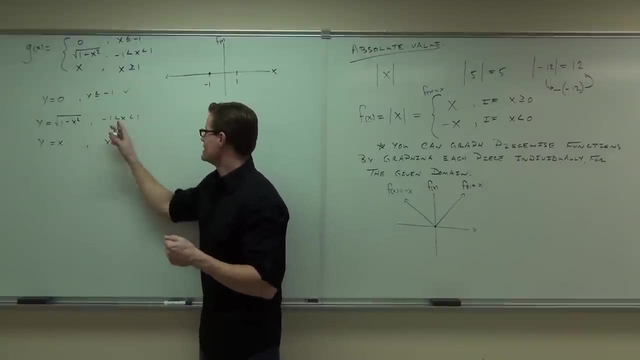 The next piece works between negative one and one. Now do you also understand why we might have to have no equal sign here and why, if I did this, it would not be a function, It would be overlapping. It would be overlapping if these were different. 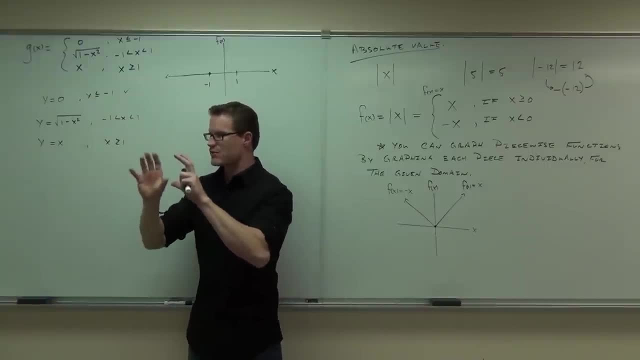 That's right. so you're never going to see equals, equals. You're always going to see it for the same value. You're not going to see that, So let's go ahead and see what the what is that? Oh my gosh, what is that? 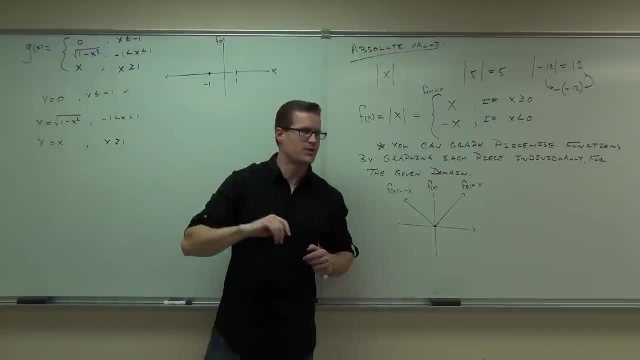 Do you recognize it? We had it before on the board, except the numbers were a little bit different. What is that Circle? That's a circle. If you squared both sides, you'd get y squared over there, wouldn't you? 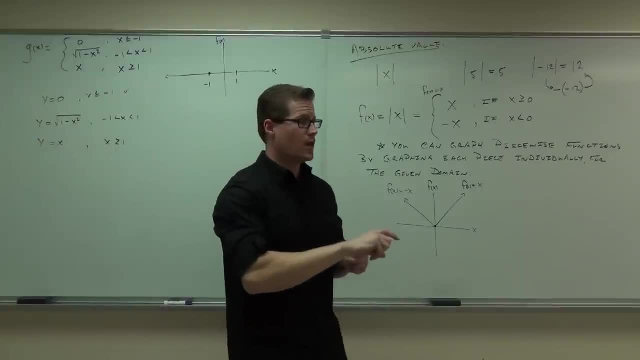 If you added the x squared, you'd get x squared plus y squared plus y squared equals one. That's a circle. It's centered where, do you think? The origin? Origin? Somebody else tell me what's the radius? 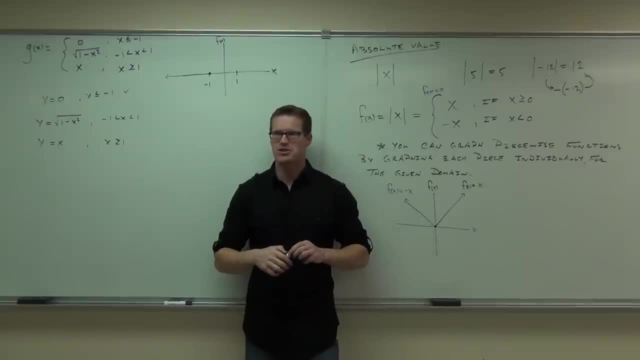 One, Mm-hmm, that's one. Guys, if you have questions now, now would be a good time. Are you okay that this is a circle? How many people feel okay that that's a circle? You can see it. 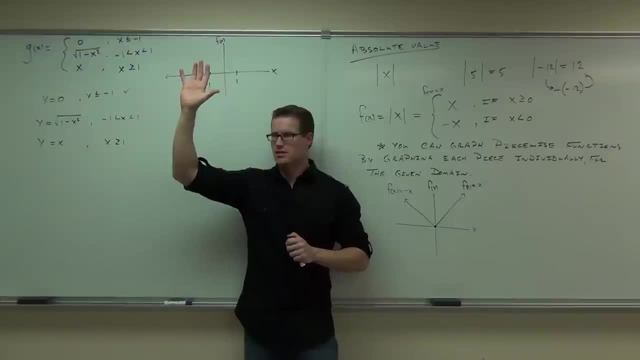 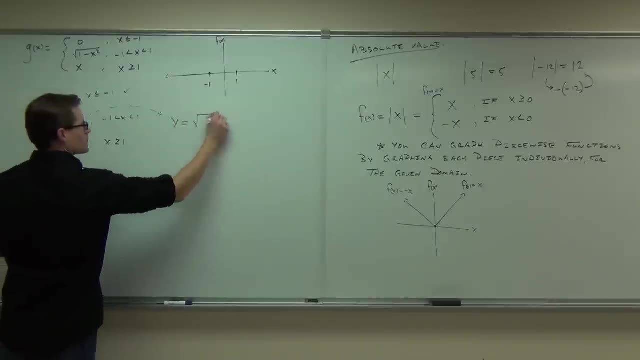 If you can't see it, don't raise your hand. Can't see it, don't raise your hand, Can you see it? Not so much If you can't see it, if you're like: oh my gosh, what in the world was that? 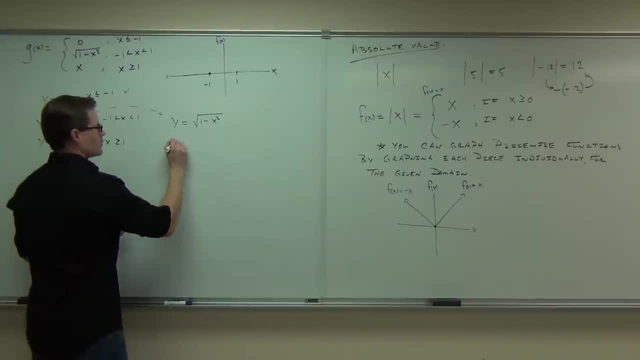 Square both sides, you get y squared equals one, minus x squared. If you add the x squared, you get x squared plus y squared equals one. Now, this isn't. we cheated. a little bit We cheated, because this is not an entire circle. 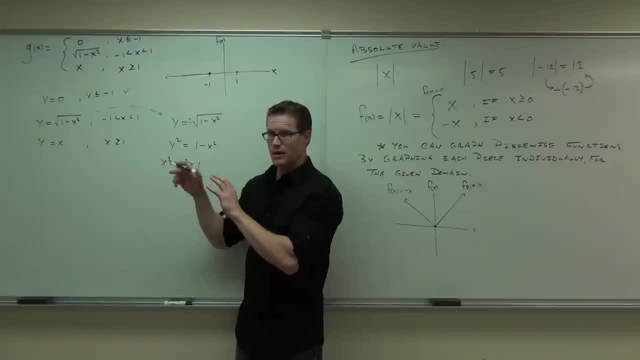 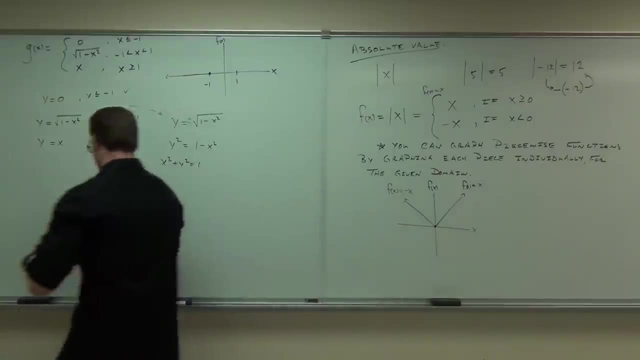 An entire circle would be that You clear. That would give the top half and the bottom half. What are we talking about? The top half or the bottom half? Which one Top half? We're just the top half. We're the top half right now. 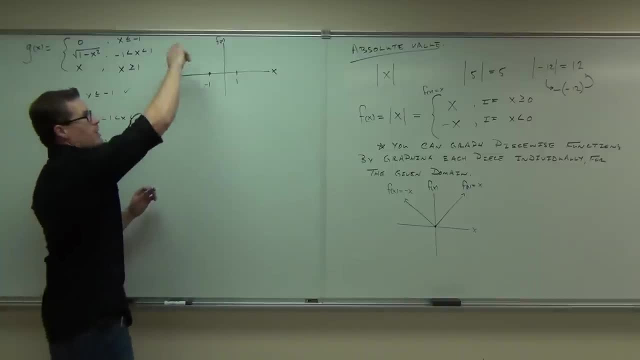 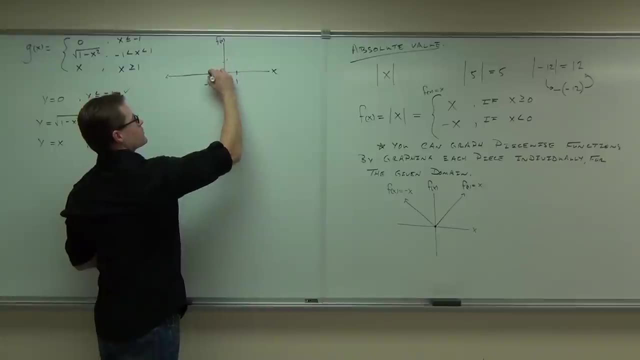 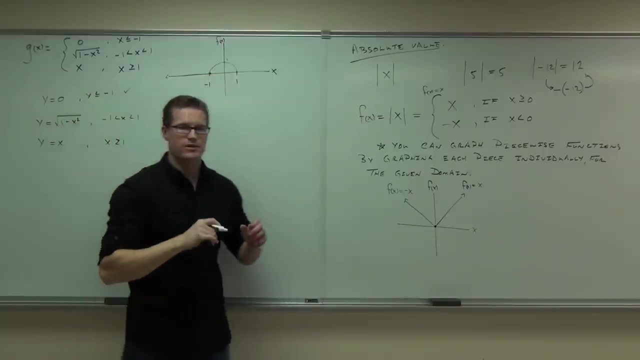 So we want the top half of the circle, centered at 00, with a radius of one. Well, that looks to me like it's going from here to there. It's going to have an open circle right here, but it's been closed in by the previous function. 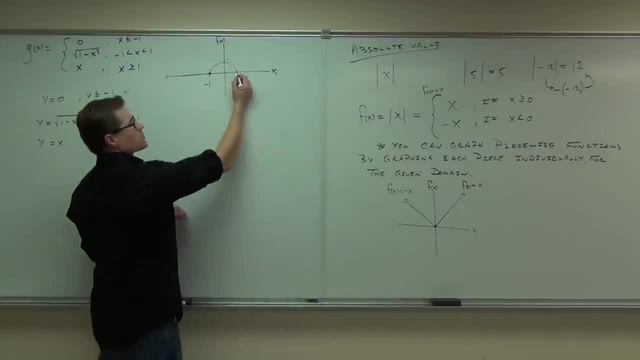 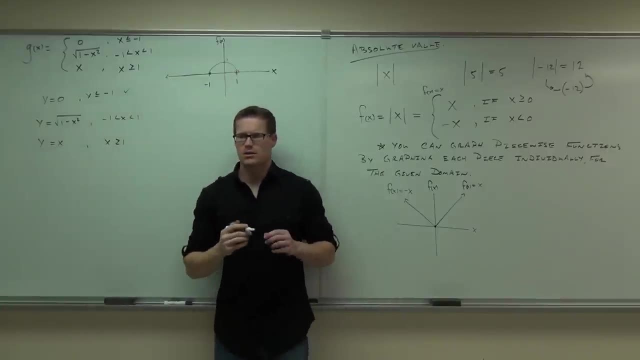 That's kind of cool, right, We don't have an overlapping point. Is it going to have an open circle or a closed circle here? Open, Yeah Again. why is it open? It's not open. Mm-hmm doesn't have that little equals. 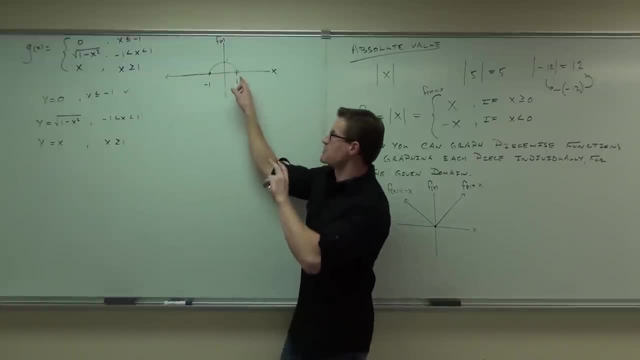 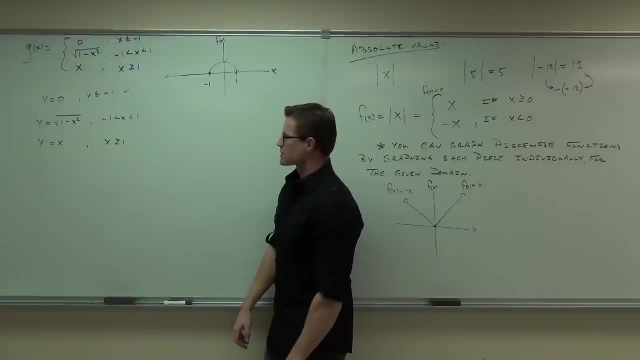 So we've got our first piece. we've got y equals zero. We've got our second piece. the top half of the circle centered zero, zero, radius one. The last piece, oh the last piece: y equals x. How are we gonna do that? y equals x. 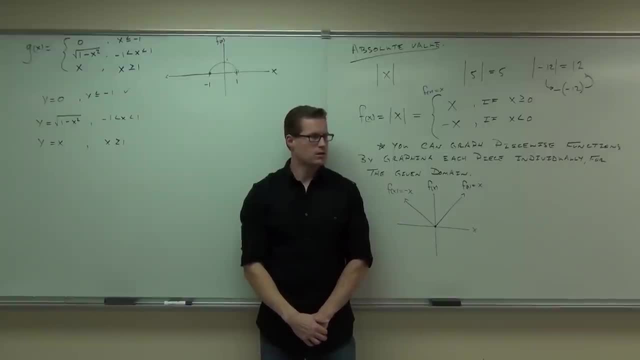 What's y equals x. look like It's a line that goes through the origin. Okay, okay, so normally we would just have a diagonal line. yeah, We've actually already graphed that. it's right here. So if we were to graph that, we'd have this thing. 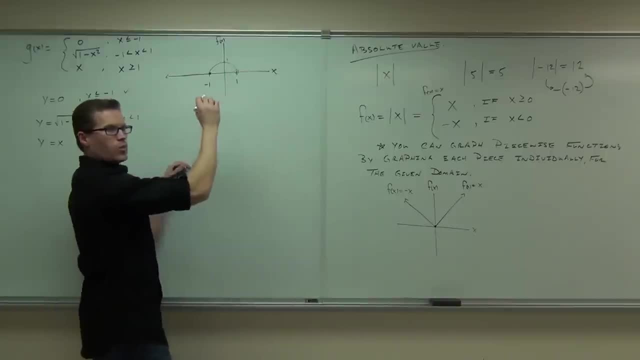 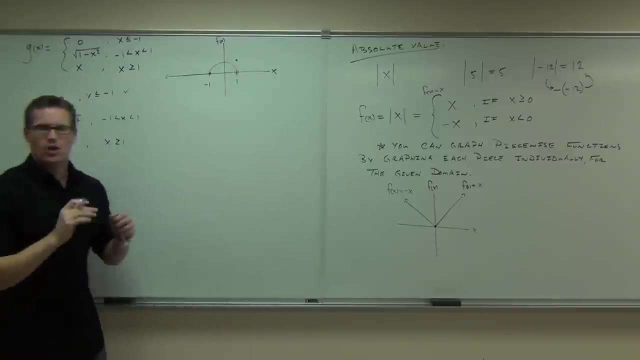 It'd be through the origin, it would go through the point one. one wouldn't it, Because when you plug in one you get out one. So I know that it's gonna go through that point and in fact it's gonna be solid. 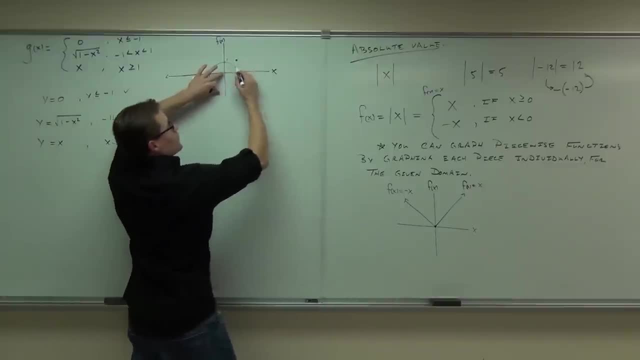 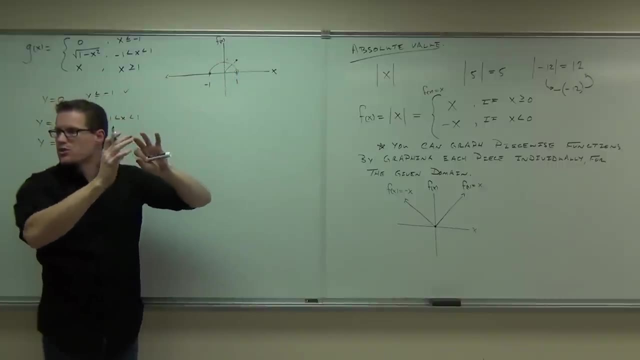 because there's an equals there. So if I were to graph it, it would be that diagonal. However, I can't have it exist. I can't have it exist over here, because then this whole thing wouldn't be a function. We're talking about just the piece. that's that way. 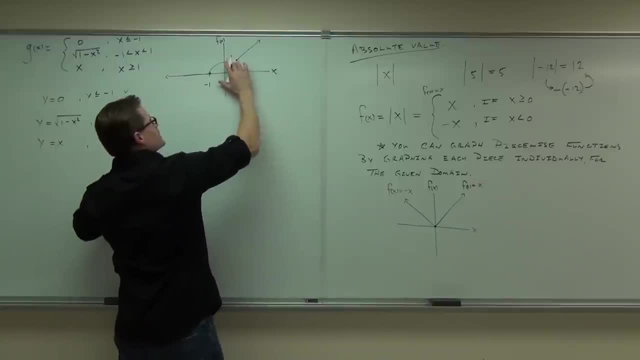 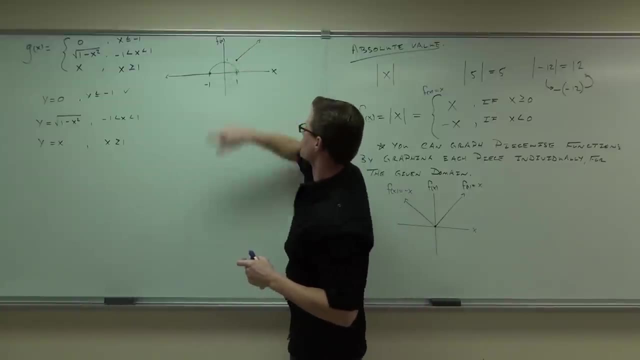 So I'm gonna extend that line, Erase this piece, because I can't have it there. I've already got my piece in the function for that part, that interval, This is the interval we're looking for. That's the piece in the function. 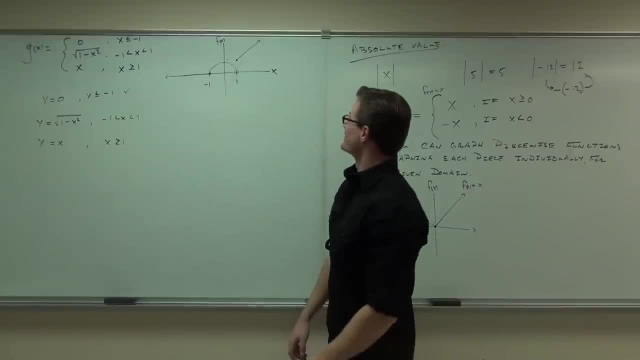 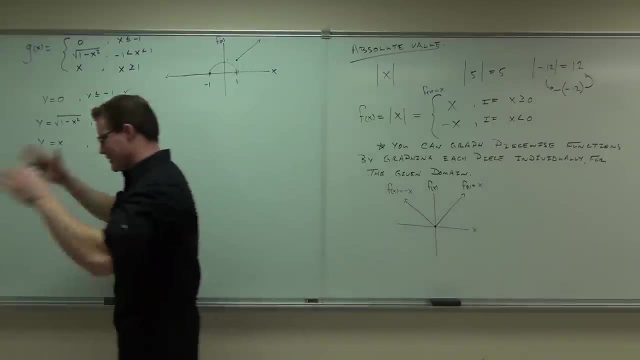 Isn't that kind of cool looking? I think it's cool looking. Are you able to understand it? Can you follow How many feel okay about that one? Good, so piecewise delineate your oh. what do you mean? 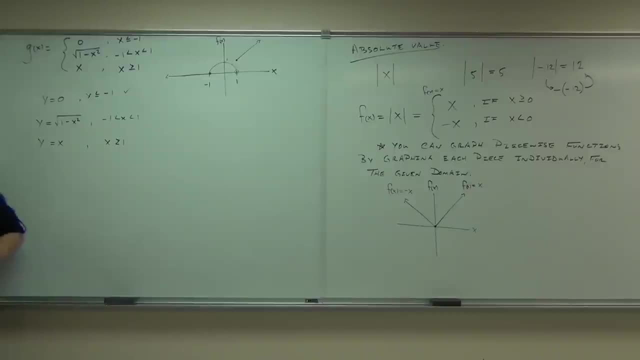 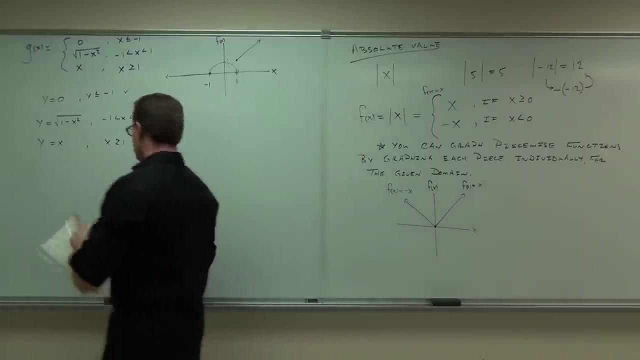 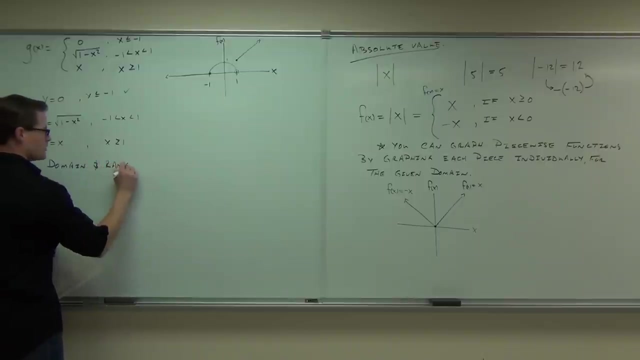 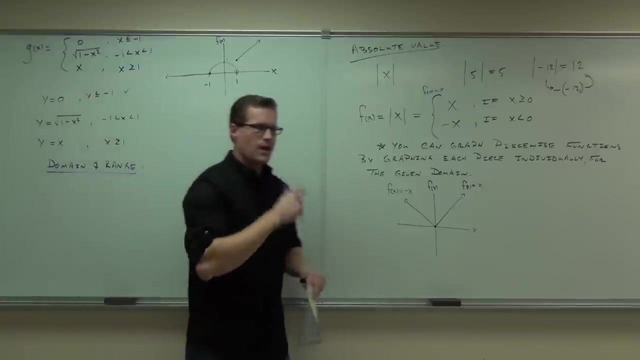 Delineate that x-axis by the appropriate intervals, graph each piece and you get that Cool. The last thing we're gonna talk about for this section, we're gonna talk about domain and range. More about domain and range. Hey, when I say domain to you, 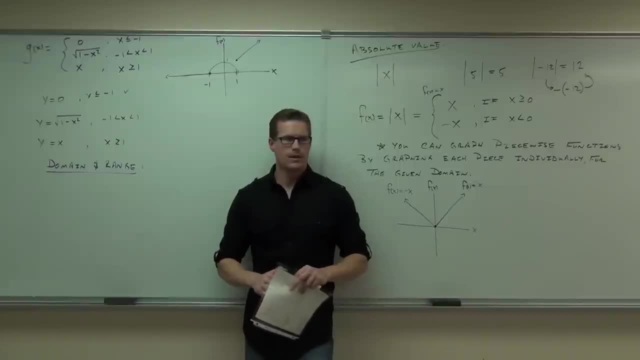 what do I mean if I'm talking about the domain More general than just x? what if I'm using different variables? What does domain someone over here? what does domain mean? Yeah, the inputs. yeah, you're absolutely right. 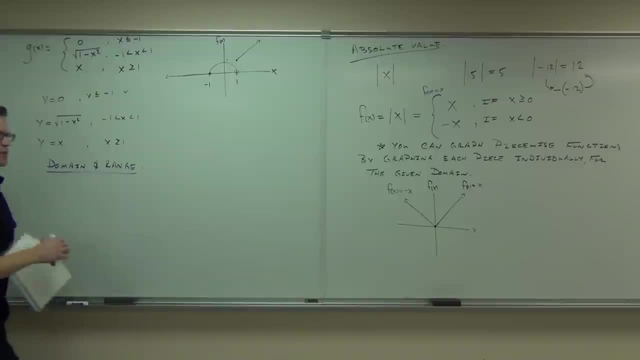 So when I'm talking about domain, what we mean is all the values you can input into a function. And yeah, you're right, they're usually x's, typically, Unless you're dealing with, like a position function. then you're talking about time. 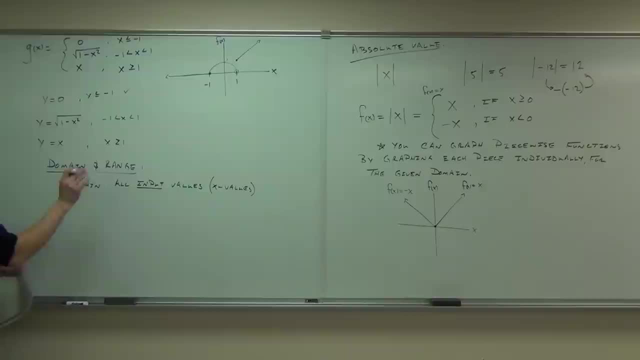 because it has to be time. If domain means all the inputs, what does the range mean? Yeah, graph six. Okay, These are usually your y values or your f of x or whatever function you're dealing with Now. in most cases, we have some sort of constraint. 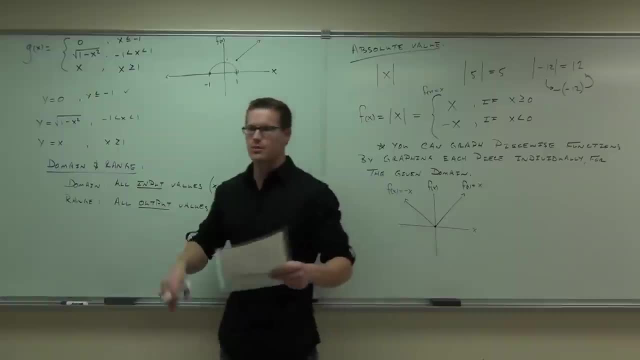 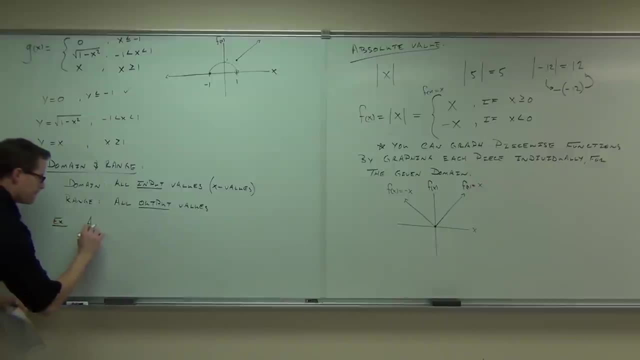 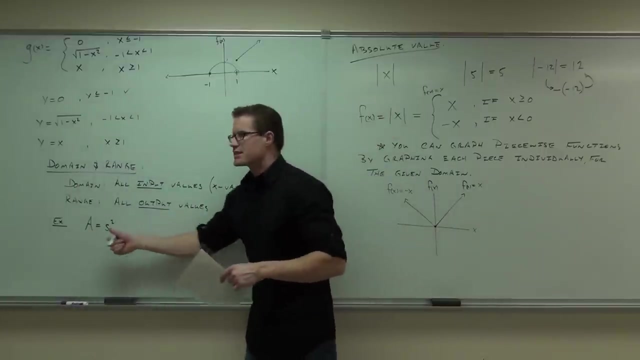 in real life especially, we have some sort of constraint on the domain. Let me give you a couple examples on this. Let's say that I give you an example here: The area of the square, The area of the square. Now, the domain is all the lengths of the sides. 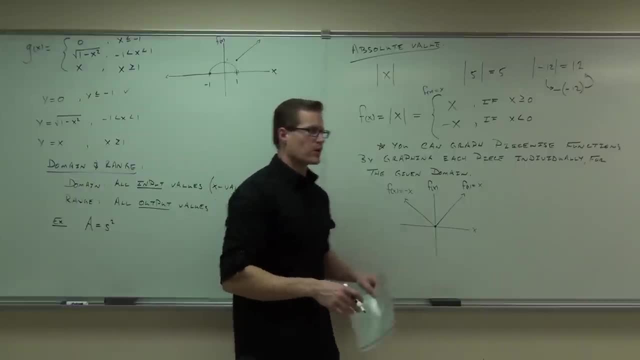 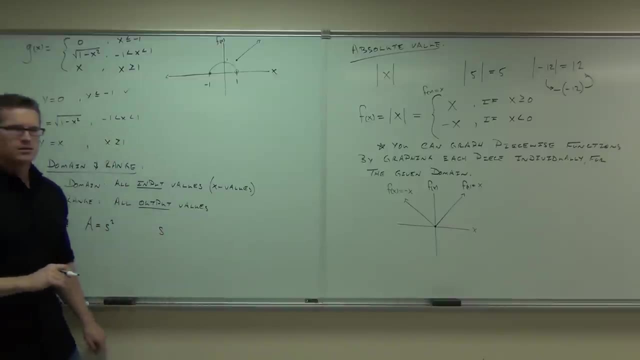 of the square that you could plug into this function and get out an appropriate area. Can you tell me if there's any problems with numbers I plug in here? For instance, does s have to be? is s restricted in any way if we're talking about an actual square here? 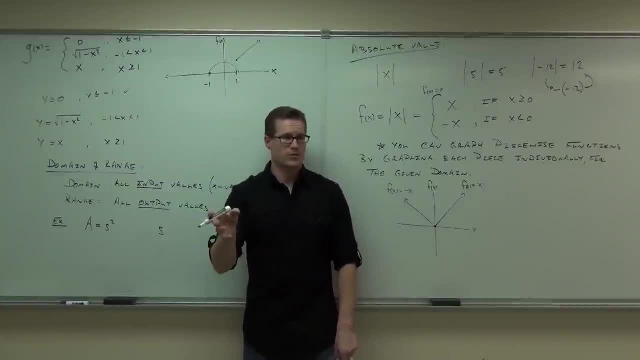 They all have to be the same. They have to be the same. Oh, the sides do have to be the same, but I'm talking about Can't be negative. Why can't it be negative? Because in real life, there is no negative side. 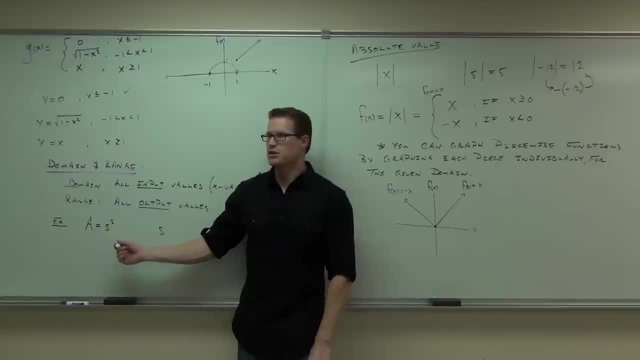 Sure, In the formula you could plug in negative three, couldn't you? It's gonna give you nine. But in real life, can you draw me a square right now with the side length of negative three? Can you do it? Draw me negative three. 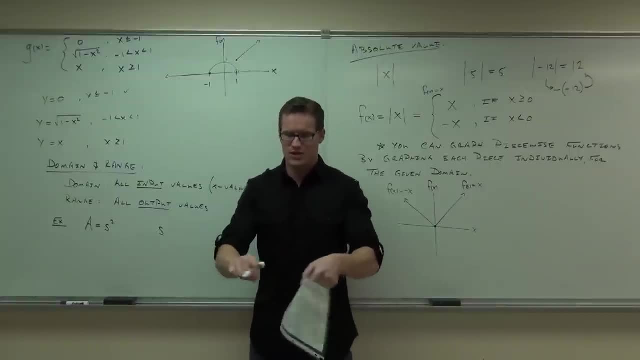 Oh, You can't do it right. You're not gonna make a square that has. if you measure it on a tape measure, it gives you negative three. That doesn't happen because we don't measure actual distances and units of length in negatives. 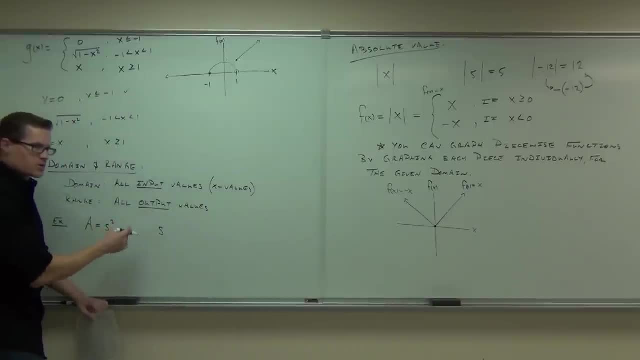 So we'd say here: yeah, the area of the square is s squared, but we have a restriction: The side length has to be greater than or equal to zero. You could have a trivial, a trivial length of s squared, but we have a restriction. 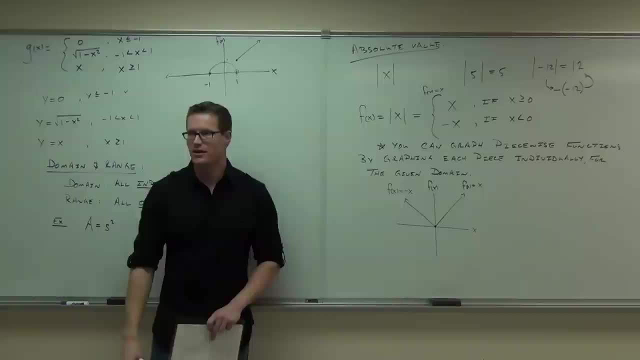 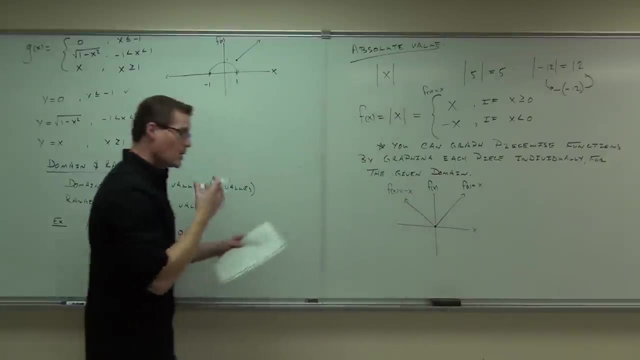 No area. trivial square: here it is, That's, it has zero area, no length of the sides. You could have a zero length, but you can't have a negative. that's impossible. We also could have some formulaic restraints. 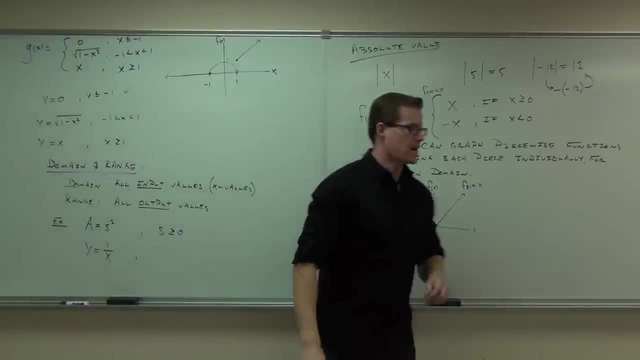 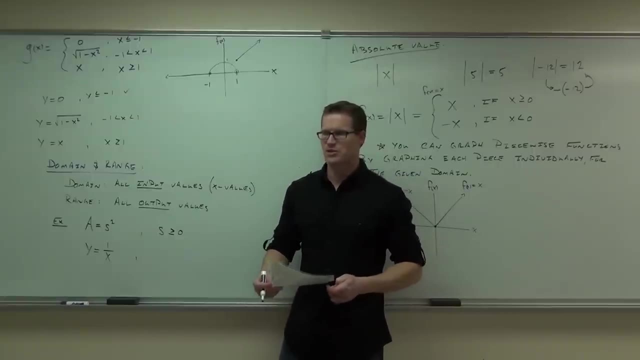 Like that one, Like that one. y equals one over x. Is there any number? I can't plug into that Zero. Sure, why not? It's 75.. Yeah, because your teacher, the first time they showed you a fraction. 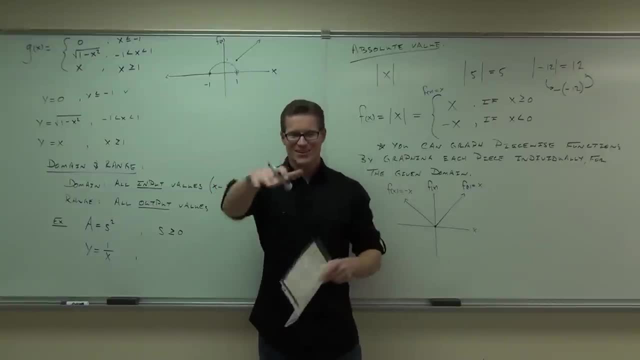 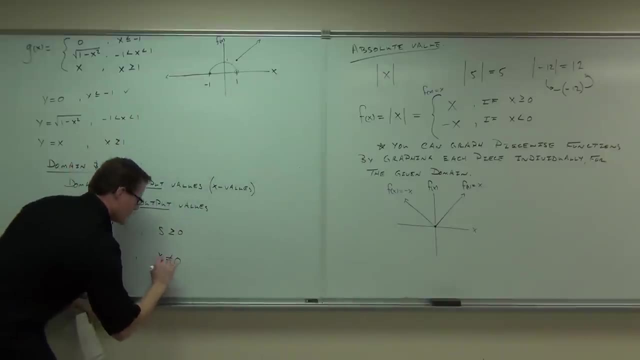 said now, what number can't you divide by Zero? and like, oh good job, little Johnny, you got it right. Never told you why. right, But you can't divide by zero. Any other numbers gonna work: Positive, negative, you're fine, but not zero. 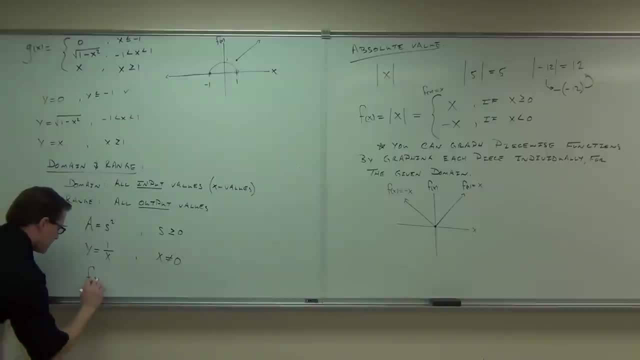 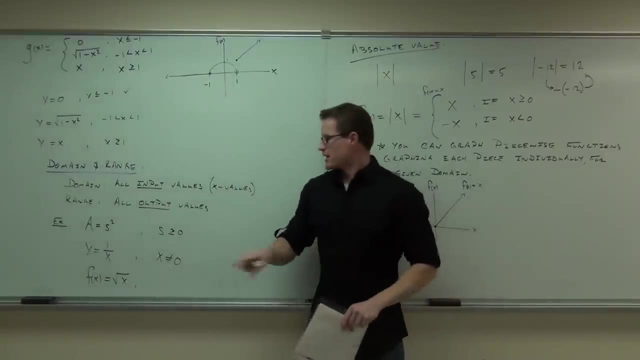 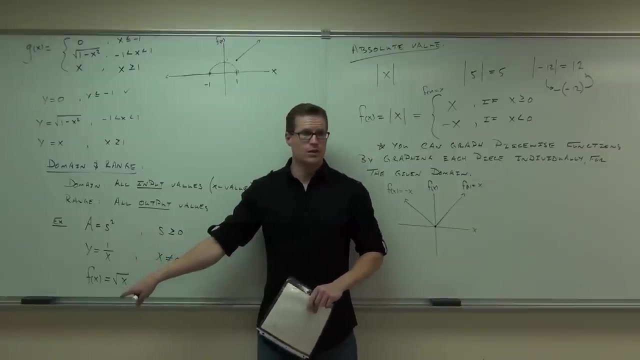 How about this one? F of x equals the square root of x. Here we couldn't have x equals zero. Can I have x equals zero there? Can you plug in zero to a square root? Yeah Well, let me ask you what's the square root of zero? 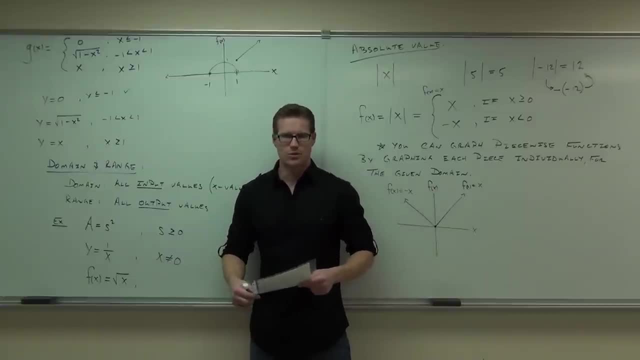 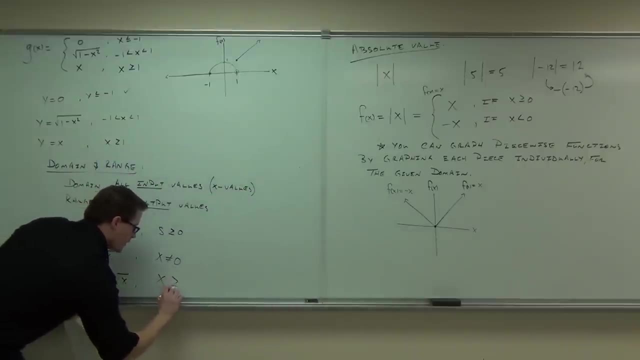 Zero, Then you can do it. What can't you plug into square roots Negative, Yeah, not inside. So we'd say: sure, this has a restraint, where x it could be equal to zero, but it can't be less than zero. 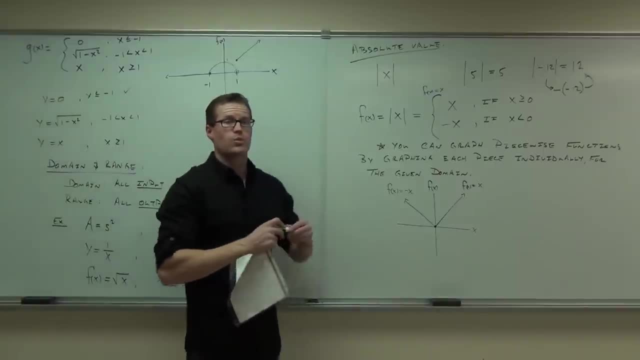 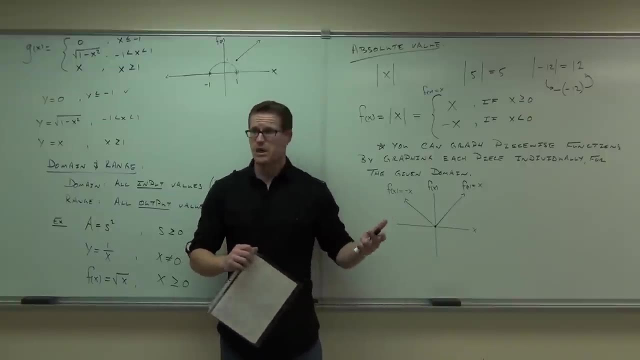 it can't be negative Otherwise. well, in the real numbers at least. now let me make a little statement there. If you're talking about complex numbers, can you do it Absolutely Sure? yeah, you'd have an. i. 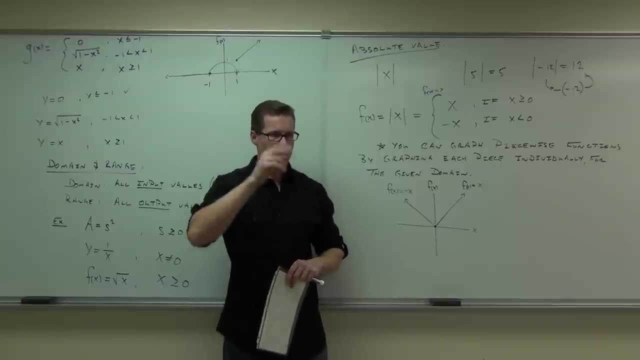 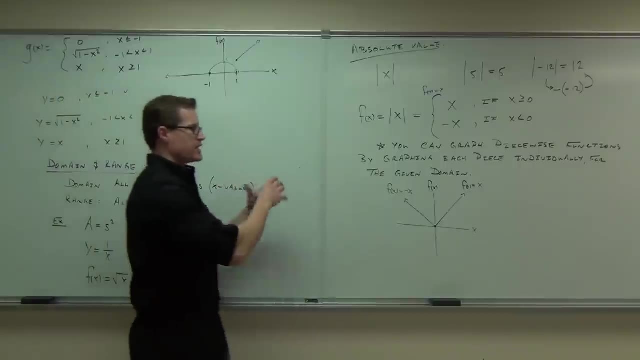 But if we're talking about complex numbers- I'm sorry, real numbers and graphing them on a real number system, well, we can't. We can't do that Now. what we know is that we're going to redefine domain just a little bit. 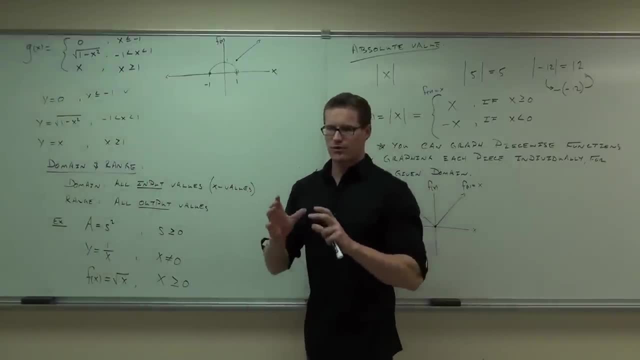 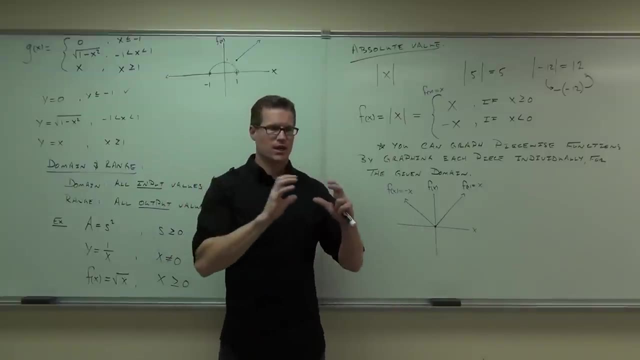 I don't know if your book does this or not, but how we define domain, we're going to define domain in a special way in this class called the natural domain. The natural domain is basically everything that works in the formula, including the maybe natural restraints of the problem. 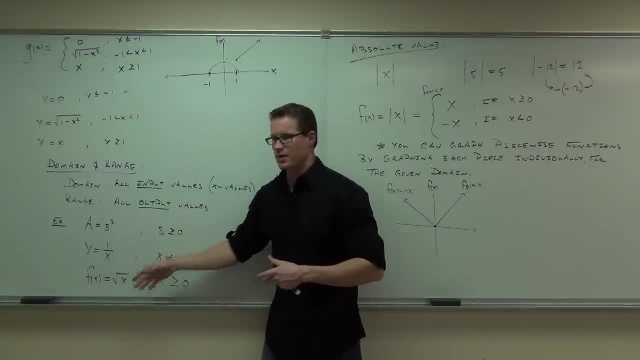 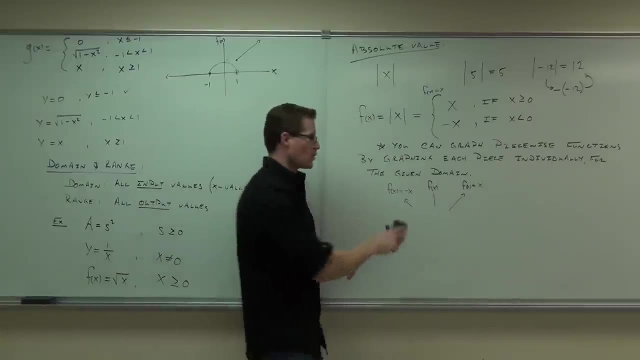 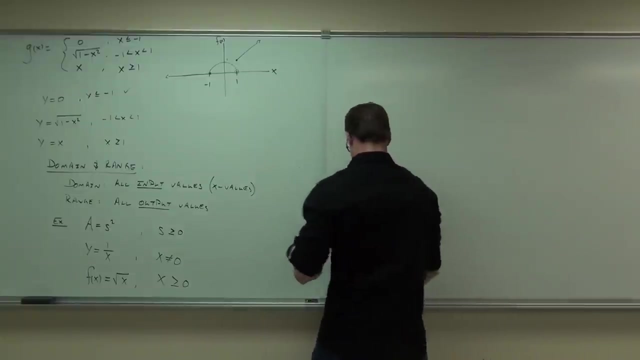 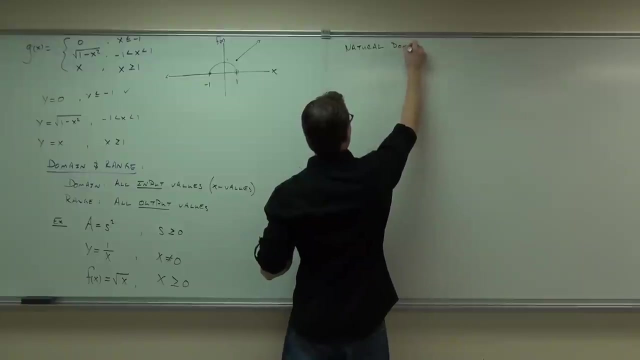 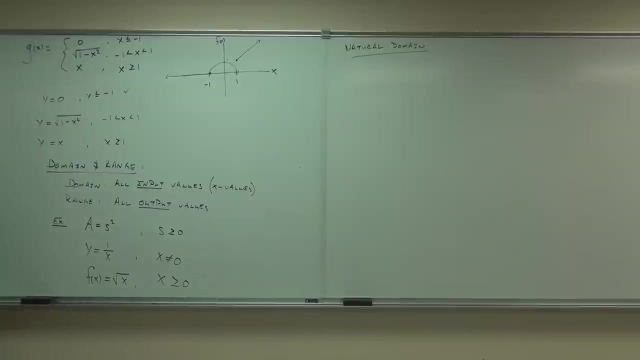 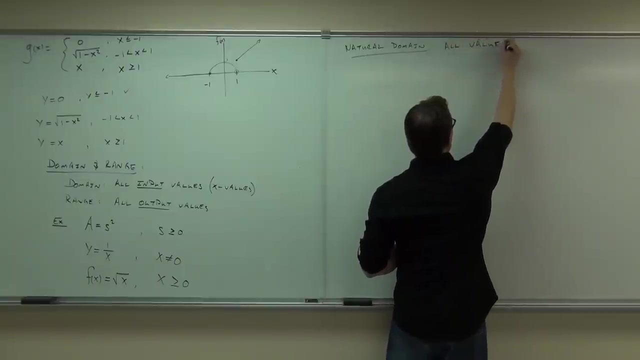 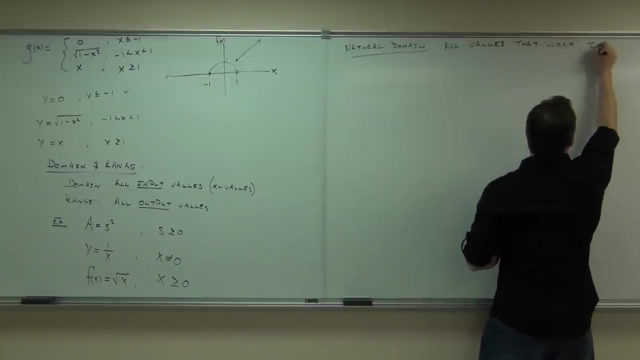 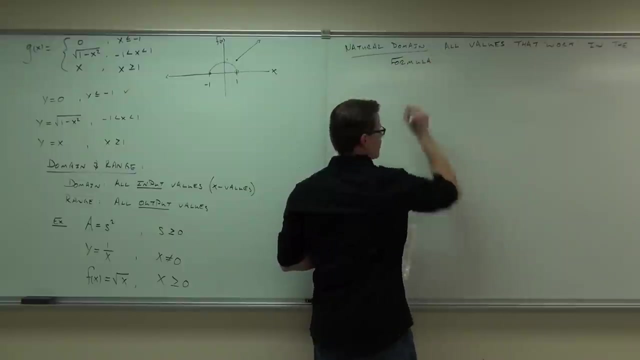 like at the side length of the square or the formulaic restraints of, like a square root for dividing by zero. So natural domain basically means everything that works in your formula or your function, All values that work in the formula. Would you guys like to do some examples of finding natural domain? 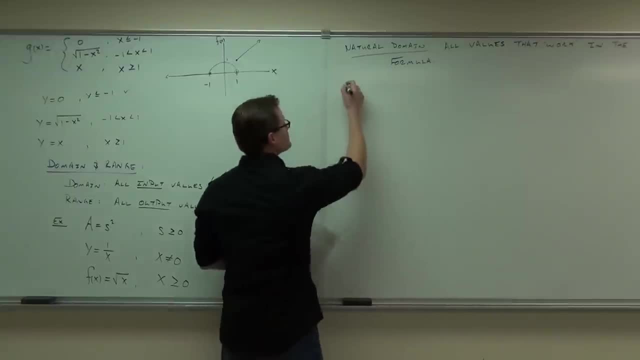 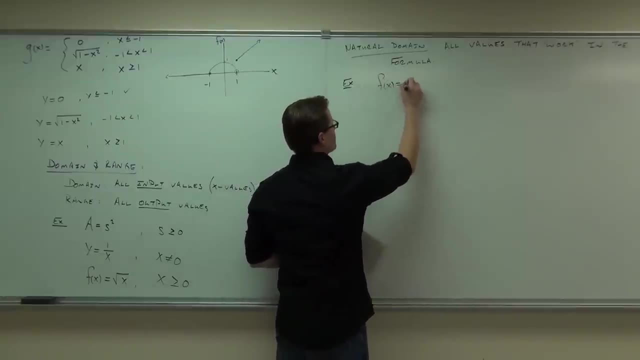 Or domain in general. I was hoping you'd say yes. Natural Domain asked this question. it says: are there any problems with plugging in numbers? basically, So let's look at a real simple one. we've got f of x equals x cubed. 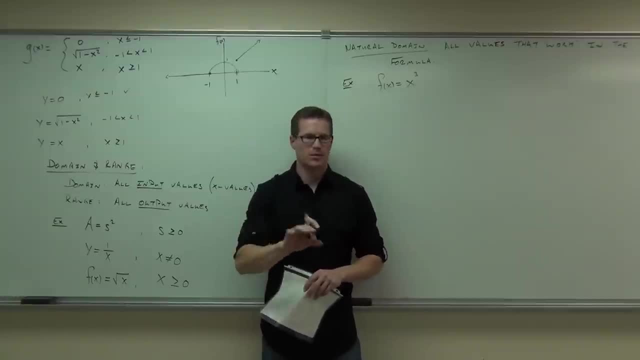 It asks: is there anything that you can't plug in, that you can't input into that? Can you think of anything? Can you plug in positives? Can you plug in zero? Can you plug in negatives? Are there any problems you can think of? 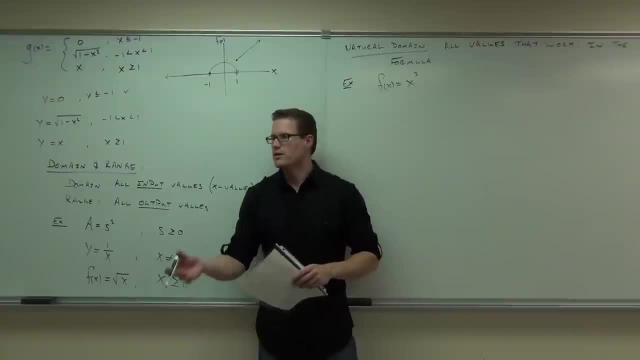 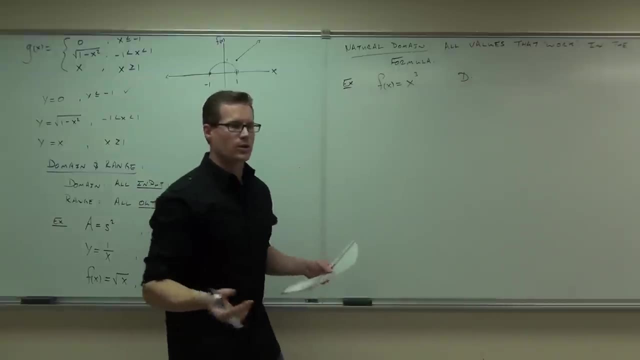 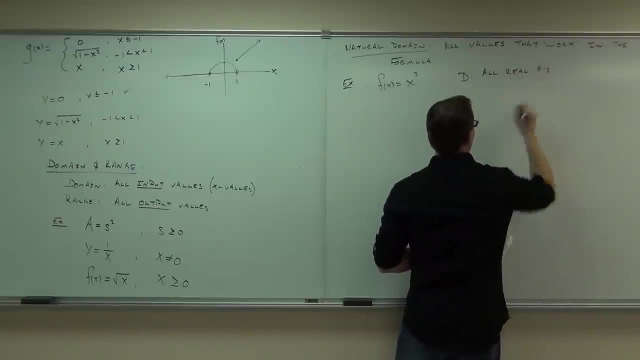 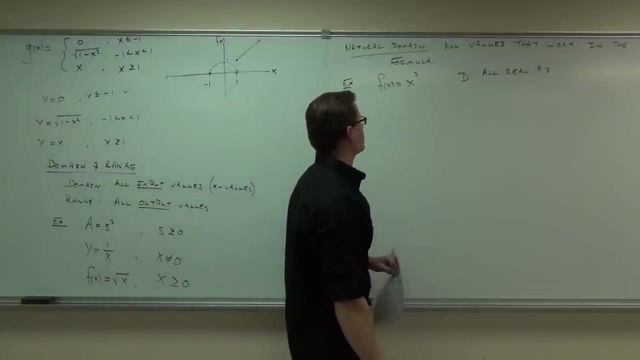 Can you plug in fractions? Yeah sure, You can plug in anything you want. If you can plug in anything you want and there's no problems. what we do is we say: domain is simply all real numbers. All real numbers- For those of you who like to be very symbolic, you can do it differently. 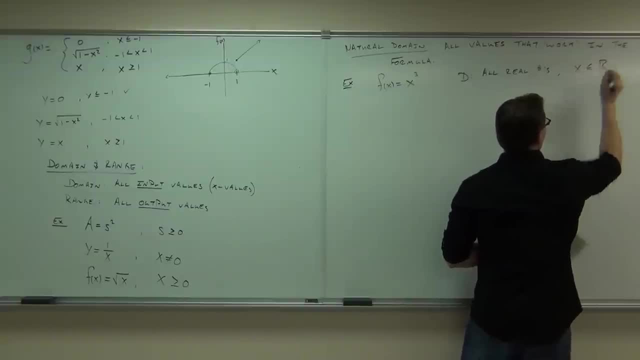 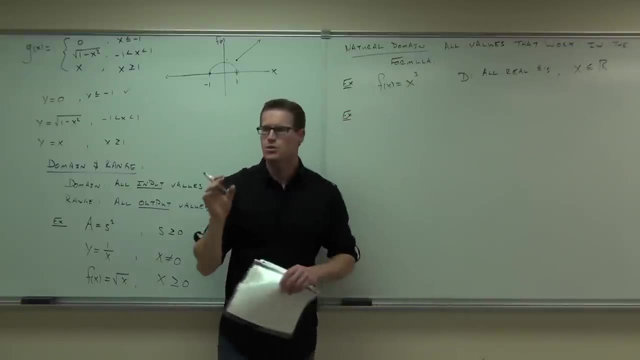 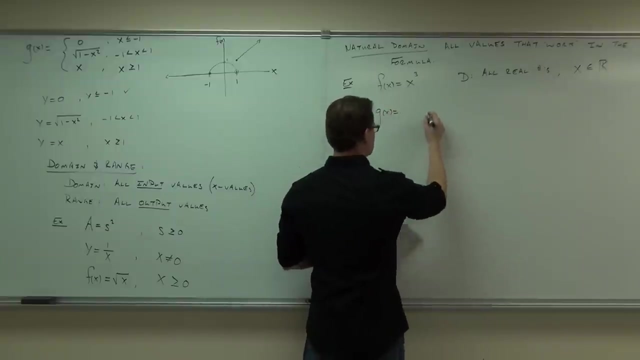 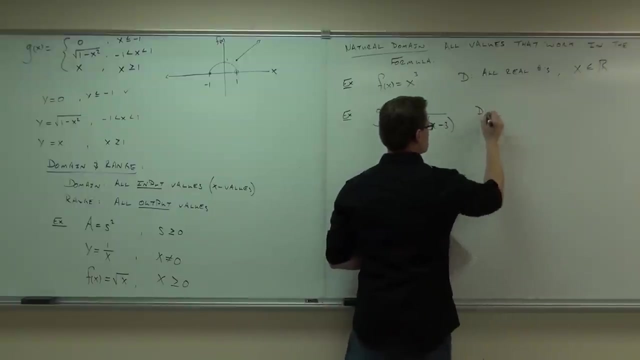 You can say x is an element of the real numbers. That's another way you can say it, So there's no problems there. That says that you can plug in any number within the real numbers and you'll be just fine. paar, How am I good at this? 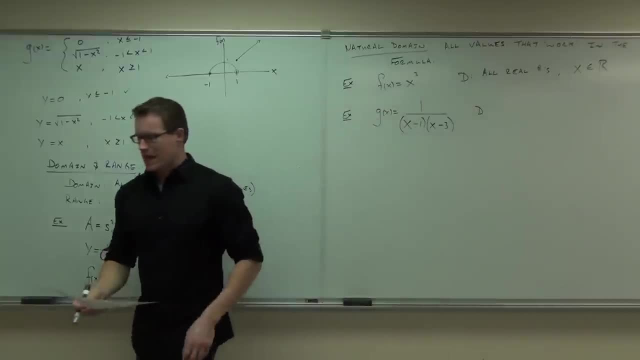 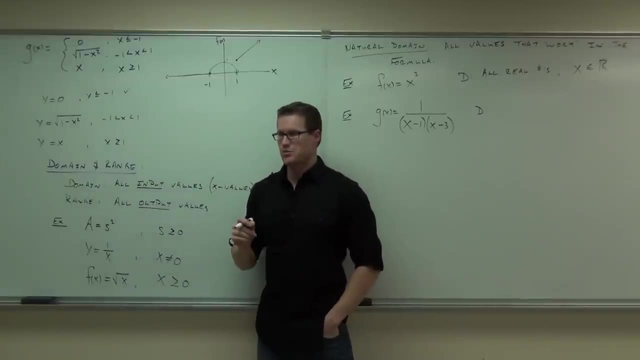 구요. How about this? How about that one? Can I plug in any number? I want to this problem and get something out of it that's reasonable, that's defined. Okay, Can I plug in zero? Yeah, yeah, Even though we can't have zero in the denominator, if I plug it in. 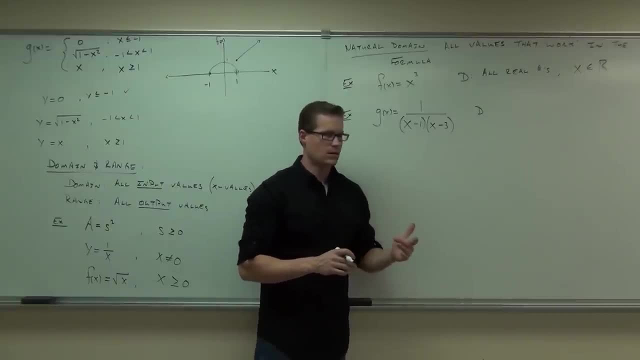 well, I'm not getting zero in the denominator. What numbers can't I plug in One, One, Sure, Now you're doing this in your head, but I want to show you. here's how you find domain in general. 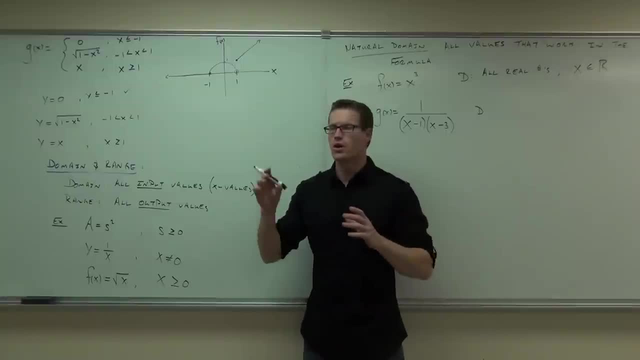 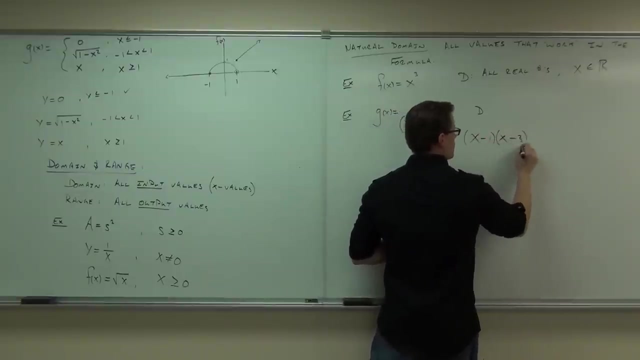 You look for situations where you could have problems. Those situations are roots- square roots specifically, maybe fourth roots- And denominators, To find out what your domain is really. here's what you're doing in your head. You're saying: I want to make sure that I know that if this denominator is equal, 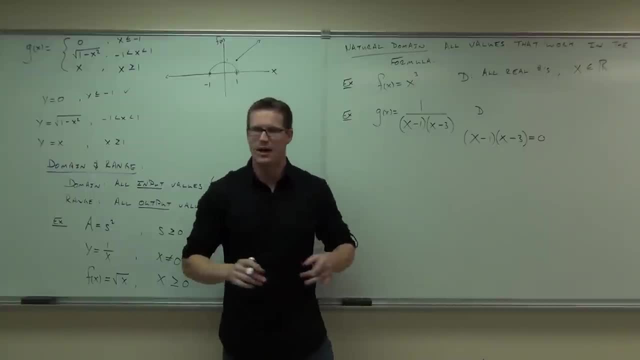 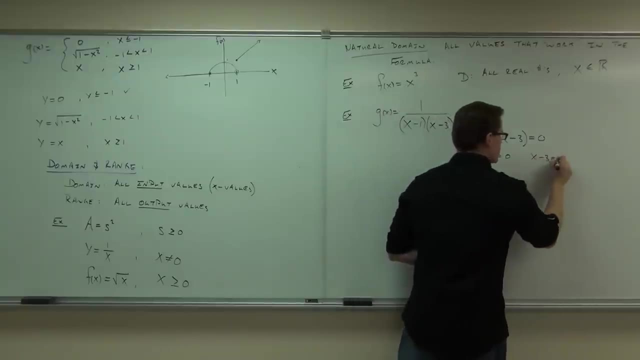 to zero. I've got a problem here Now. the zero product properties didn't come up with their answers. It says: I know X minus 1 could possibly equal zero and give me a problem. I know that X minus 3 could possibly equal zero and give me a problem. 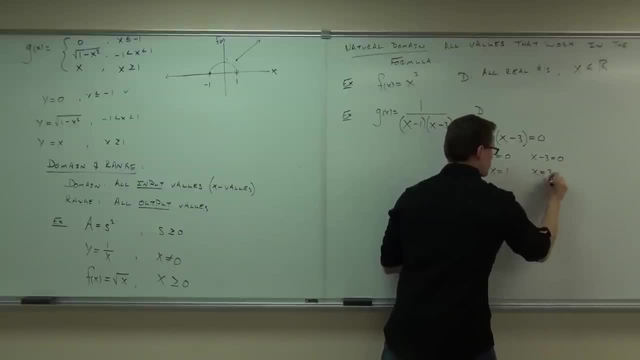 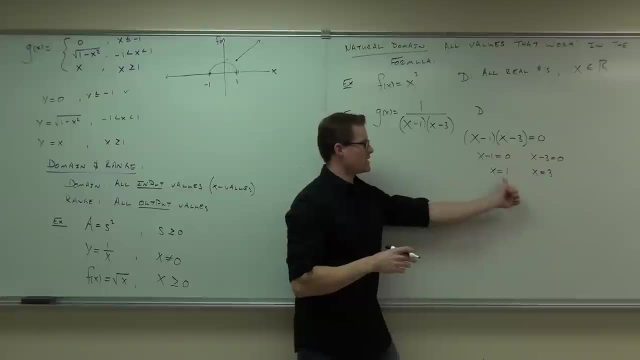 If I solve those, I'm going to get your answers of 1 and 3.. Mathematically, that's what you're doing right here. Do you guys see what you're doing? You're saying: I can't plug in 1,, I can't plug in 3, because if I do, bam, it's going to give me zero. 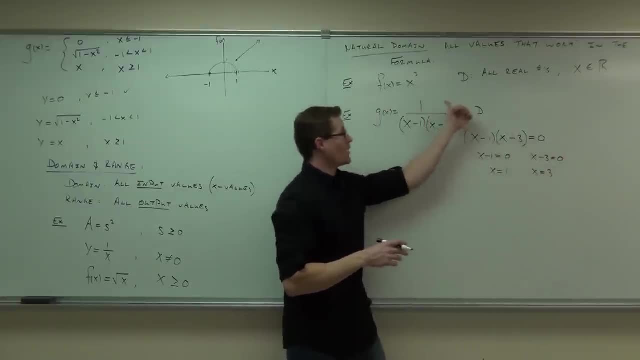 And even if I multiply it by something, it's still going to give me zero, and I know I can't have zero on the denominator of any fraction. So by setting a denominator equal to zero or not equal to zero is how I used to teach. 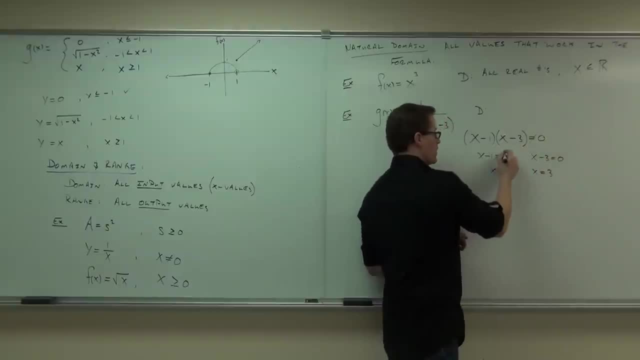 in some other classes. you can do this too. I know it can't be equal to zero. therefore, that can't be zero. that can't be zero and these two things I cannot have X equal to zero. That's another way you can solve this problem. 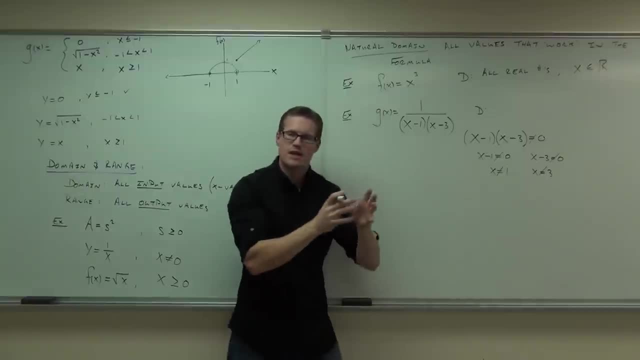 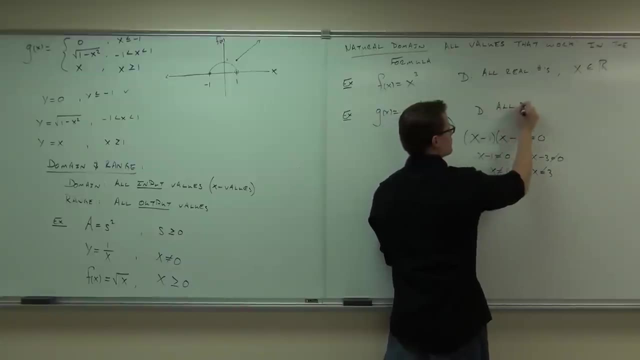 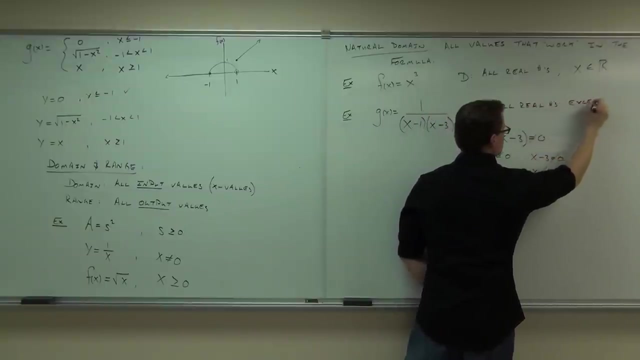 Another way you can do it by setting that equal to zero. solving it down, you find out your problems within your domain for denominators. So here we'd say: X is all real numbers except or but. X does not equal 1, and X does not equal 3.. 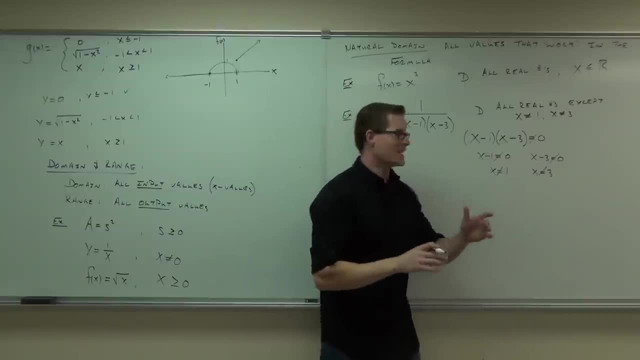 Please don't ignore that does not equal. okay, because if you do this- I know I just used equal sign and that's what a lot of you have been practicing doing for your math careers- but if you do this, except X equals 1 and 3, that says 1 does work. do you see that? 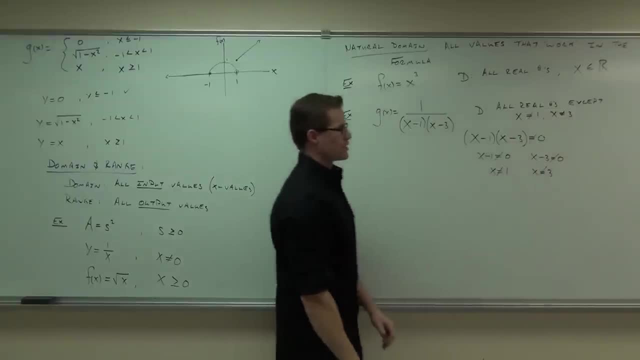 We have to have the not equal 2.. So once you find those problem numbers with the not equal 2, we're going to find out later that what these things are. if you cannot simplify them out of your function, those are going to be asymptotes, vertical asymptotes. 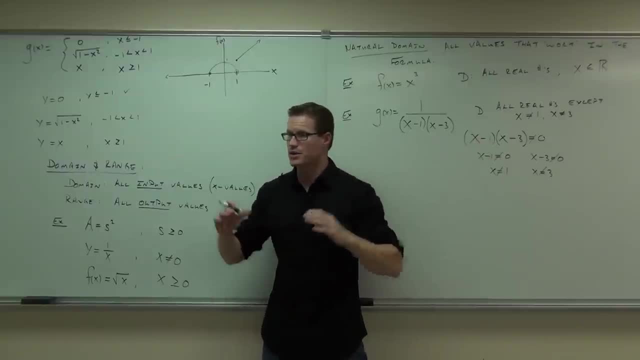 So this is not going to be defined at X equals 1,. it's not going to be defined at X equals 3, those are either going to go up like that Looks like I'm doing my dance moves, but that's what they're doing. 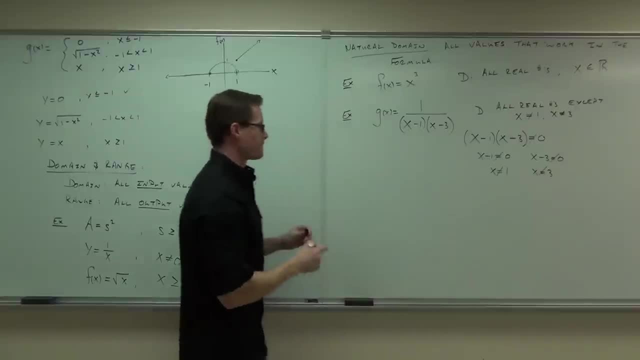 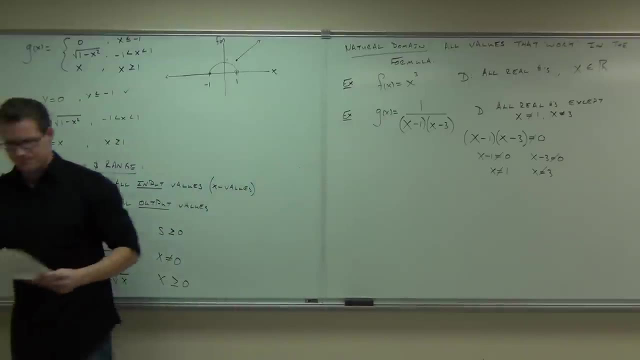 They're going to go up at an infinity down infinity, something like that. Do you guys feel okay with this particular domain? Let's try a couple more. I want to get through a few more problems here. Okay, how about this one? 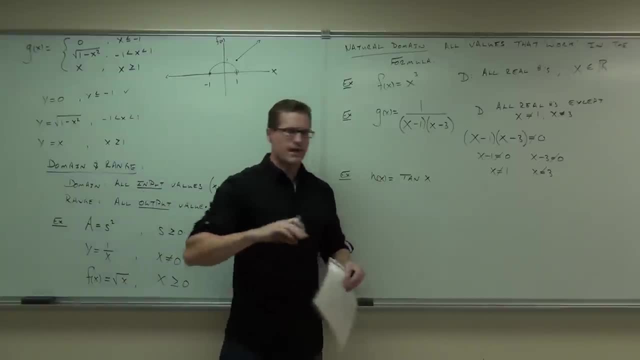 How about tan X? Tan X, Is that defined everywhere? Sin goes like this right and cosine goes like this. Does tangent go like this? No, How does tangent go X? It makes those kind of weird S's of the snakes all the way down your paper. 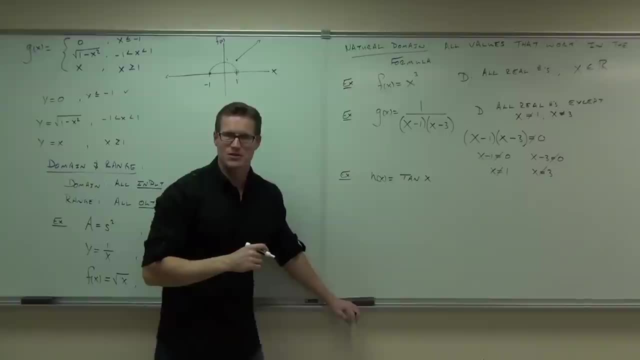 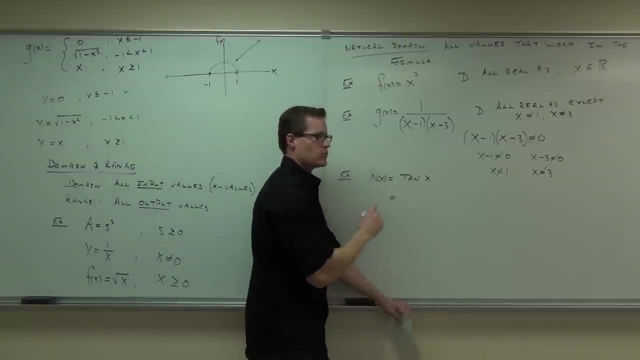 Why does it do that? Why does it do that? Listen to rhetorical. Why does it do that? Sure, it's undefined. Why? Why is it undefined at certain points? Skipping the X value. Fill this in Sin Sin. 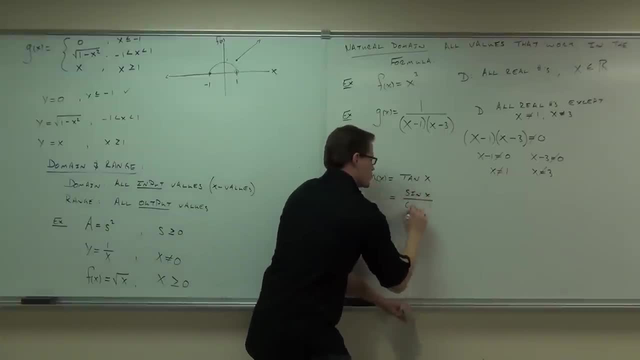 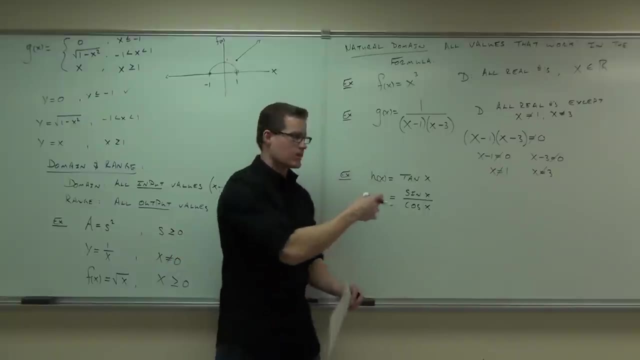 Cosine, Cosine, You remember how? I just told you how functions aren't defined if they have denominators, where those denominators equal zero. Well, check it out. If we look at this, this is tangent right. If we set this denominator, I'm going to use the not equal to zero. 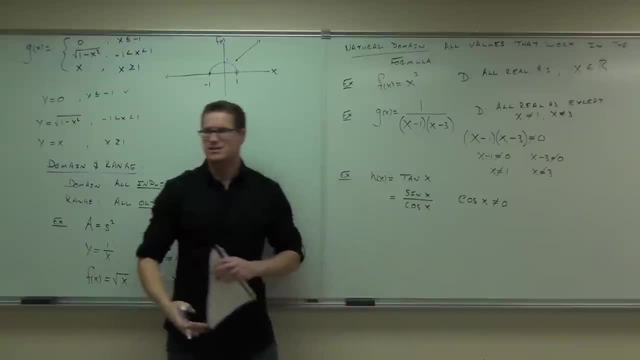 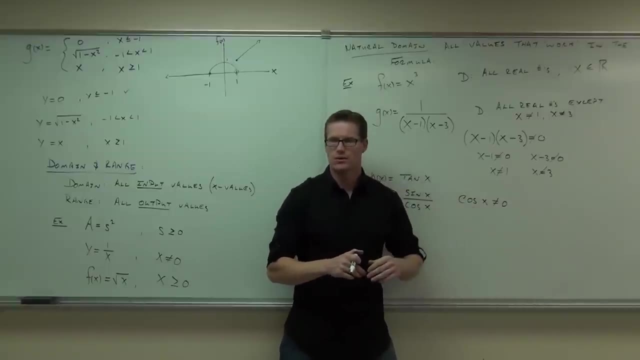 because we know we should not have that equal to zero. If cosine X can't be equal to zero, which is what I'm saying here, what values of cosine make it equal to zero? Where Do it in terms of radians? Pi over two is one of them. 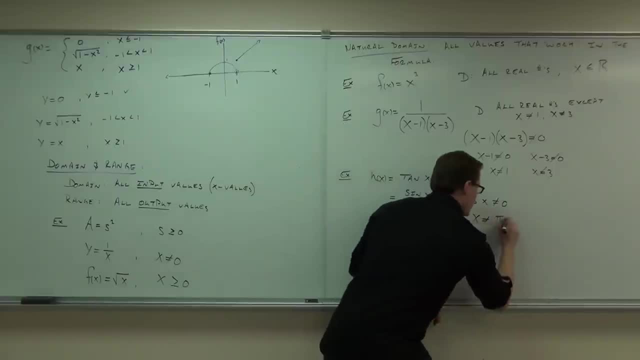 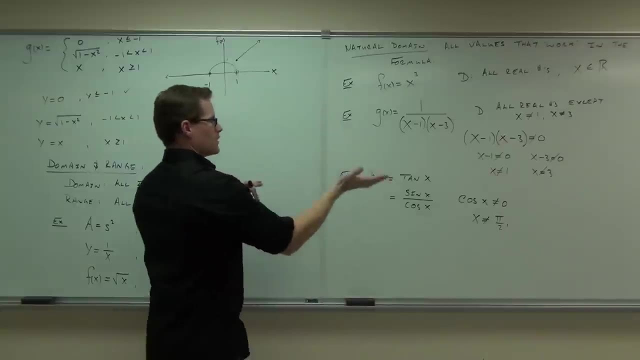 So X can't equal. that's why I'm using this right here: X can't equal pi over two. X can't equal. if you keep on going, you're going to get. let's see for you guys. here's pi over two cosine zero. 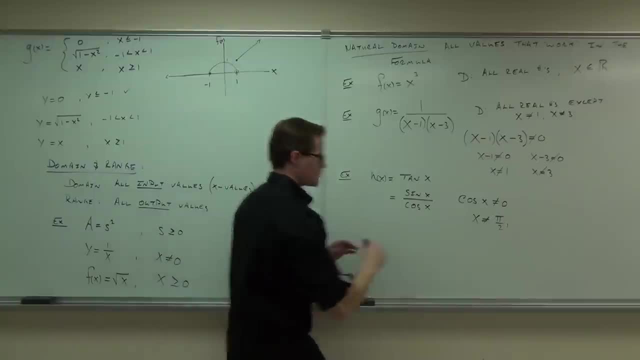 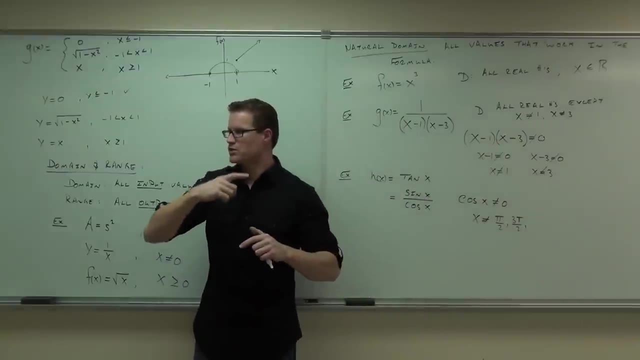 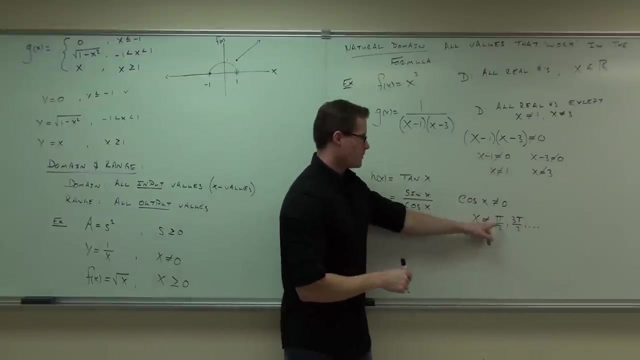 True, You're going to keep going to three. pi over two. If you keep going around the inner circle you're going to get a lot of different values. It's going to keep repeating, both backwards and forwards, every pi from that. So pi over two plus or minus pi k pi. 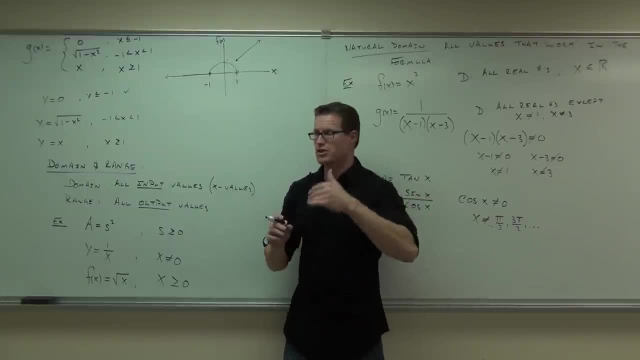 where k can be positive or negative integer, it's going to give every part where tangent is not defined, Because Cosine will be zero at those points. Do you see why this works the way it does? Do you see why the tangent is not defined at those? 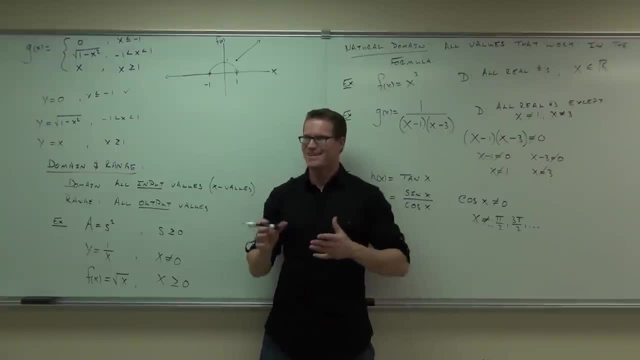 Simply because cosine is not defined. at those points You guys see that Kind of neat right. It doesn't matter if the numerator is equal to zero. Sine of zero over something that's defined, That's okay, But something over zero, that's not okay. 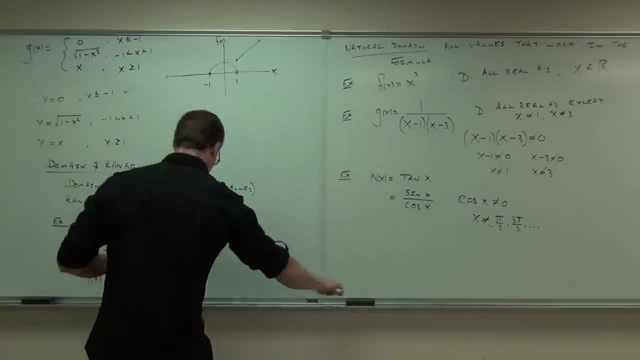 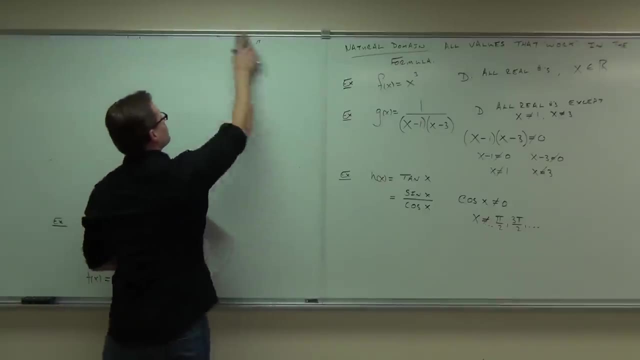 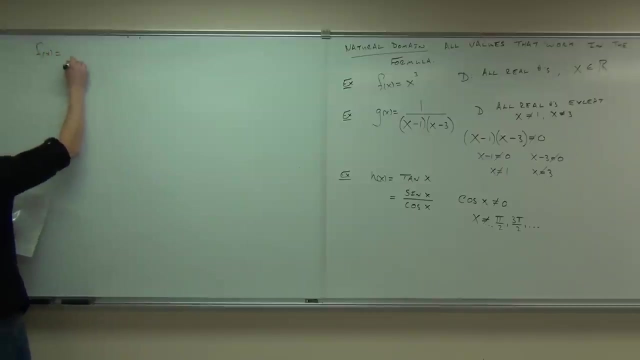 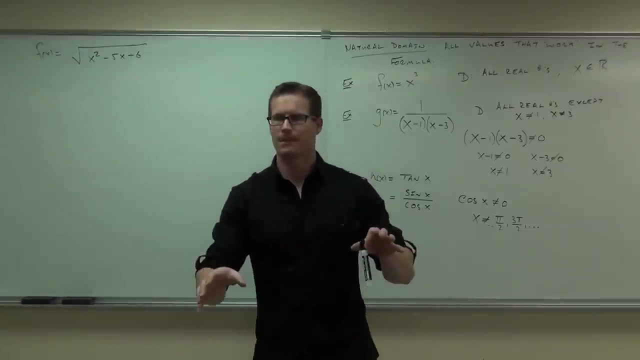 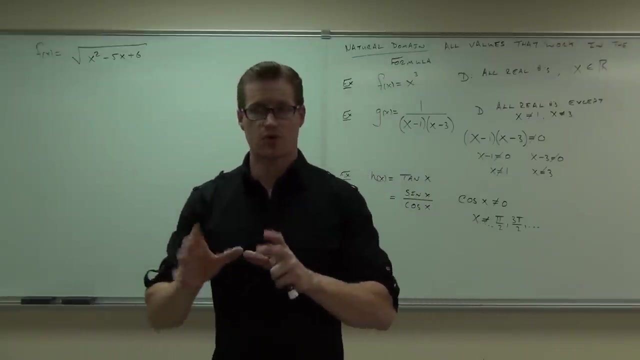 Okay, last one we're going to talk about and then we'll call it a day. It's a Froot. Do I have any denominators here? Any denominators? anything Over anything, And I think, over anything any. this square root. 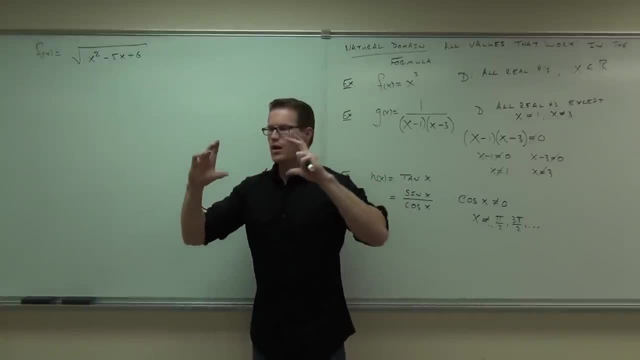 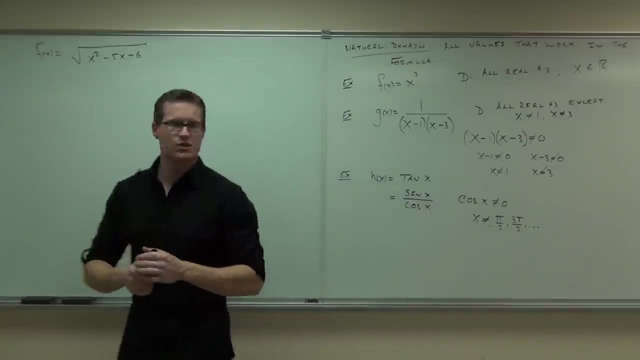 What do you know about things? the radicand, that's what's inside the radical. what do you know about the radicand of square roots? They have to be positive. So when you're dealing with these roots, denominators, I showed you how to do that. 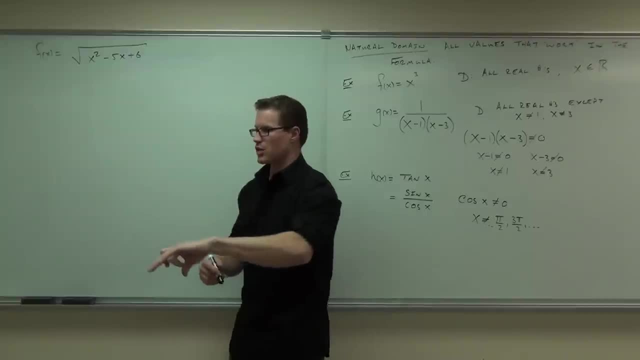 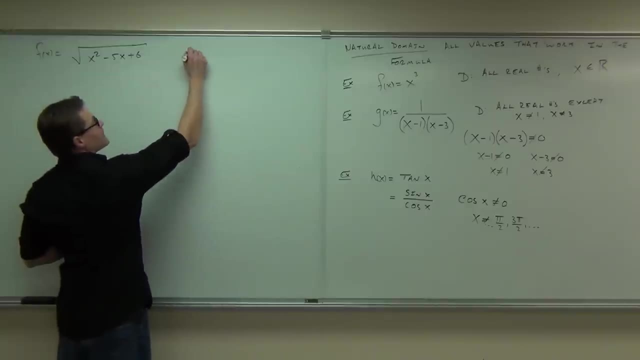 What you're going to do is set the denominator equal to zero or not equal to zero. solve that down. that will give you your problems in natural domain. As far as the radicals go, you know for a fact that this thing is going to have to be bigger than or equal to zero. 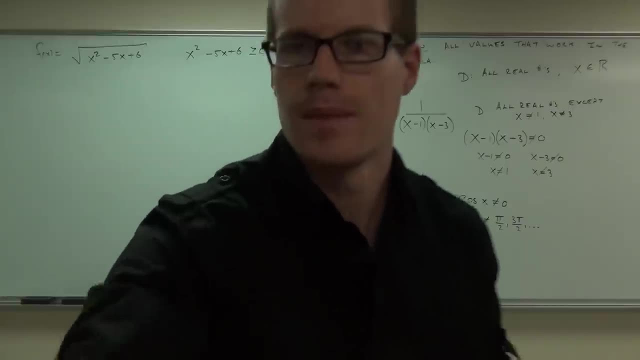 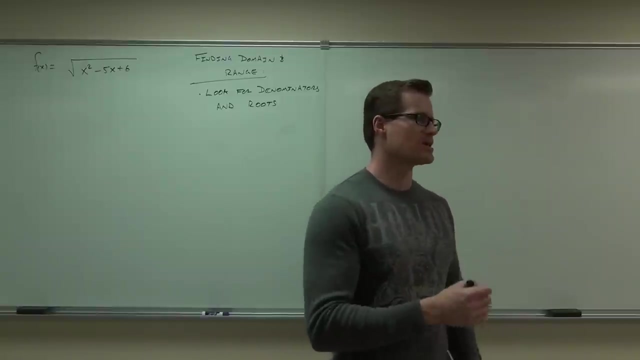 All right, you know what we're going to start this next time I'll show you how to do that. All right, so we're going to continue finding some domains and some ranges of some functions. Now, basically, when you're finding what I said was the natural domain, that's just really what works in a function. 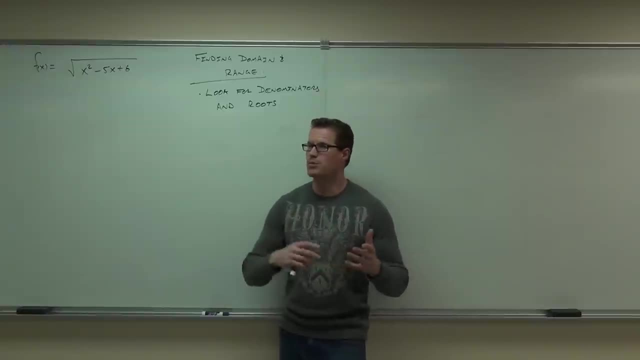 what we've got to do is look for our problem areas. If we can define our problem areas, that really defines what we can plug in and, specifically, what we can't plug into a function. Really, what that comes down to for us is: you're always looking for denominators and roots. 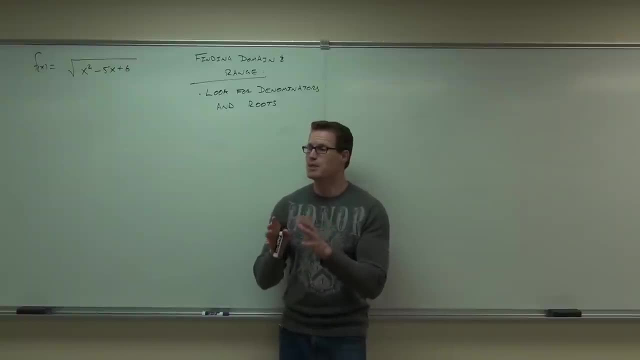 If you have denominators, you know that at some points you might be undefined. If you have some roots, there might be some ranges of numbers that you can't even plug into your function. So with us up here we're going to have an issue inside that root. 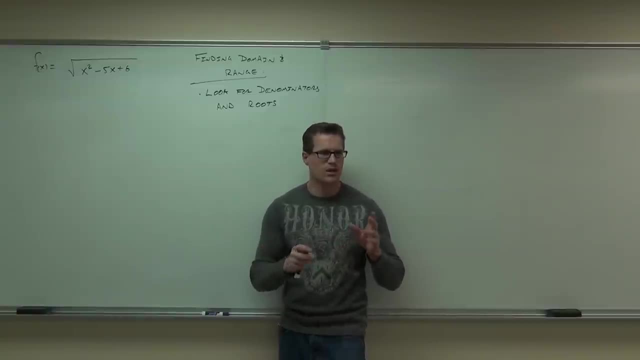 What do you know about square roots? I think we might have talked about this last time. What do you know about those? What numbers can't you have in there Now? can you plug in a negative here? You might be able to, provided that when you work it through the radicand, the inside of your radical, it's positive, That'd be fine. 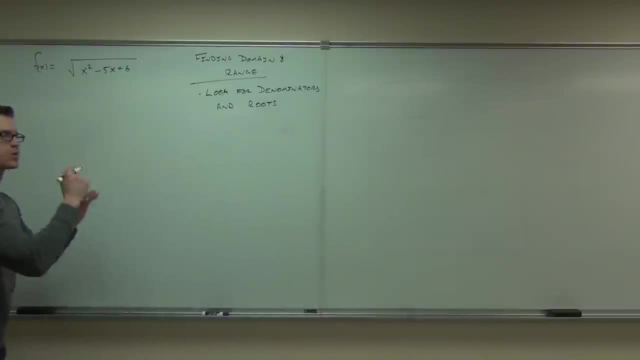 Really what we want. with any root, with any square root, we want the inside part, the radicand, to be greater than could it be equal to zero. Is that okay to have a root with a zero inside of it? Sure, So really, we want this. If you remember from last time, we had some denominators. 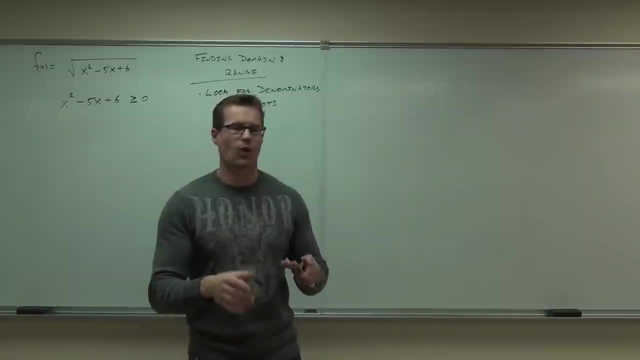 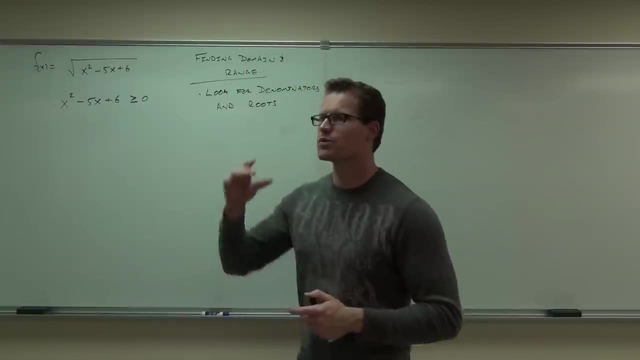 What we did was we set our whole denominator equal to zero, or I even used the not equal to zero because it can't be zero. And you can solve it that way with the equal to zero, finding out your problems With our roots, what we're going to do. 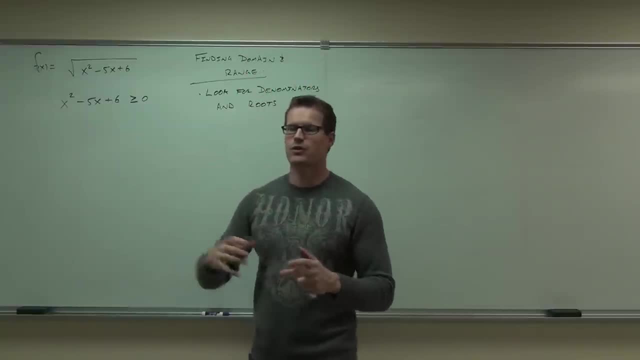 is make the inside greater than or equal to zero. We're going to find out those ranges at work. Oh my gosh, that's a quadratic inequality. That's math. See, that's intermediate algebra days for you. How do you do that? 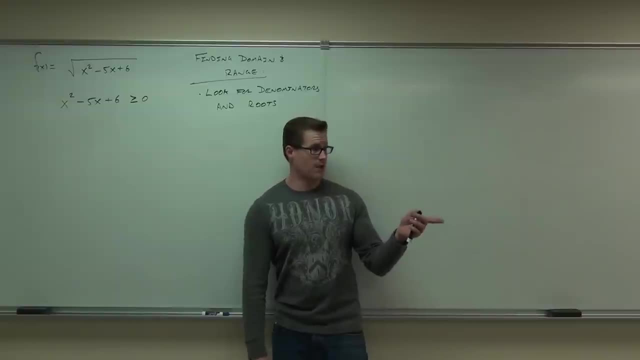 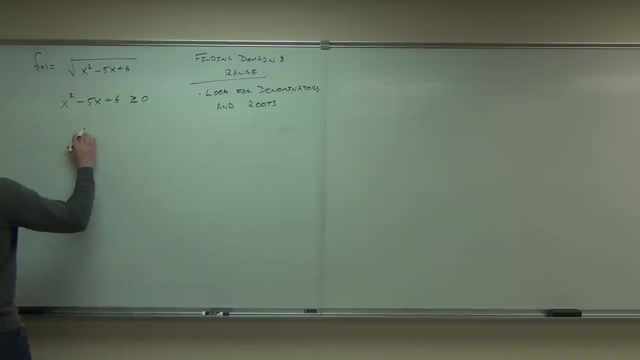 What would you do in order to solve that problem? We would definitely have to factor- at least You probably can see that because it's a quadratic right. Go ahead and factor that, See what you get. Oh, let's see, I think so. 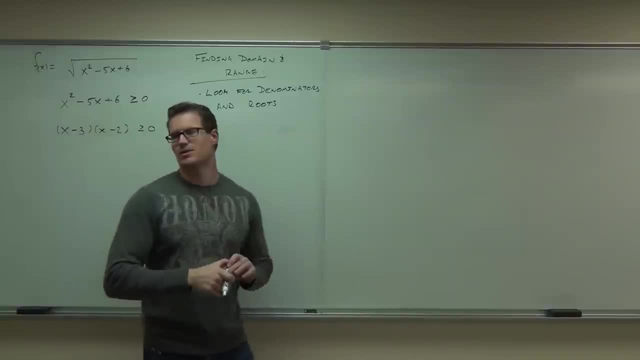 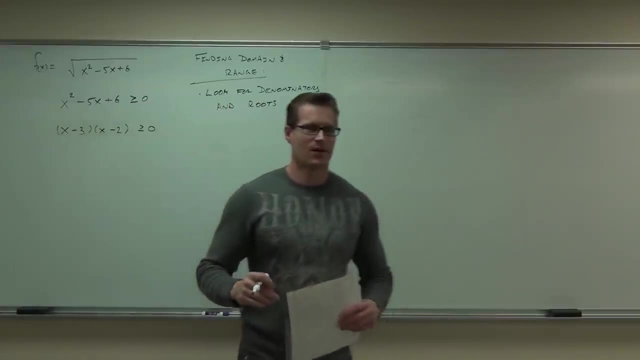 Minus three, minus two. Did you all get that too? Okay, we passed it back to him. I was scared if we didn't, My gosh Alright. How do we do the rest of it, though? Set it equal to zero. 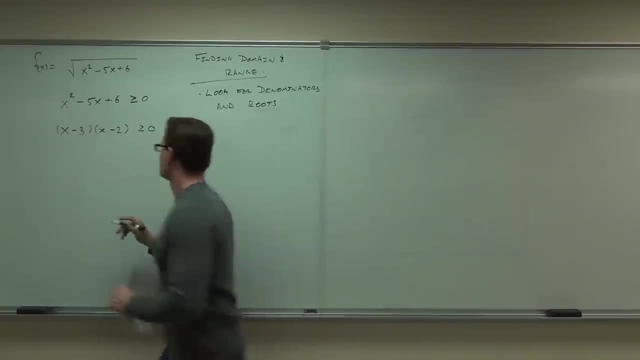 If we set each one equal to zero. you know what it's going to tell us. It's going to say that x is greater than or equal to three, And it's going to say that x is greater than or equal to two. Do you guys see that? 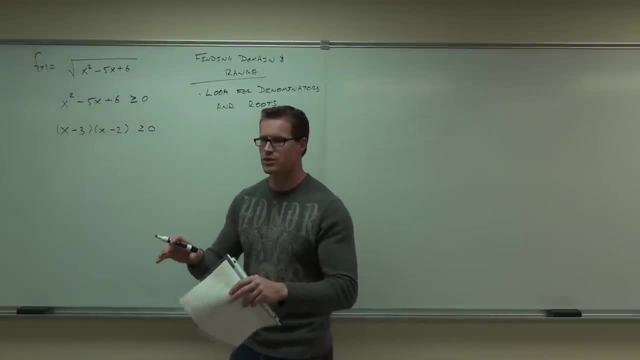 Which actually is not going to be the right thing for us. I know you want to right because you're so ingrained in saying: make this equal to zero. make this equal to zero by the zero product property. However, we don't have the zero product property because that's not an equation, That's an inequality. 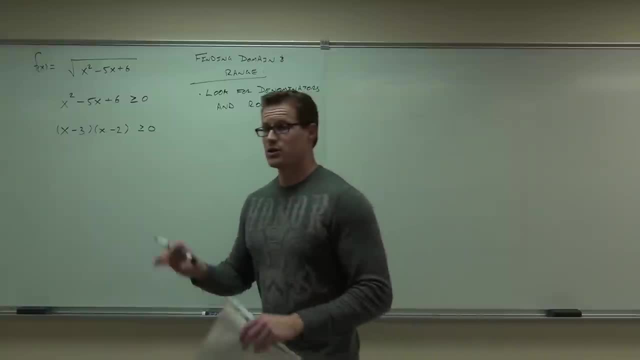 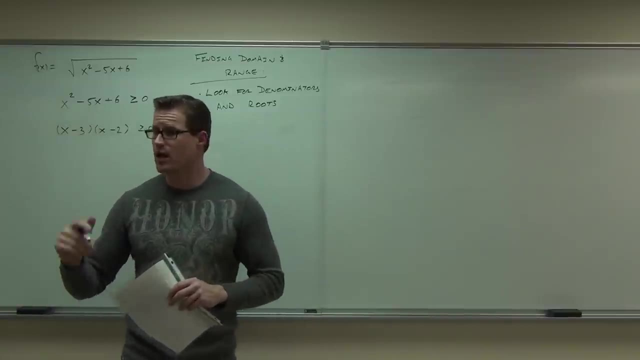 If you know how to deal with your inequality. here's what you do: You do find the places where x would equal zero. You kind of temporarily set it equal to zero in your head. You find those points. Hopefully, in your head right now are the points: x equals two and x equals three. 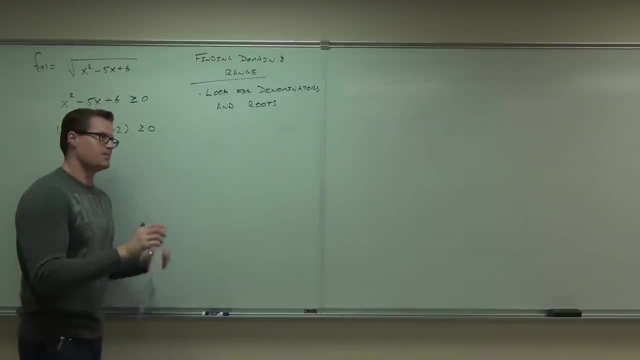 Do you guys see those points? Here's what you do with this. This is called a basic version of a sign analysis test, So we know that x equals three and x equals two are some important points for us. Here's what you do with those points. 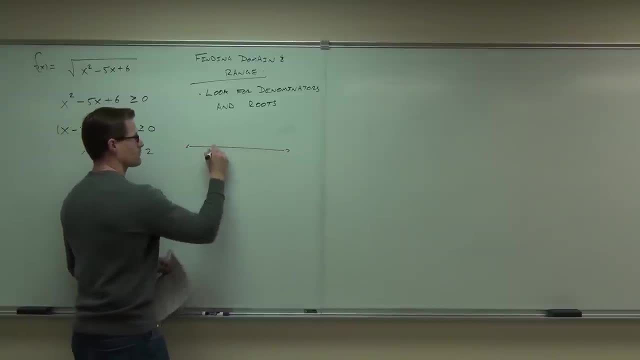 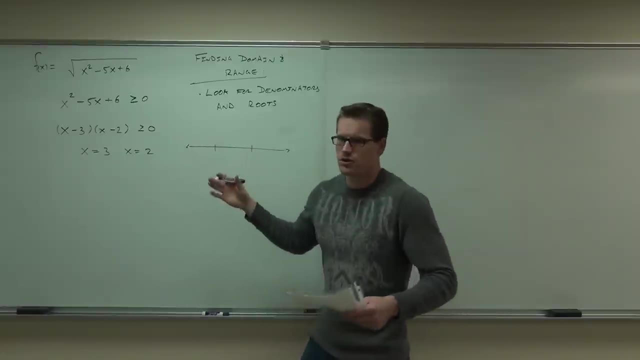 I want you to make up a number line. Put those points in order on your number line. So which one's going to come first for us, going from left to right? Me Sure, This is basically a graphic representation of your interval. what's going to work in your function here? 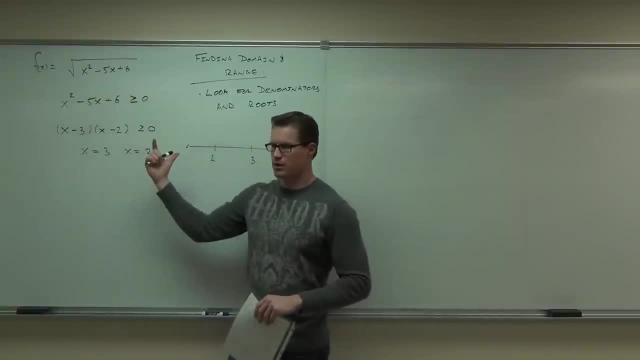 So notice what we've done. We've said, okay, we know the inside has got to be bigger than or equal to zero. We factored it. We have some key points here. We've got x equals three, x equals two. We put them on a number line. 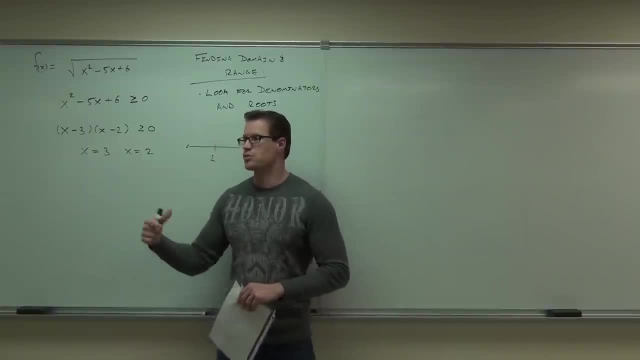 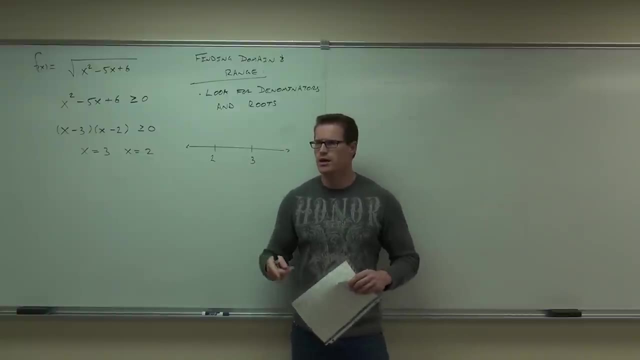 Now here's how to determine when you're going to be okay in your function and when you're not, If you test a point for each of these intervals. how many intervals do we have? Three? Yeah, it's like you're slicing bread, right? 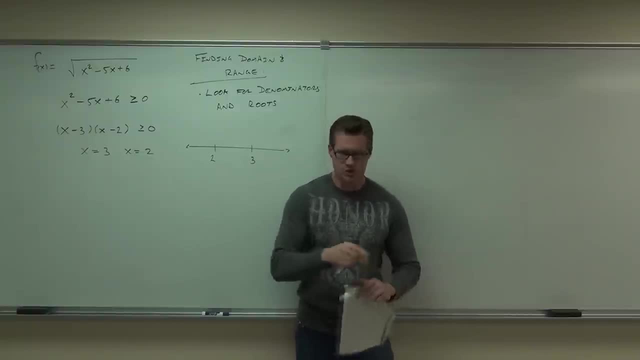 If you have a loaf of bread and you cut it once, you get two intervals. If you cut it twice, you get three intervals. So you get three pieces of bread. Here we have our three intervals. If you test each of those intervals with a point in your expression here, it's going to tell you whether it's positive or negative. 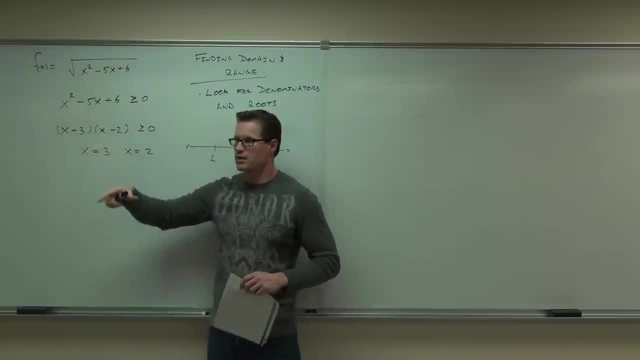 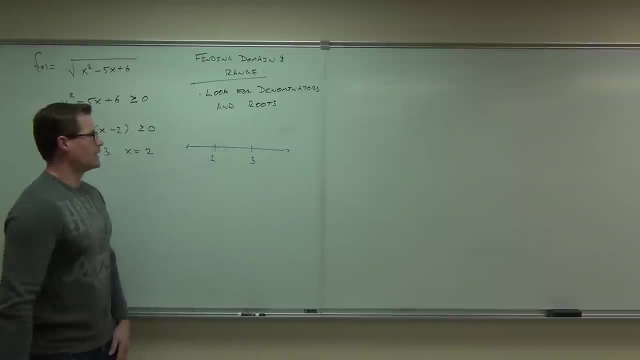 That's going to tell you what you can plug into your function and what you can't. So let's try this, You'll see what I mean. after we plug in our first point, Can you tell me what is a point to the left of two? 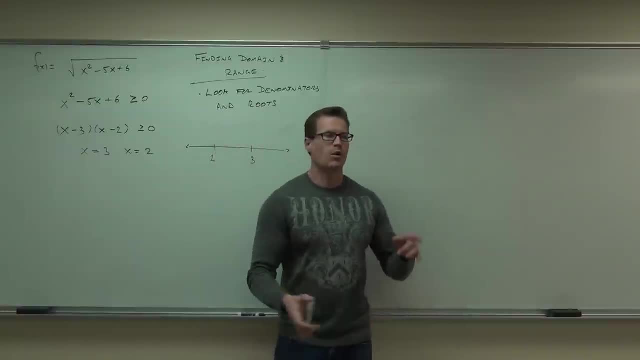 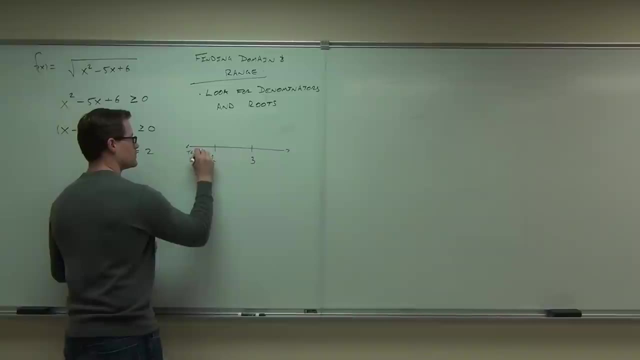 Zero, Zero. That's the easiest one to plug in. I want you right now to test zero, So we're going to test zero. Test zero on the inside of my function. If you plug in zero, how much are you going to get? 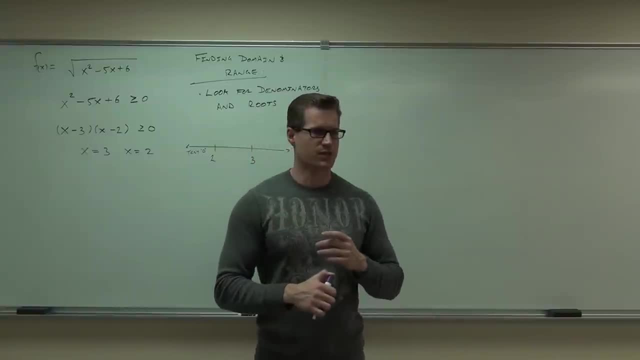 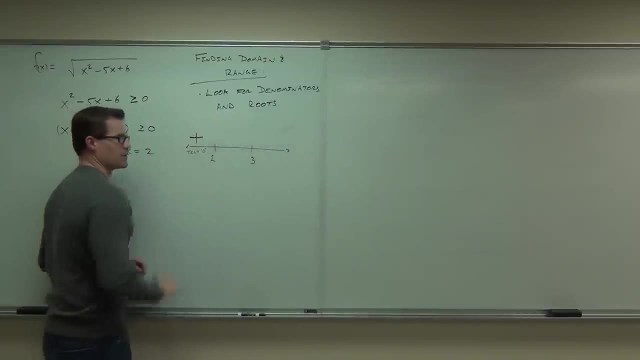 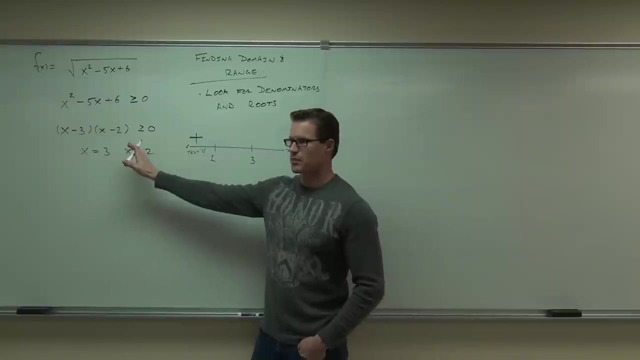 Six, Six, Wait- positive six or negative six? Positive six, So would you say that we came up with a positive answer? Yeah, so this is going to be a plus. What that signifies is that every number- try it if you want- every number to the left of two is going to give you a positive answer. 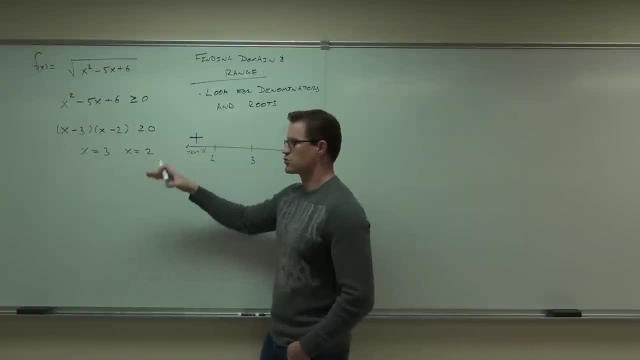 Are you with me on that? Have you tried one? Go for it. You can try it. Try any negative number. That's going to give you a positive there. Do you believe me? If you don't, well, just spend the rest of your life trying out numbers, and then you'll come back to me. 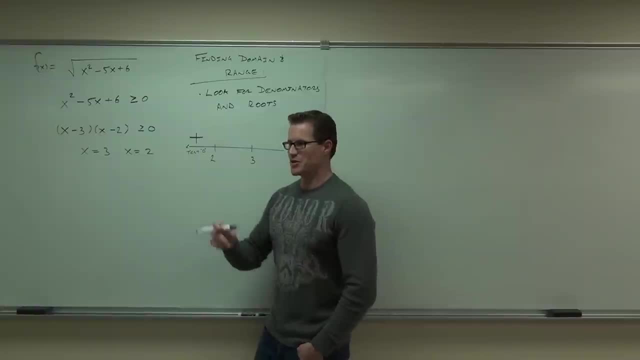 I believe you. when you're like 80 years old and I'm dead, You can put it on my epitaph for me later or something. So we've tested every number over here. We know that every one of them is going to be a positive. 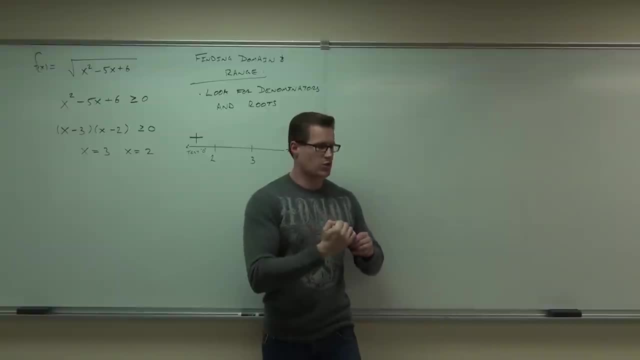 The reason why we know this. if you think about it, it's a quadratic right, And you've just found the roots right. It's actually an upward-facing quadratic. So it goes like this: Positive, positive, positive dips down at 2.. 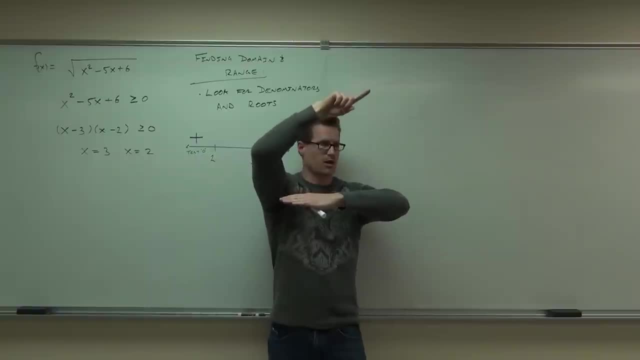 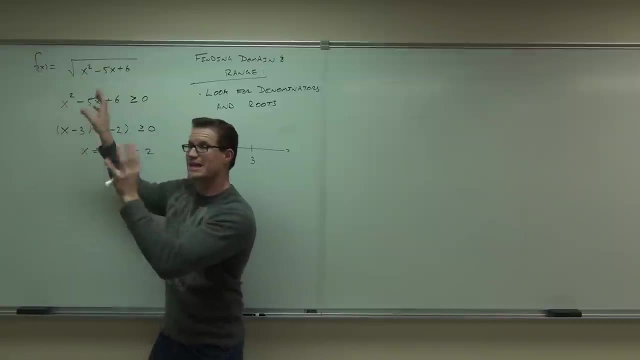 Negative, negative, negative comes back up at 3. Positive, positive, positive. That's what we're finding out right now. We want the sections that are positive, because we know we can only plug in positives or, sorry, get out positives for a square root. 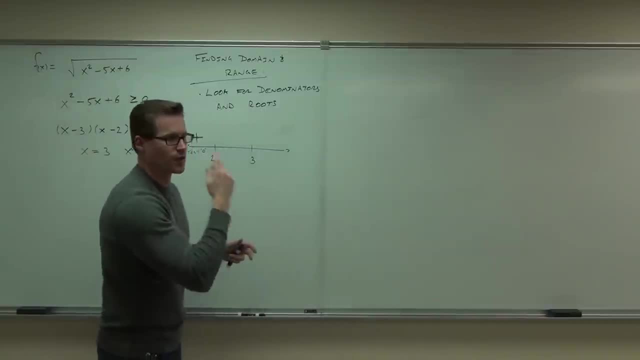 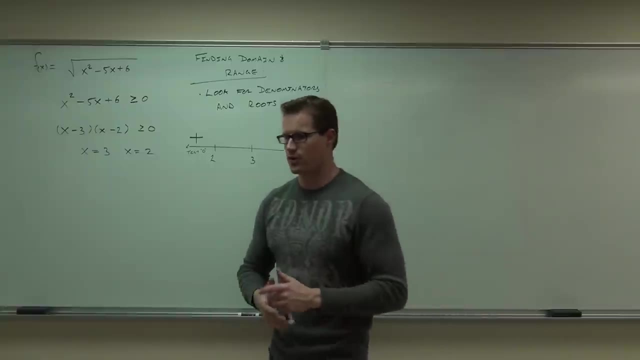 That's the idea. That's what a sign analysis test will do for you. How about a point that's greater than 3? What are you going to try? 5. 5 or 4.. Try 5 or 4.. 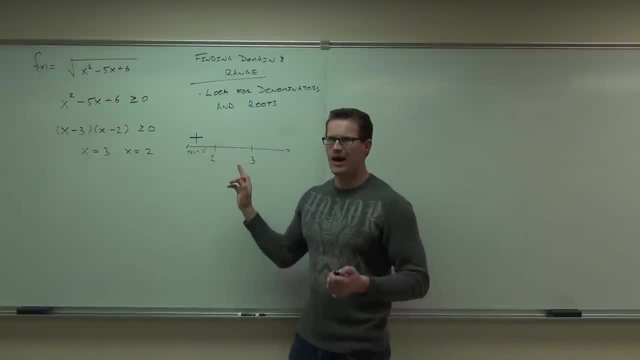 The only points you really can't try are 2 and 3.. Why, What are 2 and 3 going to give you? Yeah, that's not going to tell you anything, right? That's not positive or negative. Try 4 right now, on your own. 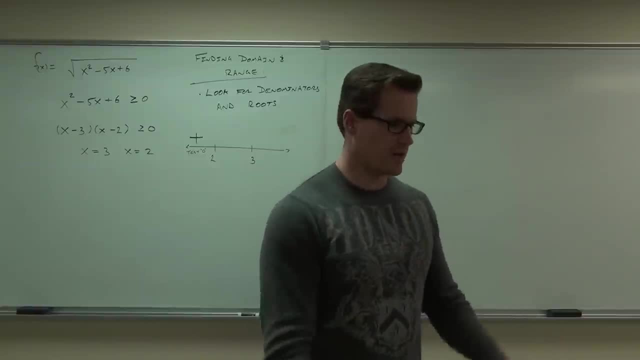 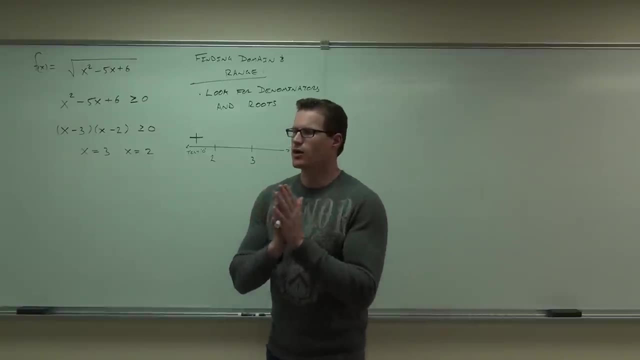 Plug that in and see what you get. You can do it in your head if you want. I don't really care about the actual value. All I'm really concerned about is whether you're getting a positive or negative. What did you get? 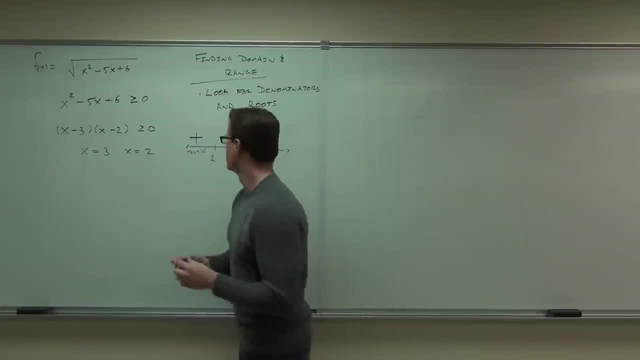 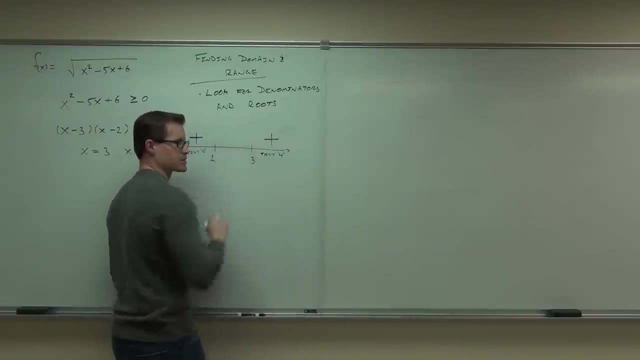 Positive. Yeah, and you really should. This is a quadratic, It should alternate. So you tested 4 and you got a plus. Can you give me a point between 2 and 3?? Because we've got to test a point in there too, just to make sure we have this right. 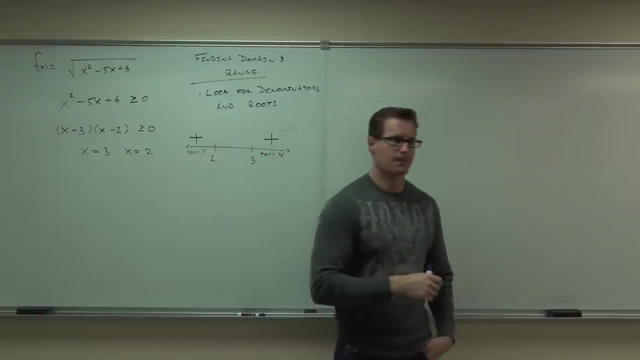 2 and 1 half. 2 and 1 half- Great, Try 2 and 1 half. Use your calculator if you want. That's your million dollar plan. You can do it. You can do it, You can do it. 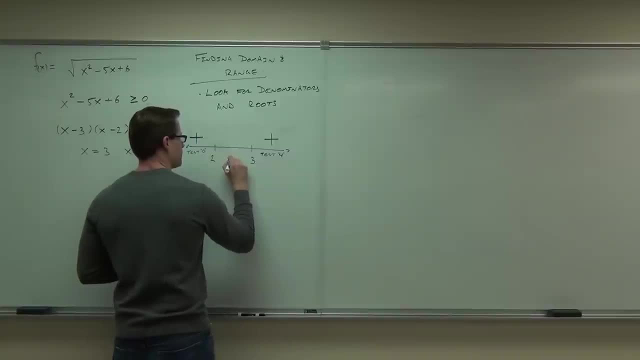 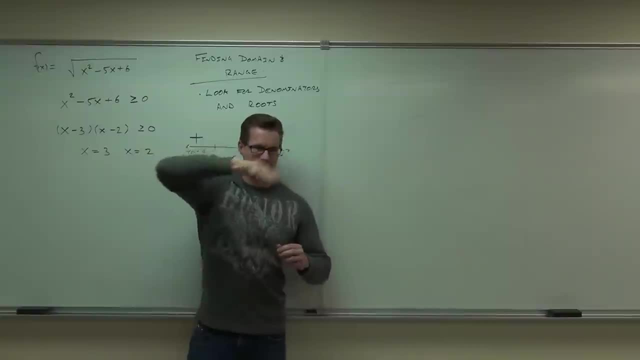 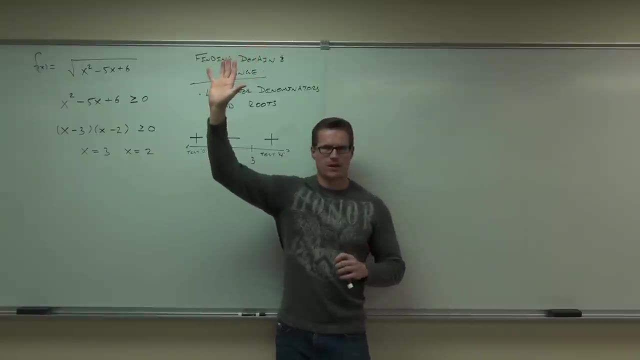 No, it's quadratic, right. It's positive here. It's positive here. It's got to be negative there if it crosses the X axis, So it's going to be a negative. How many people feel OK with what we've done so far? 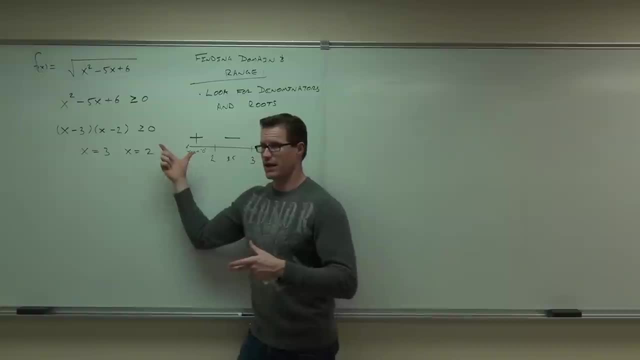 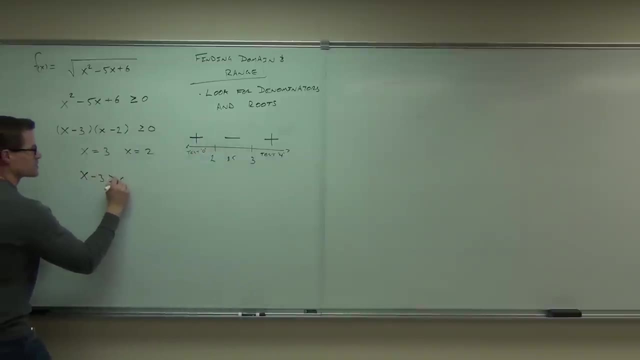 So can you just set this equal to 0 and this equal to 0 and get it right? The answer's no, No, you can't, Because if you did this watch, If you did, X minus 3 is greater than or equal to 0 and X minus 2 is greater than or equal. 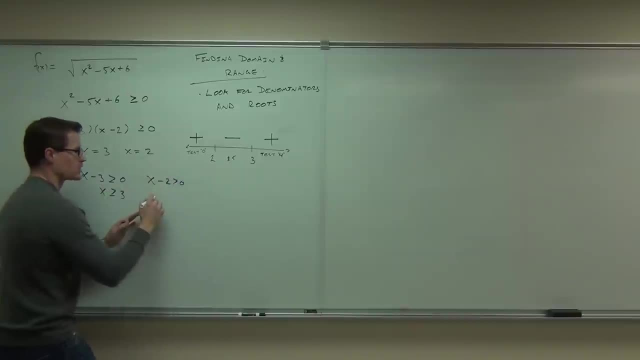 to 0.. X is greater than or equal to 3.. That's true, But you're going to get: X is greater than or, sorry, greater than or equal to 2.. That's wrong. It's not greater than or equal to 2.. 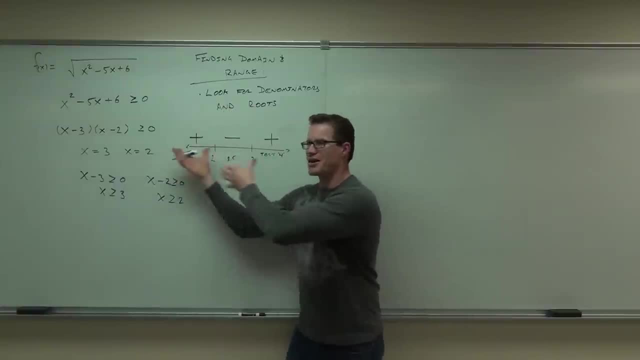 It's actually less than Do you see on our R and graph. this tells you the areas that work right. It says I can plug in any point over here and it's going to be okay because it's going to give me a positive and positives are okay inside of square root. 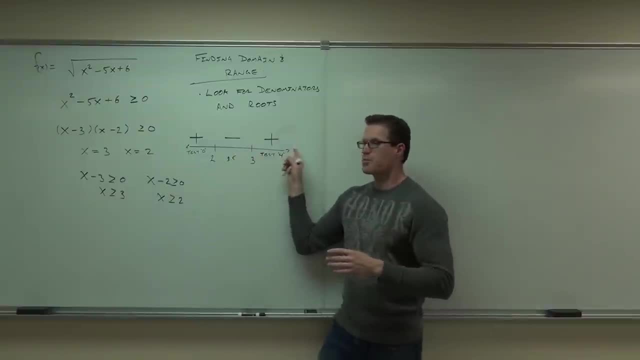 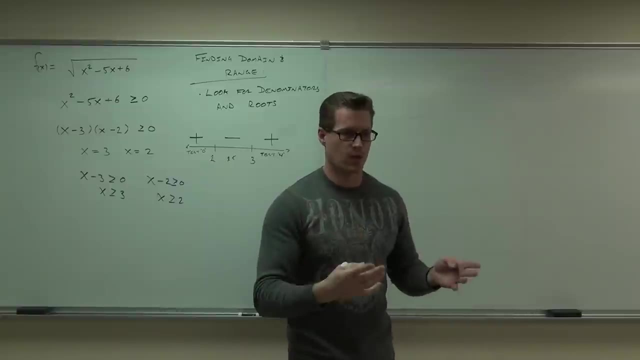 Some of you are zoning out. You can't zone out right now. This says every number I plug in over here. that's okay because it's a positive. The inside is going to give me a positive and square roots of positives are okay. 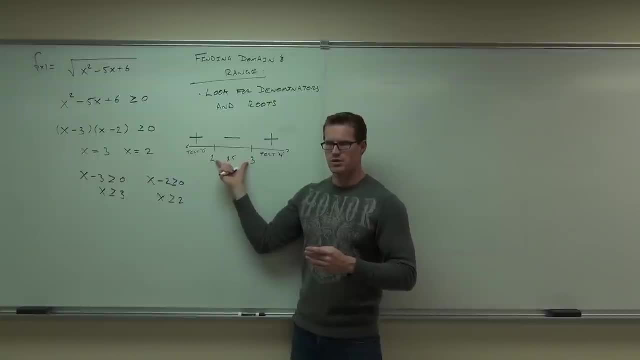 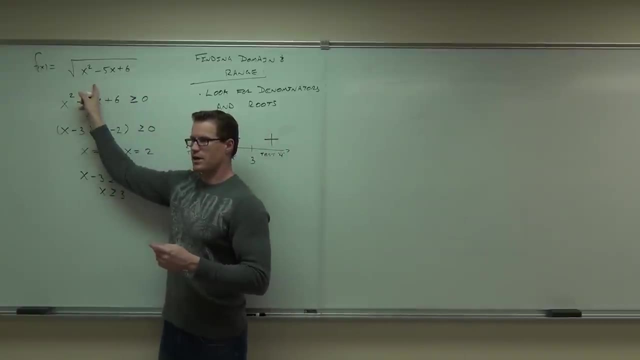 These numbers aren't so good. Why aren't these numbers good? When I plug them in, the inside part becomes negative. You follow: If we have a square root of a negative, well, that's not so good for real numbers. We can't have that defined. 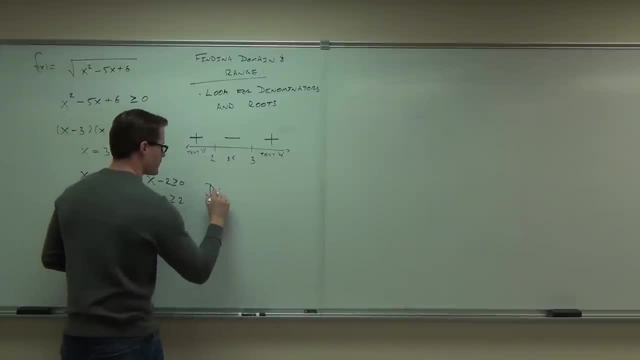 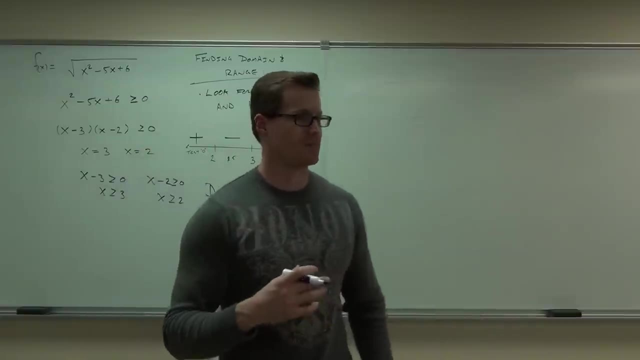 So what this does? it says your domain is all the intervals that actually work, and this is how you can do all of your roots. If you have a function with a root and you're asked to find domain, well, you do this. 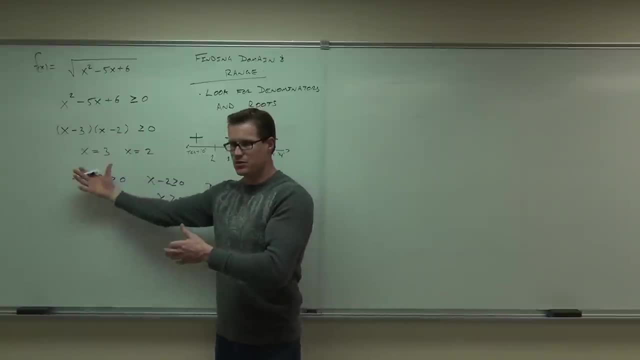 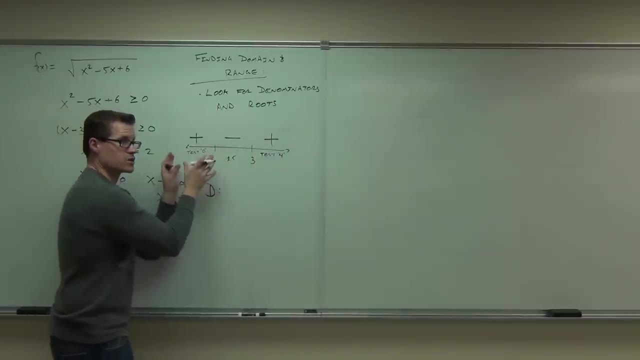 You set it greater than or equal to zero and you work it out. Sometimes you might have to do the quadratic with a basic sign analysis, but this tells you those intervals that actually do work. So take those ones that you know of and write them in interval notation. 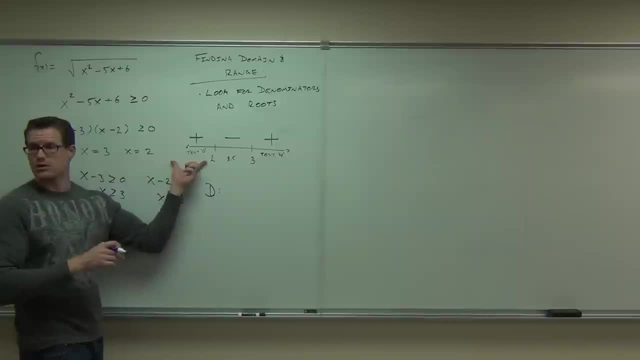 Can you tell me where this interval starts- Negative infinity, Good- and where's it end- Negative, So negative infinity all the way up to two. Now I know that's got to be a parenthesis, because infinity is always, always have parenthesis. 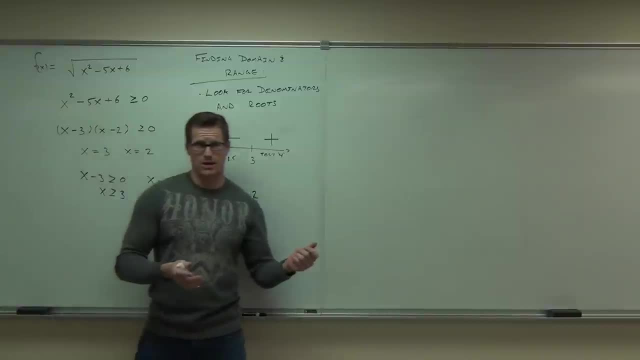 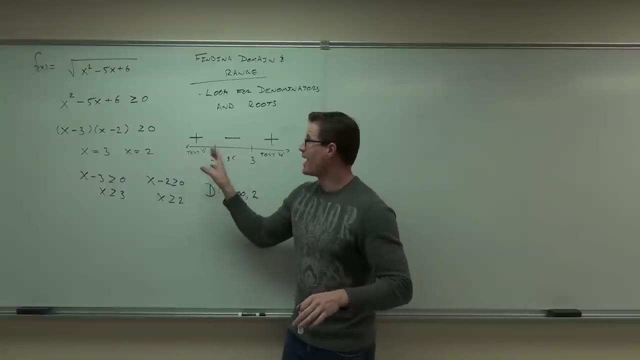 Is this a parenthesis or is this a bracket? Bracket, Why is it a bracket? Because it's equal to Good. It's equal to zero, because if I plugged in the two, it would give me out zero right, And that's okay for us. 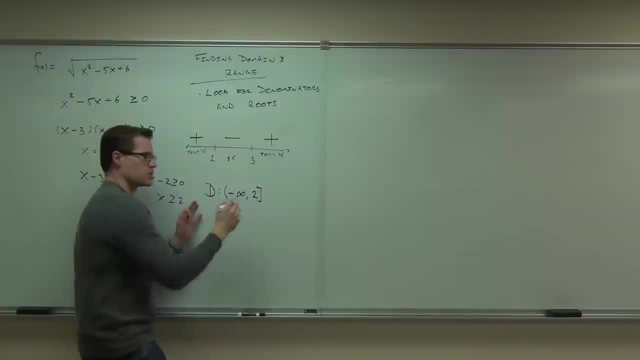 And then to show any other interval. what you do is you put this U standing for a union. I know the three's going to work all the way up to positive infinity. That's a different way and your book likes to do this. a different way to define your domain. 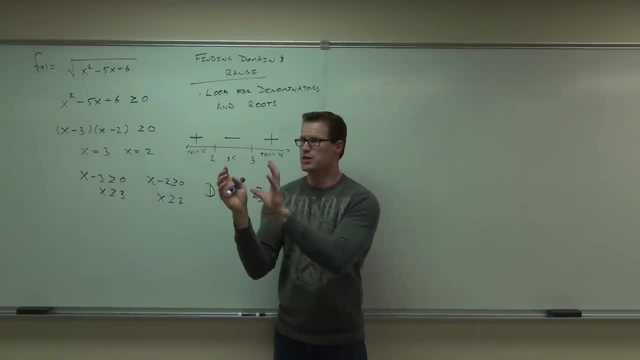 Instead of all real numbers, except you use the intervals that you can actually show. So on your book, sometimes, instead of saying all real numbers, like I showed you last time, they say things like negative infinity to positive infinity. Have you seen that yet? 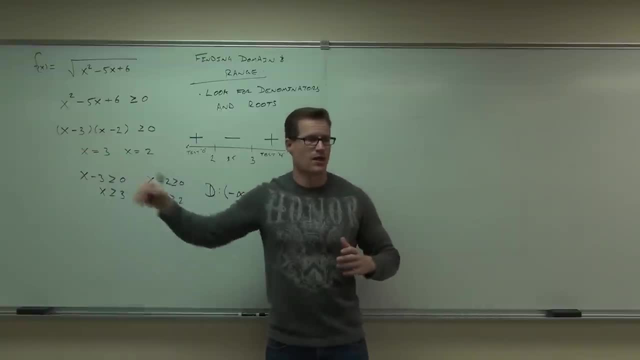 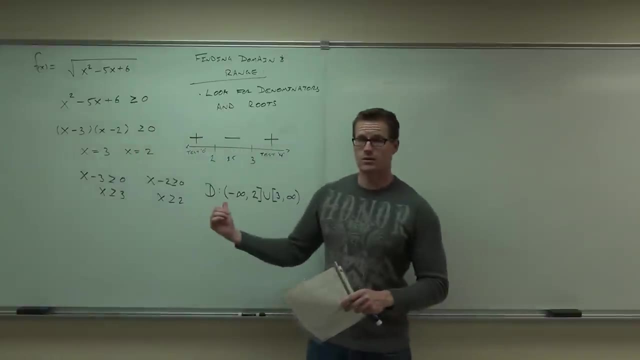 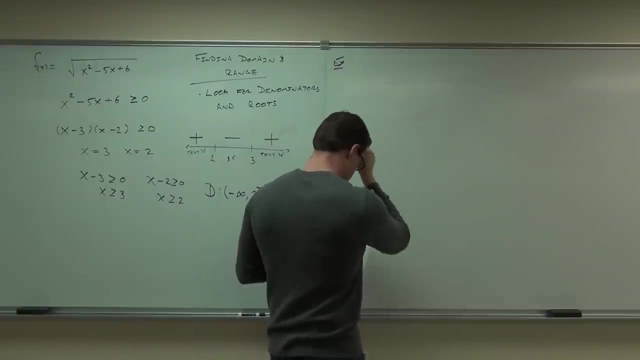 Have you read through your book? That just means everything, everything from the far left to the far right. You guys ready to try another one? Did this make sense to you? Yeah, Okay, cool, Okay, let's go ahead and try to find a natural domain for this. 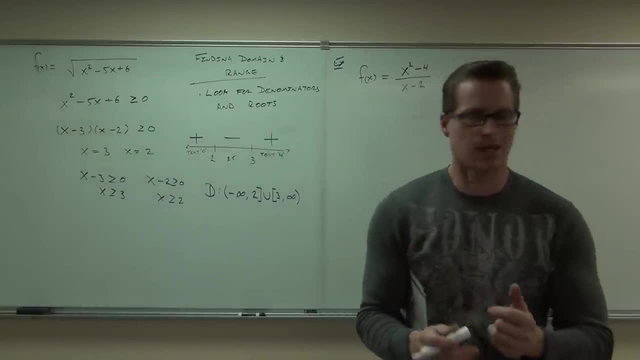 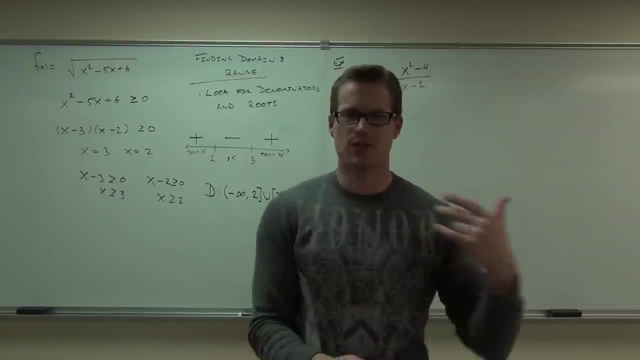 What you ask yourself for domain is: am I going to have any issues Or, basically, do I have one of these situations? Do I have denominators that could possibly equal zero, Or do I have any roots? Do we have any roots here? 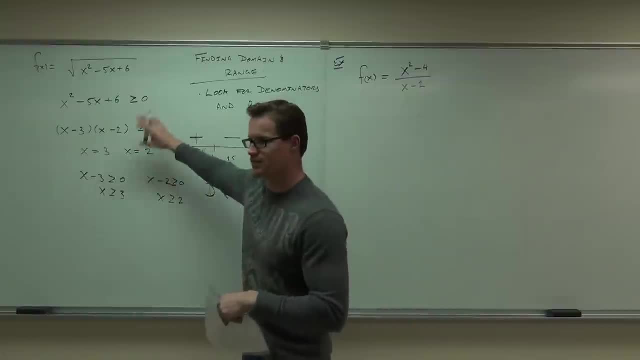 No, we don't have any roots. That's kind of nice. We don't have to do this whole mess of crap. right, We do have. what, though? What's going to be a problem for us? Denominator- We've got a denominator. 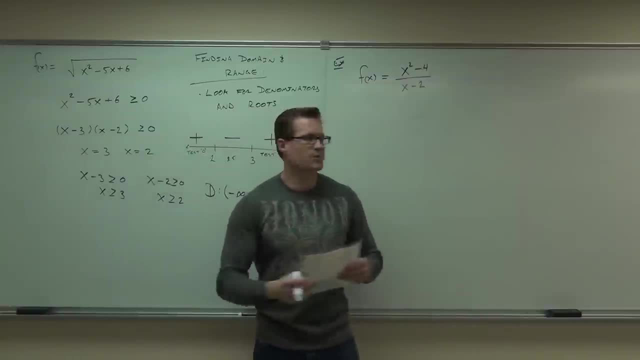 How we deal with denominators. domain issues with denominators- is we set them equal to? if you want to set equal or not equal to, We know that the x minus 2 can't equal zero. If we do, we're going to get something that's undefined. 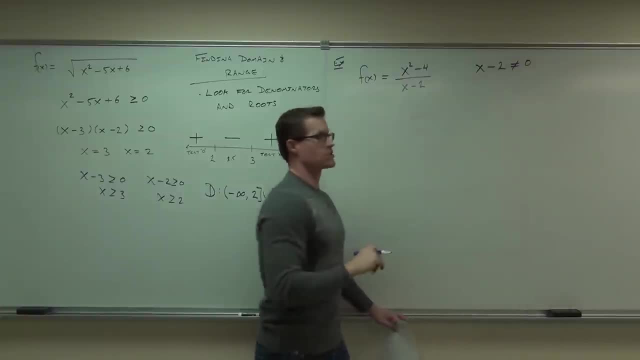 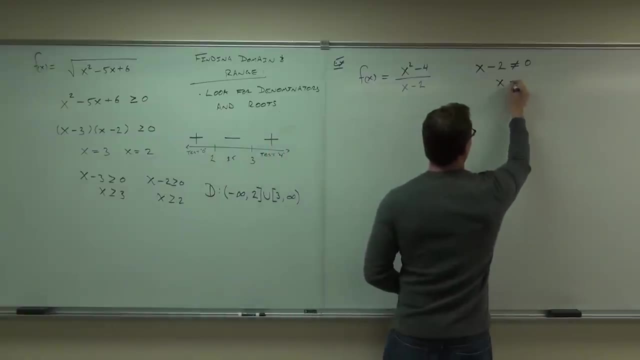 So right here, the way it is, I know that x minus 2 can't equal zero, which means x can't equal zero, Right? So x can't equal which number? Two, Two, Yeah, that's the problem. So our domain would be all real numbers except x cannot equal 2.. 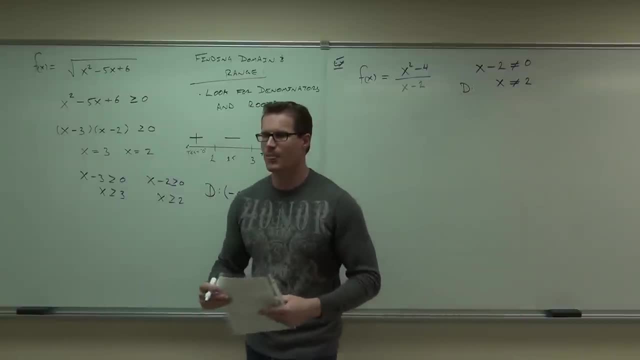 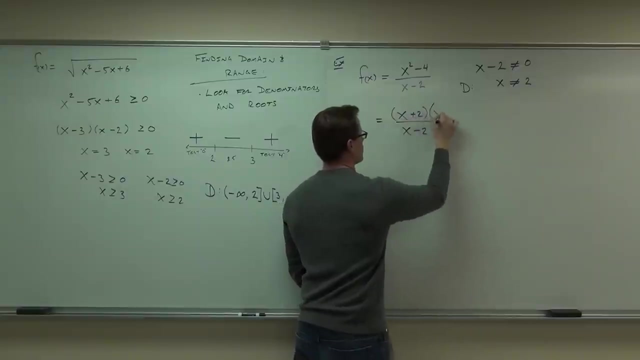 You'd have all real numbers, but x can't equal 2.. That's the deal. Now I want to show you something. This is going to come back later in our class when we deal with continuity. Check this out, True. 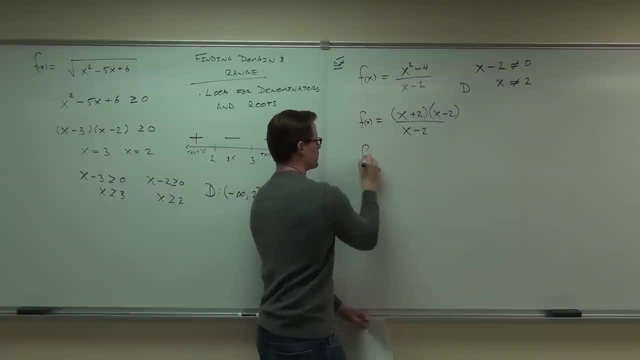 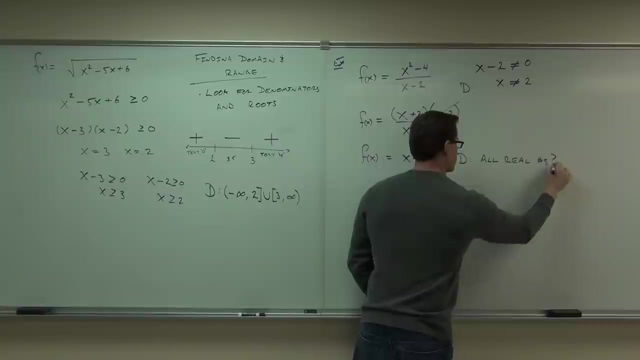 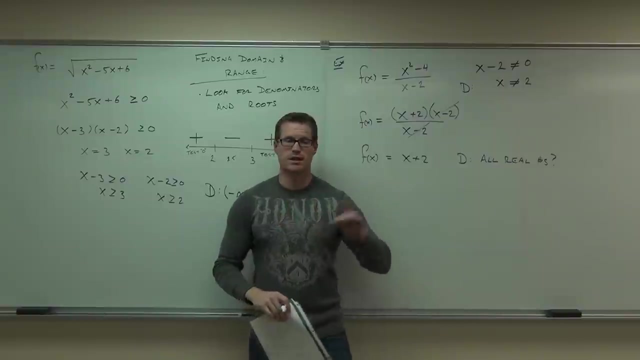 Yeah, mm-hmm. Difference of squares- True, Mm-hmm. Yes, you can do that. They're factors, True. Can you plug anything into that? If there's no roots and there's no denominators, then yes, you can. 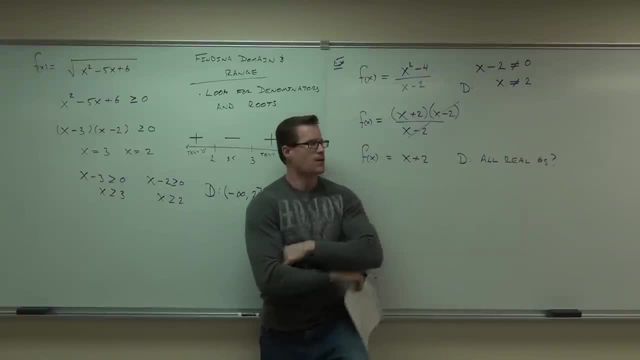 Can you plug anything into that? But wait a second. This came from a function that we knew. We knew we had a problem, didn't it? We knew we could not plug in 2 there. So what's it mean? that I can cancel out the problem? 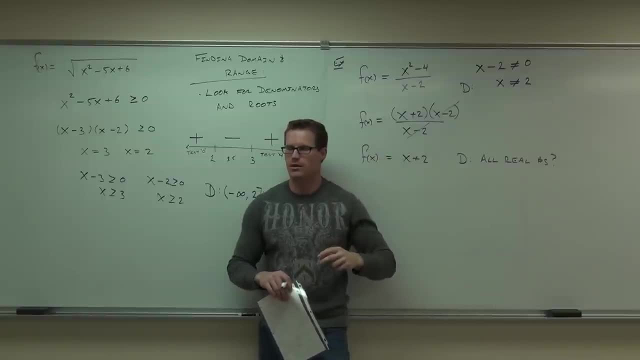 Can you actually cancel out a domain problem? Well, that doesn't seem right, And the answer is no, you can't. So, even if you can listen carefully, even if you can simplify your function, which you can here, you still have to keep the original domain. 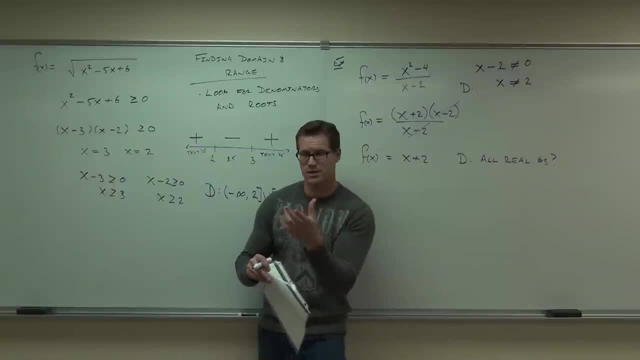 Otherwise you'd be eliminating some of those problems that you know exist. Did you follow that? Say it one more time: If you can simplify your function, do it, But you have to keep the original domain, because by manipulating your function on this particular case, you've actually eliminated one. 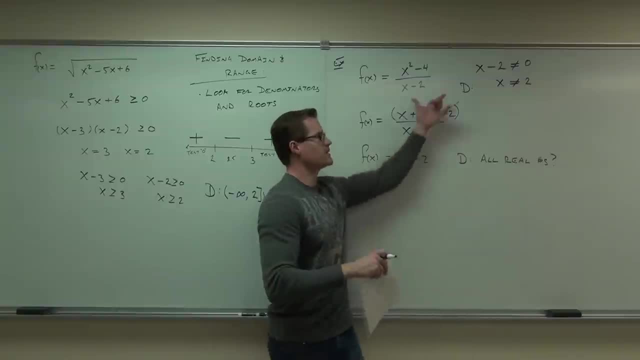 of your domain problems, which that's not right. You have to keep that original domain. This says you can't plug in 2, right, Just by manipulating it. you can't all day and say, hey, now I can, Harry Potter, here's my math wand. 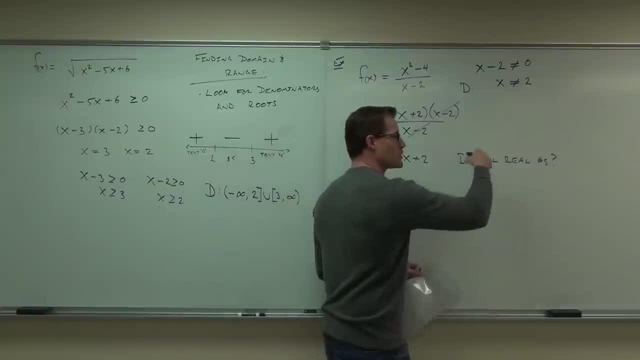 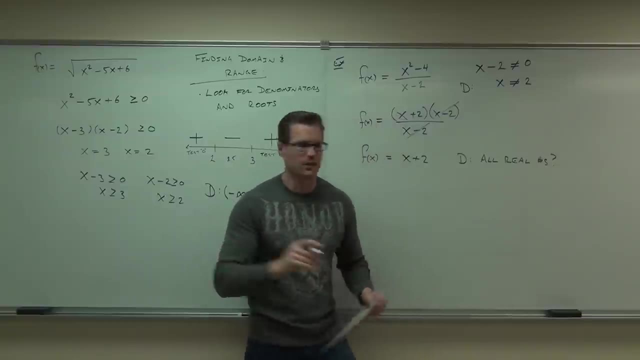 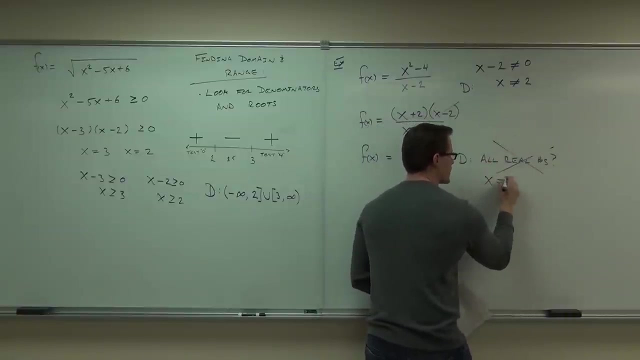 Done. You can't do that. So if you're going to do this simplification, just make a little note that with simplification you've got to keep your original domain, So our domain stays the same. X still cannot equal 2.. 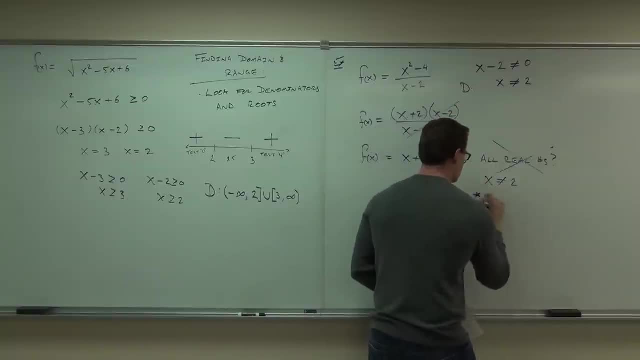 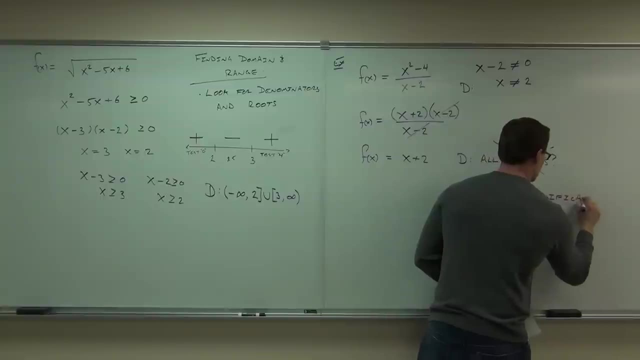 So for simplification, keep your original domain. With simplification, keep the original domain And it's your old domain. So with this you're keeping your original domain. It's not going to matter how many problems you have to do. 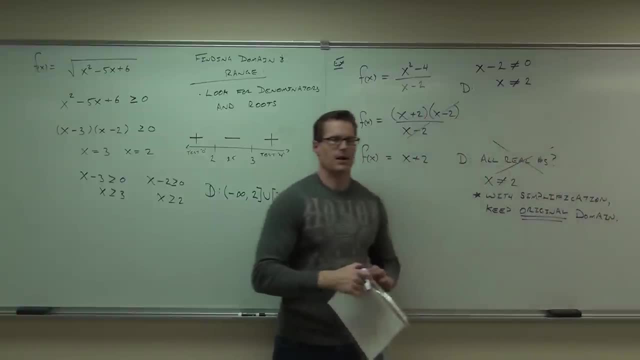 every problem you've got to specifically solve on this one, It's with simplification. you're keeping your original domain. I'll say it to you another way, And this is how I always like to think of it: You can't ever make your domain better by combining or simplifying functions. 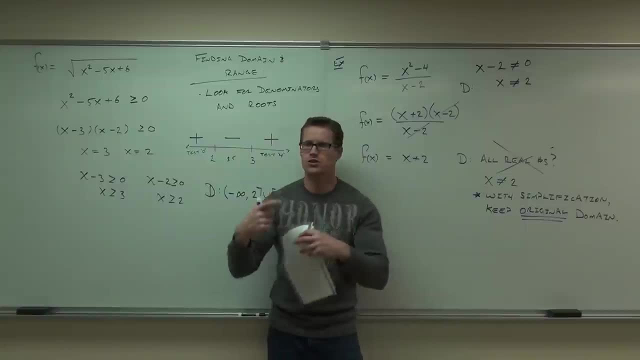 You can't ever eliminate problems. All you can do is make more problems. So how your functions start, those are the problems. you're dealt As a hand. you're dealt okay If you add or subtract functions together and compose them. 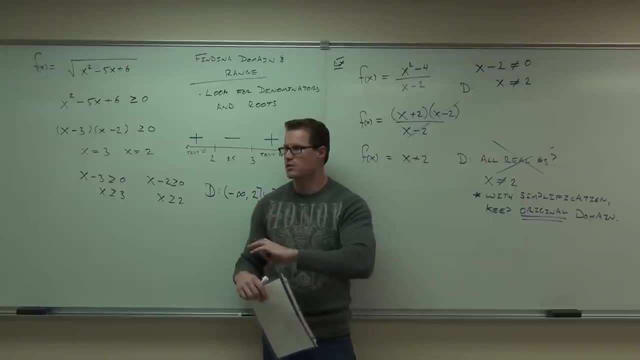 the only thing you can do is create more problems about them And that's all. you need No problem problems. You can't eliminate problems. What you start with is what you start with. So if you have a domain right here with this function, that's the domain, unless you mess. 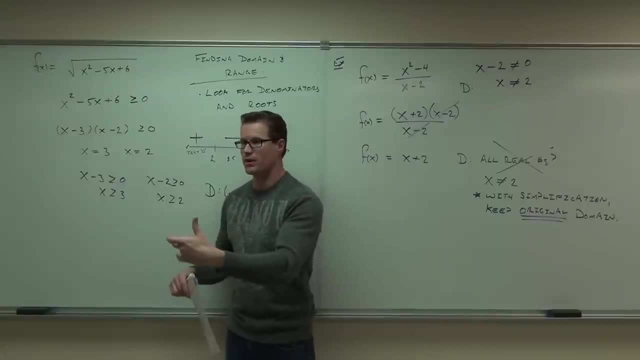 it up even more. You can't ever make it better by allowing more points. Does that make sense to you Now? would you like to see what this actually is? Do you want to see what this does? The answer's always yeah, Okay, good, I hope so. Can you graph this? Can you graph? 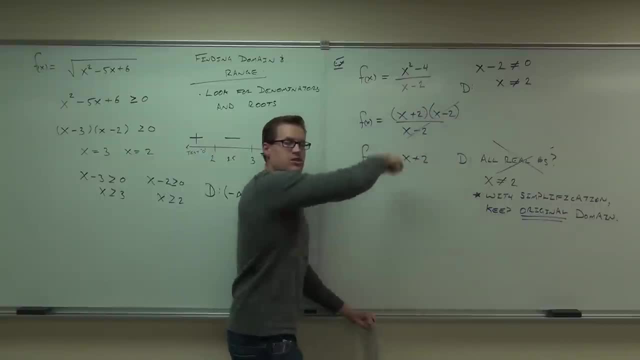 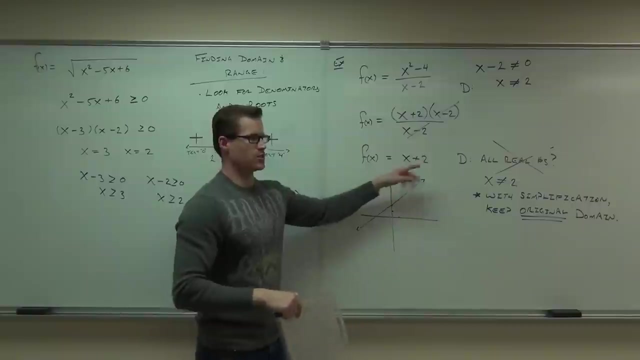 this in your head? Actually, the answer's: yeah, These are the same graph. Check it out. This graph right here is: well, that's a y-intercept of two. What's the slope? That means you go up one over one. This is x plus two. This is the graph of x plus two, with no domain. 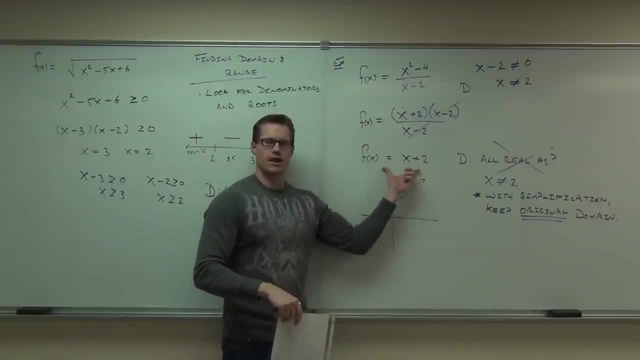 restrictions. It would say: if I was just given this function and I didn't know about this. that's how I graph it Now, what this function is, what this one is with your domain issue. it says that you shouldn't be able to plug in the 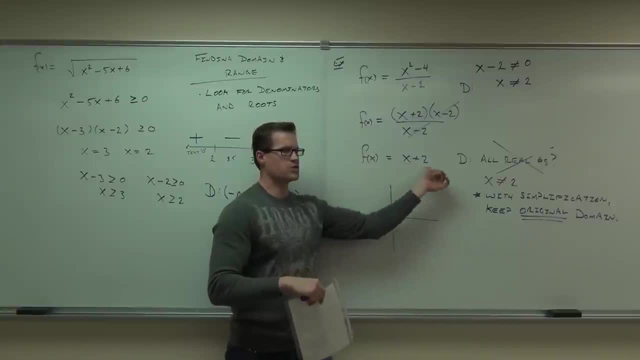 two. right, If you were able to plug in two, how much would you get out of it? Plug in two, How much do you get out of it? Okay, So what happens? what this says is that when I plug in two, I should be getting out four. However, I know for a fact from my original. 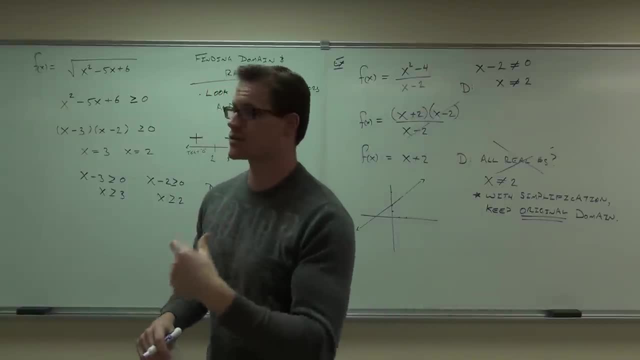 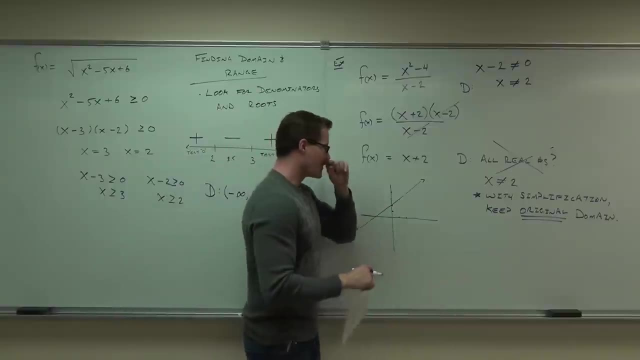 function. I can't plug in two, because that would create an understatement. So now I know what this doesn't mean. So here's what it says: If you plug in two, you can't get out four, which means you have a hole. What that is called in the future is what: 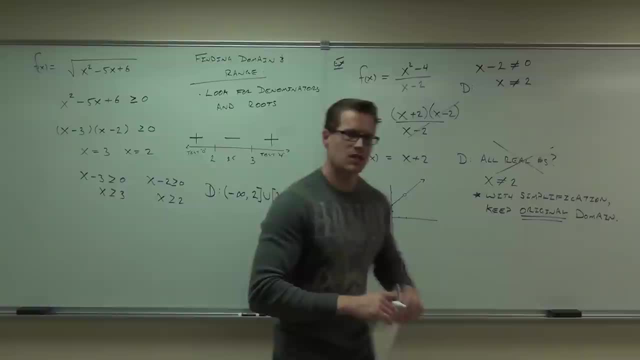 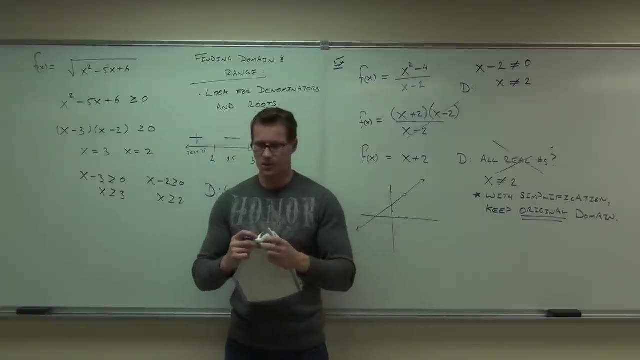 you call a removable discontinuity. It's not continuous, because you have to pick your pencil off the paper, so it's not continuous. However, it's a removable discontinuity, which is defined as if you allow one single point to fill that hole, if you can fill the hole. 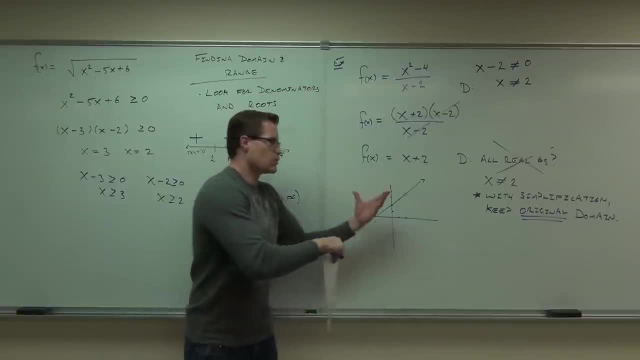 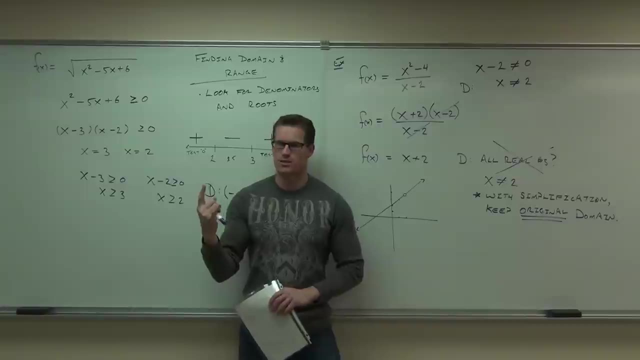 with one single point. you can get out four. Whatever, You don't have to paint, That's up to you point it's removable. so that's that's what we consider that as. so what are situations in your denominator? there are two categories. I'll say them verbally. 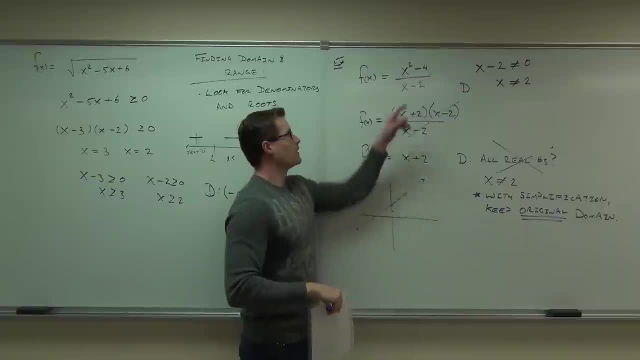 but I'll go over more in depth later- if you can cancel out- you know you love to use those words cancel out, it's really not a mathy word. but if you can cancel out your domain problem it's a whole. you with me, it's a whole. if you can't cancel. 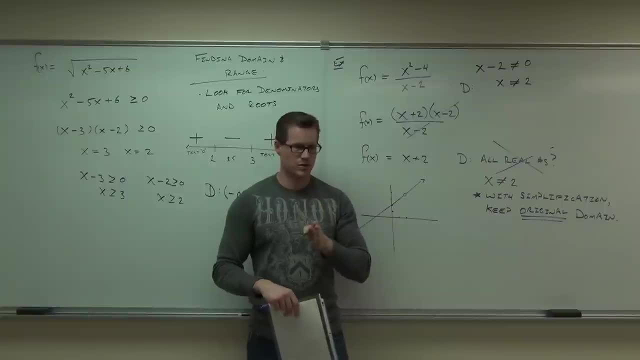 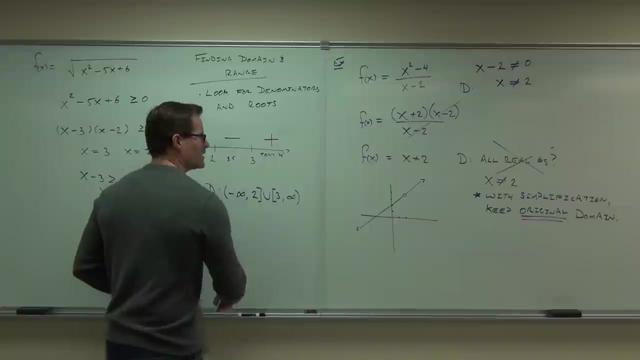 out the domain problem. it's an asymptote. those are your two categories that make it kind of simple, doesn't it? if you can cancel out, it's a whole, if you can't cancel out, it's an asymptote. that's it. let me write that down for you. yes, let me give you another example before you. 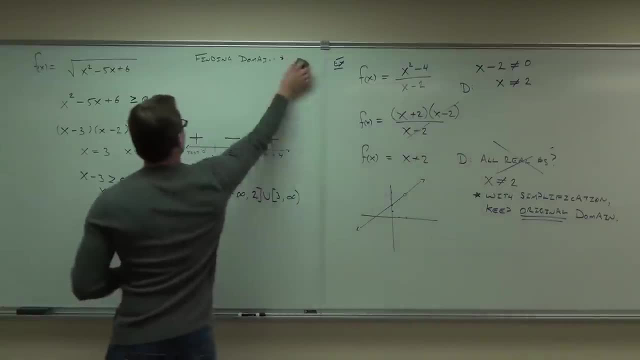 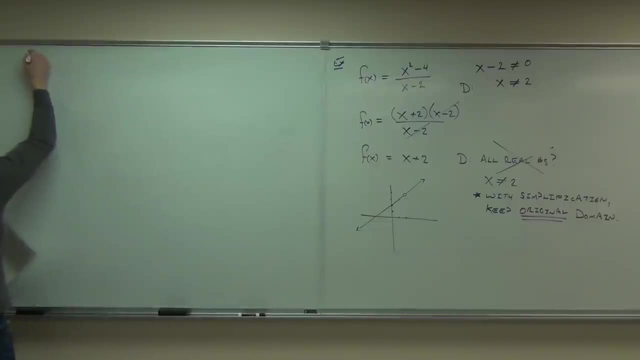 you write that down, I'll give you the same one over here and I'll give you this one. what can't x equal here? yeah, that's pretty common. gave you a very easy one, just so you can see it. of course, x can't equal four. here's the difference. can you manipulate this way? 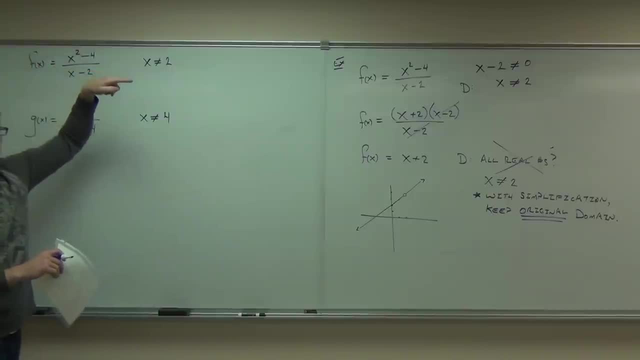 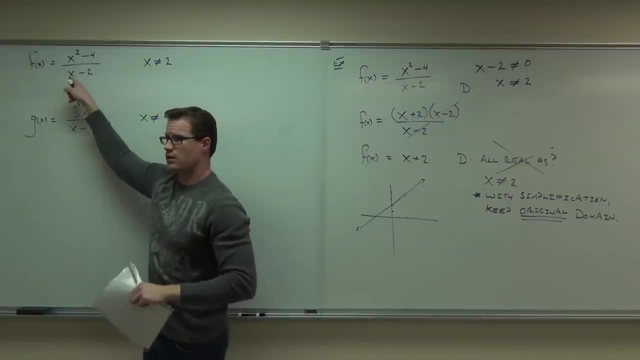 to manipulate this to get rid of the x minus two. if you cross it out, that means you have a zero over zero. if you were to plug in the two, check it out, you're gonna get zero over zero. right, you see that when that happens, that means you. 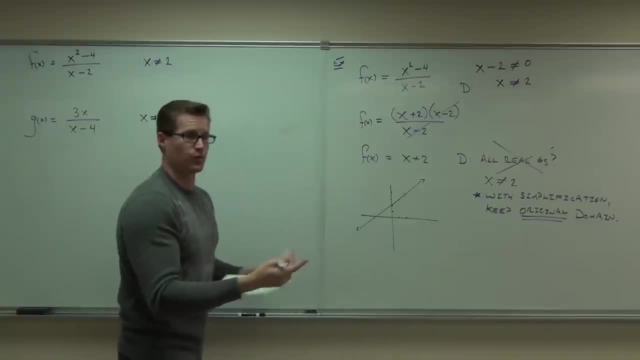 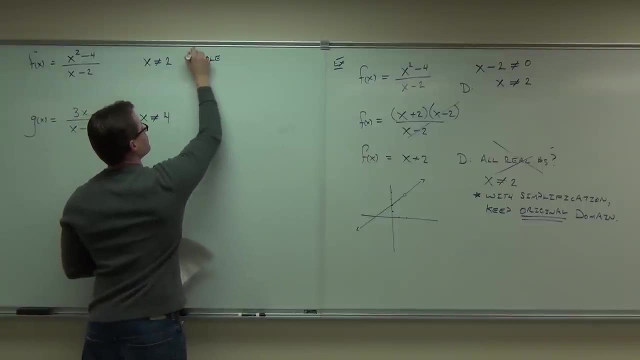 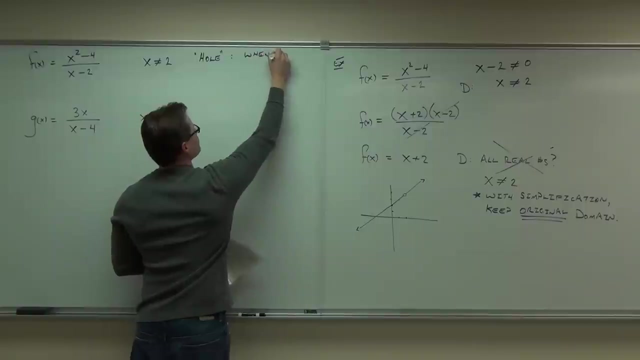 can cancel it out, you can simplify it out of the problem. that's a whole for you. so, when you get zero over zero, this is a whole, like that, when you can remove the discontinuity, aka when you can cancel it out of your problem. if it's a whole, yes, okay. so yes, that is a test instead of going through. 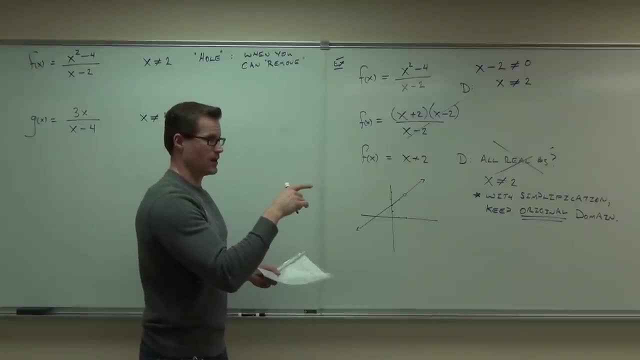 canceling? sure, that's it. I didn't. whatever number you're not supposed to use and if it comes to zero with polynomials, absolutely okay, radicals, it'd be very hard to factor that out. maybe I don't know how to do some work on that, I'll. 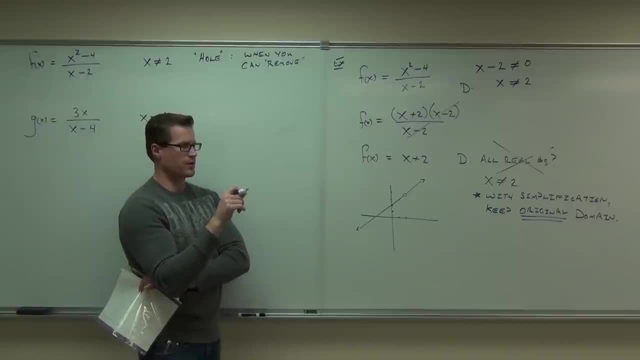 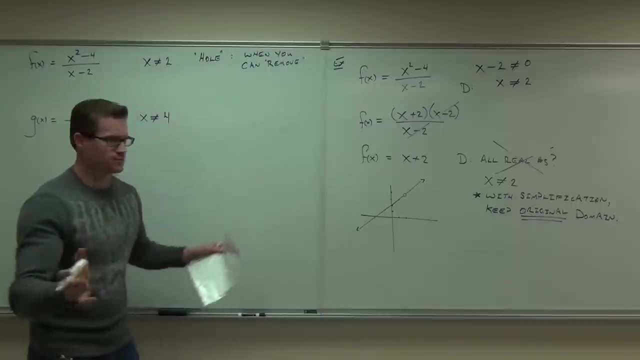 get back to you on that one with polynomials. absolutely, though, because if you plug in a number and it is a zero, that's automatically a root, means you can factor X minus that number out of your equation. that's math, that's, that's proven. so when you can remove the discontinuity, 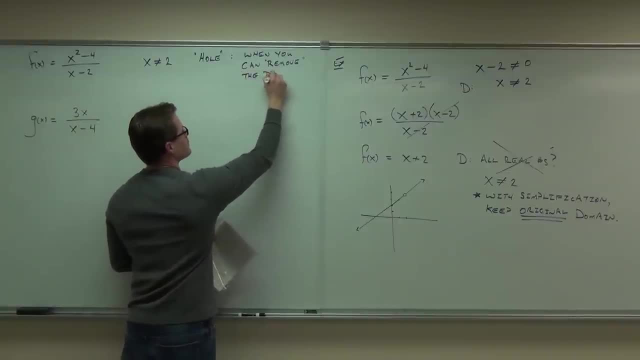 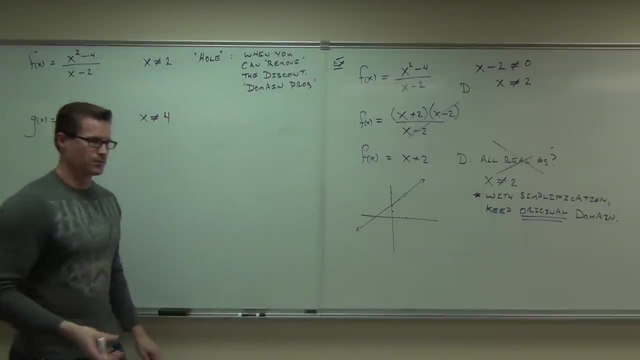 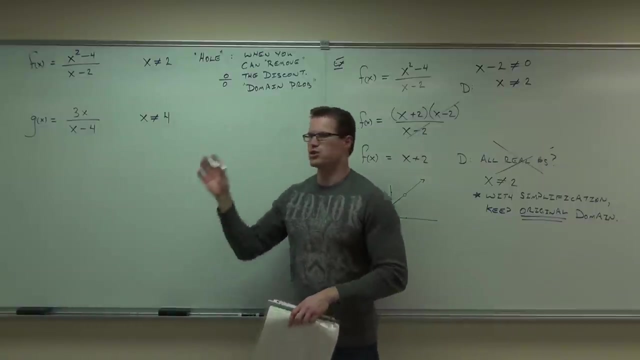 leaving. you talked about continuity before, but when you can move the domain, this means domain problem, that's a whole. that's a whole zero over zero for polynomials in general. when you can- just when you can- simplify it out of your problem and it's no longer a problem. 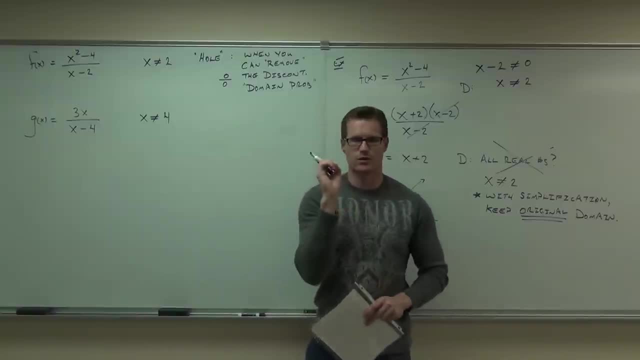 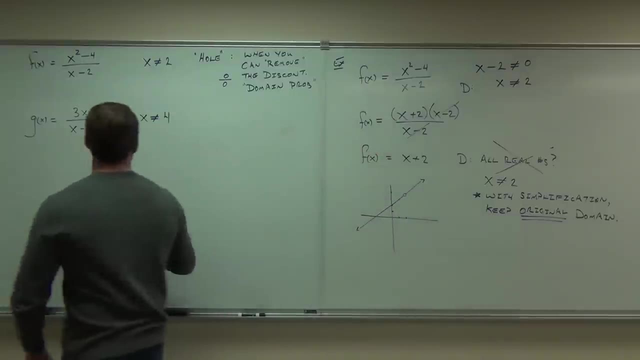 for your domain. that's what we call a whole. it's just a little spot where you don't have a point. now, if you're okay with the idea of a whole, okay now. now the other. the other thing we gotta consider is: well, what happens here? can you simplify the X minus 4 out of your 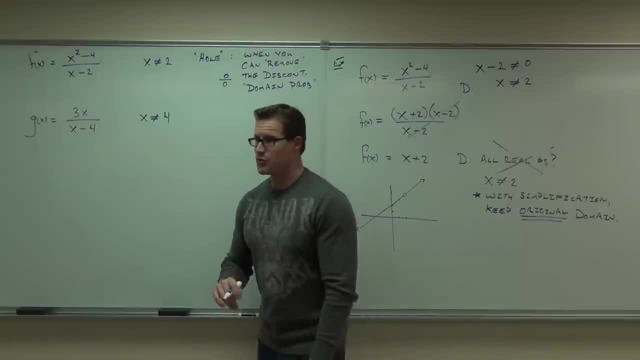 problem here. is there any way to factor it and simplify it? if you plug in the 4, do you get 0 over 0? no, no, you get. well, you get 12 over 0, and that's, that's an issue, right? that means that you're not gonna be able to factor that in any way. 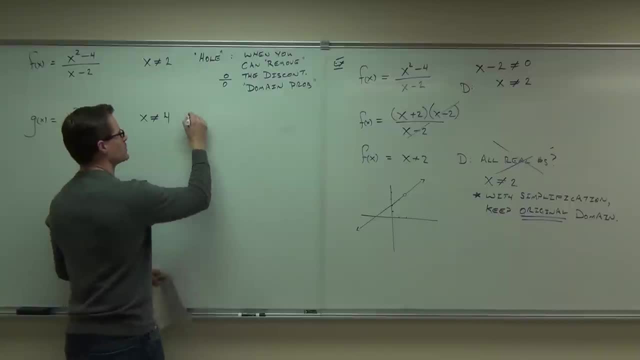 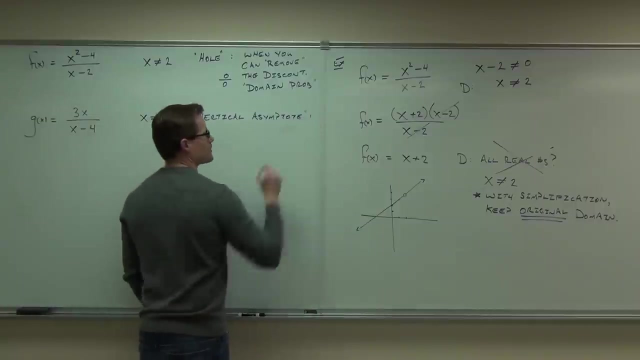 to be able to simplify that. what this is is a vertical asymptote. vertical asymptote. this happens when you have a number over 0, typically, and it means you can't get rid of the domain issue. I forgot it. those are gonna come much later. I'll show you an easy way to do. 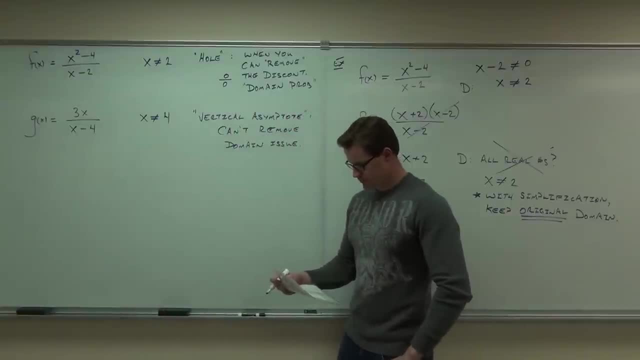 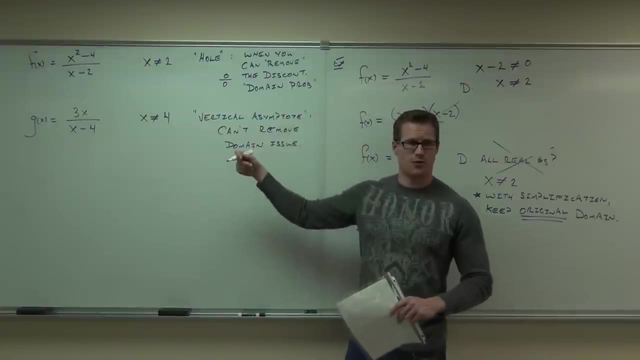 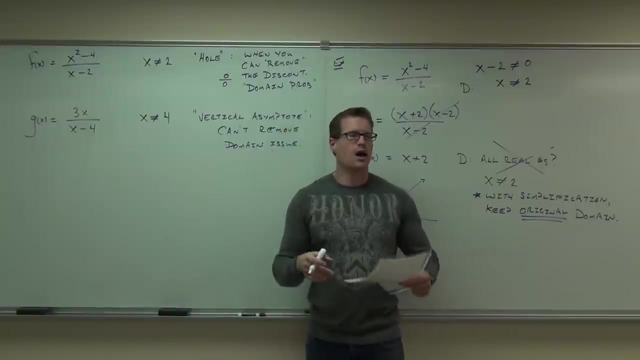 this. we're gonna talk about something called limits. does this outline better for you? so you're gonna have two classifications of domain issues. if you can simplify them out, they're called holes. if you can't, they're gonna be vertical asymptotes. we're gonna find out a little bit later on how to determine what happens with 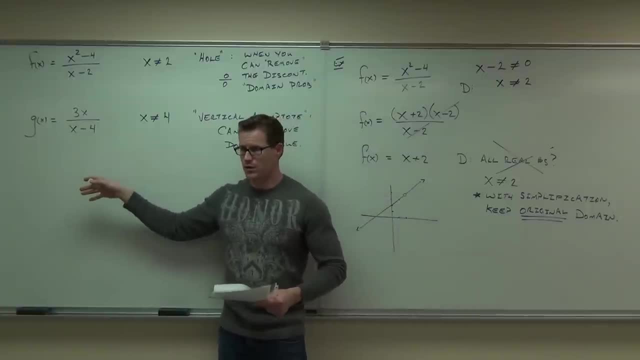 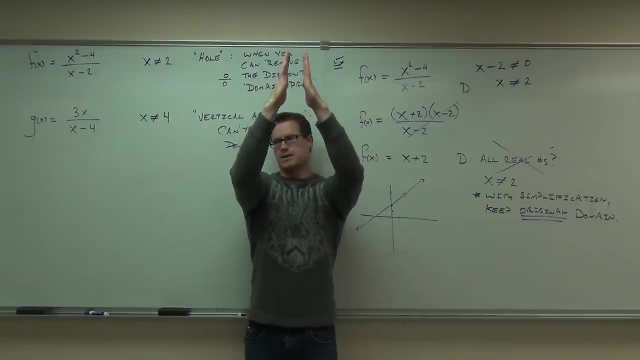 those. we'll do it another sign analysis test with 4 on our number line. we'll figure out that these asymptotes can either go upwards or downwards, or a combination of those two things. so they'll either be like this, going towards 4, in this case, or like this, going towards 4, or like this takes a lot of. 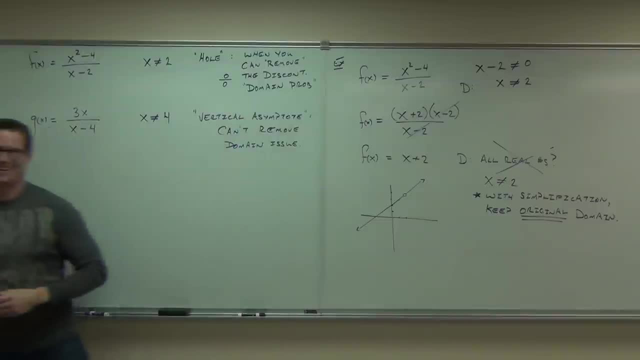 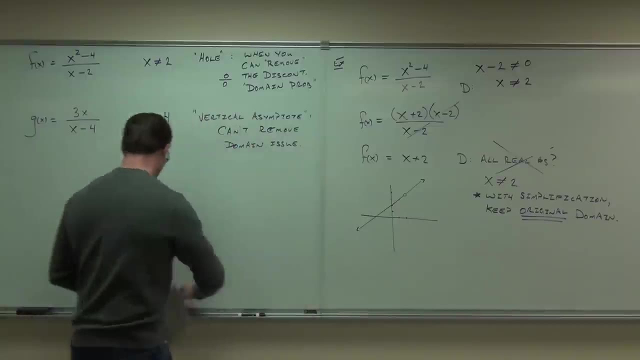 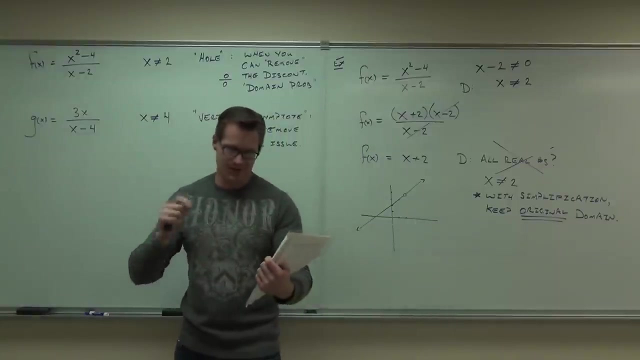 practice. do that, by the way, kind of like rubbing your belly and patting your head. it's hard to do. can you do that? let's see no cameras not on you guys out. okay, now let's do one more example. we'll go on. two more examples are going to a word problem: kind of figure out how we 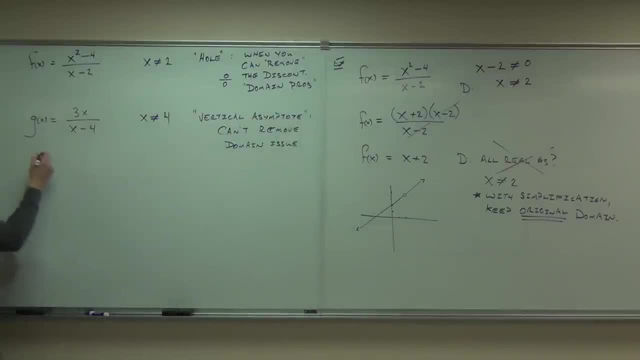 can talk about domain with word problems and then we'll continue on to some trick stuff. so I want us to find the domain and the range of this problem. find domain and range of that problem. hey, first thing, are we gonna potentially have any problems in this? any problem? what one asking you is basically are: 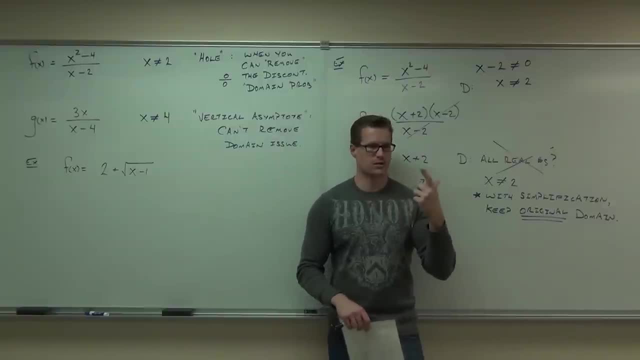 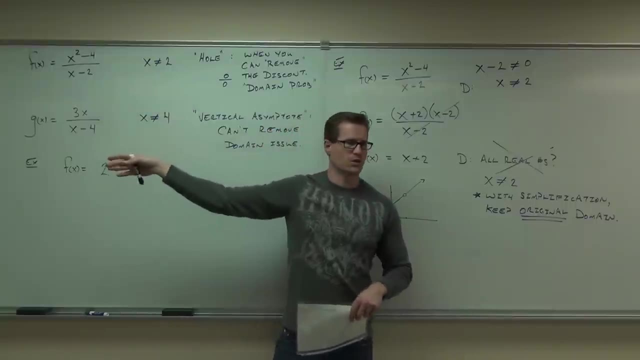 there denominators or are there roots? are there any of those two things? but there's definitely roots, so we potentially could have some problems. we don't have any denominators, so we're not dealing with holes and vertical asymptotes. what we're dealing with is area or range of an asymptote. there are two ways to do this. there are two ways to do this. one is the most common method to find the 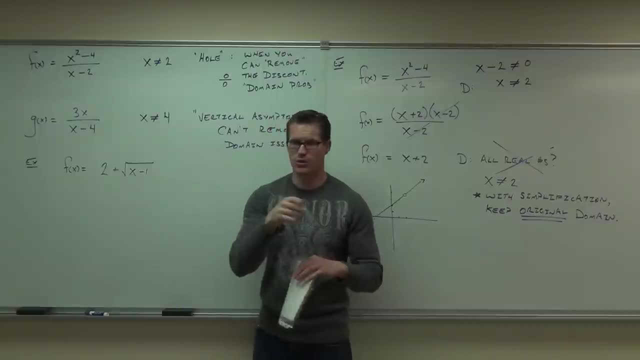 of our graph that we can't even plug in a number because it's undefined in the real number system. Do you see the difference there? It's not even defined in those areas. Now, what do you know about the roots? How do we go ahead and find those areas? 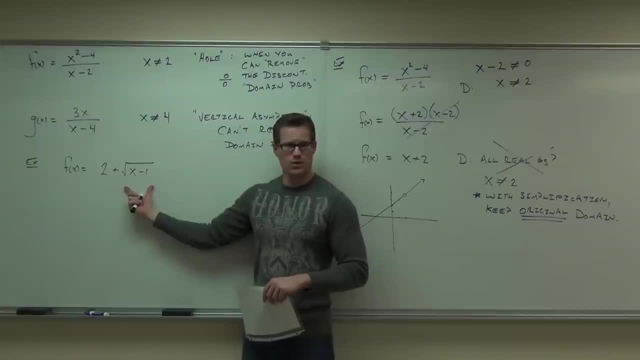 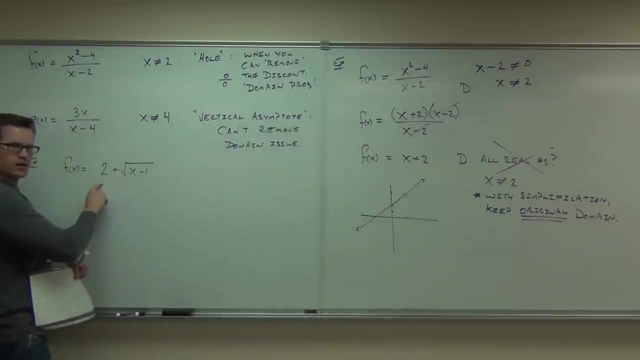 Set them. they could be equal to zero, right inside, or less than zero, or greater than zero, Greater than zero. They have to be greater than zero. So what we know is that the two is this: okay, That didn't do anything. 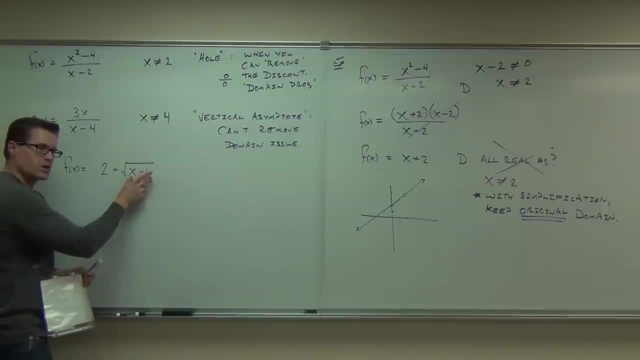 The only problem we potentially could have is inside of this root, because we know if this thing is negative, that's not so good. You okay with that, Not so good. So we know that, whatever we do, whenever we plug in this has to be greater than or equal to zero. 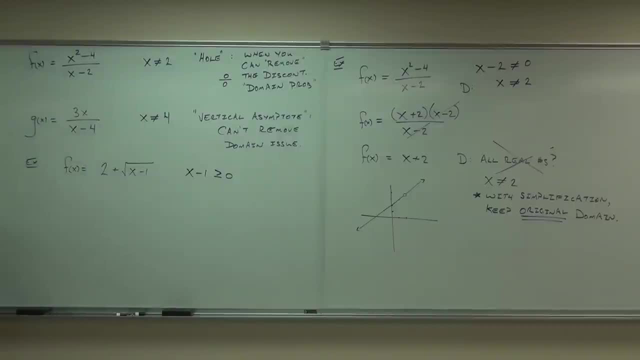 That's a must, Otherwise we come into a serious problem where we're not in the real number system anymore. Can you solve that? How would you solve that, folks? What would you do? Add what, Add one, Add one. This isn't even one of those quadratic inequalities. 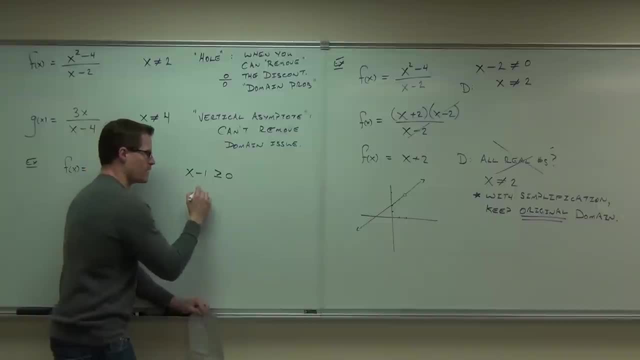 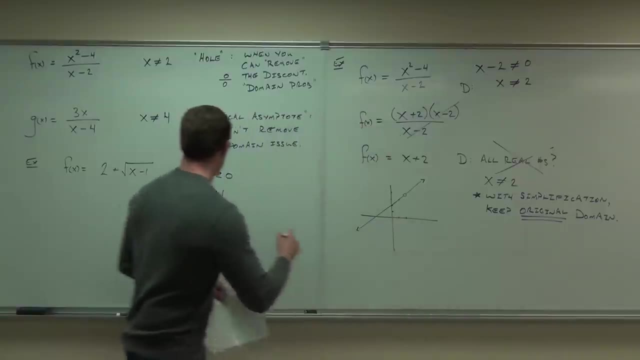 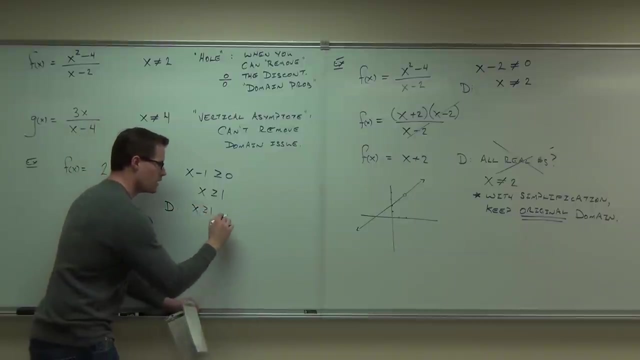 This is actually a pretty straightforward one. This says you're gonna be okay provided X is bigger than or equal to one. So for our domain you can say one of two ways. You can say: okay, the domain is X is bigger than or equal to one. 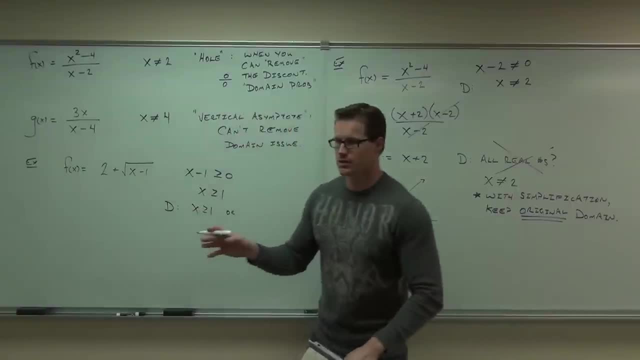 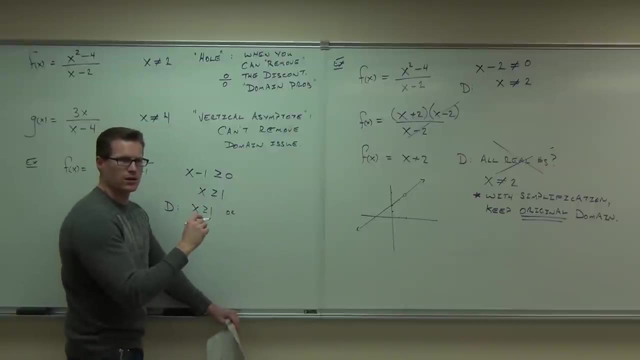 Or if you want to use the interval notation, which again, you're gonna see a lot of answers like that in the back of the book. if you use interval notation, let's say you're going from where to where, Negative infinity to 1, now that would be x would be less than or equal to 1.. 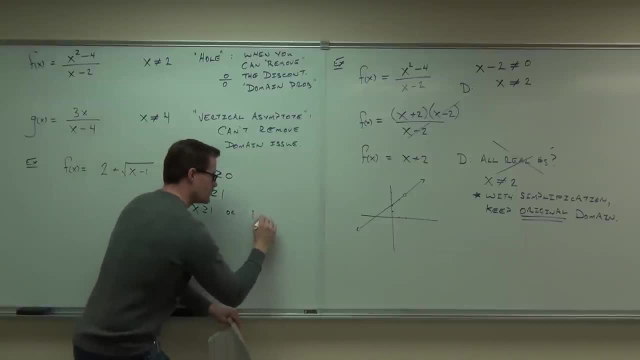 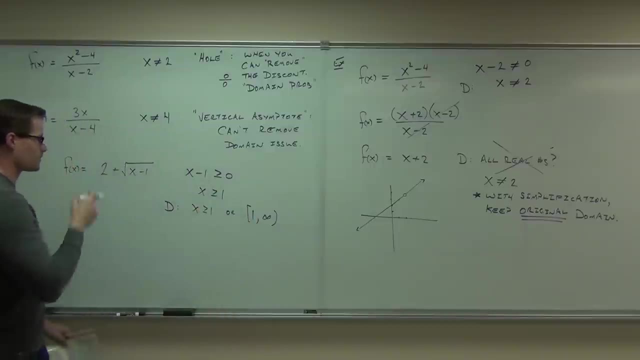 We want it to be bigger than 1 to infinity. sure, I know parenthesis here, Parenthesis. or bracket here, Bracket here. Sure, Yeah, very good. Do you have any preference on which way to write the answer? I don't care. 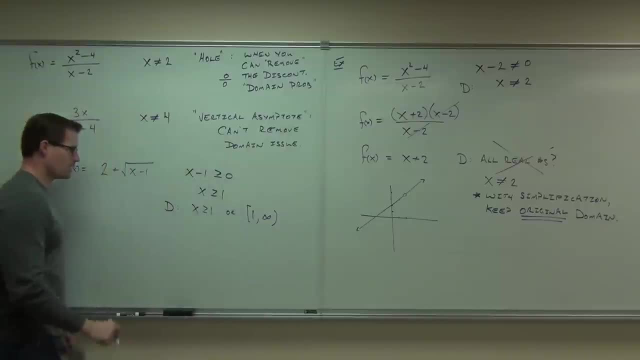 You're going to see this a lot right now, so you may as well do that. When could you not have it equal to 0 inside the square root? I'm going to change the problem just slightly so you see it. If I erase that and put it over 1 or 4, any number on the top. 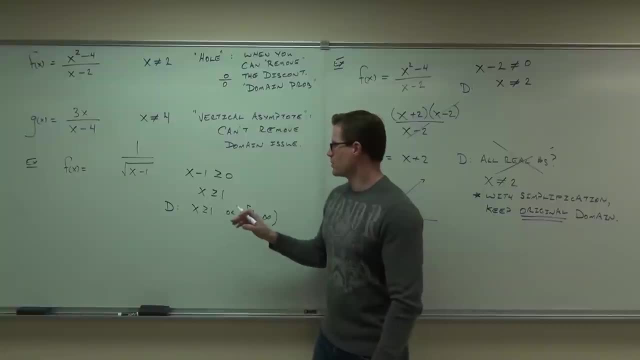 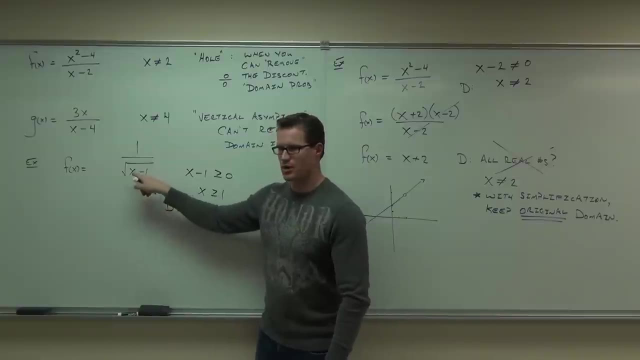 this would be the only case for your roots, when you wouldn't have this equal to 0. You see, if you actually plug that in, if you plug in your 1, sure you're going to get 0, but the square root of 0 is. 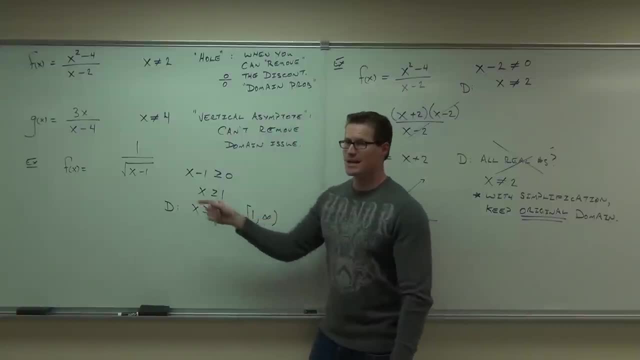 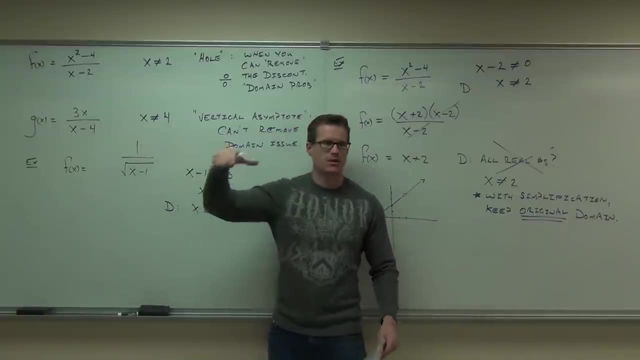 Zero And it's on the denominator. So this would say: oh wait, yeah, even though that's a square root, I can't have it equal to 0, because if I did, the square root of 0 is still 0, and that's on the denominator of my fraction. 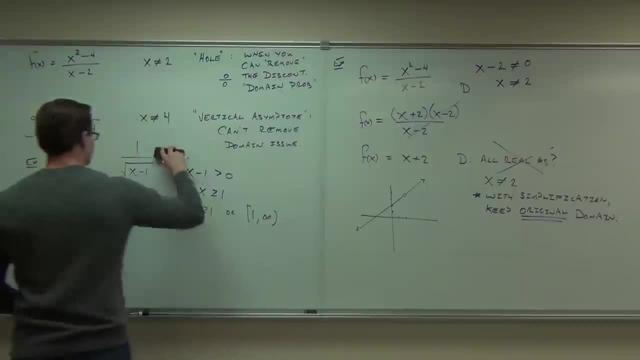 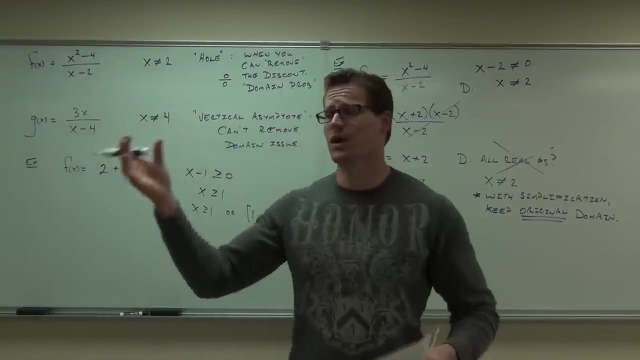 You see the problem there. Yeah, That's you. Now how do you find the range? What's the? how do you get range? How do you get something in the range? It's in the output. It is in the output. 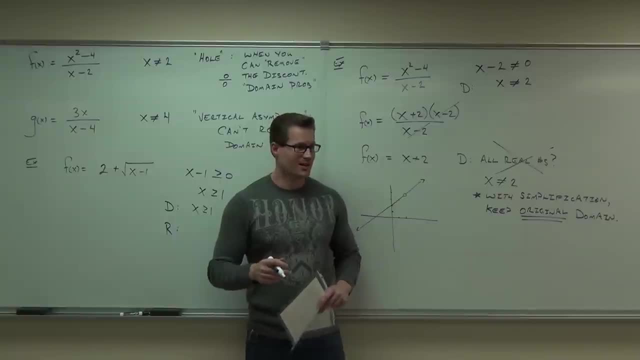 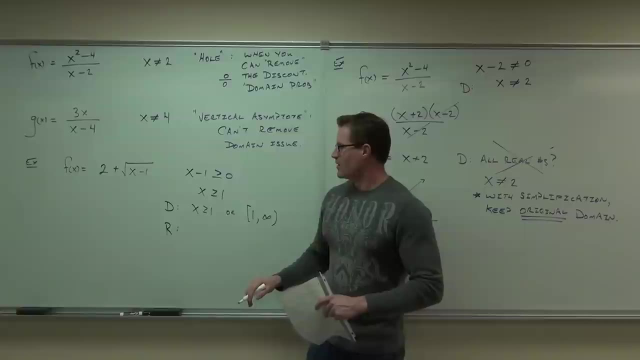 So what? wow, that was a sneeze grenade. Oh my, That was a sneeze rocket launcher. I'm allergic to this stuff, Allergic to calculus, Me too. I start getting all amped up and excited. 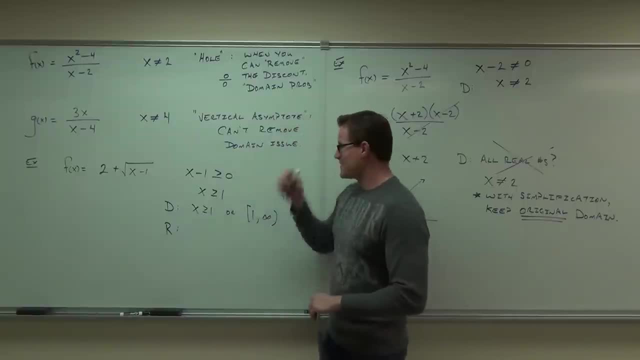 Anyway, what are my inputs up here? What can you input? Give me an example that you can input. You can input: 1. Give me something else, 3., 3. Someone else give me something, 5., 5.. 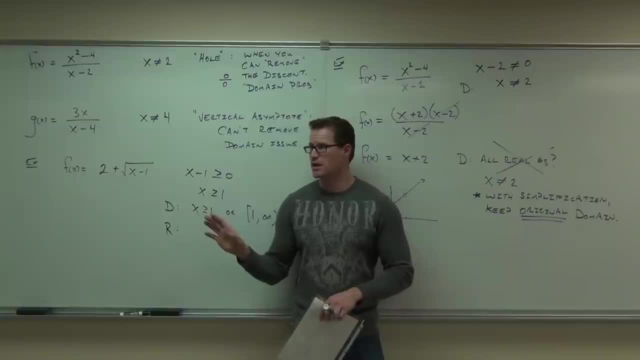 Any real number bigger than or equal to 1,. yes, That's everything I can plug in Now. this says what you can use. You can get out right. It says: plug in something, You'll get out something. So start with the first number you can plug in and plug it in. 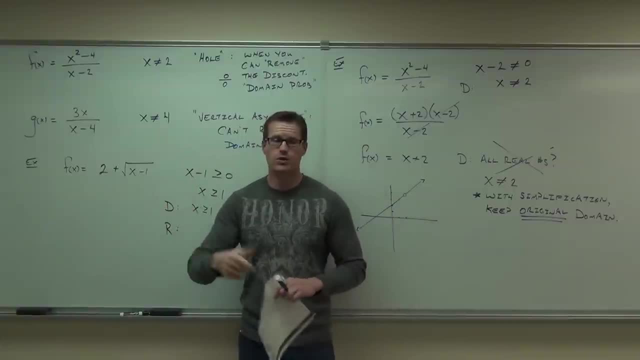 If you plug, what's the first number you can plug in? 1.. Plug in 1.. What are you going to get out? You're going to get out what? 2. 2. So this is starting with 2.. 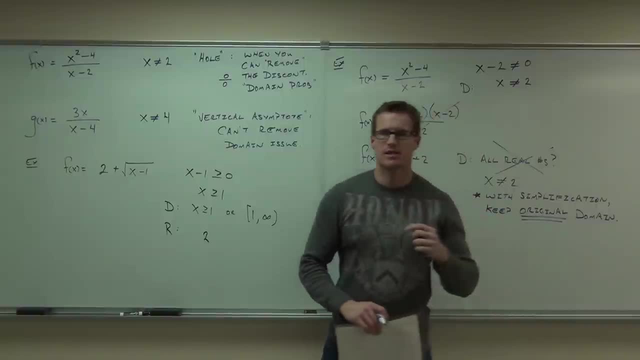 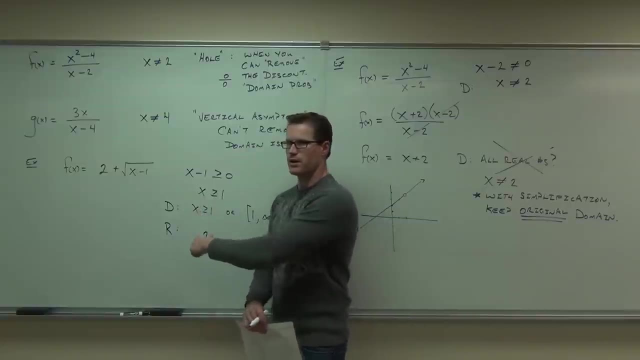 Now take another number, any number, plug it in and see which way you're going- higher or lower. So pick a number in this domain again, like 3 or 4 or 5. See which way you're going. Where are you going? 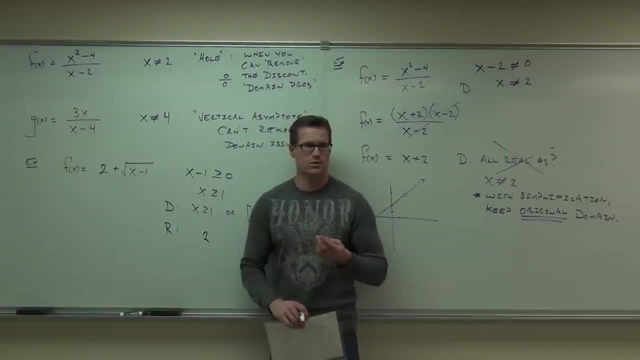 Pick out, pick 2.. What's 2 going to give you? Or pick something easier than 2. Pick 10.. I don't care what you pick, Pick 5.. Pick something like that, Pick 5.. Okay, What's 5 going to give you? 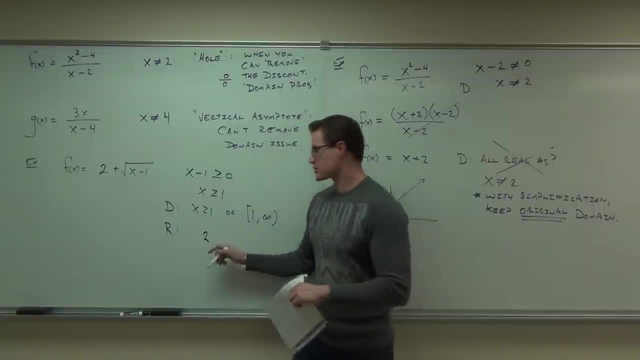 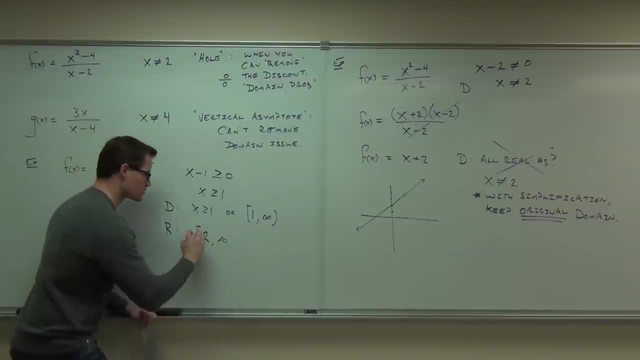 4.. Ah, there you go. Are we getting bigger or smaller than this? So we know that this is going to, as I plug in, bigger and bigger numbers towards infinity. this is getting bigger and bigger towards infinity, So my range goes from 2 to infinity. 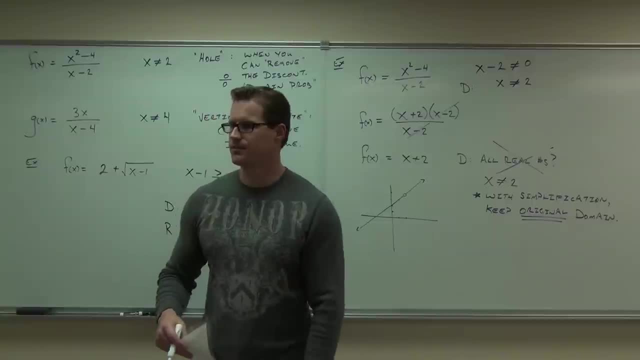 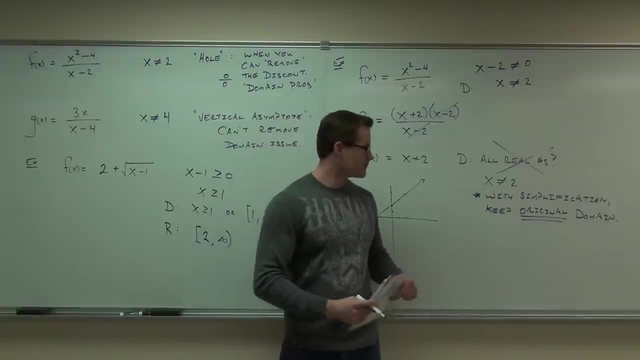 So how do you find range? Well, you plug in your domain With limits. we're going to find out how to do range a little bit differently, But for right now you plug in your domain. You still feel okay so far. 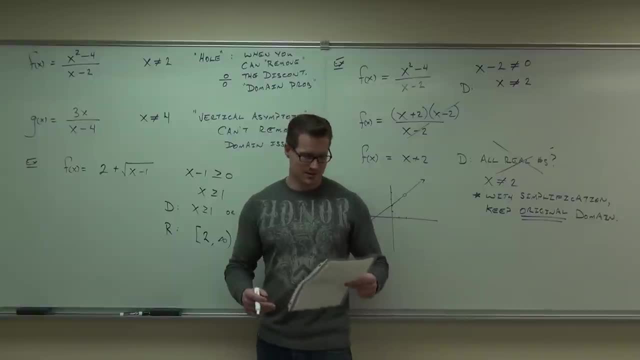 Yeah, Yes, yes, yes, Indeed, Indeed, All right, So let's try one more. We'll go on to our super fun word problem. Do you get familiar with odd and even functions? Oh boy, Oh boy. 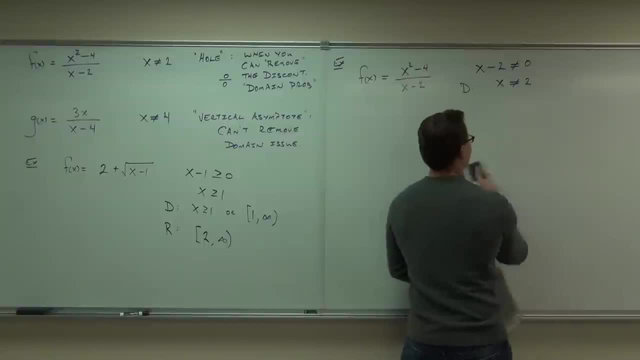 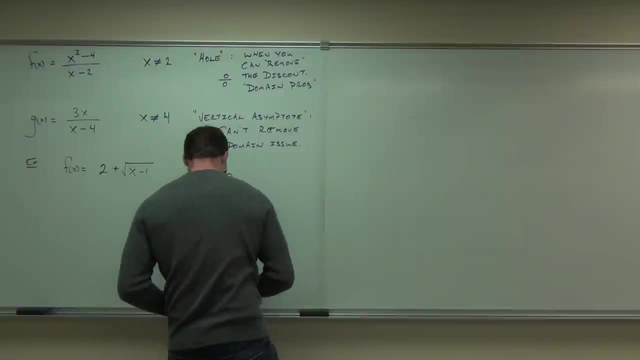 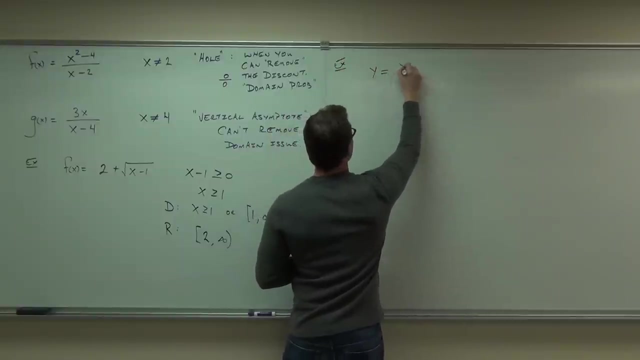 Oh boy, Okay, We'll talk about two more things then. Refreshment, Yeah, refreshment. We want domain and we want range. First things first. let's talk about your domain. Are there going to be any issues with our domain here? 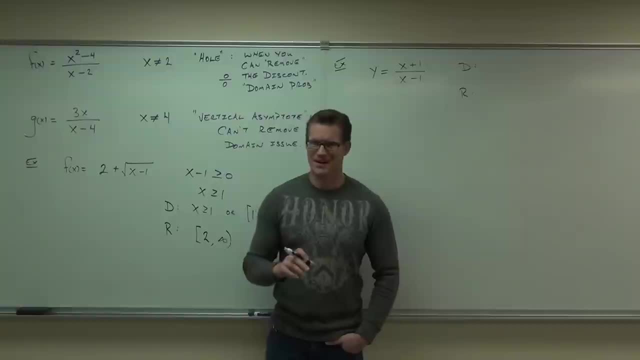 Anything that we can't plug in One One One. What about negative 1?? Is that okay? We'll get 0 over negative 2.. Is that all right to have Sure Zero over a number? that's fine. 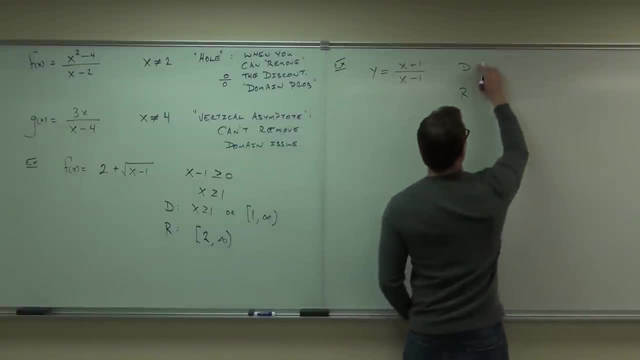 That's zero, But something over zero, that's not okay. So for our domain we go okay. I know that x minus 1 can't equal 0. So x cannot equal 1.. Well, that's pretty clear. 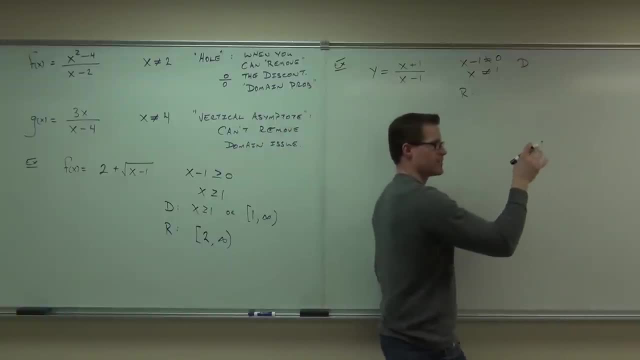 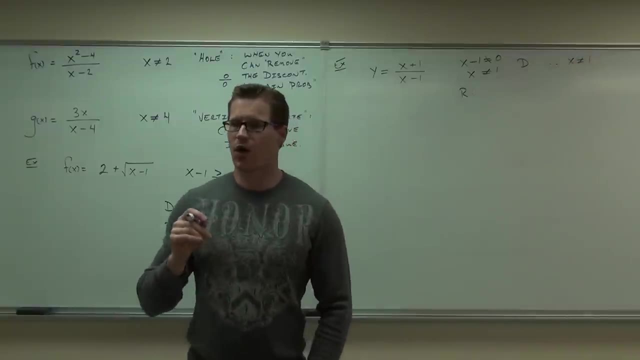 So the domain, The domain is all real numbers except x can't equal 1.. Now the question I have for you is: is that thing a whole or is that thing an asymptote Whole? What do you think? If you don't know, here's how you check. 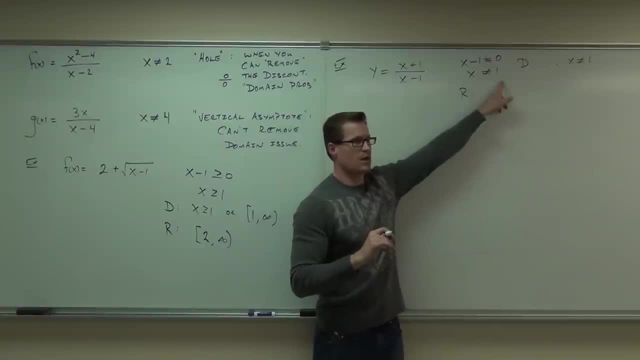 You plug in the number that you're not supposed to be able to plug in. It's like 1.. If it gives you 0 over 0, that means you can factor it out if they're polynomials and simplify it out of the problem. 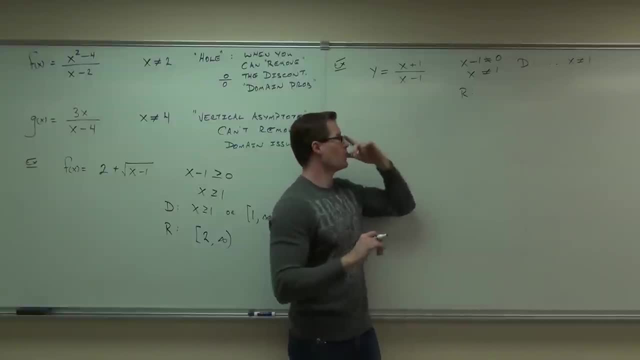 If it doesn't give you that, then you can't do that. You can't factor it out. So If you plug it in, you get 2 over 0.. Is that a whole or an asymptote? An asymptote? 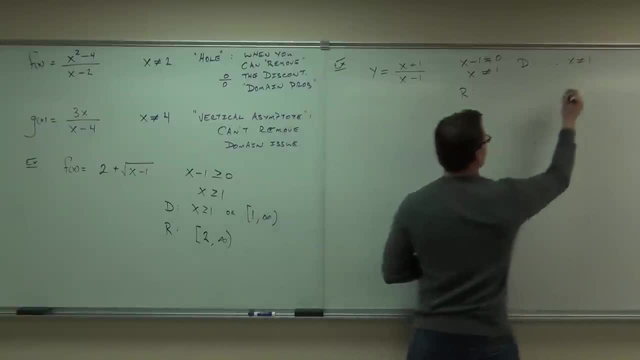 Definitely an asymptote. So we know we're going to have a vertical asymptote at that point. Now you can't really abbreviate asymptote more than that. You don't want a vert-ass, So That'd be just weird. 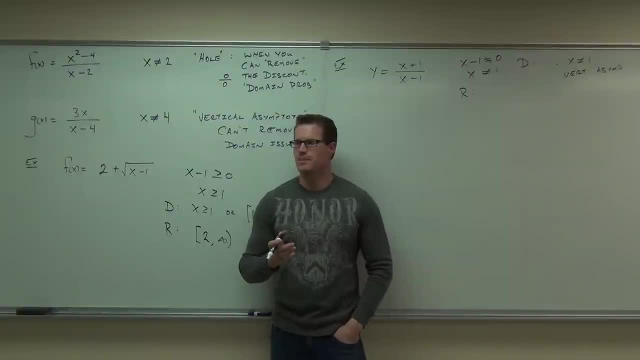 Anyway, how about the range? How about the range of this thing? That's kind of tough right. So you don't know what the range is. Well, there is one thing you can do On certain occasions. this isn't always possible. 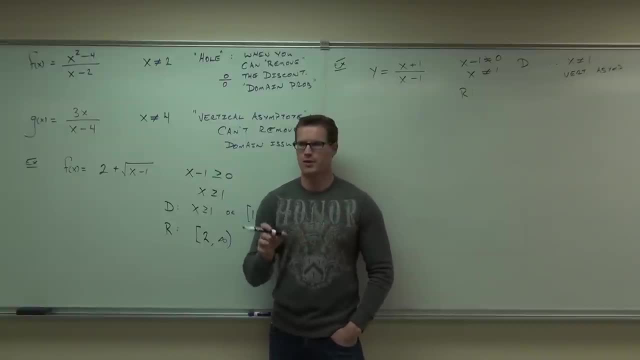 On certain things. if you can solve it for your X variable, then look at those domain problems for your Y. That's actually the range. It's kind of like you're flipping the script on the problem So you can find the range by solving. 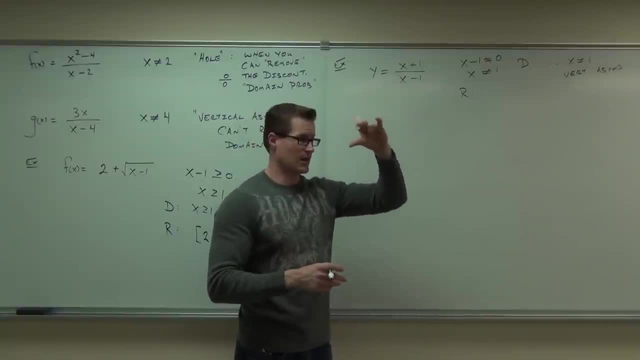 for the independent variable That's going to and then looking at those problems. So if we were to do that, Geez, I don't even know if I want to do that. I don't really want to. I guess I will. 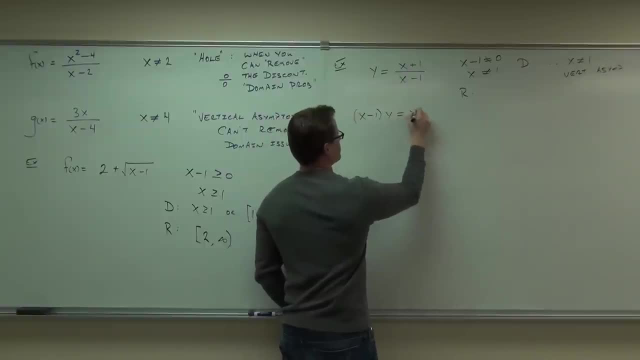 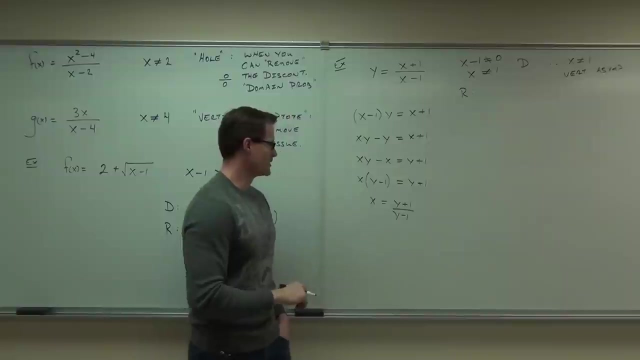 You can do it. I can't. Well, I know I can. Such confidence. I've been doing this a while. You were in math league in college. I made fun of the people in math league in college. Actually, it's a horrible person. 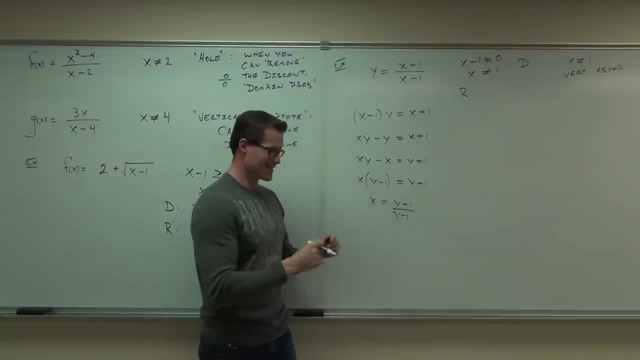 Math league is cool. Do math league It's fun? I swear It really is. I was just. I was too busy with other things to do that. Anyway, do you have problems here? Answer's: yes, It's the same. 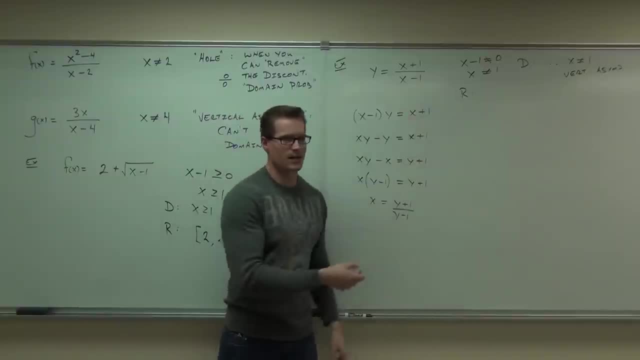 Oh yeah, it is the same. That's just. it's kind of weird That worked out exactly the same. I did this right. trust me, You can follow it down. This is correct, But now that we've solved for X, if you find the domain, 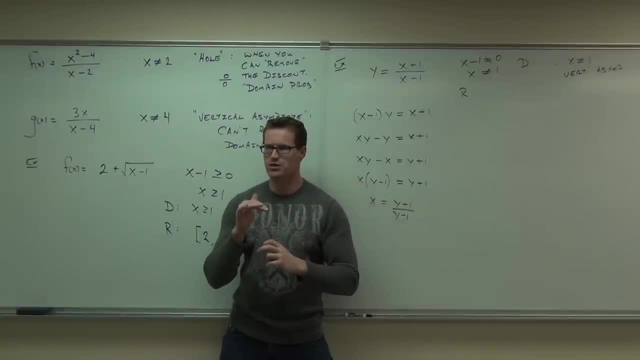 for your Y's. that's actually the range of your function, Do you see? the? It's kind of cool, right? You say, well, if we have any problems on our Y's, that means we have problems in our range. now. 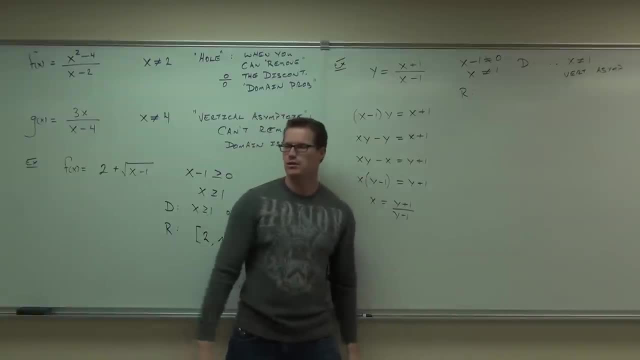 Well, we're going to get out of the function. What's the problem? What can't you get out One One? What's the problem here? What can't you get out of this? You can't get out one because Y couldn't equal one. 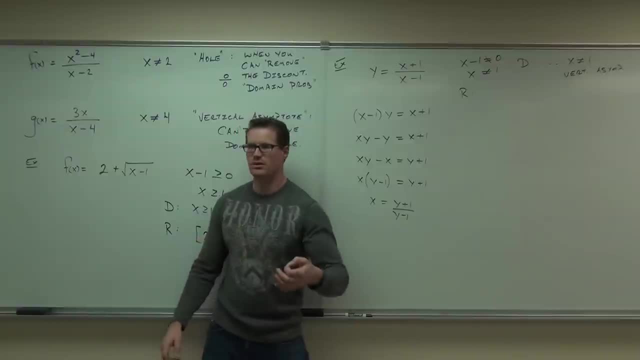 Do you see how Y can't equal one here, Yes or no? Okay, So if you do this whole idea backwards and you solve this for your independent variable and you make it so you're kind of like you're finding the domain of your dependent variable. 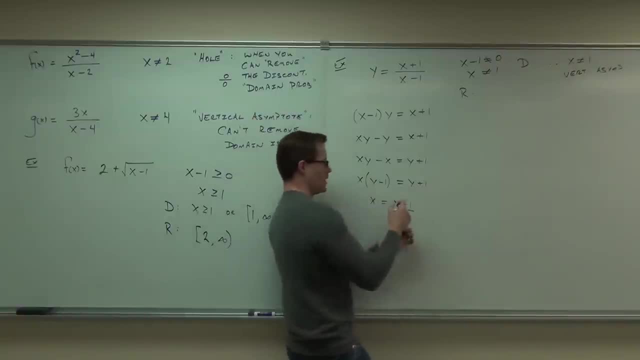 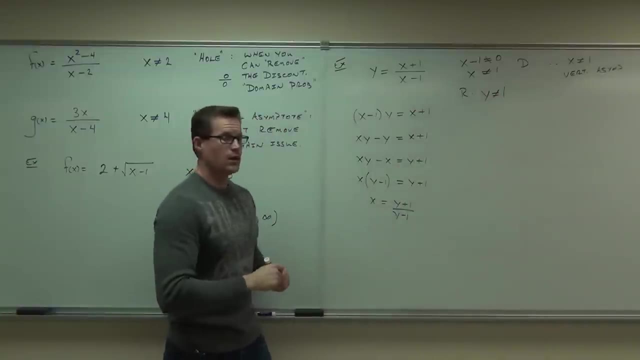 your Y here, that's going to give you a range. So our range would say: well now Y, I know Y cannot equal one. Can you simplify out this domain issue, which is actually a range issue? Can you simplify out that? 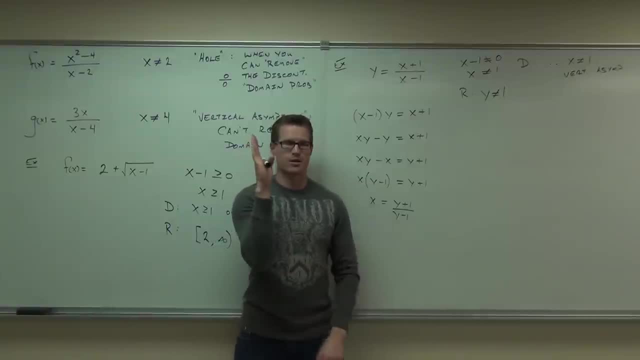 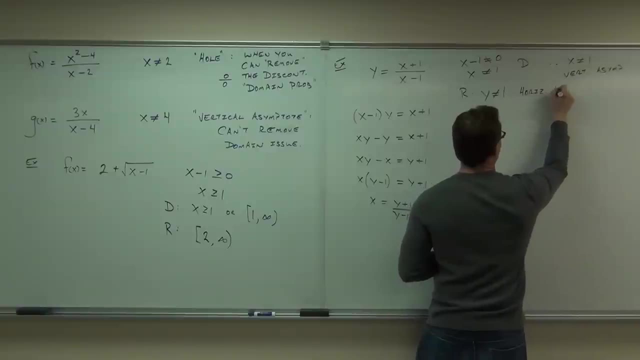 Then this is an asymptote as well. Well, it's not a vertical asymptote. What is it Horizontal? It's a horizontal asymptote. Now, we're going to have a better way to find horizontal asymptotes in the future, because, if you haven't noticed, 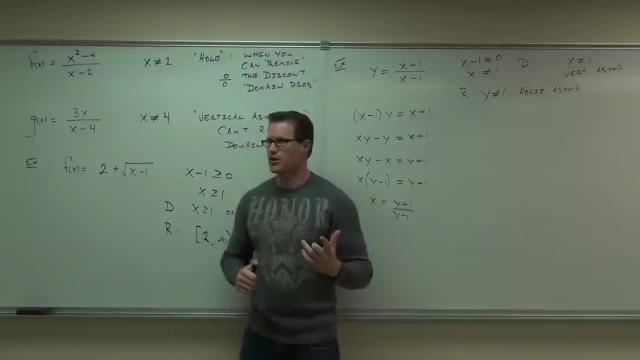 this process for here. this is really easy. But for every function, can you always solve it for your independent variable, Not even close? No, no, no, That would be ridiculous. So we're going to have a better way to do that in the future. 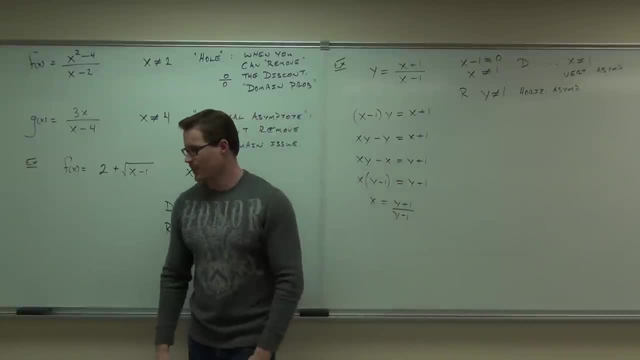 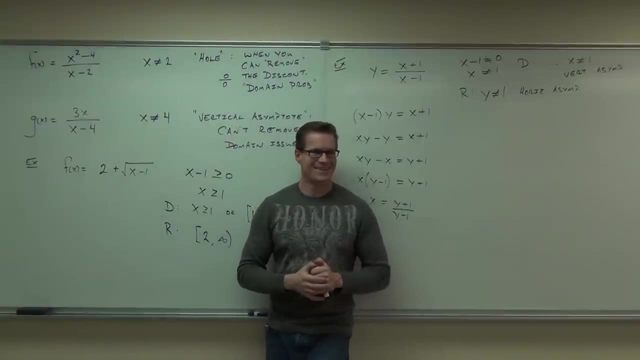 but for right now, that's how you can find your domain and your range. How many of you feel okay with what we talked about so far? All right, You ready for a word problem? No Answer is always Yes, Yes. 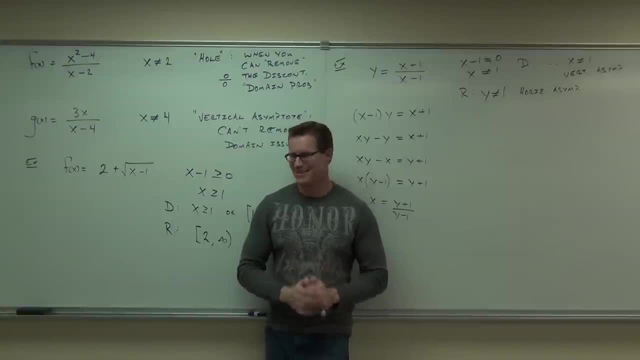 Yes, You ready for a super fun word problem? then, Sure, Why not? Why not Come on? You know you're not getting out of it anyway, so you may as well enjoy it. Wait, does that exist, the word problem? 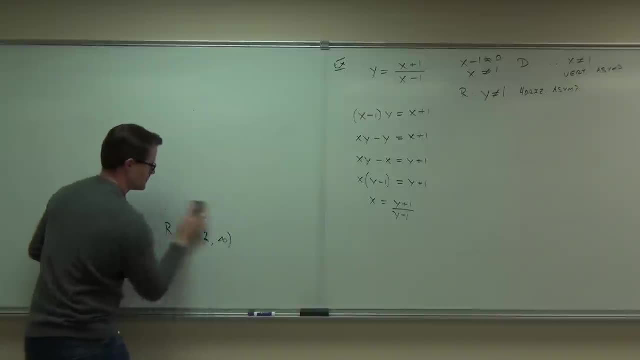 Yes, it exists. I'll prove it to you right now. It exists, It exists. It's just probably there. There, it is All right. Look at that. Here's what we're in the business of. We're in the business of making cardboard boxes. 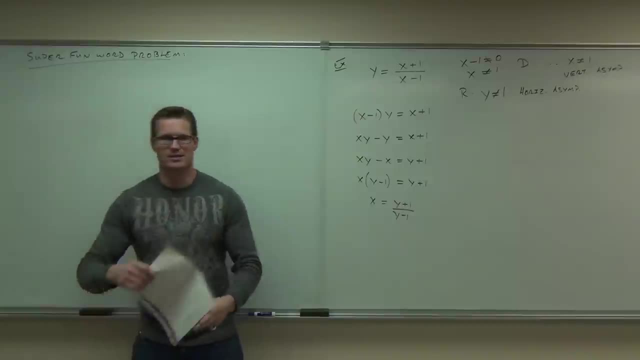 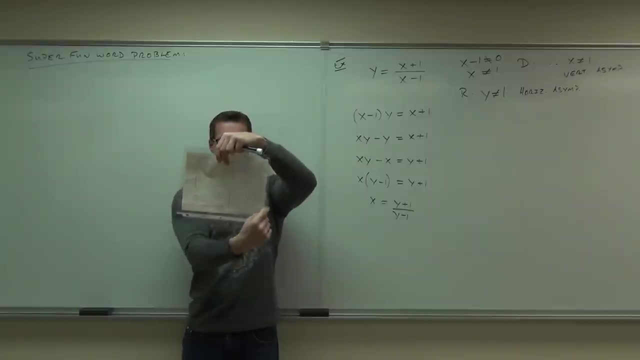 What we're going to do is we're going to take a cardboard box and make it by doing this, taking your flat piece of cardboard, and we're going to cut out a square here, here, here and here and fold up the sides. 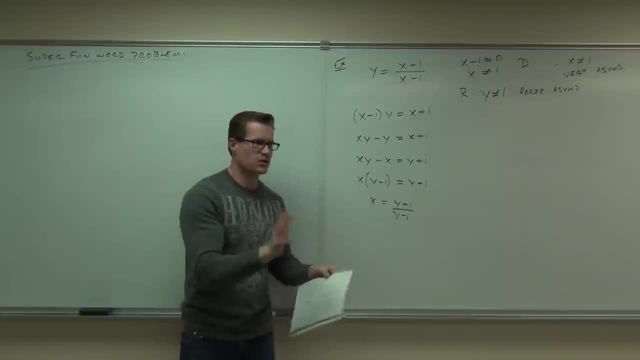 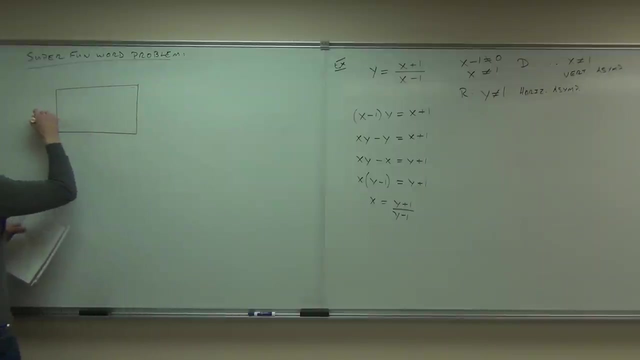 Will that work to make a box? Mm-hmm, We'll use some tape around the sides and make a good-looking box. So a very cheap way to make a box. So our box idea is: We're going to take a piece of cardboard that is 16 inches by 30 inches and we're going 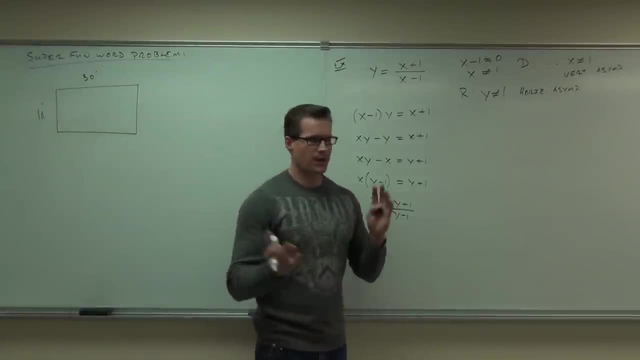 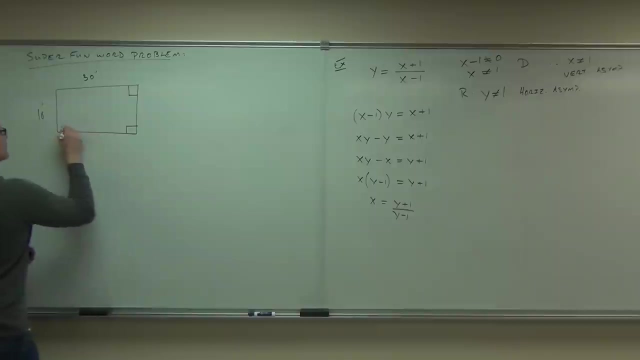 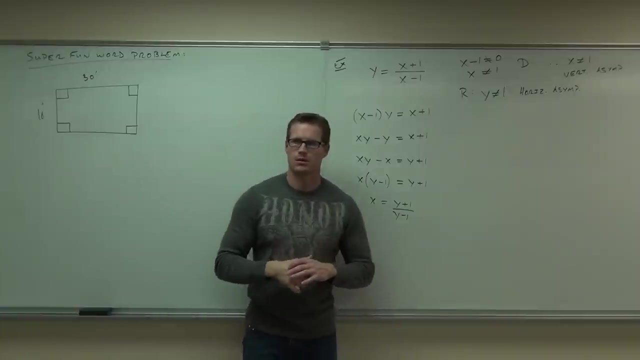 to make a box by cutting out squares in the corners and folding up the sides. Tell me what you know about the squares. Can the squares be different sizes? You have a really stupid looking box. You're like, nah, that's not going to work so well. 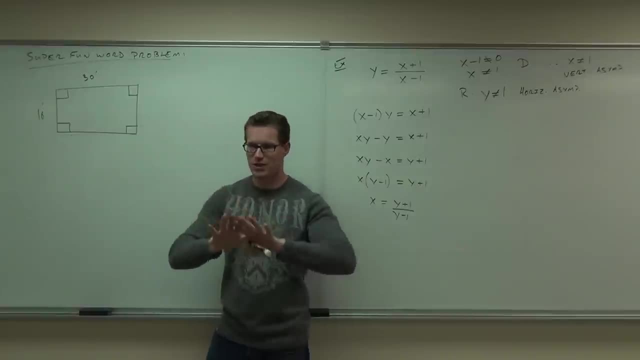 So if these aren't the same lengths all the way around, you're not going to be able to make your actual fold flat like shirt box right that people like to use for presents. So I know, if I call this x in order to make my nice corner, that's also going to be x. 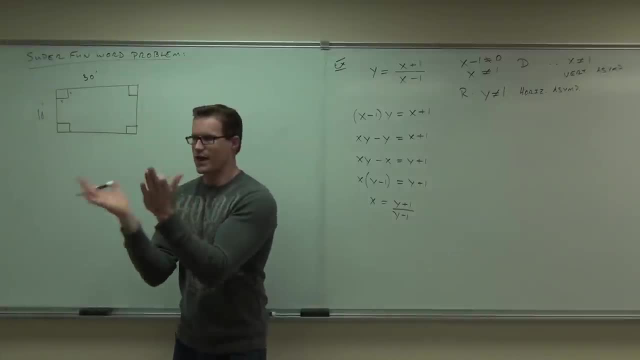 right, Yeah, But as soon as we do that, every other, Every other corner has to be exactly the same, otherwise our box is going to really not be that great and you're going to get fired from box making. How bad do you have to be to get fired from box making? 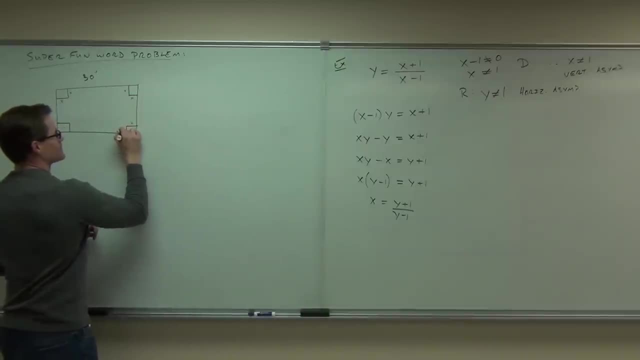 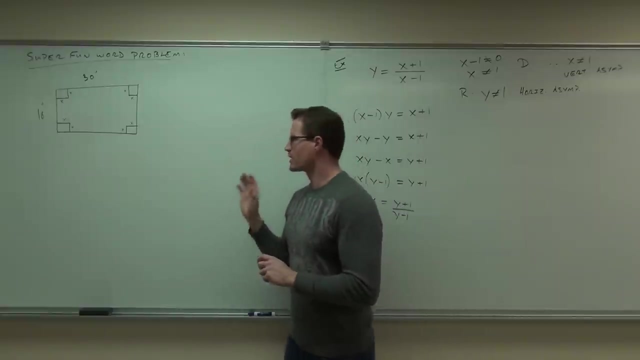 I mean, come on, No, I'm just kidding. I'm guessing you have to be pretty bad. So we've got this piece of cardboard that's 16 by 30 inches. We're going to cut out those corners so we get this machine that's going to come down. 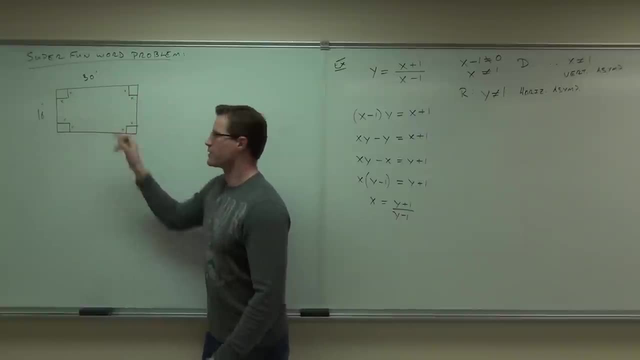 and then maybe it indents it here, here, here and here, and we're just going to fold the sides up and crease them. I think what they actually do is they fold the sides up and crease them. They probably just make one cut and then fold the sides over. but we're a little more. 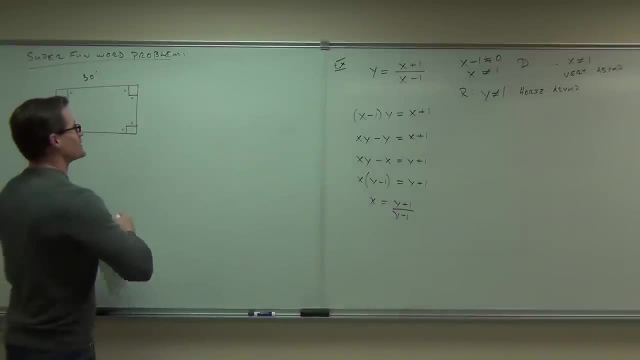 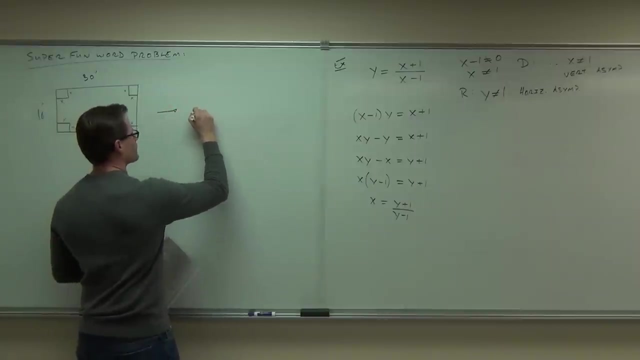 advanced than that, Our box. when we're all said and done, let's see if I can draw. this should look something like this: You took a 3D drawing class. No, I didn't. I don't want to. 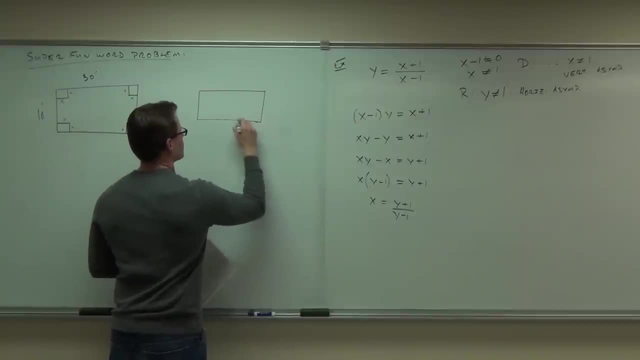 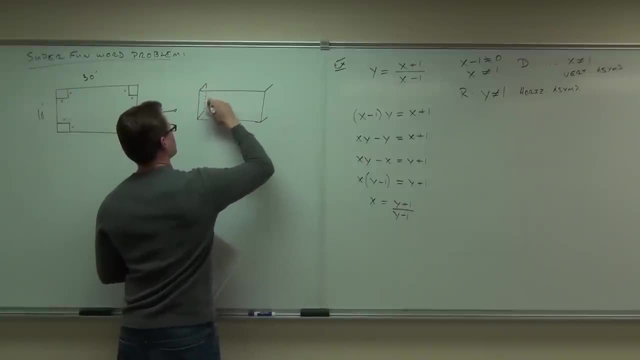 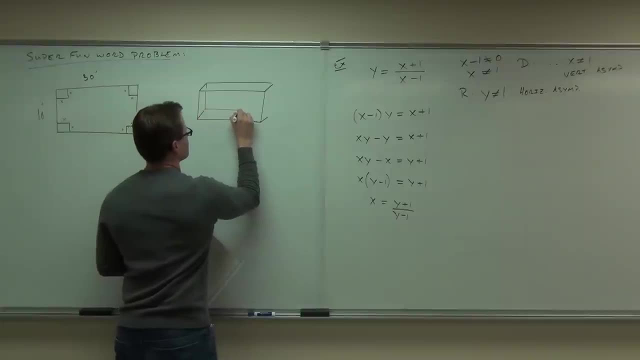 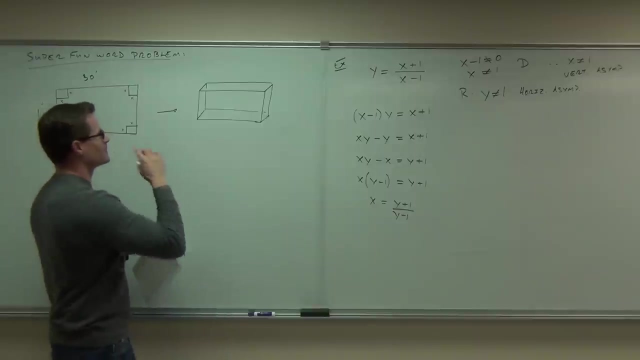 Never mind, Yeah, I was. you guys are giving way too much credit, So if I'm folding this up, it's still sitting the same way, as it's going to be on this edge. Is this still 16 inches long? Because what I want to do is I want to find a formula for the volume dependent on X. 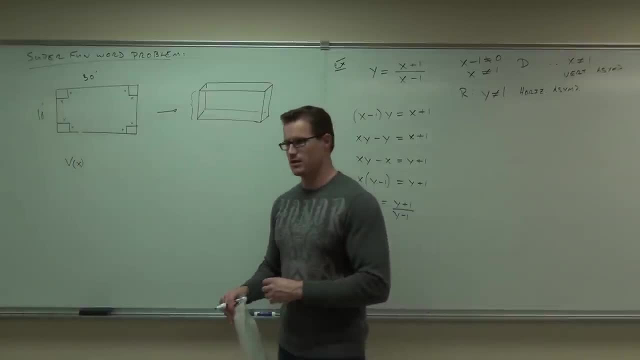 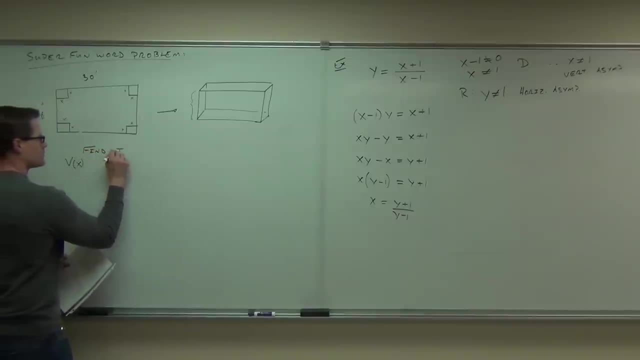 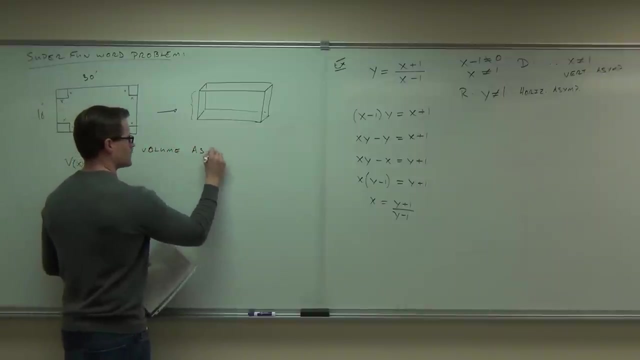 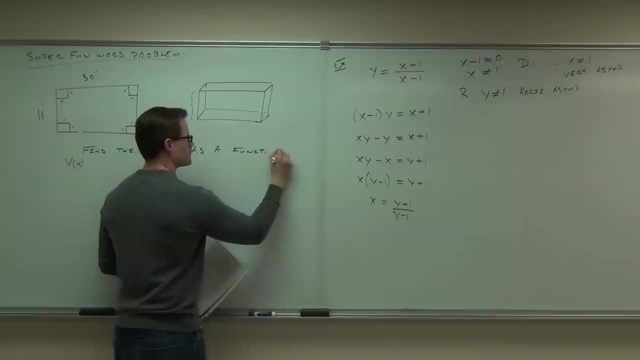 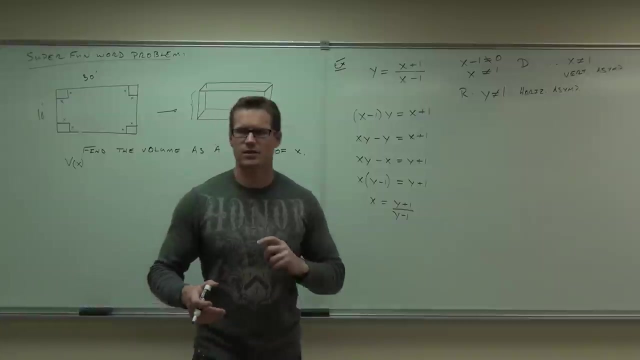 I want to find a formula for the volume depending on the size of the cut we're making in this cardboard. So find the volume as a function of X. How far is that? Is it still 16 inches? How much is it 16 minus X? 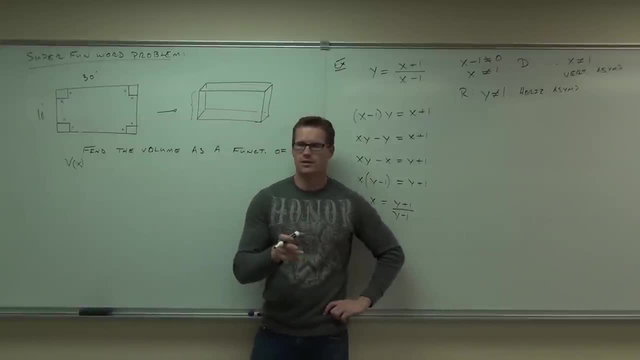 Yes, 16 minus 2X. Why 2X? Because you have to do it in each corner. Yeah, if we cut both corners and fold that up, we're missing not only one X, but the other X as well. 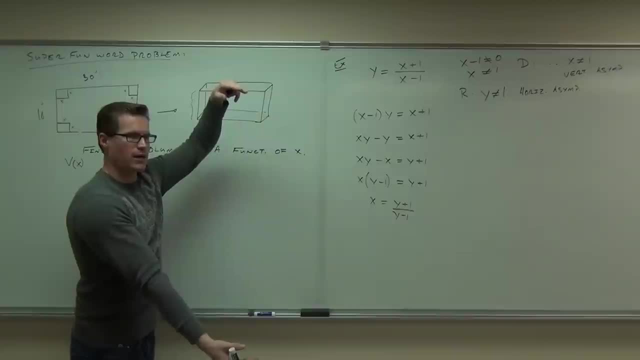 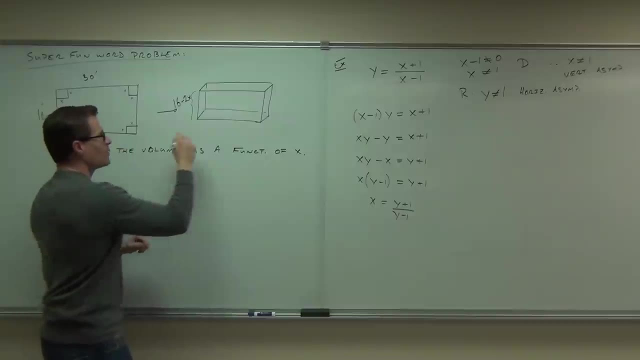 So if I were to find this- yes, I know the maximum length is 16, right, And if I subtract both those cuts, I'm going to get 16 minus 2X. absolutely. What that means is: how about this length? 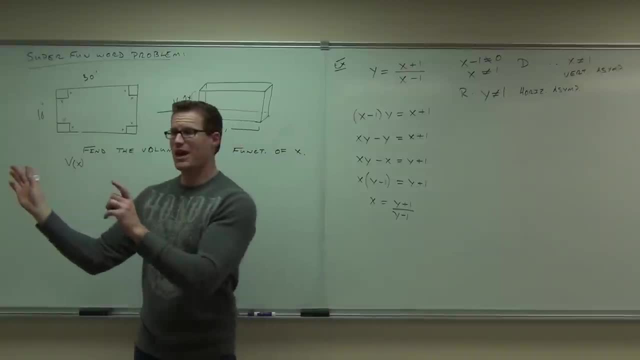 What's that length? 30 minus 2.. Sure, We still have the same X, right, because they're squares. So we're going to have 30 minus 2X. What about the depth of our box? How much is the depth of our box? 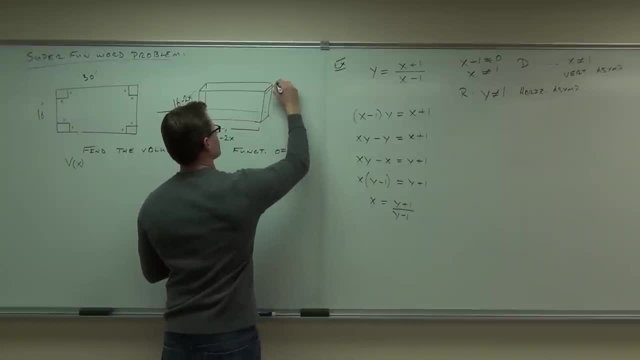 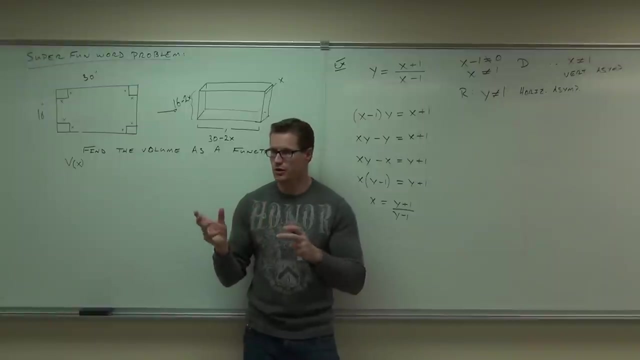 X, X. The depth is X. Okay, How do you find the volume of a rectangular prison like this is: Say what now? So as long as we multiply those three dimensions, we'll have the volume, So our volume should be okay. 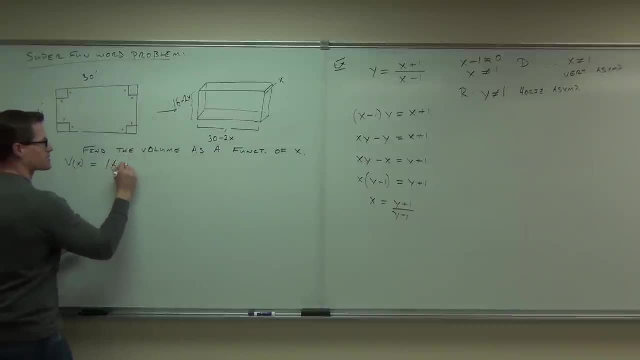 Well, we know that one side is 16 minus 2X. The 2X again comes from the fact that we're cutting out two boxes from each side and folding it up. Then we're going to get. well, the length of this is 30 minus 2X and the depth of this 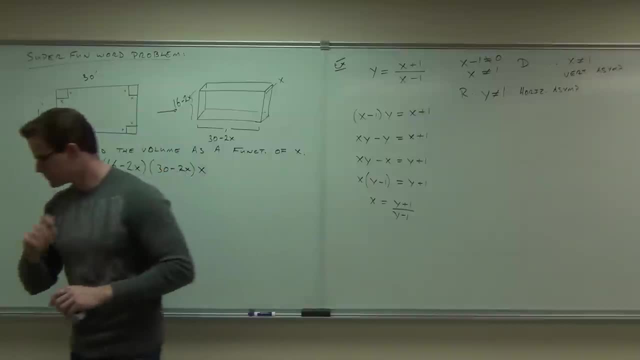 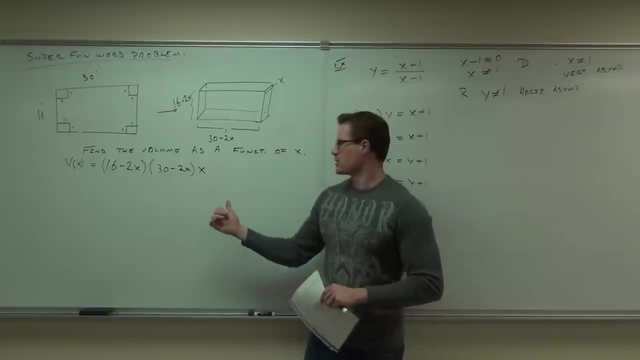 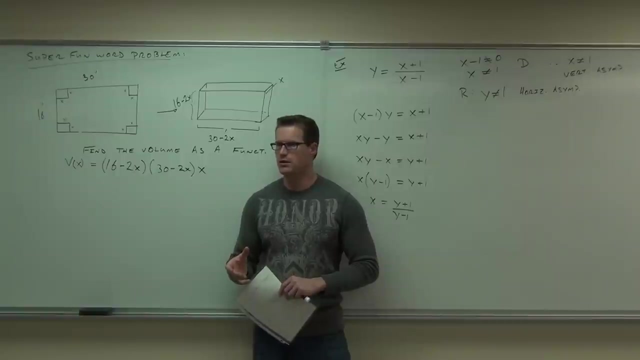 is X. Do you guys feel okay on how to do that? Mm-hmm. If you graph that, could you find out an approximate maximum volume if you put that on your graphing calculator? Mm-hmm, Yeah, if you did, if you work on that and plug that in, or just plug it in, just like. 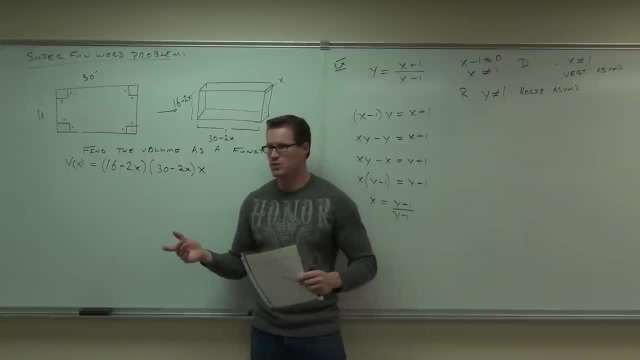 that you're going to get some sort of graph right. It happens to be a cubic graph, So if you found the maximum height for our domain that we're about to find out, you could find an approximate maximum volume for that. That's kind of neat, right. 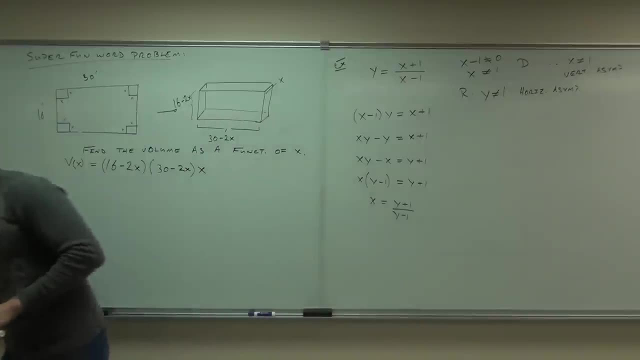 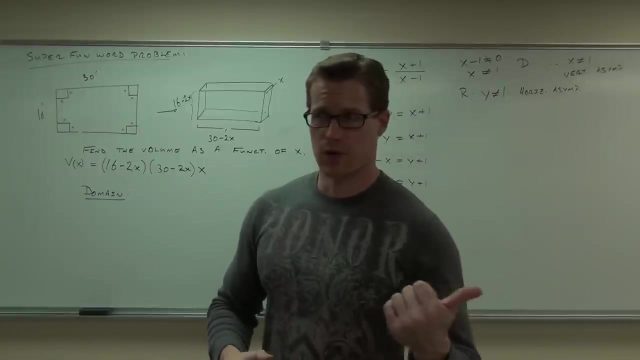 I think it's neat. Okay, That's awesome. Let's talk a little bit, though, about the domain. Are there any issues that we are going to run into with the values of X that we're supposed to plug in? So, firstly, we've got to check for any denominators. 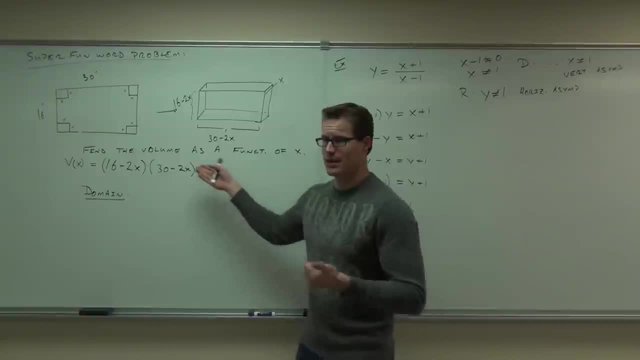 Are there any denominators? No, Okay, That's okay. That doesn't fill that part. How about roots? Do we have any roots? No, So we have no issues with that. How about some realistic constraints, though? Is there anything that I'm not supposed to be able to plug in for X? 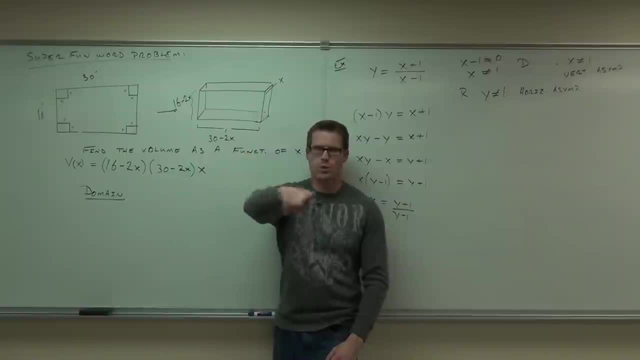 Because I'll tell you, when you put that in the graphic calculator, it's going to go: Negative measurement. What now? Negative measurement? Explain, Why not a negative measurement. You can't measure negative centimeters. Yeah, I can't tell you. 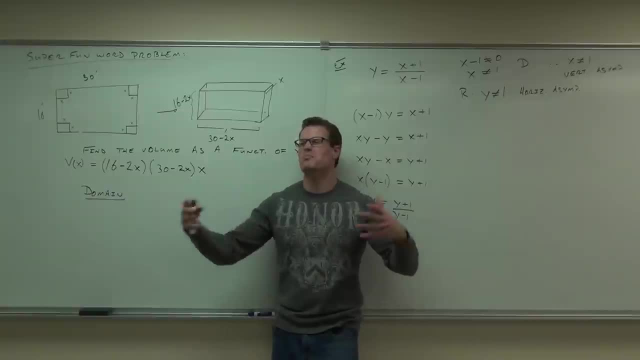 Would you make a box up please and put a negative two-inch cut in it? It's going to be bigger, It's imaginary. Can you do that? Yes, It's not going to hold very much right, It's going to be flat. 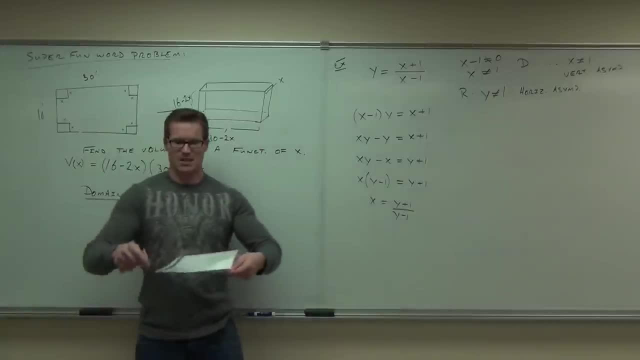 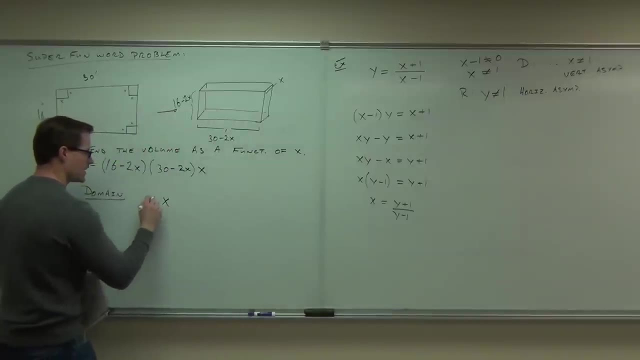 Well, yeah, You can't even do it. You can't say: make a negative, cut out of my piece of paper here. That doesn't make sense. So we know for a fact that, Okay, We know for a fact that X has got to be greater than zero, for sure. 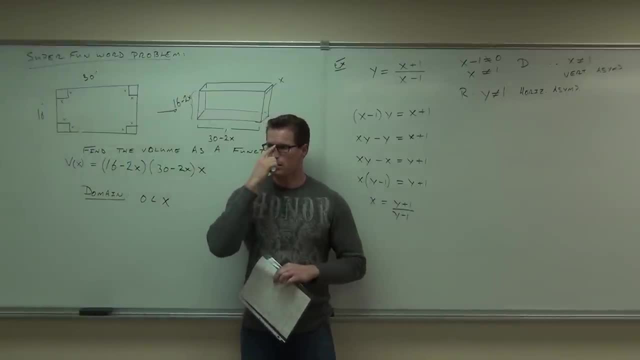 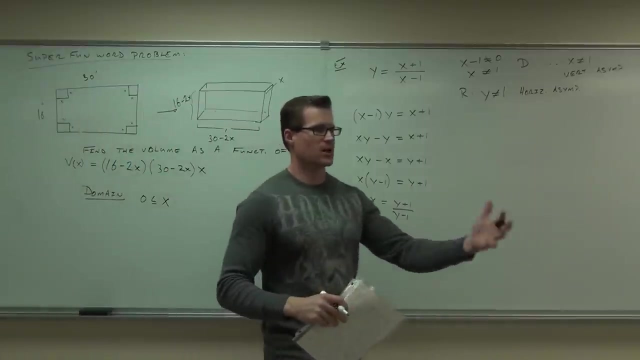 Could X equal zero? But could it equal zero? Could you make no cut? Here's your box. Try to put a package in that. Yeah, it could. It could equal zero, for sure. Is there a maximum cut that we can make for our box? 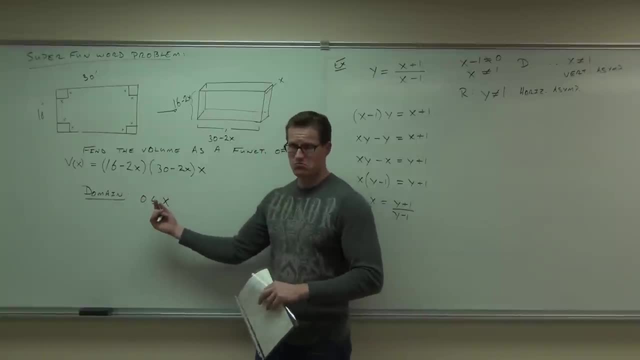 So I know I can't make a negative. I could make a cut of one inch and two inches. Is there a maximum to that? Nothing bigger than 16.. 16., Okay, 16.. Could I make a cut of 16?? 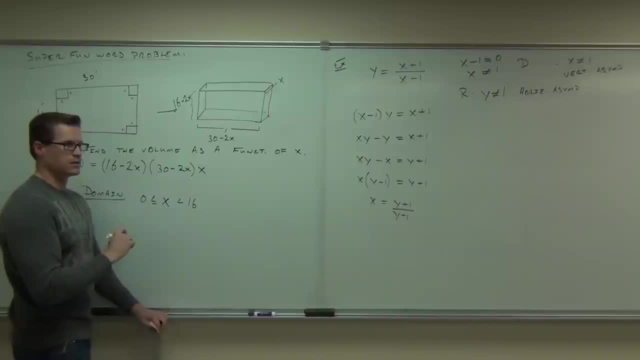 No, Why not? Because I'd cut off your side. Would that make a difference? Yes, Okay, Let's also. I want you to think about that number for a second. So here's your box, right, And what you're telling me right now is: if you have a maximum cut of 16, check this out. 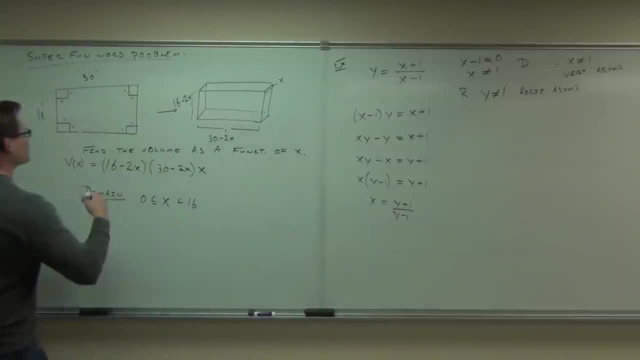 This side, like this. 16, right, You're cutting out two squares, One from the top and one from the bottom. So you're cutting out two squares, One from the top and one from the bottom. So you're cutting out two squares. 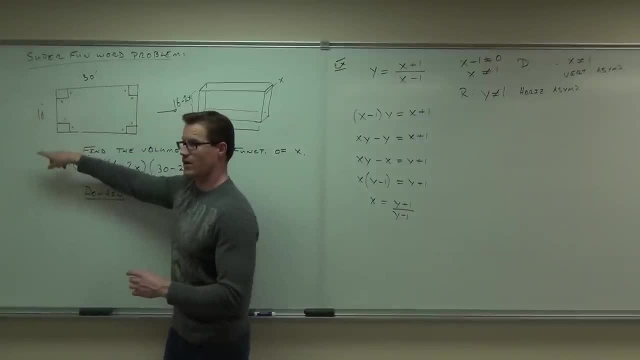 One from the top and one from the bottom. Can I cut out a square of 16 and still cut out a square of 16?? Remember, this would be like a square of 2, 4. And 4 would go there. 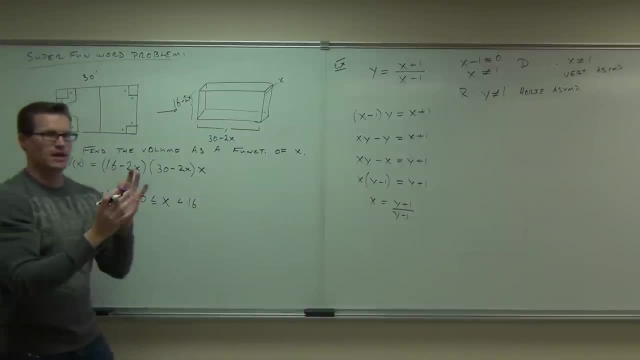 If I take a square of 16, it's the whole thing. That doesn't leave any room for the other square to be cut out of it. Did you get that? That's a problem. Let's rethink that idea. It's not 16 here. 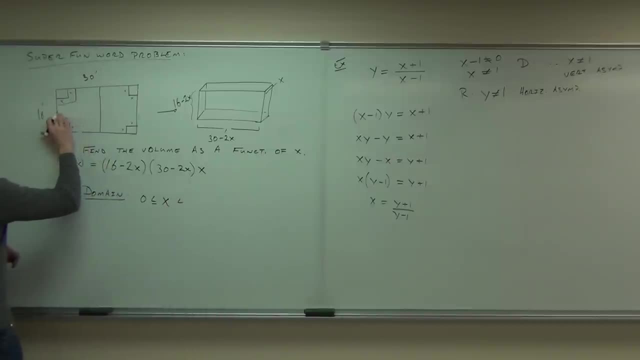 We can't do that. What's the maximum length I could cut? Eight, It'd be eight. It'd be half that length, Because if I made a cut of eight here, I made a cut of eight here. that would be the most I could go without overlapping. 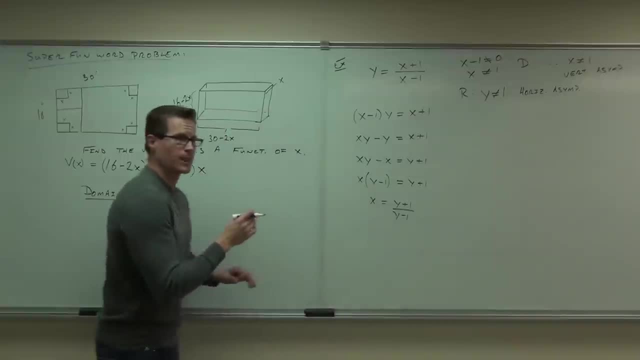 If you overlap, you're cutting stuff that's not there anymore. Yes, But you still wouldn't be able to make a box out of that. No, you wouldn't, but we weren't able to make a box out of this either. 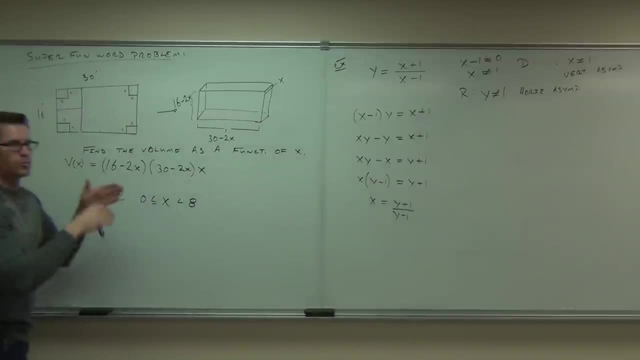 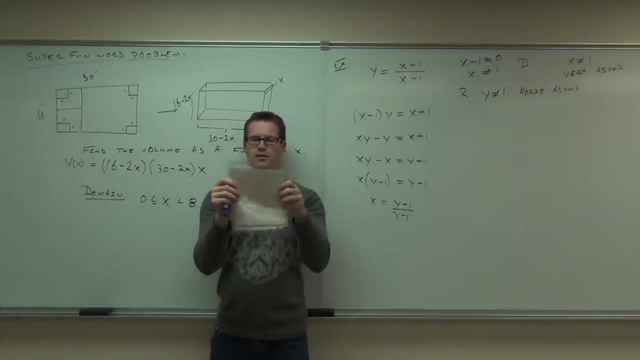 So if we cut eight and eight, can you take off that whole piece of material? Yeah, your box, and you did it from the other side. your box is going to look like: oh, you cut this side off and cut that side off, equal amount. 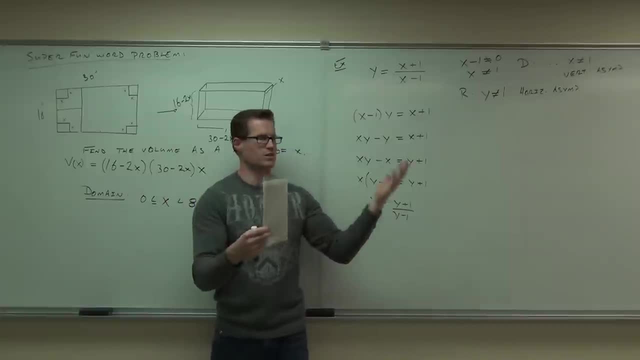 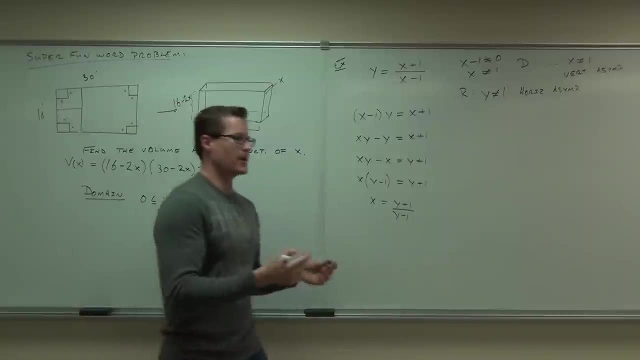 That's now your box. It's a flat piece of paper that's much smaller. You just wasted all your material, But you could do it right Again. you'd be fired from box making, but you could do it, And that's our domain. 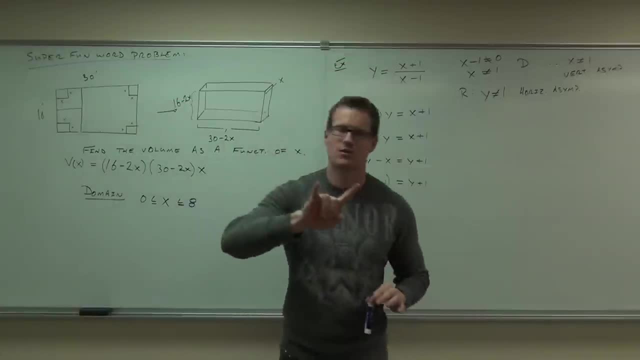 You've got to think about these things. Don't just go with the formula. I know we look for two things in the formula. We look for denominators, We also look for roots. But even if those things don't exist, this is a realistic constraint. 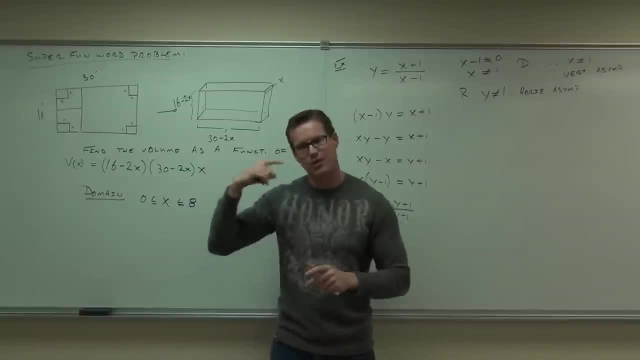 you've got to take into account. If you're dealing with realistic stuff you've got to really think about. don't let yourself get tripped up by the 16. Really think about what you can and can't do with your product. 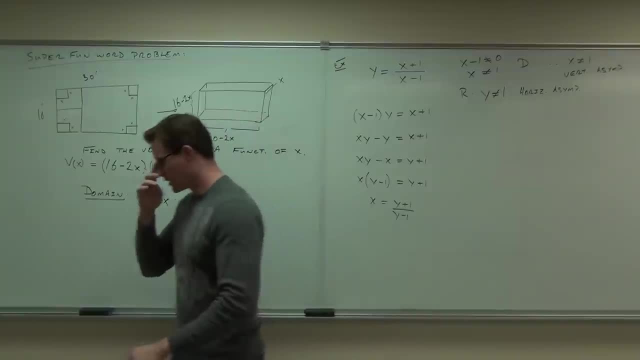 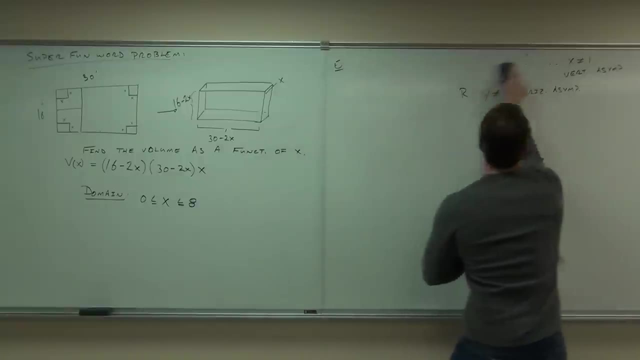 I'm not sure if you're all right with that. Okay, now, I wasn't going to do this, but I'll give you a little refresher on some odd women functions. Okay, Let's talk about this. Let's talk about this. 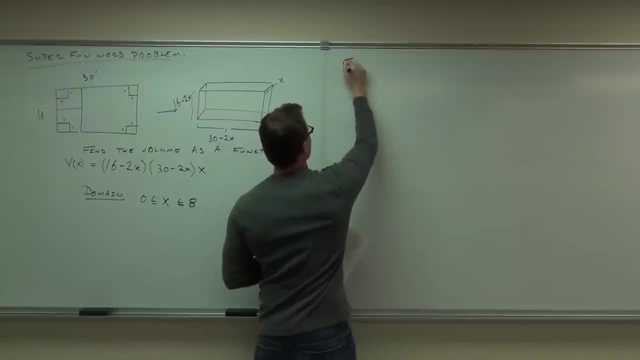 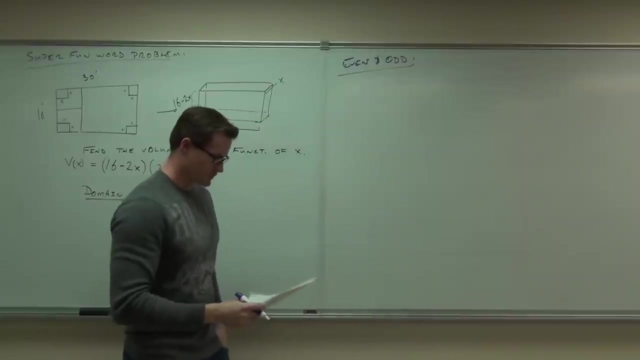 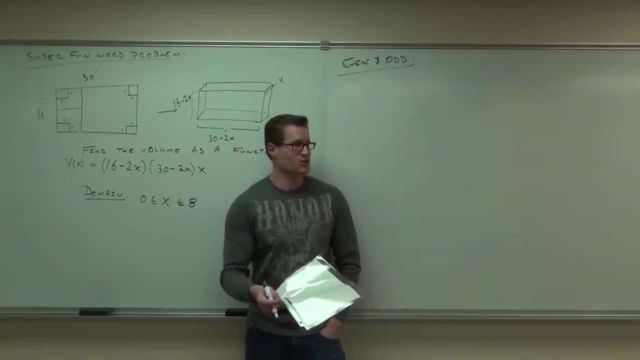 Let's talk about odd and even functions for just a little bit. Even functions are functions that have 2s, 4s, 6s and 8s in them. Well, that's not completely true, but the powers should actually look like that. 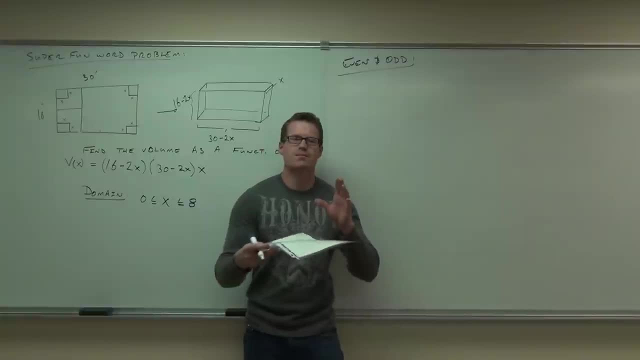 Odds are usually the 1s, 3s, 5s, 7s. What we say mostly, though, is that even functions are going to be symmetric across the y-axis. Odd functions are symmetric. They're symmetric about the origin, which means, if you took them. 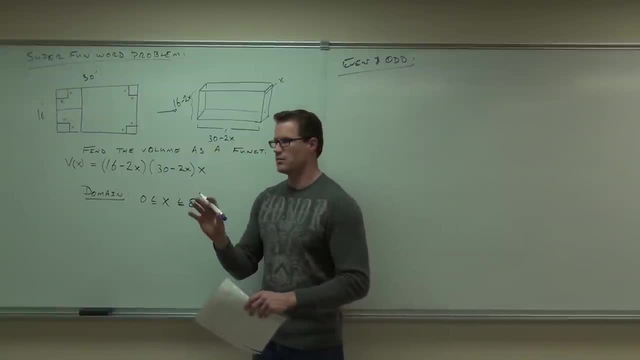 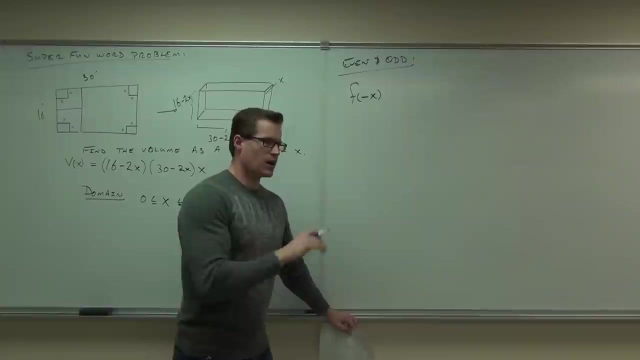 and you rotated them 180 degrees about the origin, it's going to make a mirror image of what you have already. So for even functions, here's what even means, like algebraically or formulaically, when you plug something in. Even function says: if you plug in a negative number or if you plug 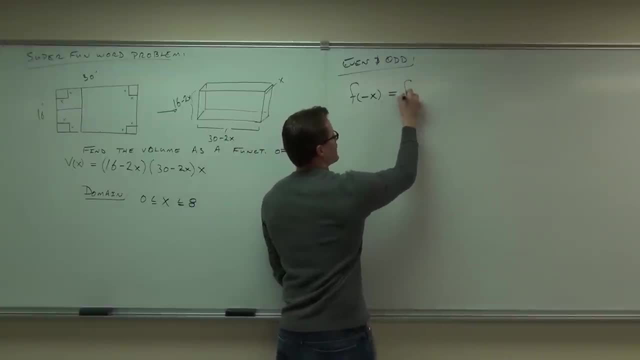 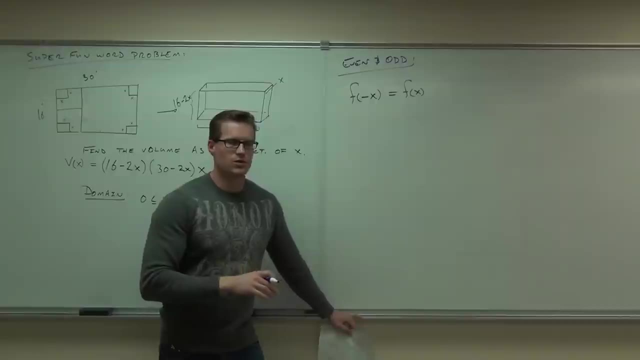 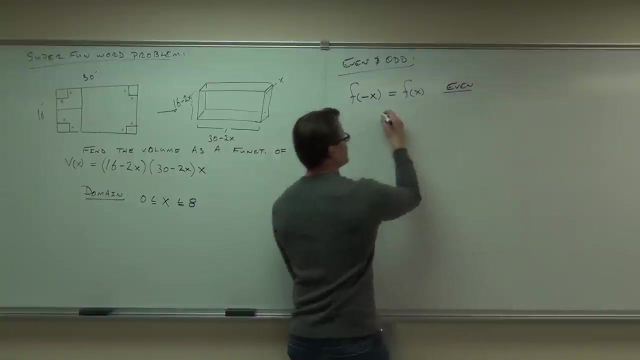 in a negative x per se, it's going to give you back out the function just as if you had positive. So if I plug in negative 2 or 2, it says it doesn't matter. That's even, It is symmetric. about the y-axis: 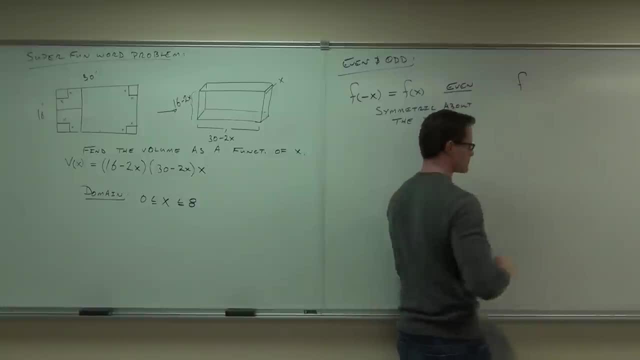 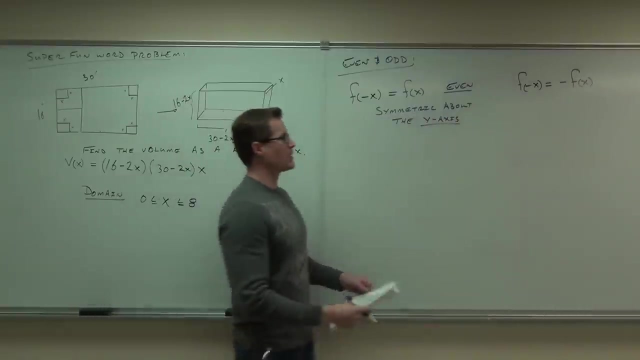 Now, odd functions say this. It says: if you plug in a negative number, it's like taking the function, plugging it in the positive of that number and making it negative. That's what happens with the odd function. It says: if I was to plug in negative 2, it would be like I plug. 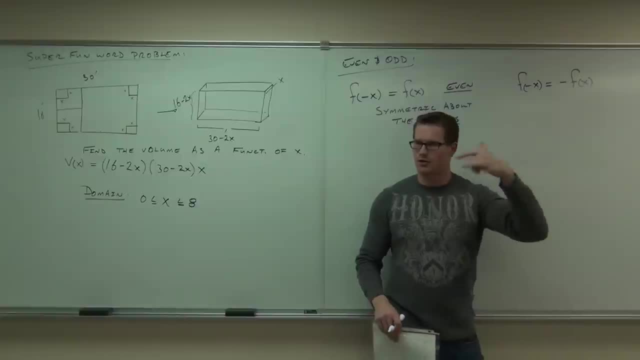 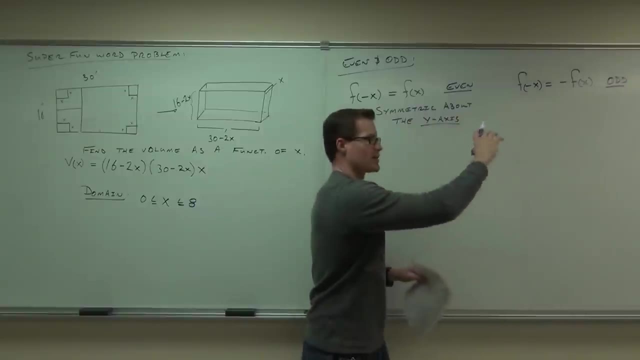 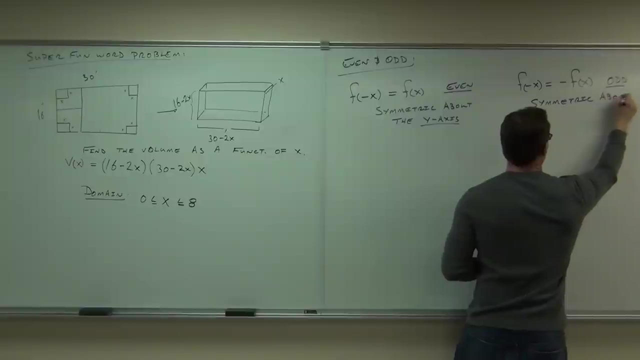 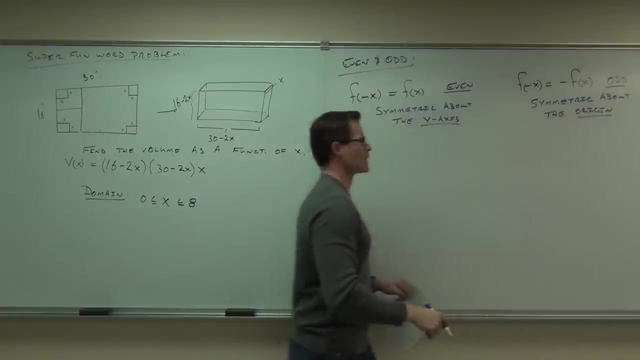 in positive 2, got the answer and then made it negative. Do you see the difference between these two things? All right, This is odd And it's going to be symmetric about the origin, All right, So I can see examples of functions that are even and odd. 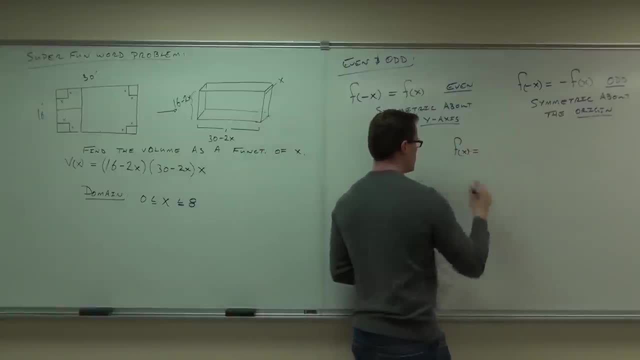 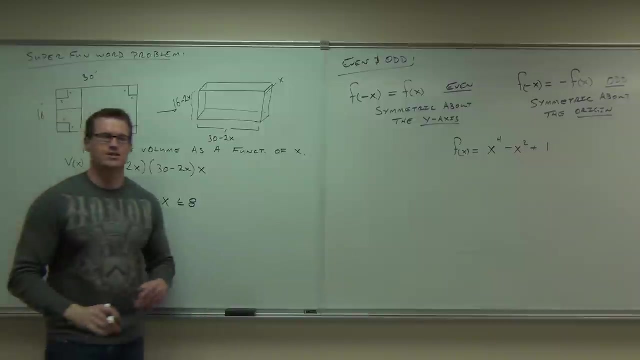 Let's find one out. It's just one, each One, each. Well, you guys are asking for the moon today. Here's how you test whether something is even or odd. What you do is you plug in the negative x and you see what happens. 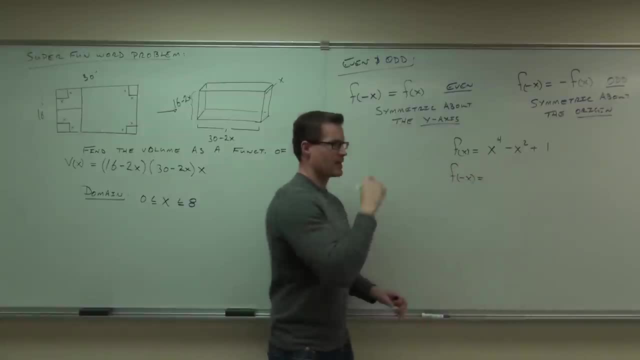 So I'm going to find f of negative x. What that means is that for everything that's even and odd, you plug in the negative x and you see what happens. So I'm going to replace: I have an x. I'm now going to put a negative x inside some parentheses. 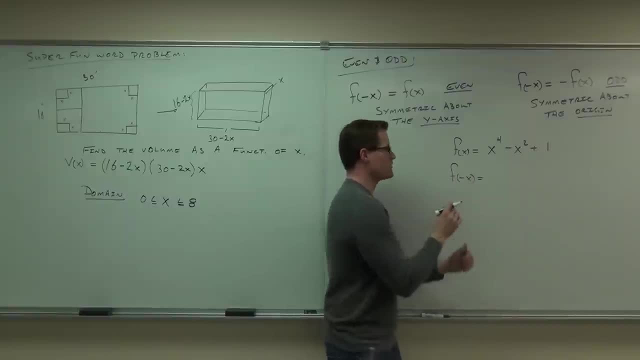 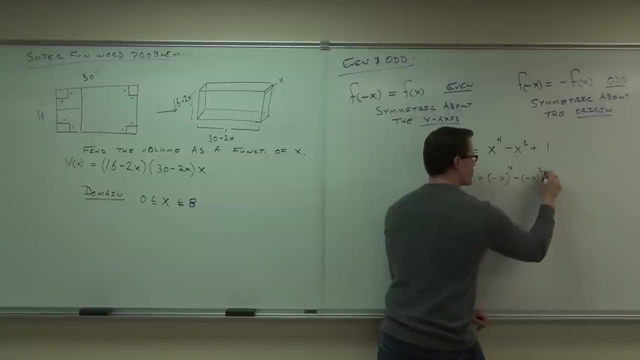 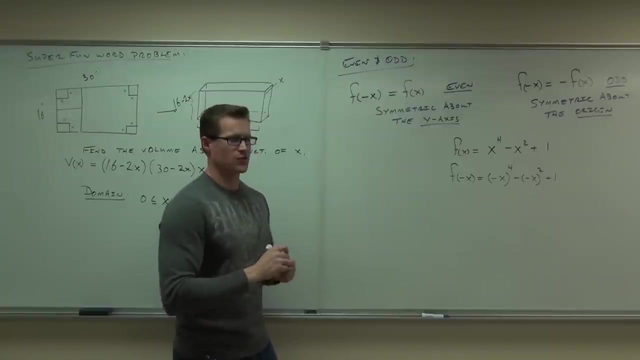 It's like you're composing a couple functions, okay, You're just replacing x with negative x. So that means for this, you'd say, I want to see what happens with negative x to the fourth, minus negative x squared plus 1.. So far, so good. 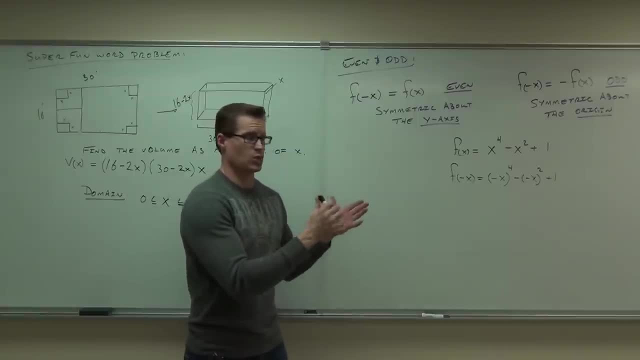 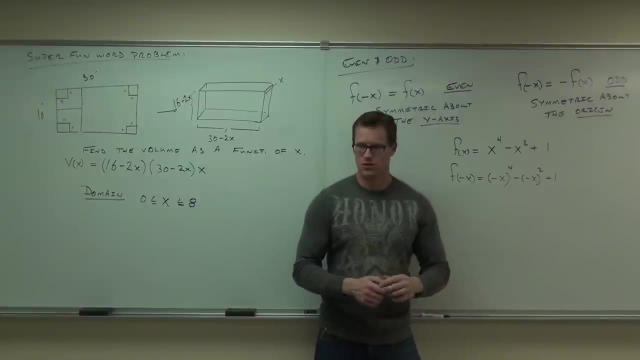 Don't use an actual number. You don't need an actual number, Just use the negative x. It's still going to work out for you How much is negative x to the fourth, X to the fourth, Because the negative also gets to the fourth power, right? 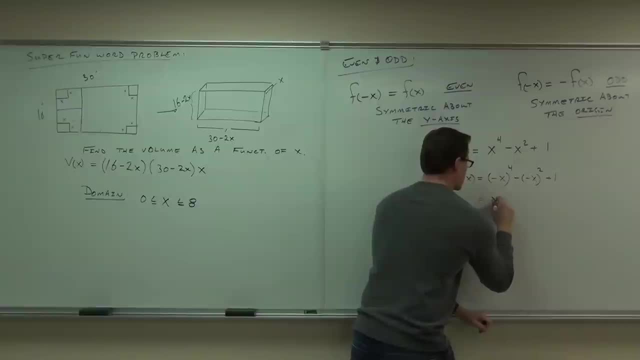 It's going to go away, It's going to be positive. So this is going to become x to the fourth. How much is it? What's this going to become? So minus x squared and then plus 1.. Did we get the same thing back again? exactly the same thing back again. 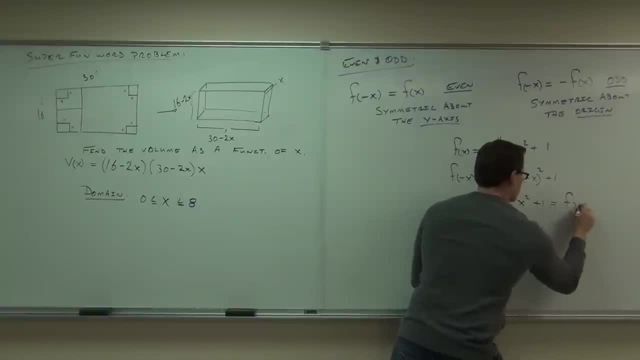 Yeah, This actually equals f of x. If you plug in the negative x and it gives you back out your original function, your f of x, does that mean it's odd or does that mean it's even? This is definitely an even function. 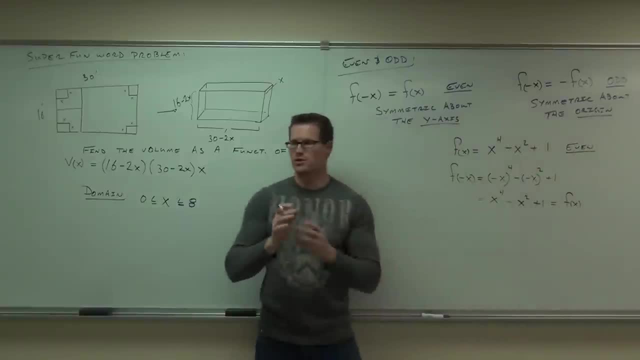 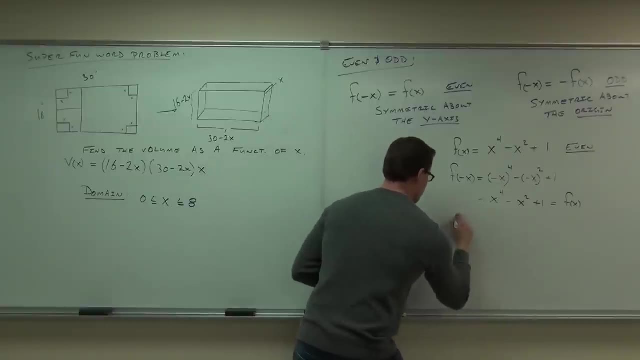 And that's how you tell This is going to be symmetric across the y-axis Mirror image. Gee, I bet you don't know what this one's going to be. Well, I could trick you, I could trick you, I could trick you. 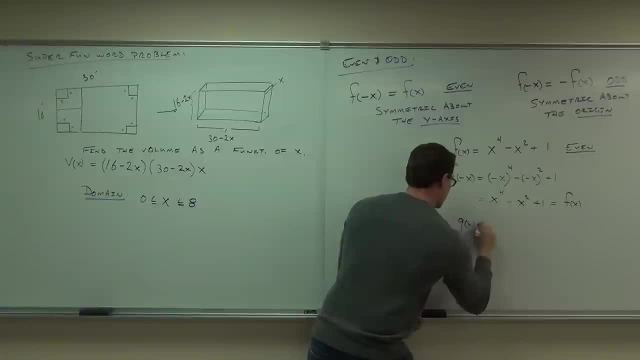 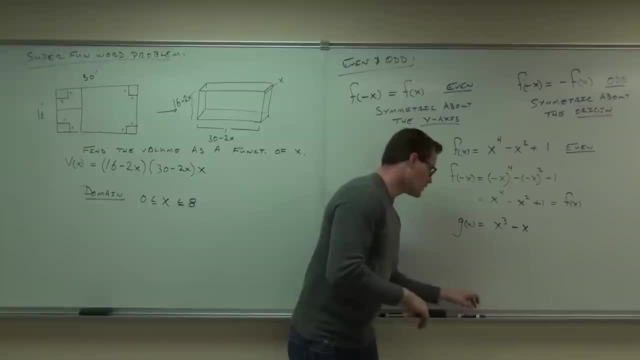 Again to check odd. or even you plug in the negative x. You see what happens. So with our problem we'll have g of negative x, If this says you're just going to take that negative x and plug it in everywhere. you see. 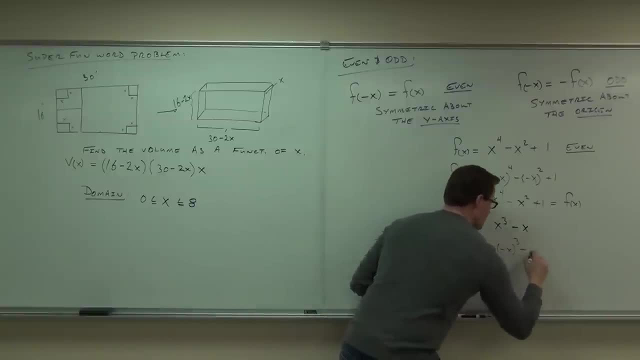 x. So negative x cubed minus negative x, just like that. Notice: negative x cubed. Okay, we got it. And the negative x takes that place. That minus still there, regardless of what you plug in. So that has to make sense. 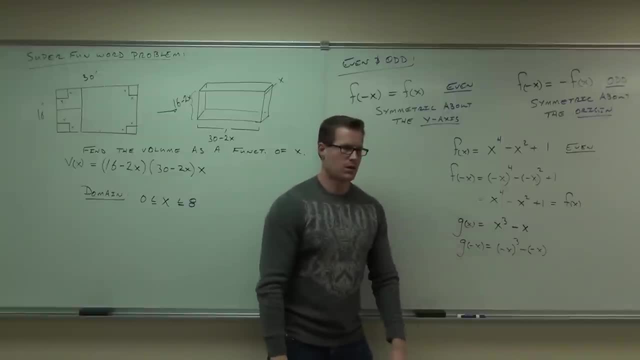 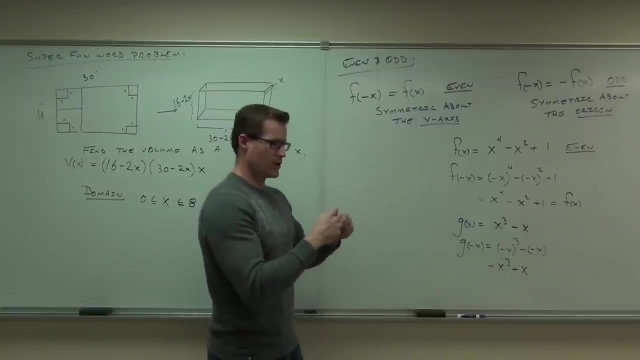 to be there. what happens with this problem? well, yeah, negative, negative X cubed. is that back to our positive X? or do you get a negative X cubed out of that? and this one? yeah, that's for sure. plus, here's how you tell you the the odd. 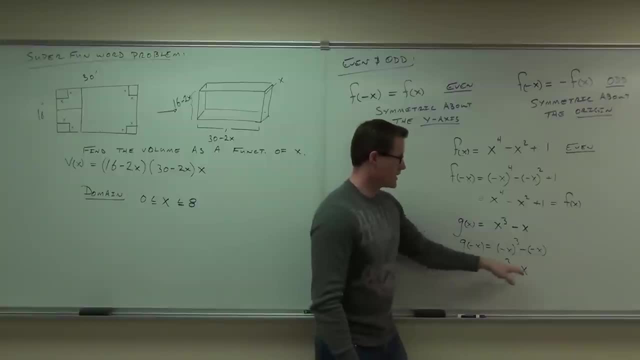 if your every term in your function is opposite of what you started with. that means what you could do is you could actually factor this out. if you factored in negative one, you would actually give me that negative X cubed minus X. do you see how, if I factor out that negative, I'm getting back my X cubed minus X? yes, 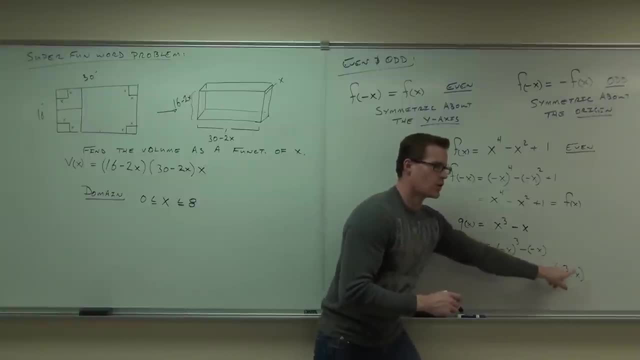 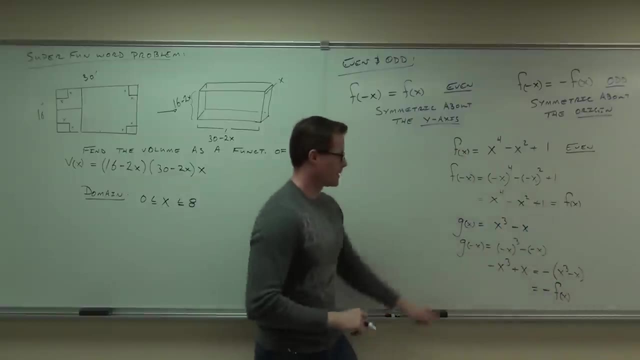 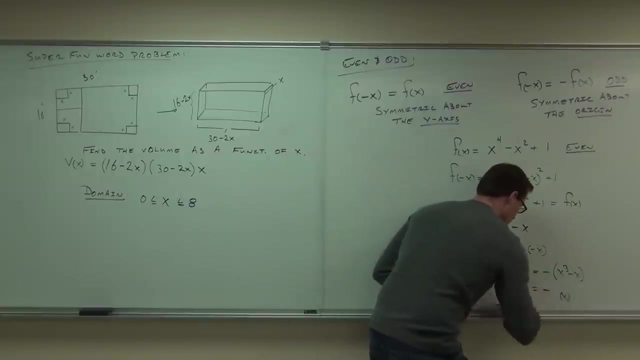 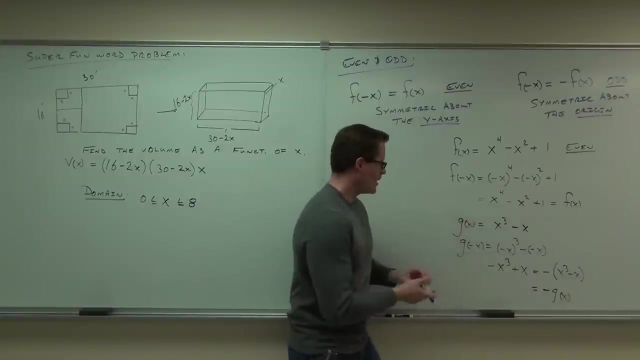 no, this is negative of your original function. this is negative. negative, that's my original. so I now, folks, right, I use an F instead of a G. shame on me. I mark you off two points for that on a test. I really do actually. so be careful that. so if G of X when I plug in 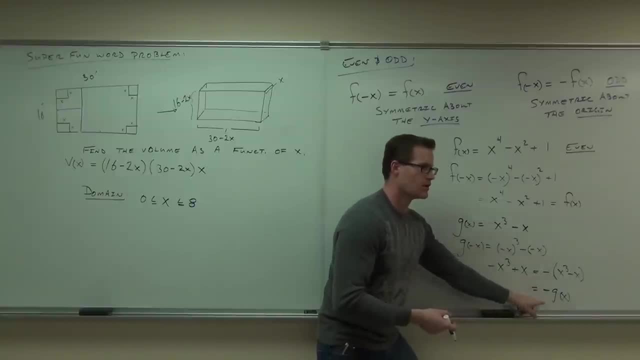 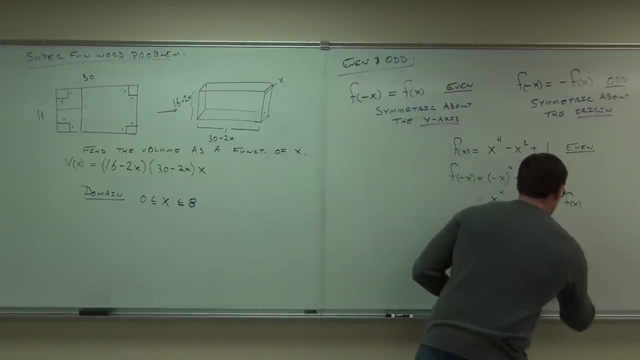 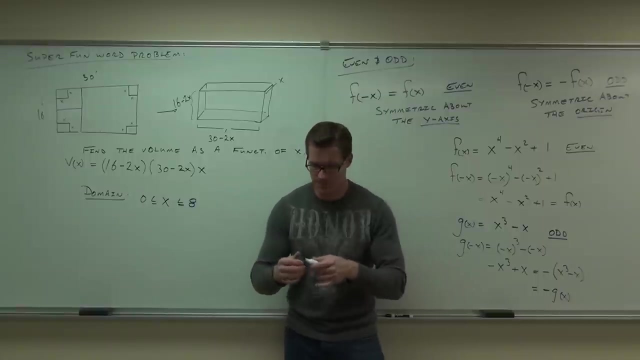 the negative back, negative G of X. that means it's even or odd. what is it definitely odd? it'll be symmetric about the origin. usually s curves are like this: again, have a good understanding that, even an odd concept. now, if you look at what we talked about today, y'all make sense.